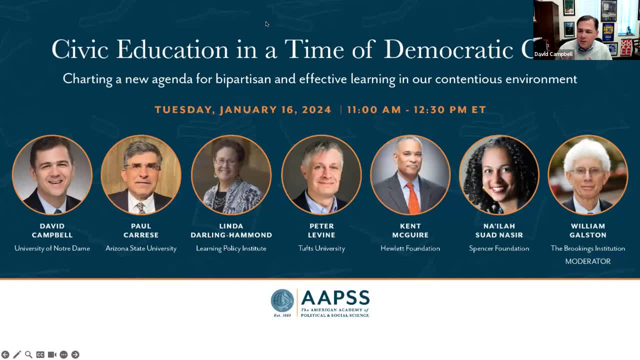 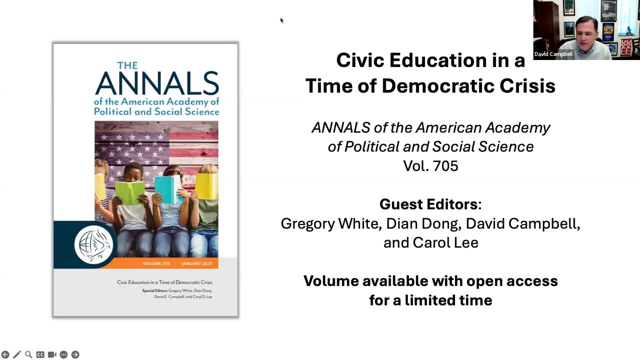 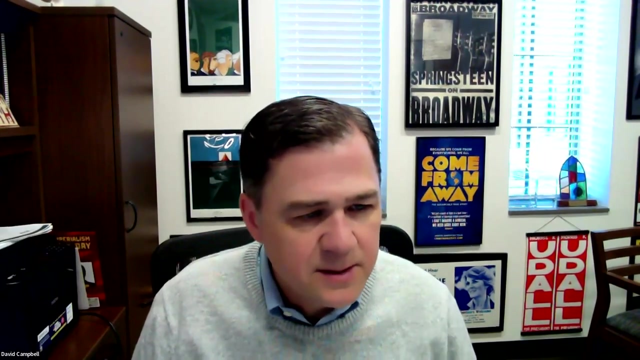 And I'll be sure to highlight the volume of the panels of the American Academy of Political and Social Science. You can see this on the on the screen right now. I'll talk a little bit more about that volume in just a few minutes, But let me begin by introducing each of our panelists, all of whom come to us with considerable experience and expertise and a deep knowledge of the important topic of civic education. 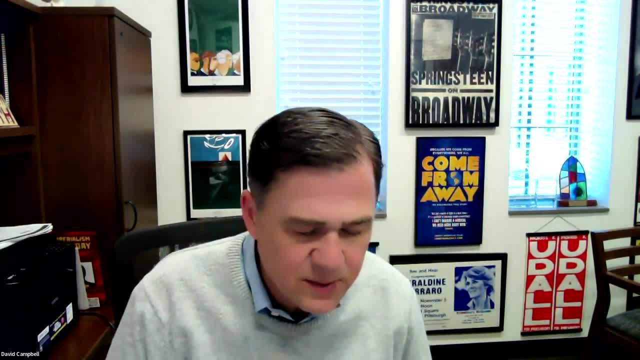 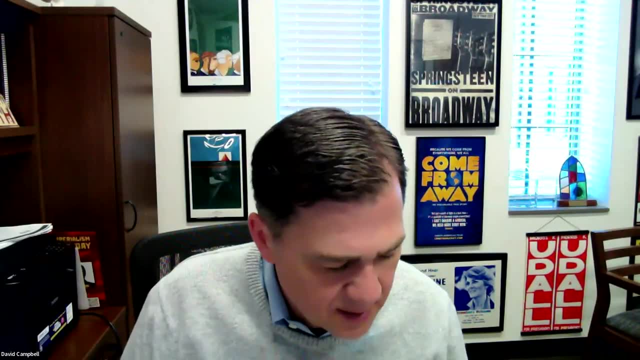 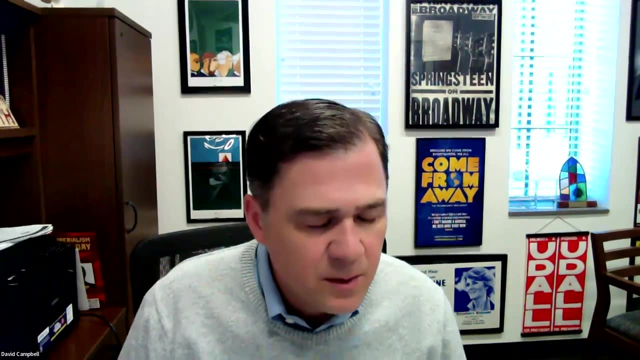 I will begin with Paul Carice, who is the founding director of the School of Civic and Economic Thought and Leadership at Arizona State University, and Paul has been quite active in the field of civic education and we look forward to hearing his comments today. 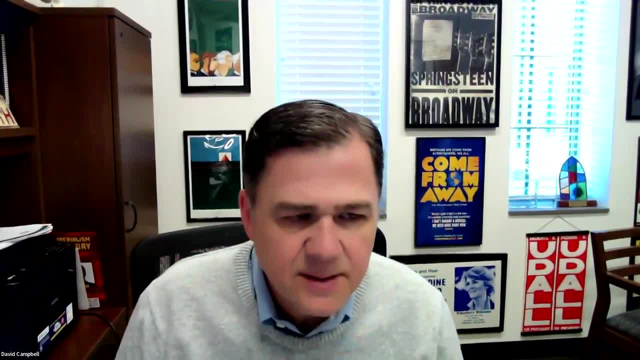 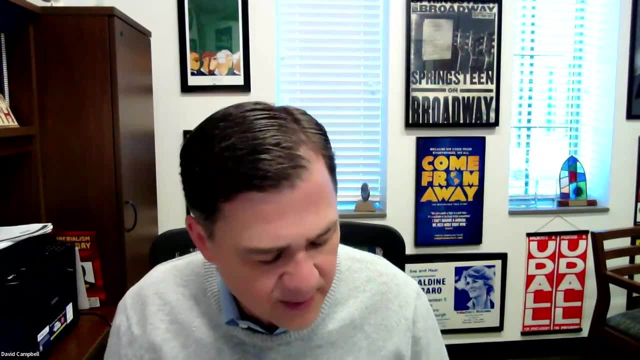 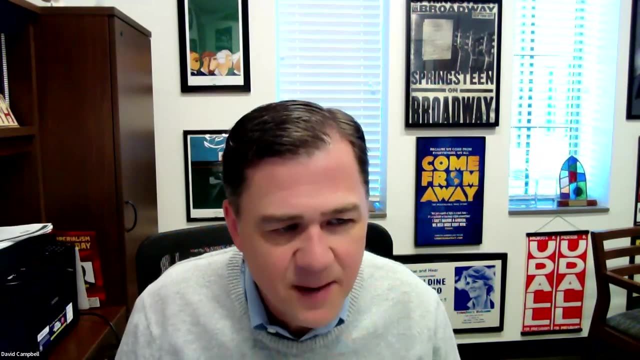 I will move next to Linda Darling-Hammond, who is the president and CEO of the Learning Policy Institute. She's also an emeritus professor of education at Stanford and serves as president of the California State Board of Education. Not sure how she has time to participate in webinars like this, but we're 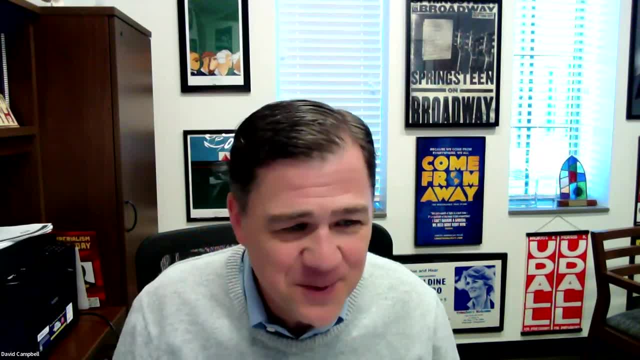 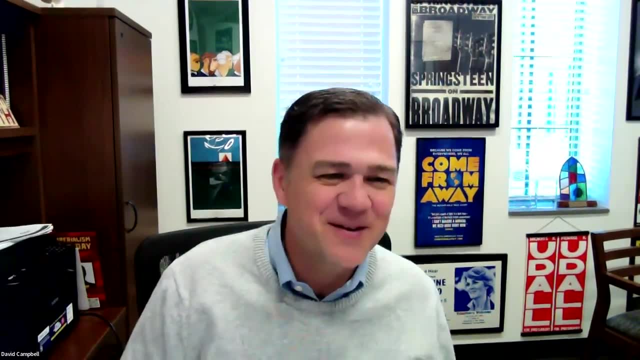 grateful for her, And I should note that both Paul and Linda are participating from time zones far in the West, so it is early in the morning for both of them and we're grateful that they got up early. In fact, I believe the sun is rising as we are speaking. 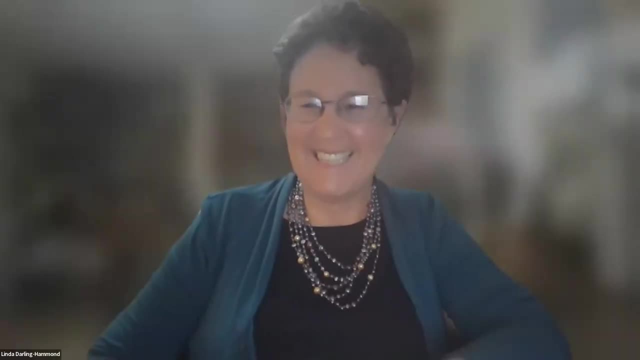 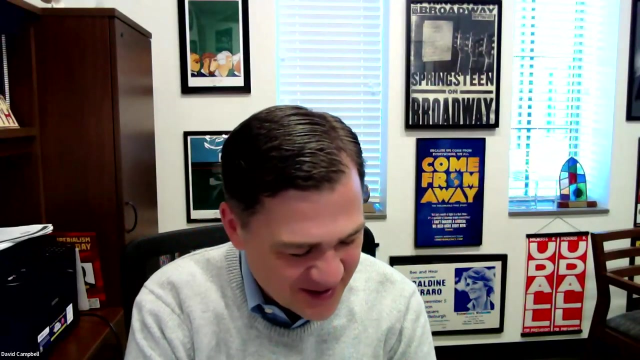 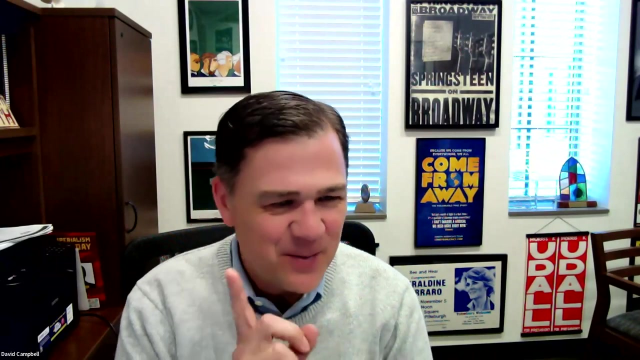 Is that correct, Linda, where you are It is. Next we have Peter Levine, who is the Lincoln Filene professor at Tufts University in their Tisch College of Civic Life. Peter, of course, has done many things in the world of civic ed, but I will put a plug in for his most recent book, What Should We Do? 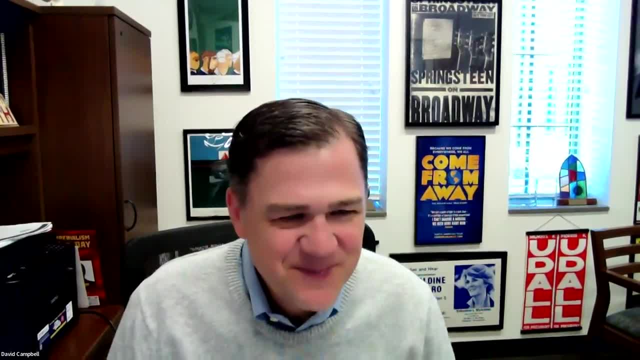 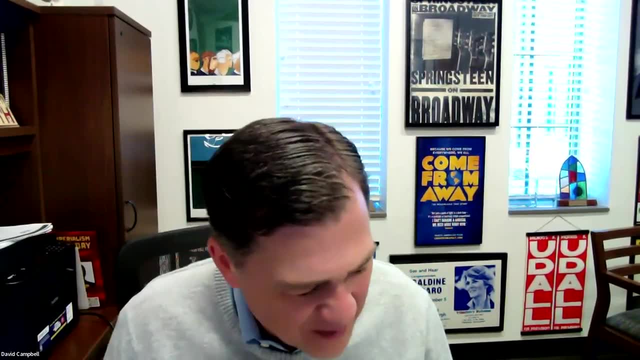 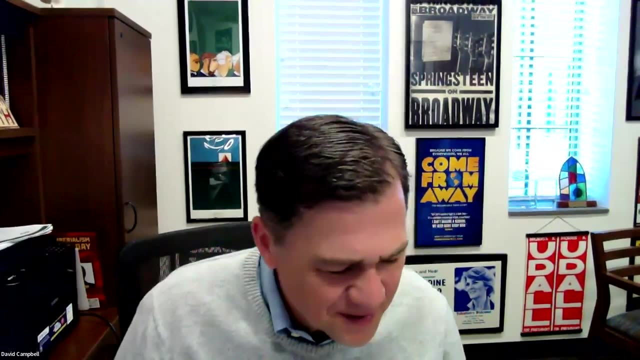 A Theory of Civic Life. I'll move next to Kent McGuire, who is the program director of education at the William and Flora Hewlett Foundation, which of course has been an important source of funding and a voice just very active in the field of civic education. 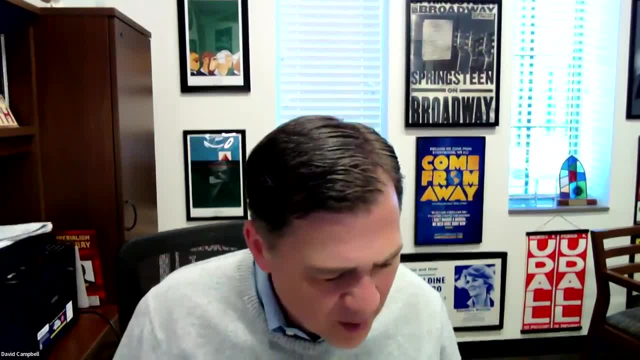 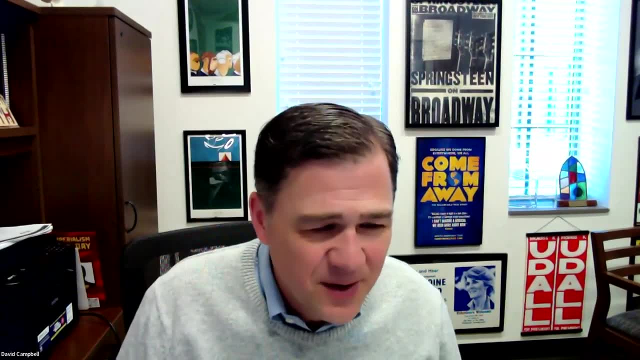 He's done a variety of things in philanthropy. He's done a variety of things in philanthropy and academia, but worth noting that he was the assistant secretary of the US Department of Education from 1998 to 2001,, and so comes to us with that background as well. 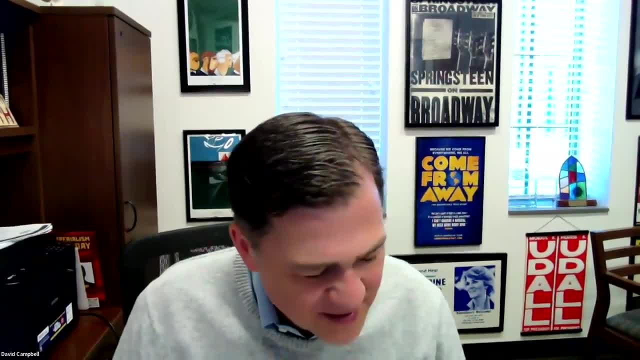 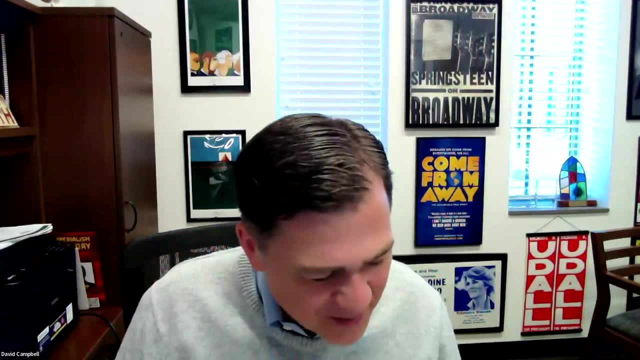 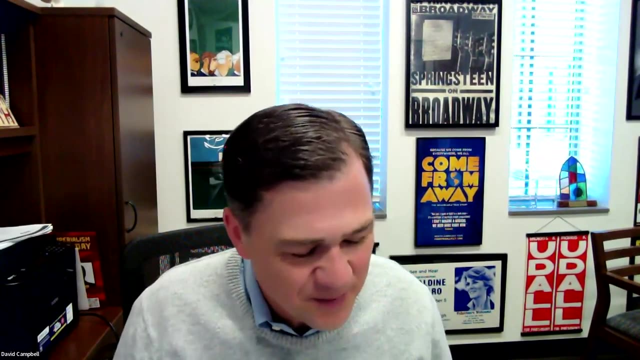 And last but not least, we have Naila Suad Nasir, who is the president of the Spencer Foundation, although she also has a background in academia, with appointments in education and African American studies at Berkeley, and she served as a vice chancellor there as well- for equity. And last but not least, we have Naila Suad Nasir, who is the president of the Spencer Foundation, although she also has a background in academia, with appointments in education and African American studies at Berkeley, and she served as a vice chancellor there as well- for equity and inclusion. And last but not least, we have Naila Suad Nasir, who is the president of the Spencer Foundation, although she also has a background in academia, with appointments in education and African American studies at Berkeley, and she served as a vice chancellor there as well- for equity and inclusion. 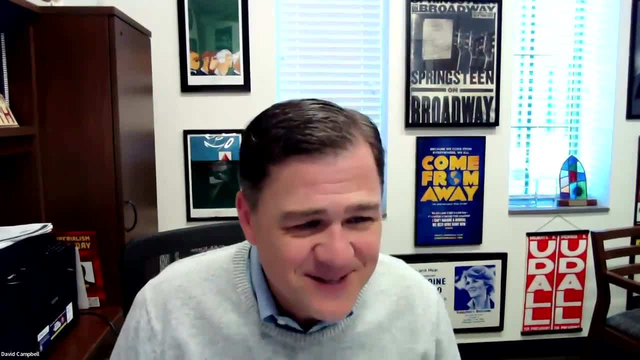 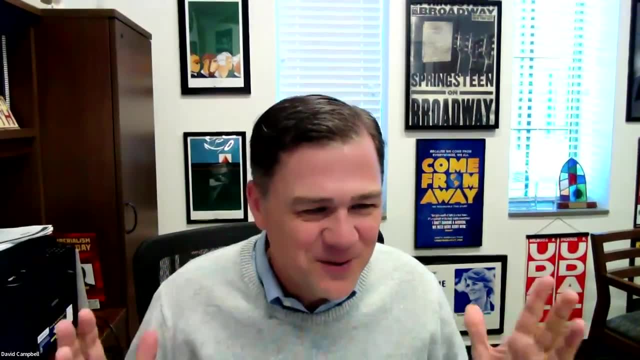 There's, of course, much more I could say about each one of our panelists, and I hope they will forgive me for not going over all of their many accomplishments, but I can assure all of those who have assembled for our webinar that these are folks who know what they're talking about. 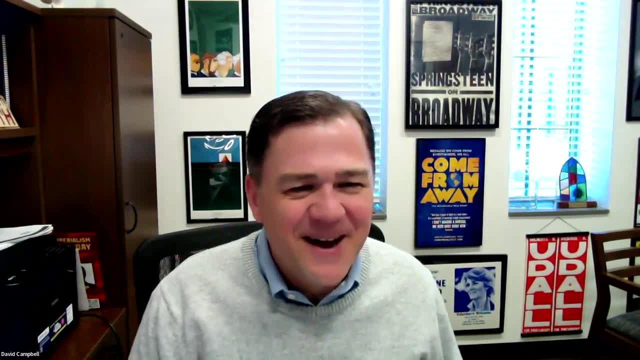 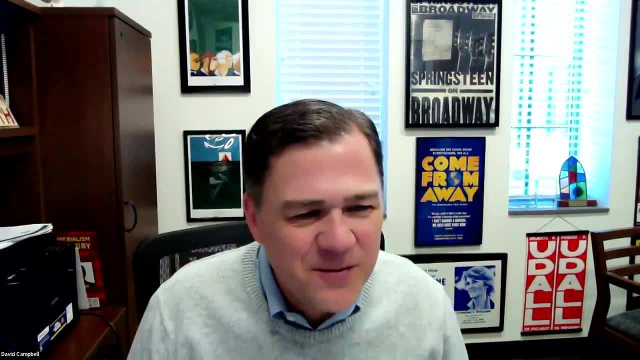 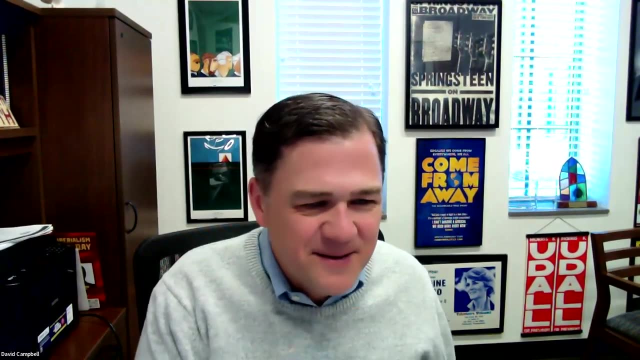 And what are we talking about? Well, let me address just for a moment what has brought us together here, which is this special issue of the Annals of the American Academy of Political and Social Science. The title of the volume is Civic Education in a Time of Democratic Crisis. 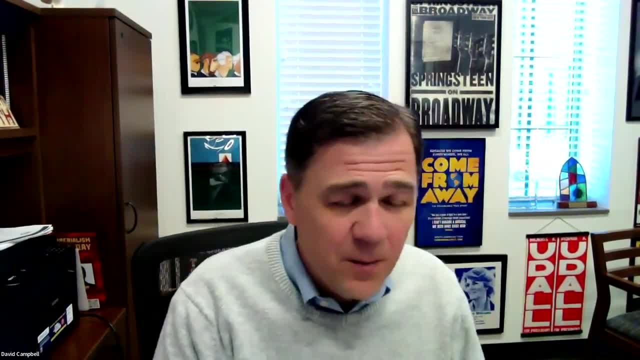 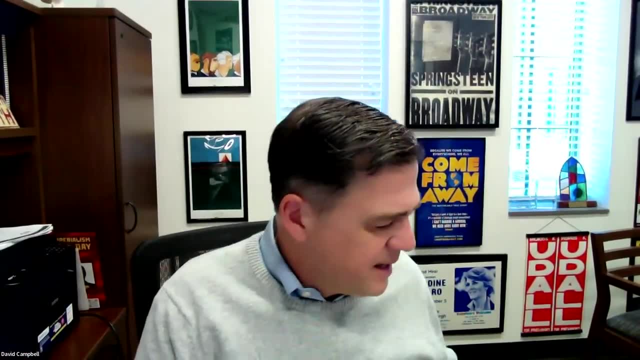 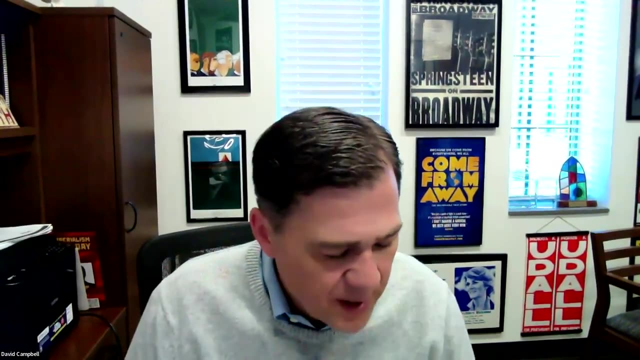 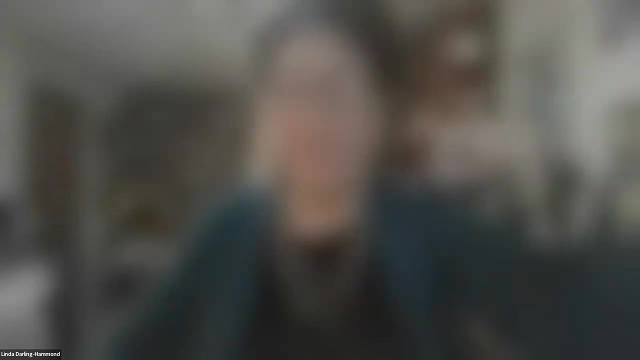 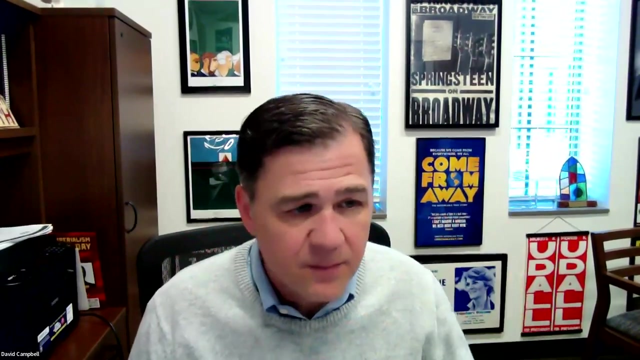 And just by way of background, you should know that this volume actually began with a report from the National, The National Academy of Education on the topic of educating for civic reasoning and discourse, and that gives me an opportunity to acknowledge the tremendous work of Carol Lee, who I don't believe is with us today, but also Greg White and Diane Dong from the National Academy of Education, who have been their co-editors in the volume but more than instrumental in pulling this all together. 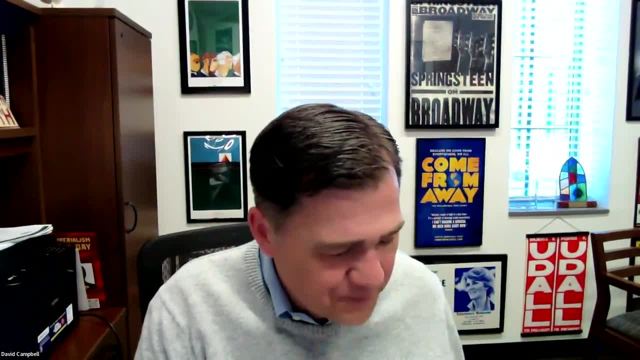 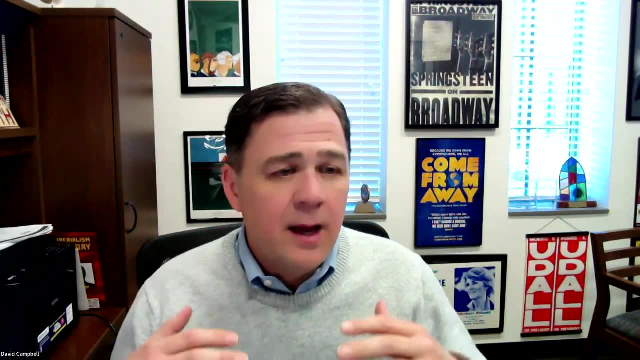 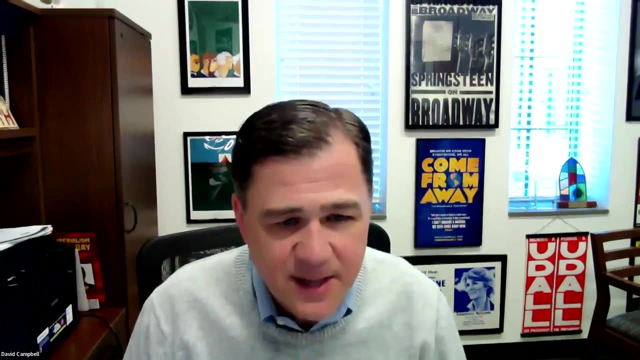 And so I'm grateful for For their work as well. You should all know that the volume on which this is based is available to the world for free for roughly the next month or so. It's a limited-time offer, but if you're interested in learning more, digging deeper, you can consult the volume. 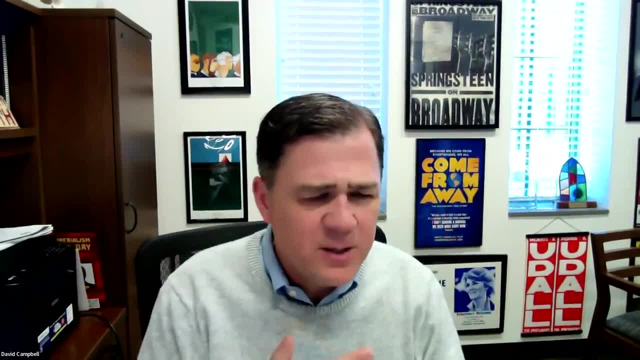 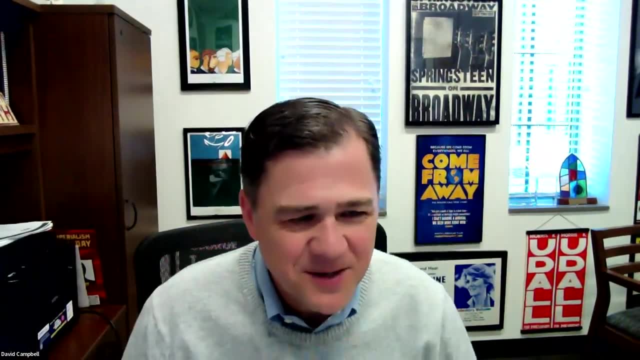 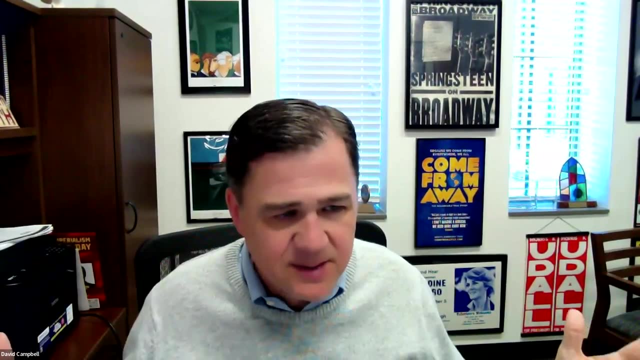 You can find it online. We encourage you to read it, to engage with it, to cite it, to assign it. We want this to be Really an opportunity for people to dig deep into what many of the leading scholars across different disciplines have to say about civic education at this polarized time. 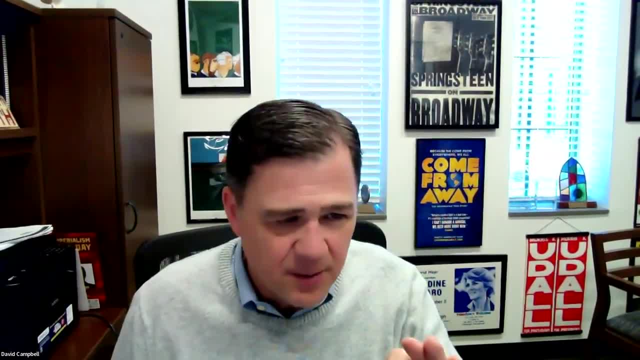 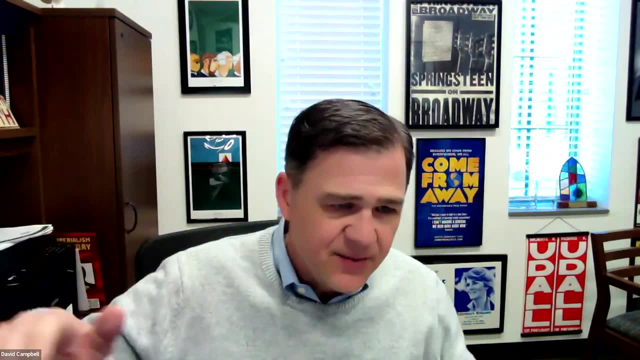 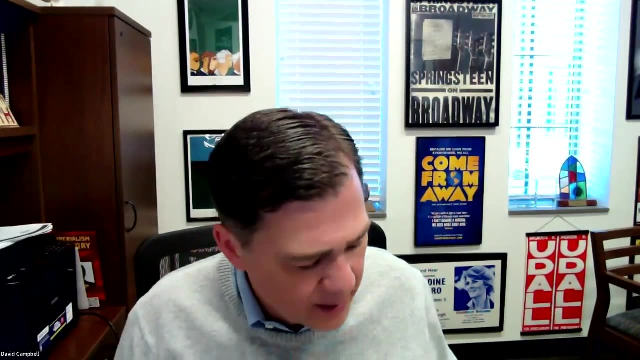 And I do want to emphasize that the whole idea behind the volume is that it actually spans multiple disciplines, So people from education schools and political science and sociology, and just a variety of disciplines, each of which have, I think, an important contribution To make to civic education. 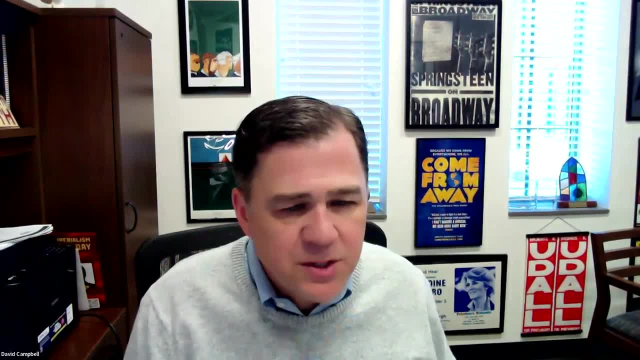 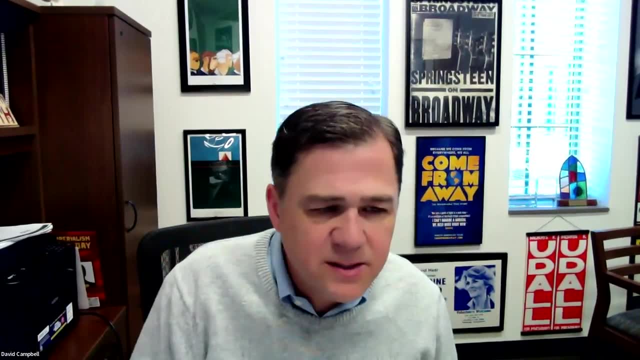 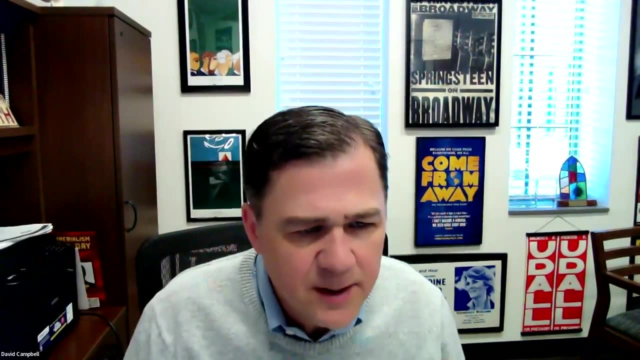 With all of that out of the way, I think we should move to talking about civic education. So the way this will work is: I will pose some questions to get us started to our panelists, We'll continue with that discussion for a while, for roughly 50 or so minutes, and then we'll have some Q&A from the assembled audience. 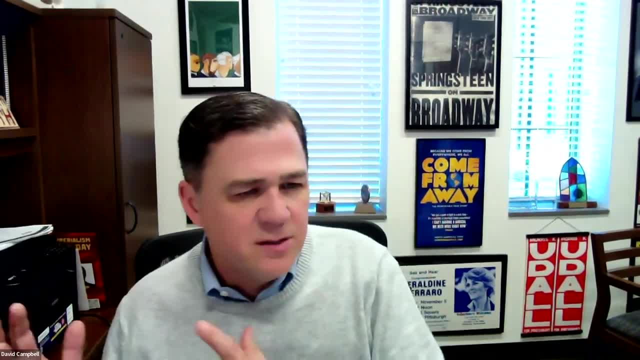 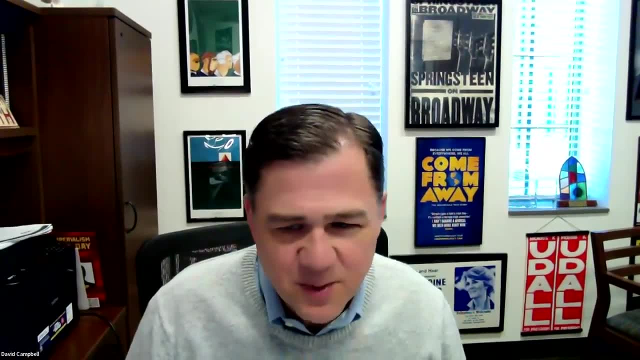 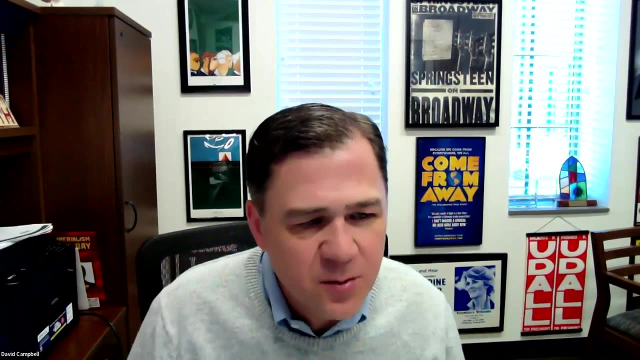 Now, this being a webinar, not a conventional Zoom Session, means that we, as the panelists, cannot see those of you who are participating, So it's a little bit like, I suppose, being on a radio show, But you do have an opportunity to pose questions to us through the question and answer box. 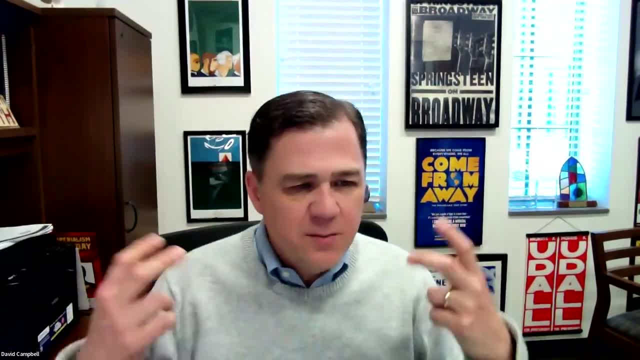 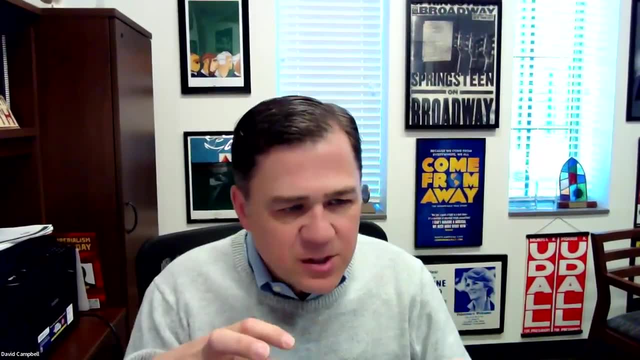 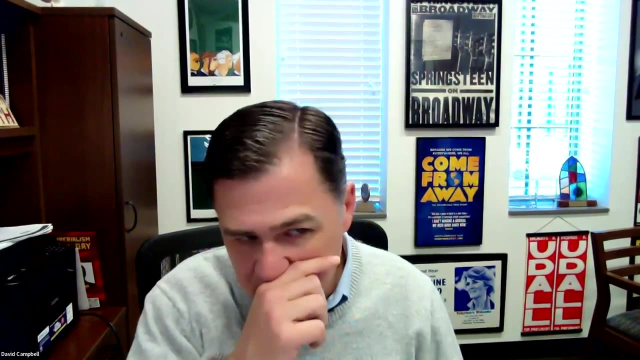 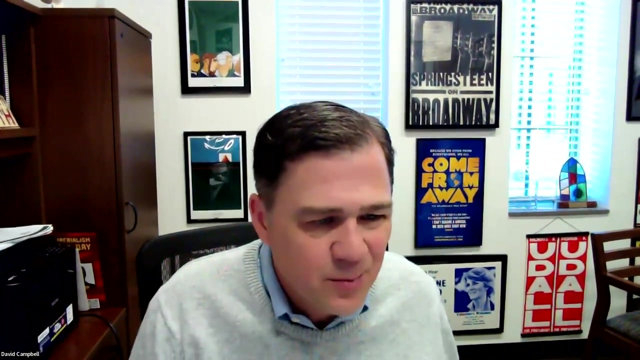 Those will be moderated, so they will be fed to me and then I will pose them to the panelists, And there will probably be points at which we will combine questions or try to synthesize what people Are thinking and saying. So just keep that in mind. when we turn to the Q&A session, you will pose your questions again through the question and answer box provided there on your Zoom interface. 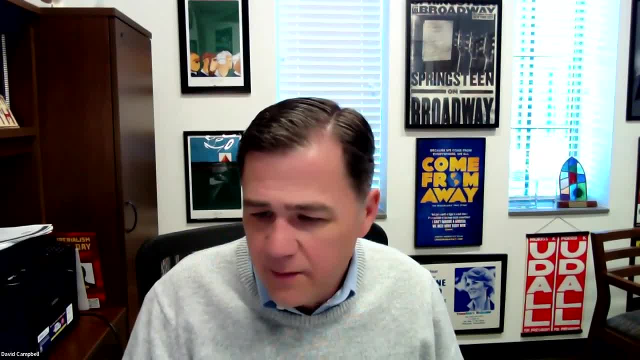 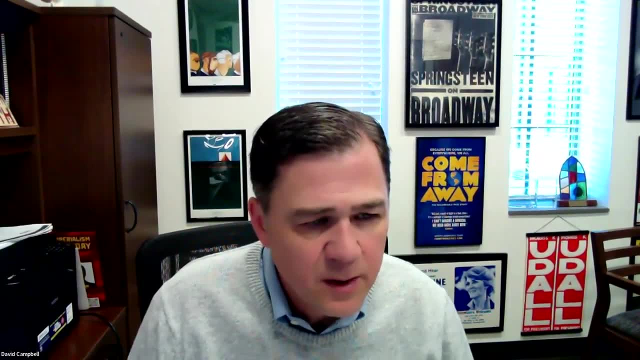 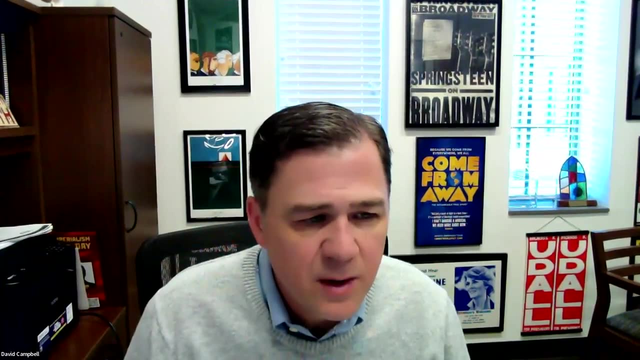 I'm just looking here. we We've had the link sent to us as the panelists. We've had the link sent to us as the panelists. We've had the link sent to us as the panelists. If I could ask maybe one of the panelists to figure out a way if we can send the link to the volume to everyone listening to the webinar? that would be great. 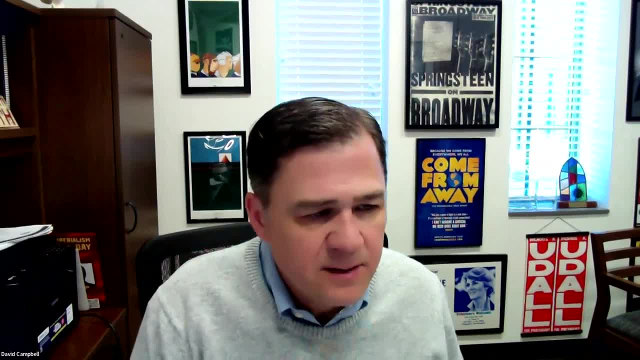 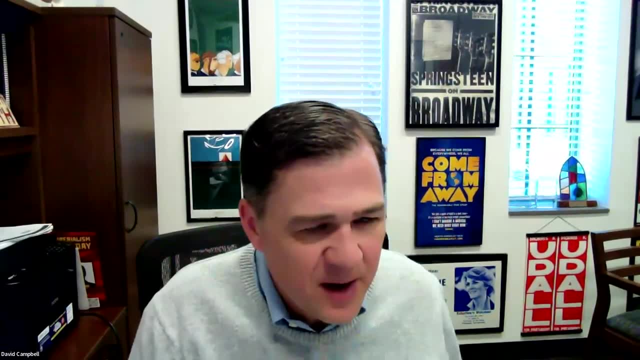 All right. so as we get started, let me just remind everybody who might have joined us a little late that I am not Bill Galston. I am instead Dave Campbell and I'll be serving as the moderator. Just a little bit about me. I'm a professor at the University of Notre Dame. 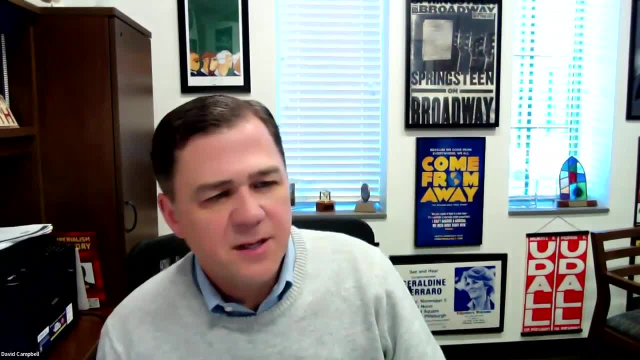 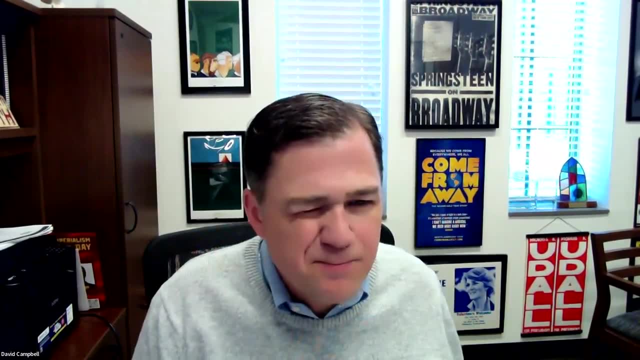 Just a little bit about me. I'm a professor at the University of Notre Dame And I've written a little bit about civic education and democracy and social capital and such things over the course of my career. But my job is primarily here to serve as the moderator. but I may interject some of my own thoughts along the way. 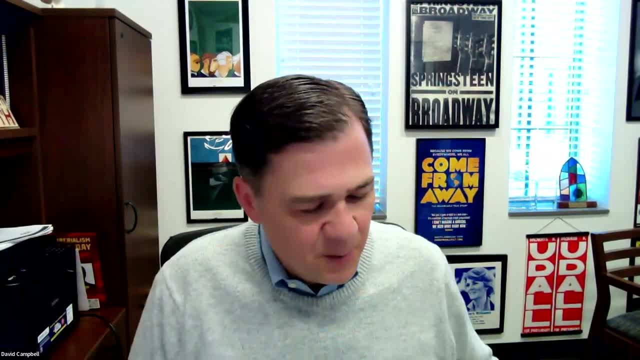 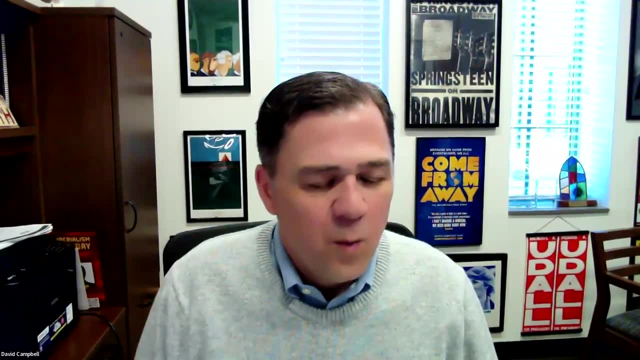 But my job is primarily here to serve as the moderator, but I may interject some of my own thoughts along the way. I may not be able to resist, But let's start. I'm going to start with a question about. I'm going to start with a question about. 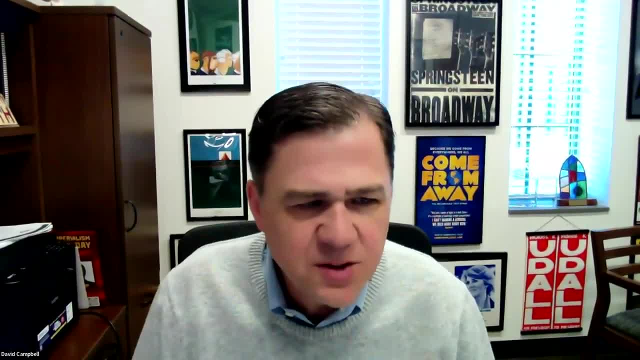 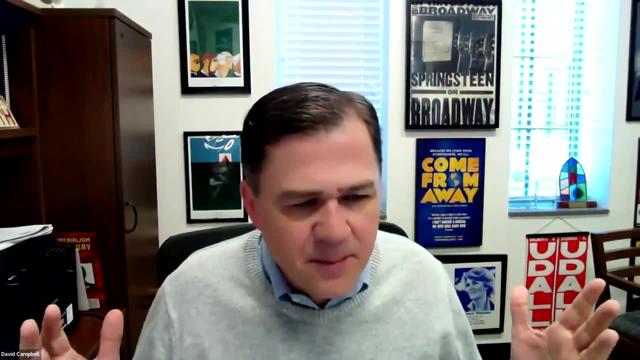 renewed civic education. We're at a very interesting point, I think, for those of us who care about civic ed. seems to me there's a lot of attention being paid to this topic across the political spectrum, from policymakers, from educators, from the general public. 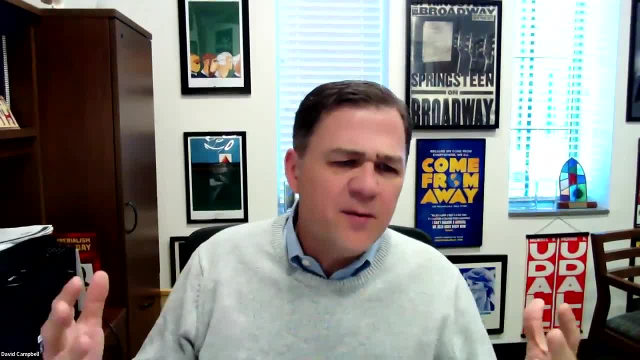 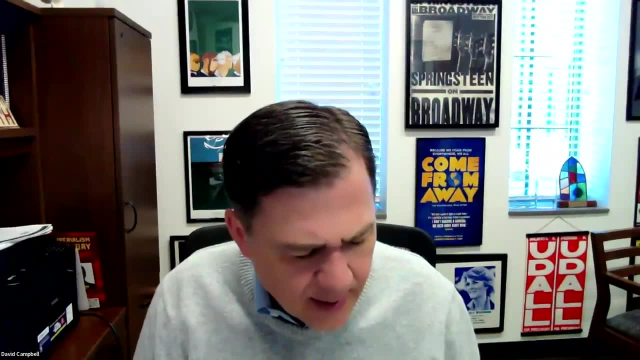 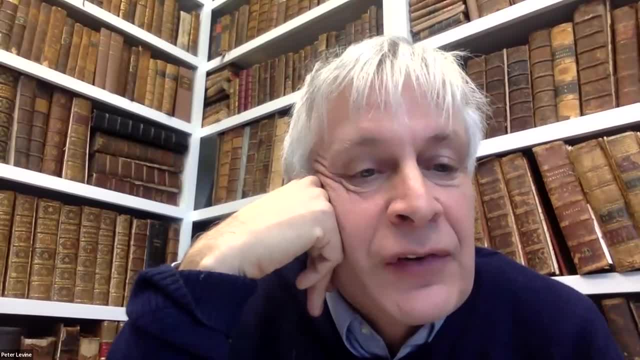 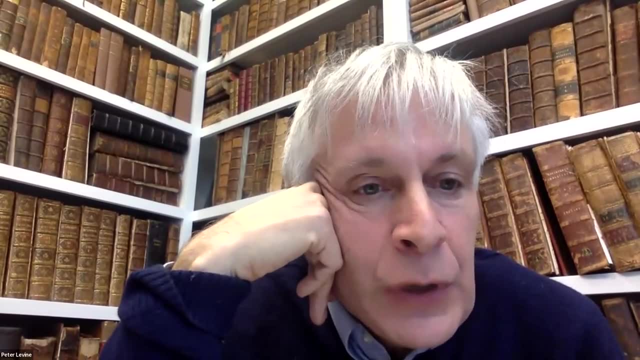 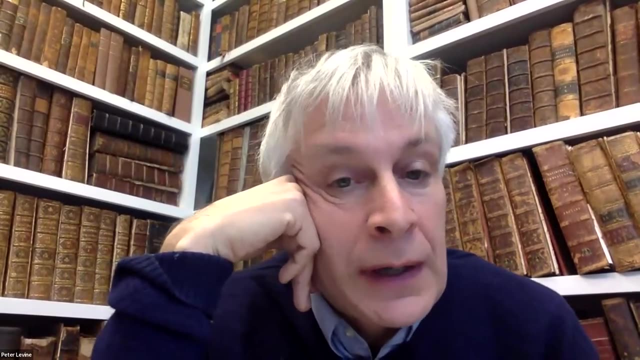 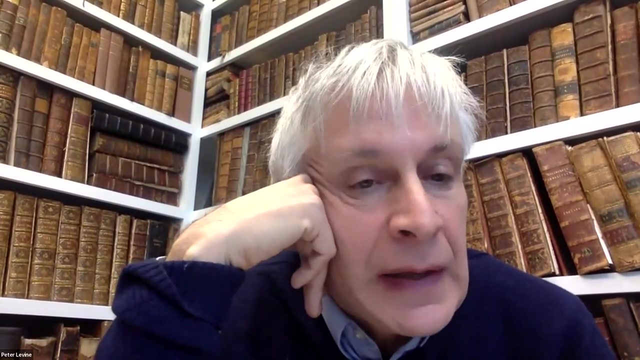 I mean, this is a this is a challenging Question, so there's not a slam dunk easy answer. I think it Part of it is- is an affirmative statements by prominent people, and also by Kemper, And also by bipartisan groups that say that addressing controversial issues and school is actually something that we want, because we want to teach Civility and civic friendship, which is the term that we use, and you can't really do that if you marginalize anything that people 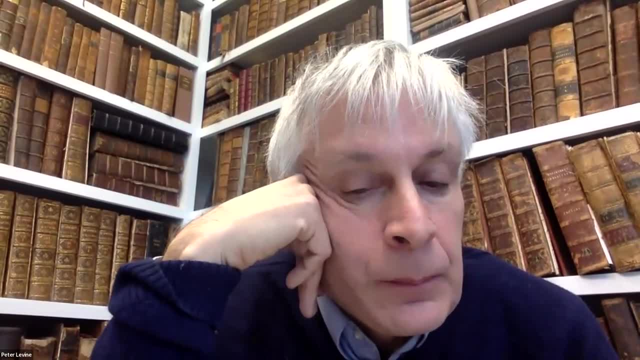 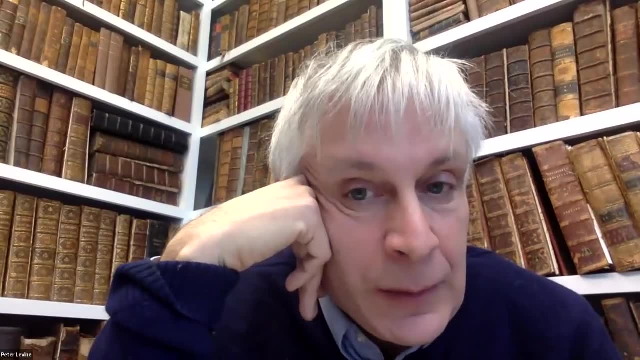 disagree about, And you can't really do that if you marginalize anything that people disagree about. and freedom of speech is of value, And one of the ways that this plays out is that when a conversation in a school goes badly, at least by some people's lives, but sometimes it just really does go badly. 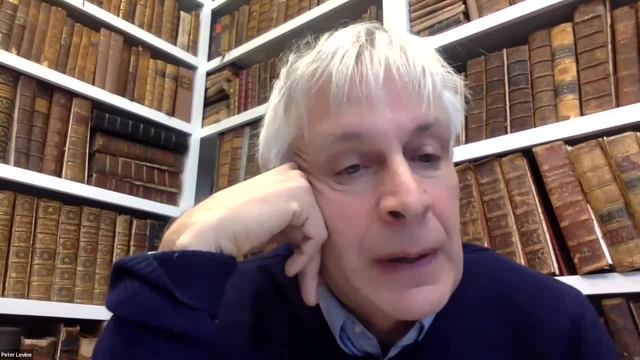 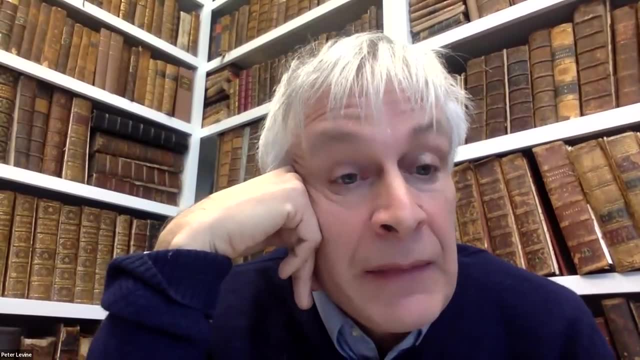 that makes news and that becomes a controversy, And the takeaway is that maybe we shouldn't have schools dealing with these issues at all And very few people ever say: but we want students to talk about art issues, Then in order to have that go well, there has to be good professional 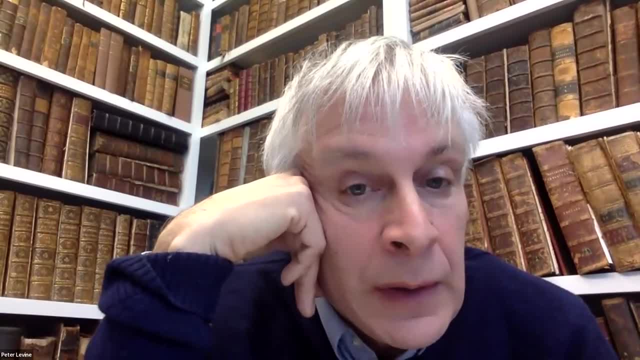 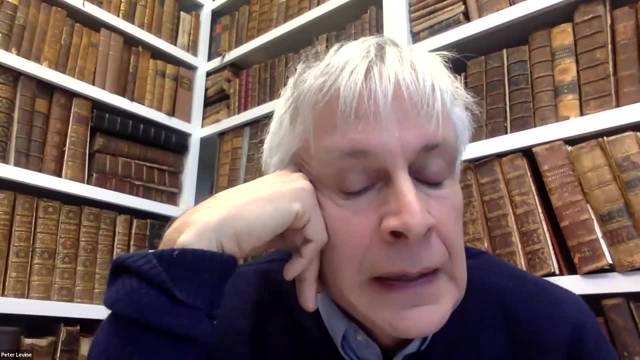 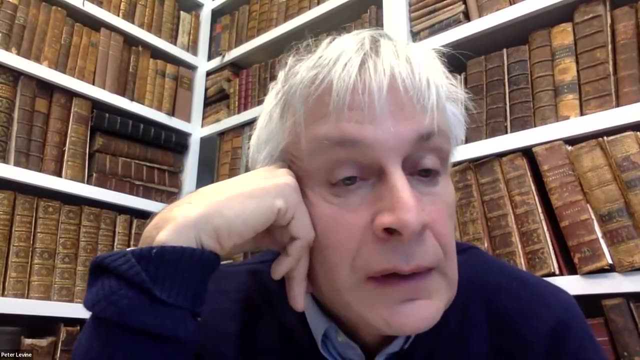 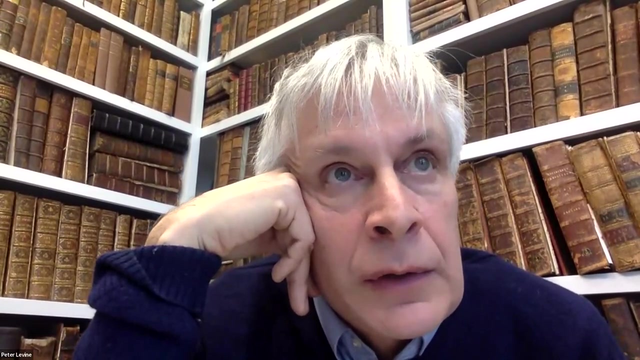 development, because it's actually very challenging to moderate a discussion of a controversial issue with children or adults. Well, children or adults, yes, but also adolescents, And you can learn about that, And we also need school district and state policies that are supportive. Dave, I also wanted to sort of say something quickly about your original question. 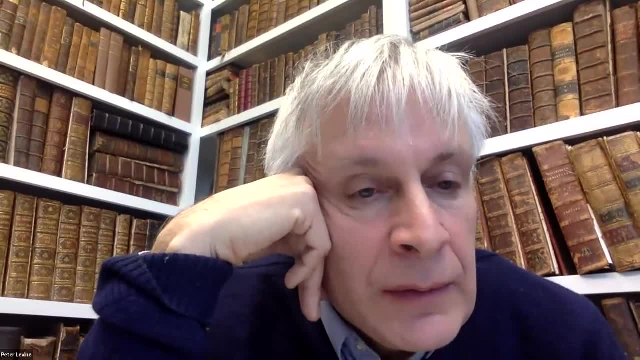 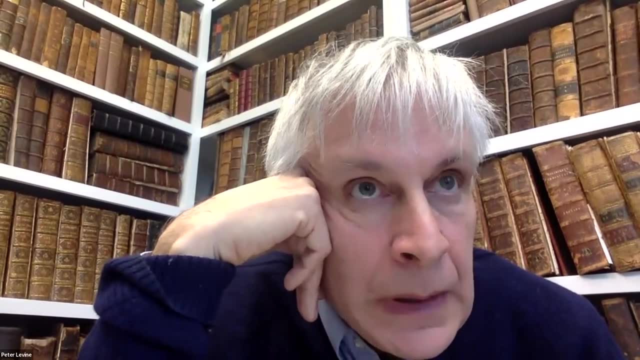 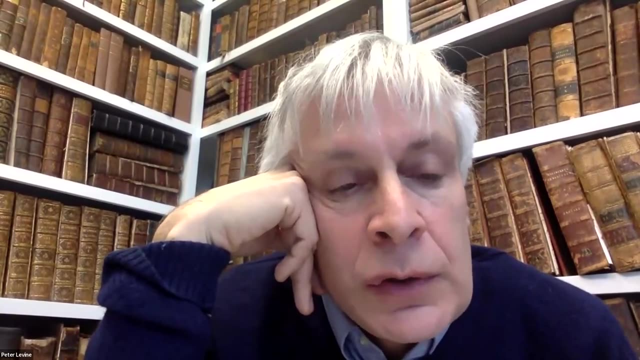 which is about sort of what are the lines of disagreement within the civics field, And you posed a kind of action versus understanding or knowledge. I think that's real. I think there's a kind of continuum between people who are very enthusiastic about experiential 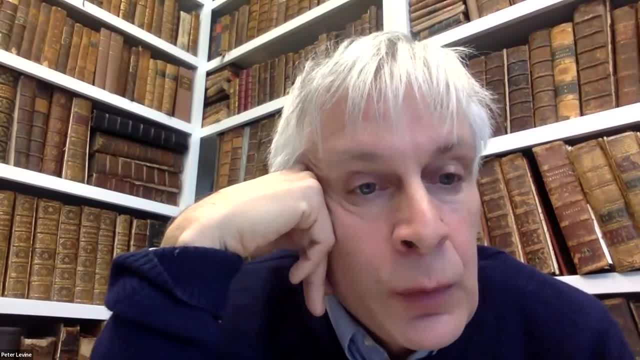 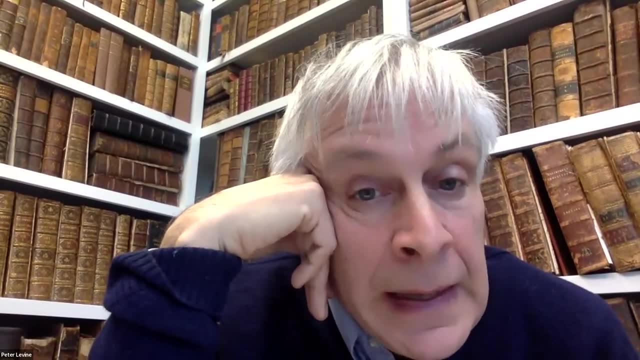 learning and getting your hands doing the work, and people who believe in sort of theory and academic study and books and articles and things like that. That doesn't map onto right or left, It really doesn't. That crosses. I believe that just is completely wrong. 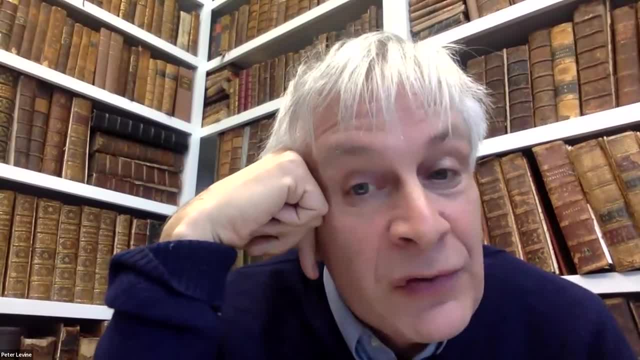 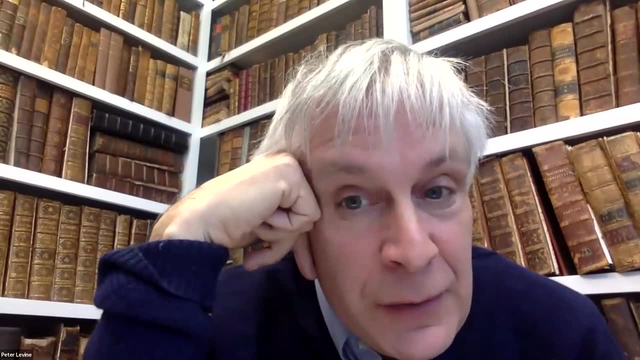 It's completely orthogonal to the right or left distinction because, for example, if critical race study theory was really taught in schools- which it pretty much isn't, but if it was taught it would be- it would be theory. It's called critical race theory for a reason: It would. 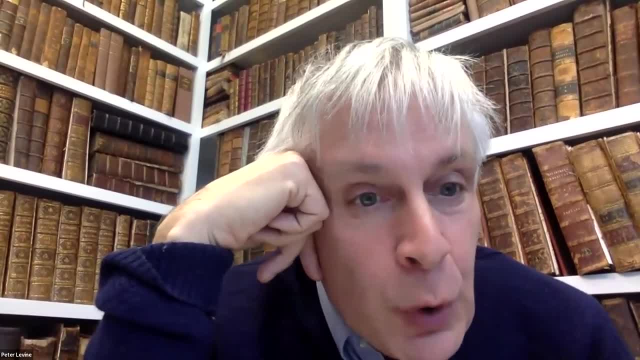 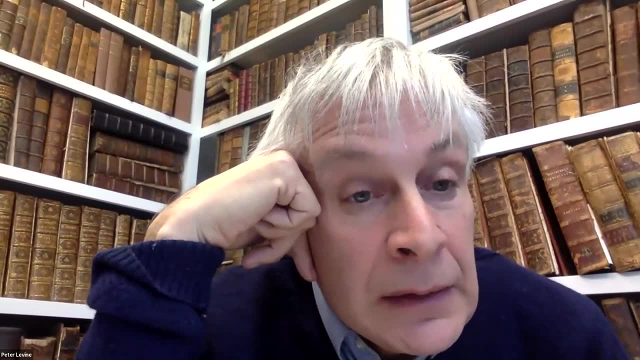 be reading Du Bois and Kimberly Crenshaw- And you know it would be books and articles in the past. And then on the other hand there's that kind of you know let's serve in our local community to understand how local community works. That's very conservative. at least little C's conservative. 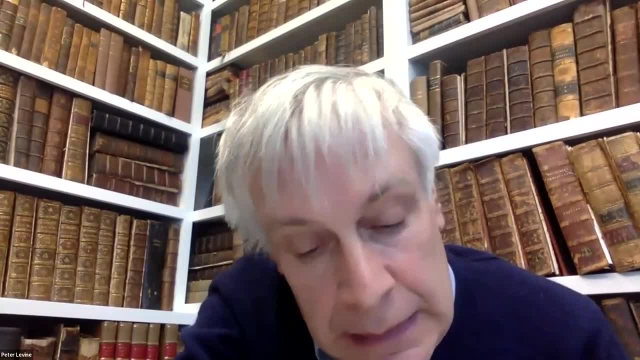 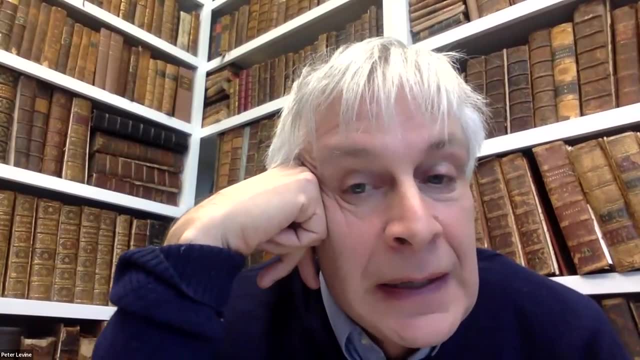 It's very So. so that's A distinction, though, between more academic and more experiential. I mean with Na'ilah I would like to say both, but especially over a K-12 curriculum. you have a lot of time. 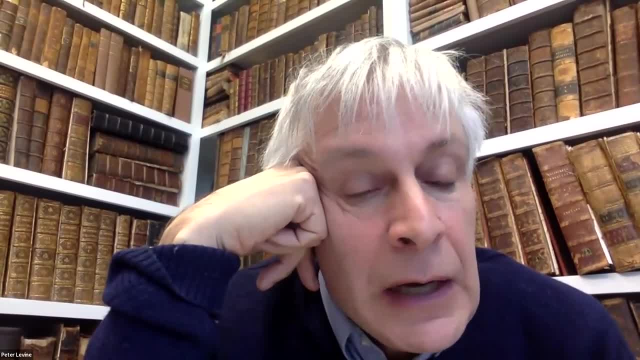 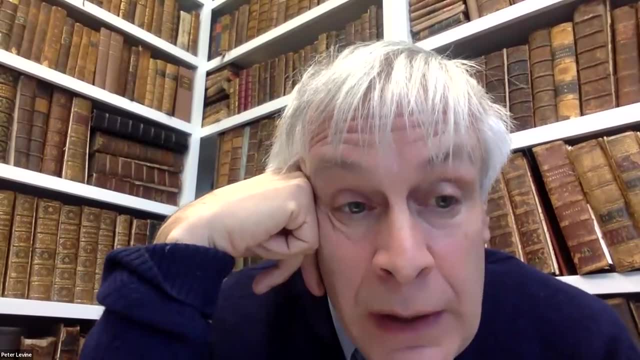 Another distinction that's underneath things, I think, is sort of how, how pro pro system versus how critical people are. That also doesn't exactly map onto right or left, because you have people on both right and left who are anti-system. Perhaps the place where people are most pro. 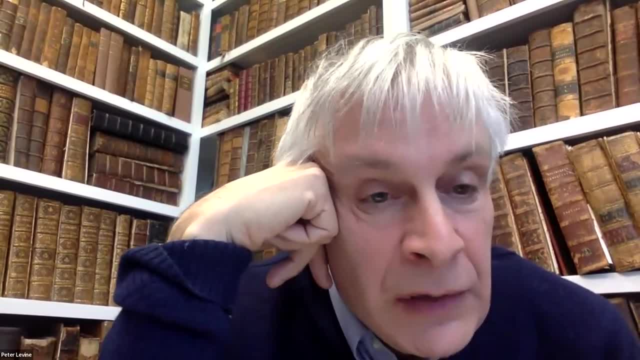 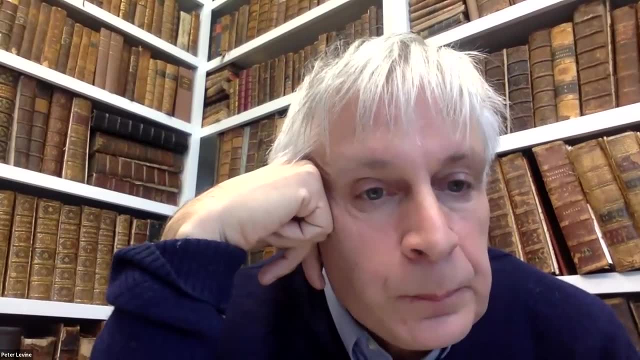 system is in the middle, in the center. But Anyway, reasonable people can disagree on how pro or anti-system they are, but that's percolating underneath And you know, I, I, so I think we sort of have to. that's the kind of thing you have to deliberate about if you're 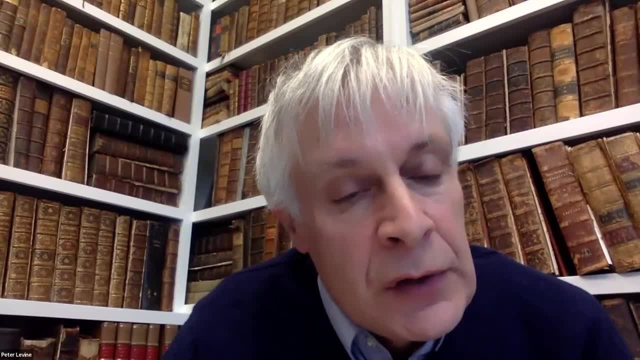 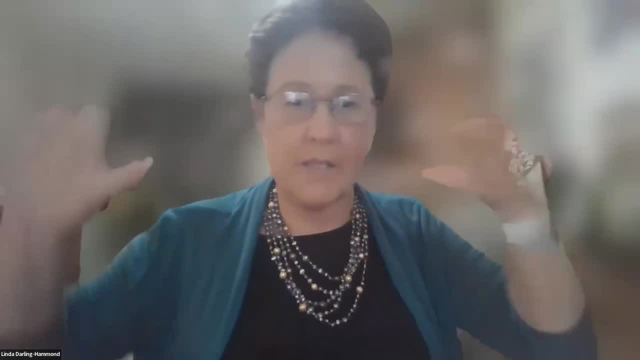 actually trying to figure out a policy or a curriculum or a textbook or anything that is an intervention here in this area. But I'd love to put in a word for disciplined inquiry. You know, sometimes there's sort of this notion that you're off doing something experiential and 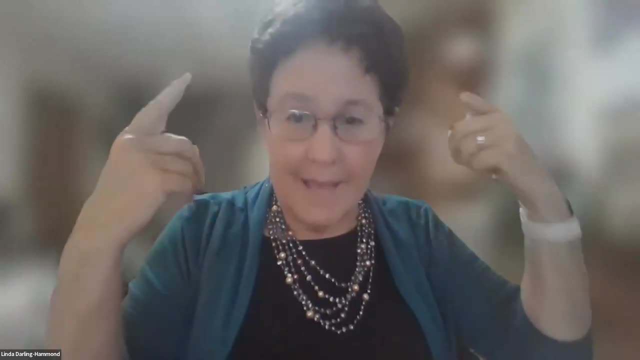 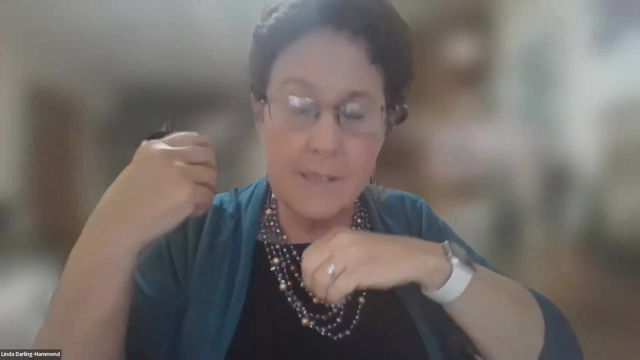 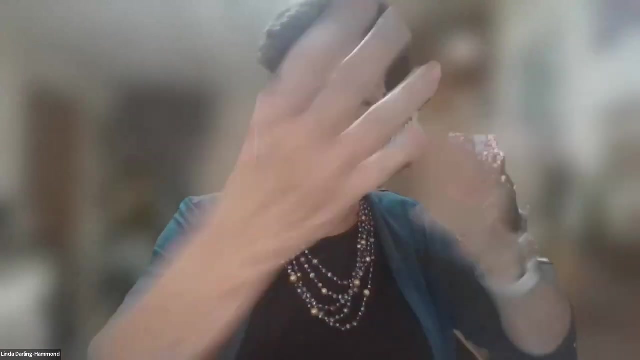 you're otherwise, you're studying things, But there's a, A habit of mind that you want to develop in in young people. that has roots in how they can listen and read and look at and analyze evidence and think about what the evidence suggests and then 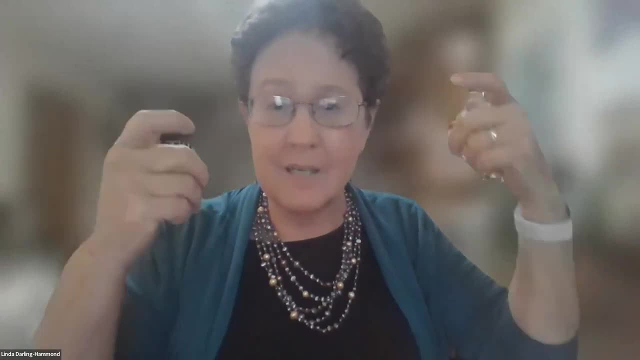 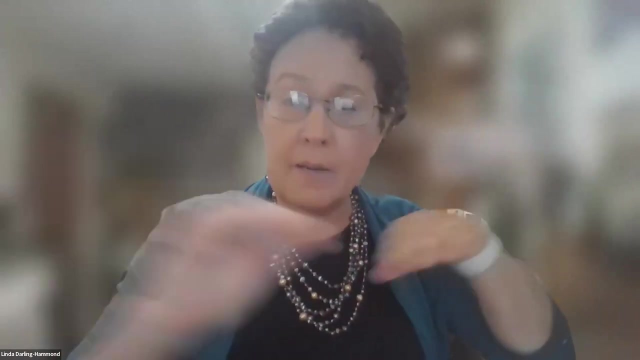 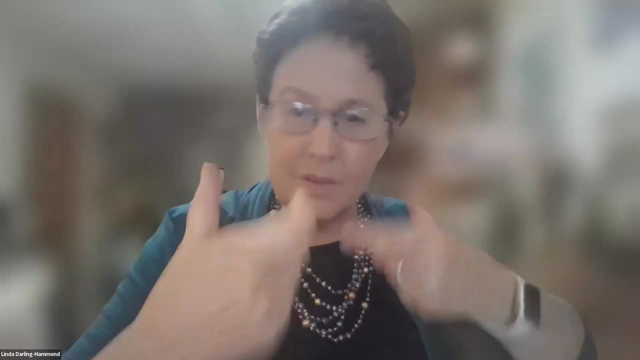 hear other evidence from others and then analyze. you know the ways in which those agree or disagree. The schools now that are beginning to do conflict resolution and cooperative learning, training across the school in every subject area, are helping Students learn how to listen, you know, to each other. learn how to bring evidence to bear, modes of 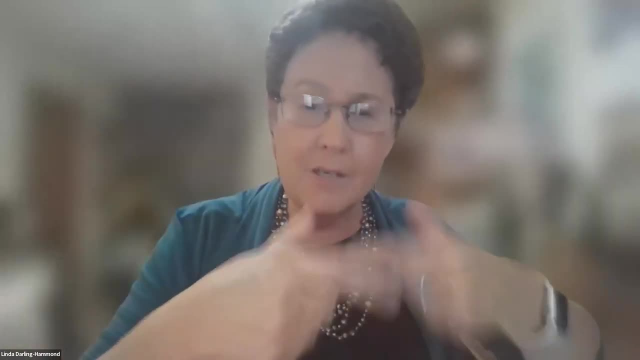 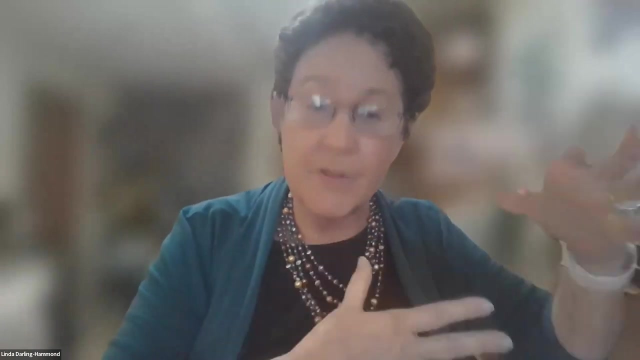 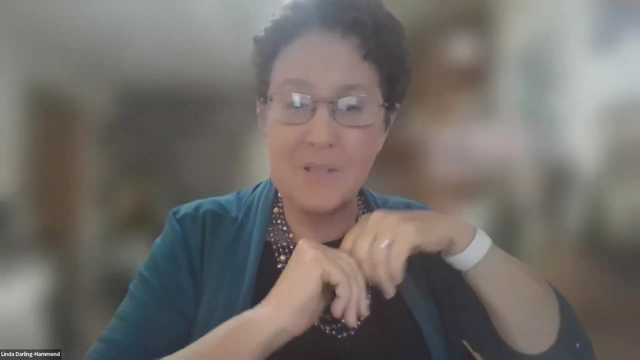 operation that can help people get to consensus are actually a discipline of their own that enable people to think things that you know. hear each other speak, you know, think about what each other have said. I, you know, I appreciated the little exchange between Paul and Peter about who's right and who's 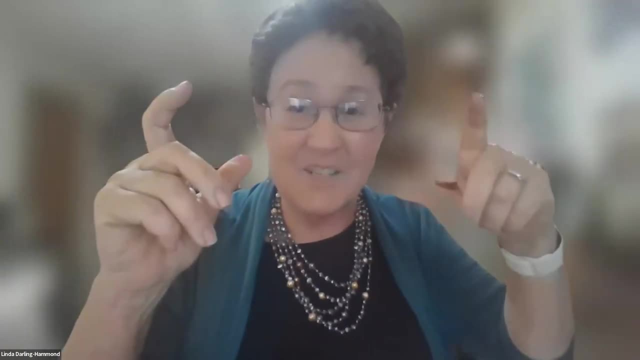 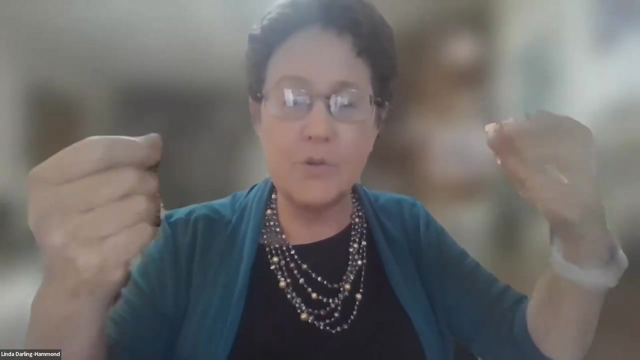 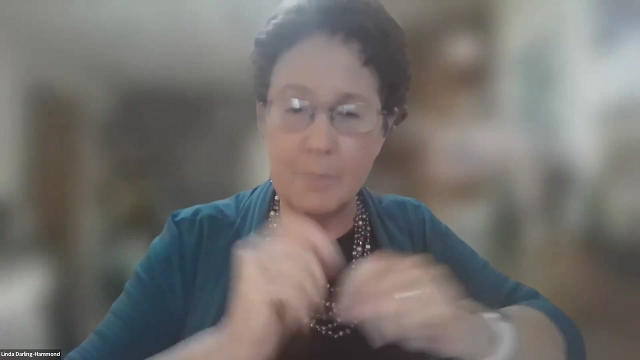 wrong, But I'm quite Sure that in the course of discussions that you've had, there has been some attention to the points of view and some consensus building, and learning to do that is a skill in itself that should be developed in every content area and every part of the school and in every part of the experience. 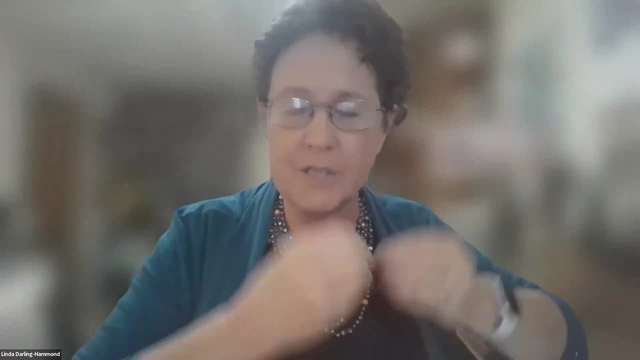 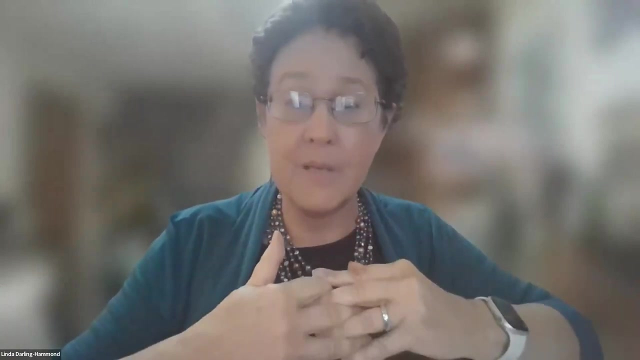 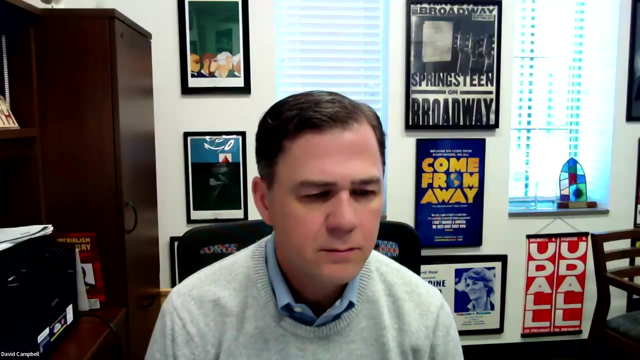 And so the I think the problem with either just a transmission approach or an inquiry approach is that it doesn't always take into account the habit of mind and skills That are needed for productive, you know, discourse and consensus building, and so on. Let me, let me take. 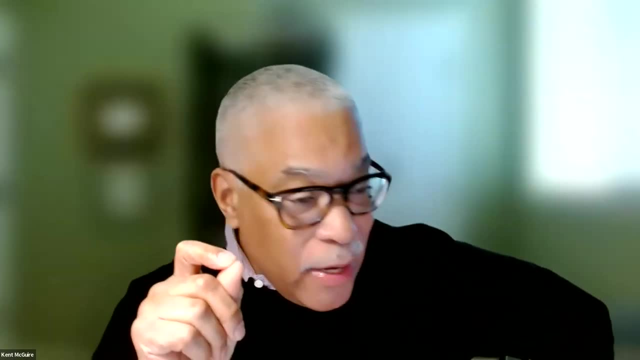 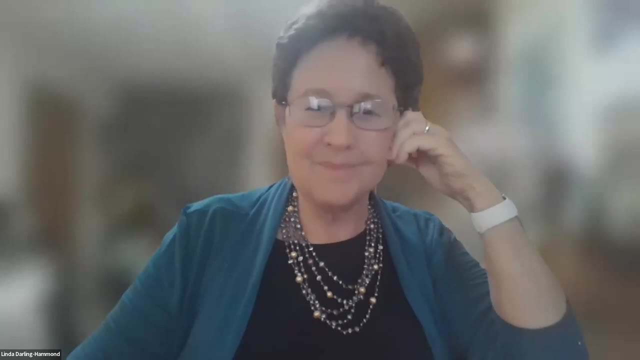 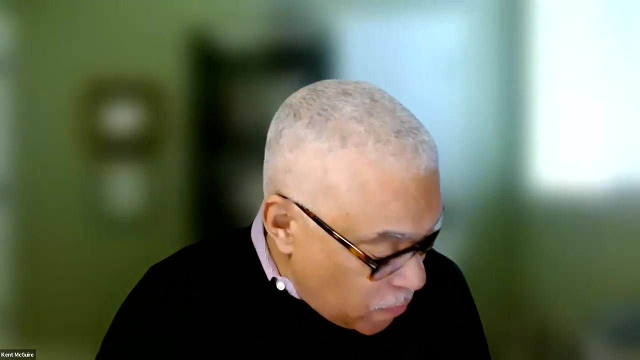 Linda's comment And turn it into a list, You know, maybe easier for folks to to to follow, You know. so I'd start by saying that you know our schools need to impart the knowledge, skills and dispositions For 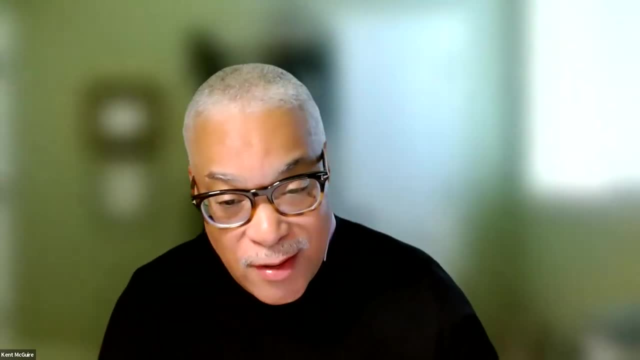 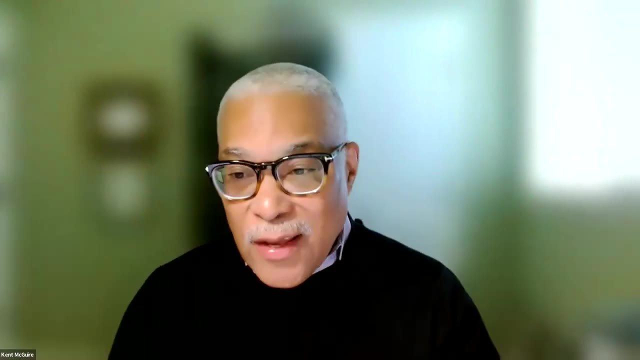 Right, Right. I mean I think that's one of the things that we need to be thinking about is that we need to be thinking about how we're going to make sure that our schools are effective, democratic and community engagement. I mean, that's the I, and I think this mindset is a big part of that. 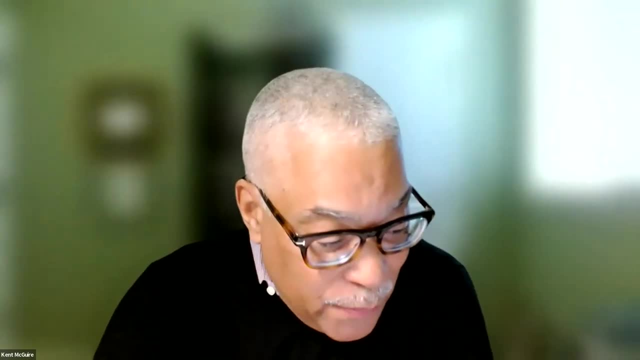 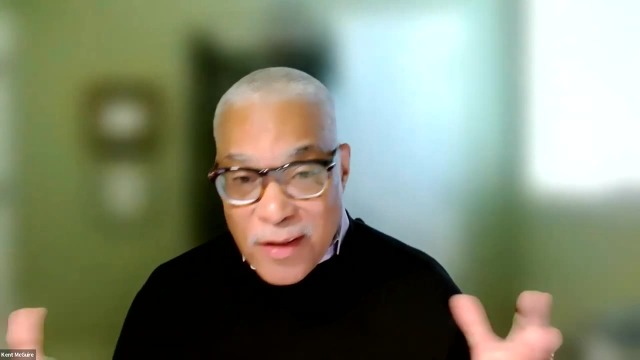 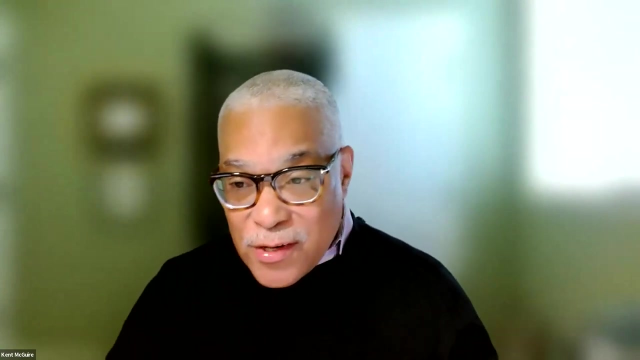 I think our schools should. I don't think it would hurt if they could do a better job of conveying common facts and information. I think that the one thing you've gotten to do is to help them discern fact from fiction, So learning how to grapple. 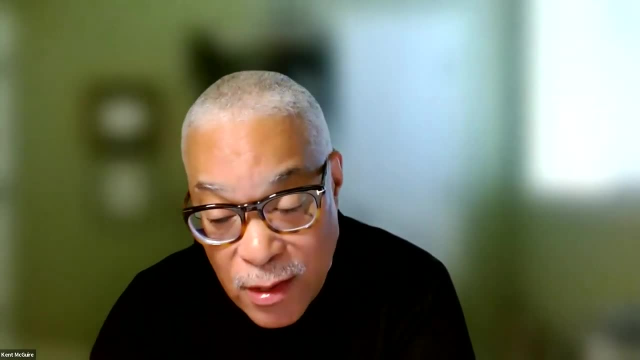 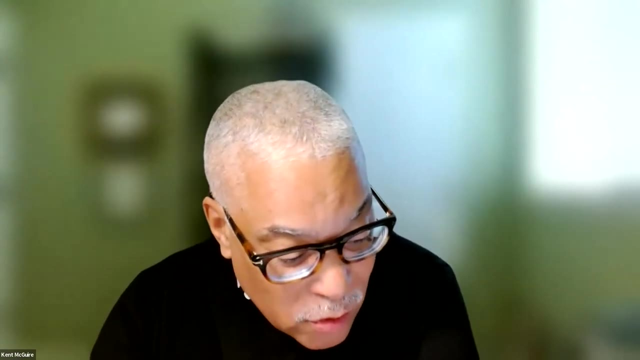 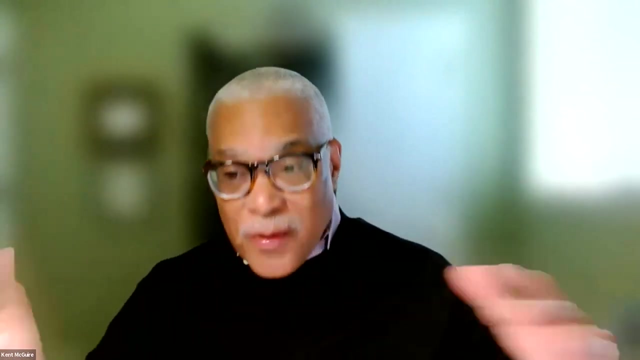 You know, with with information would be enormously Helpful. and maybe this might be the hardest, you know, the one where where teachers Peter need the most help, but but if our schools could get students New frame For thinking about societal problems. 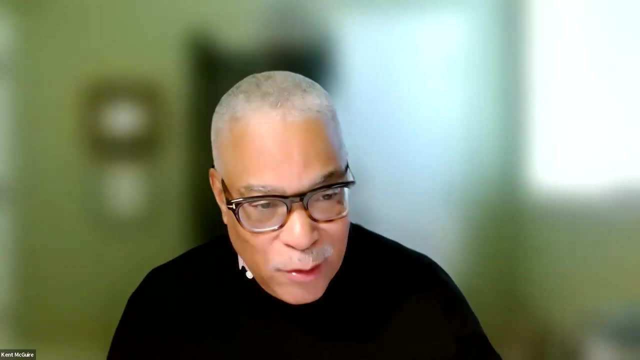 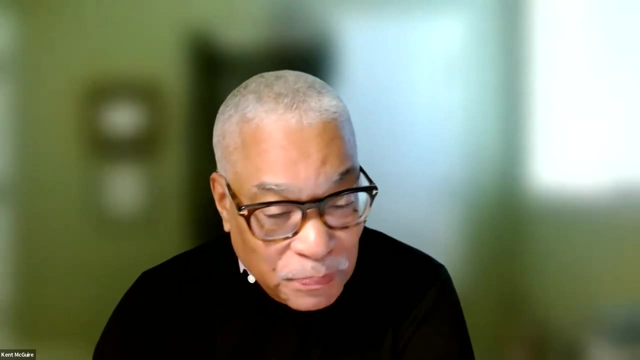 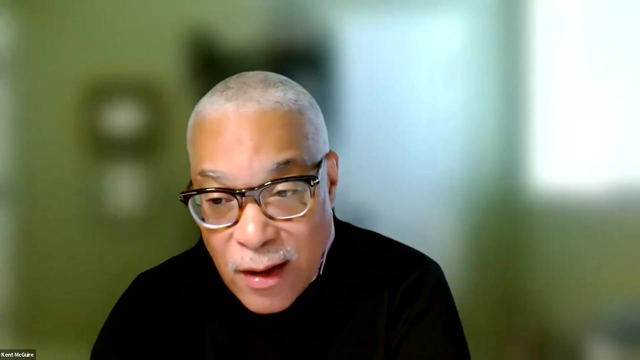 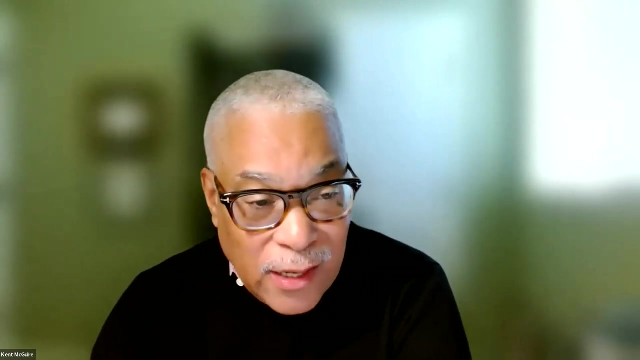 You know, a better tool box for grappling with what's going on in the world. that too, I think, would help enormously. What isn't helpful is the efforts to restrict what students can read and what teachers can do. I appreciate some of the motivation for where that comes from, but that actually, I think, is 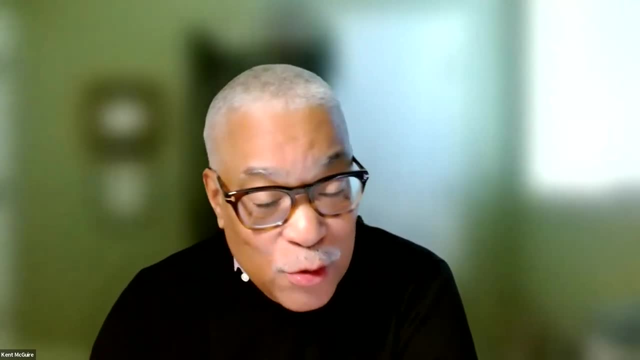 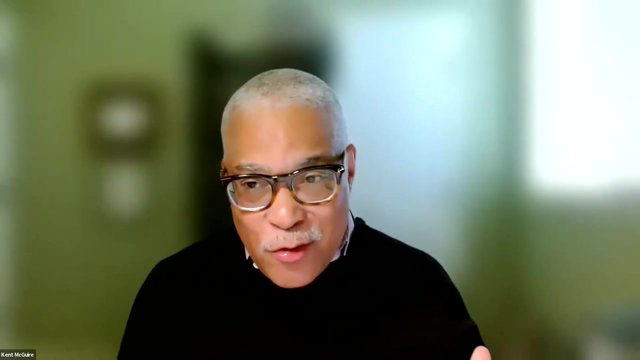 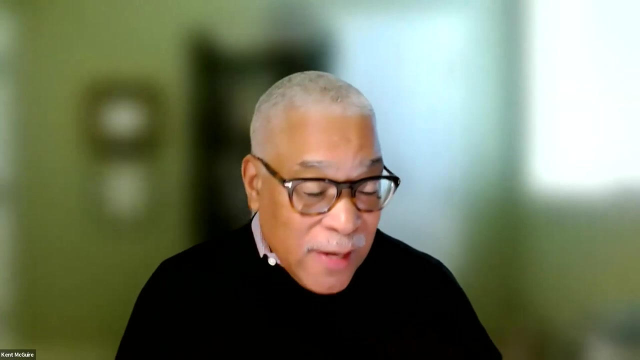 counterproductive. I do think knowledge of how a constitutional republic works goes hand in hand with grappling with problems in the democracy. The irony here is that we actually do need kids to know a lot more foundational knowledge about how the government works, because they'll be much better prepared. 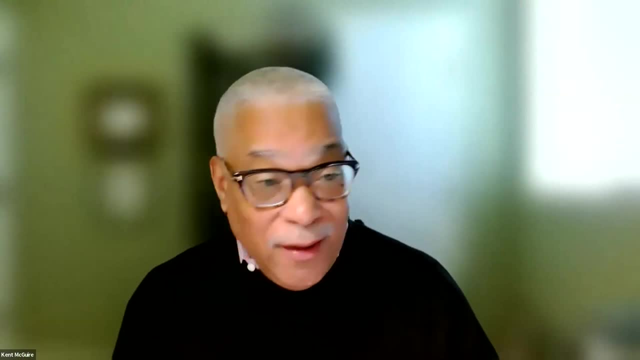 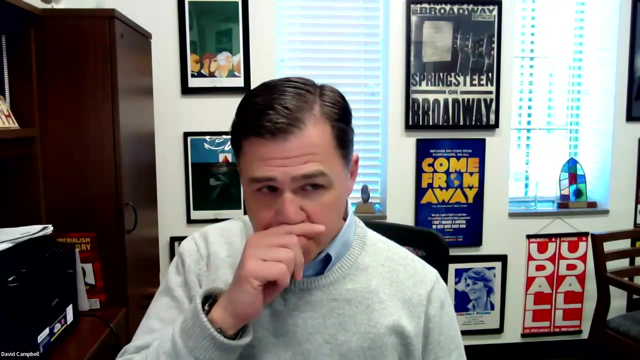 to actually think and behave democratically if they do. Thank you, I know that there are questions coming in and we'll be sure to get to those, but there were a couple of themes I wanted to make sure we hit with the panelists as well. 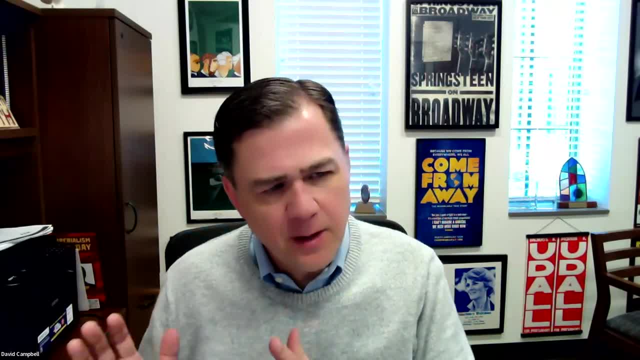 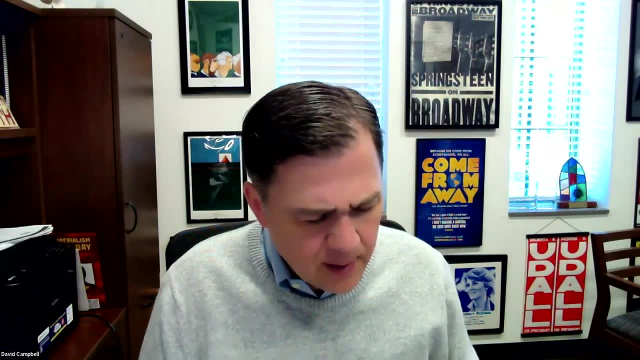 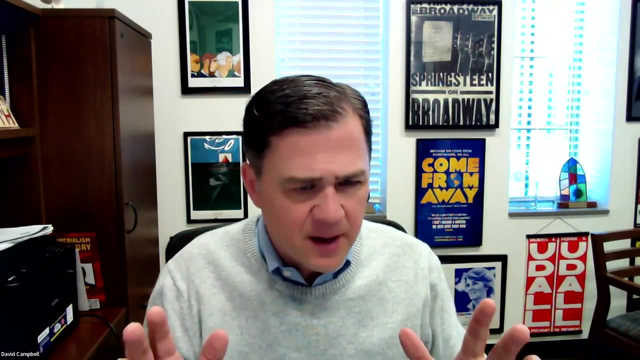 I'm going to pivot a little bit to an important theme in the volume that has come up implicitly so far, but let's make it explicit, and that is: what can the literature on learning science and whoever takes this question maybe take a moment and just define for the audience what learning science, or learning sciences, consists of? 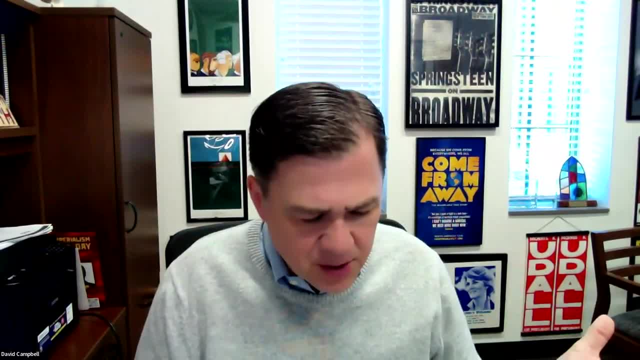 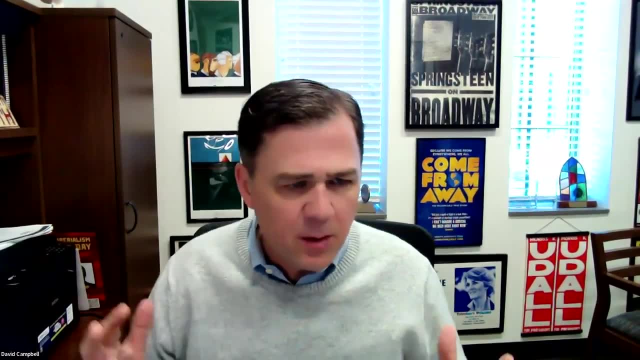 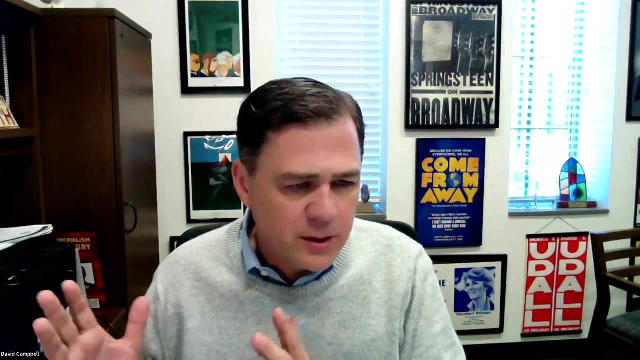 but what do we know about that body of research that can inform effective civic education? That is, how can we take what we know about what people learn and translate that into the civic space, Which is a subject to be taught in the way that others are? It's not like it's sitting off on its 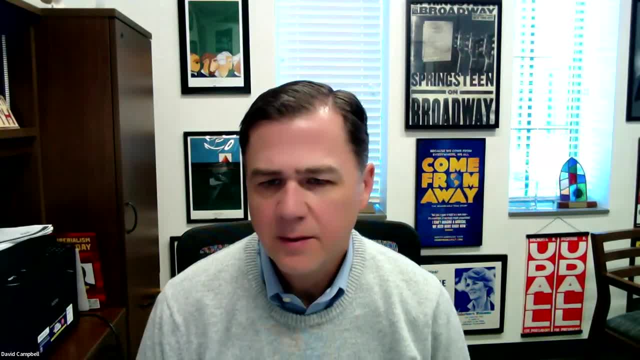 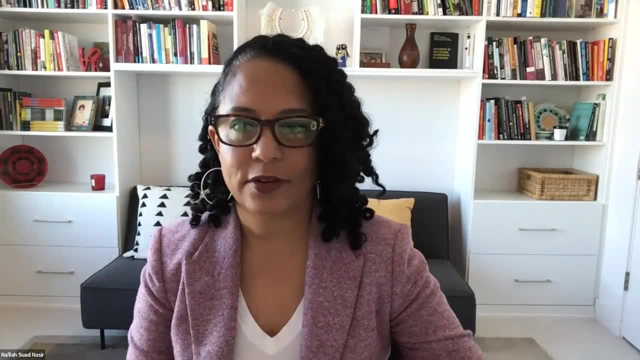 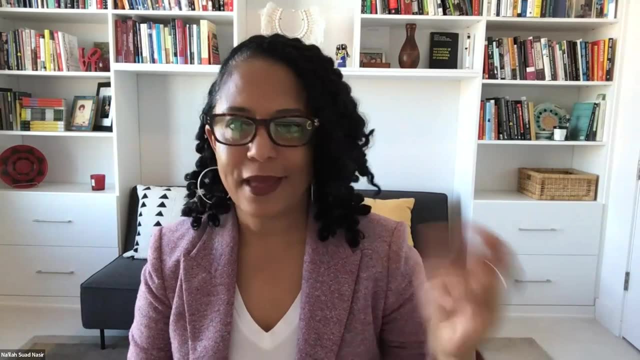 own island, Nayila. do you want to take that? Yeah, happy to jump in. I contributed a chapter with my colleagues Carolee and Mary Helen Emerdino-Yang. Carolee is a learning scientist, Mary Helen is a neuroscientist. In that piece, 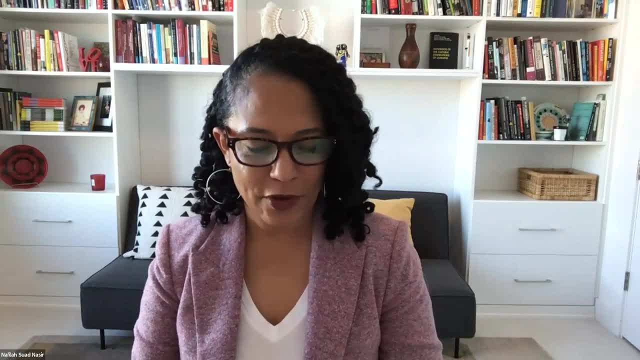 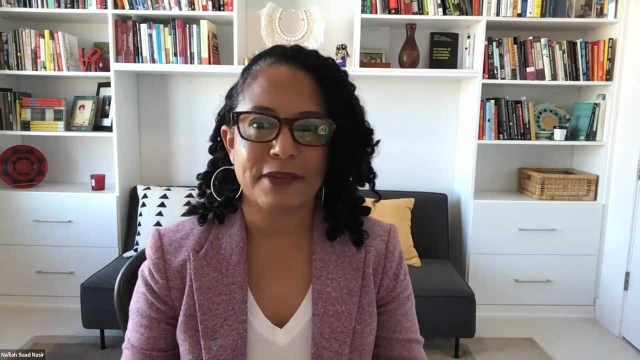 we kind of delve into the like: what is it that we know from the learning sciences, which is really the study of how people learn? What is it that we know from the learning sciences that might be useful to the set of questions that we're kind of collectively grappling with around civic education? 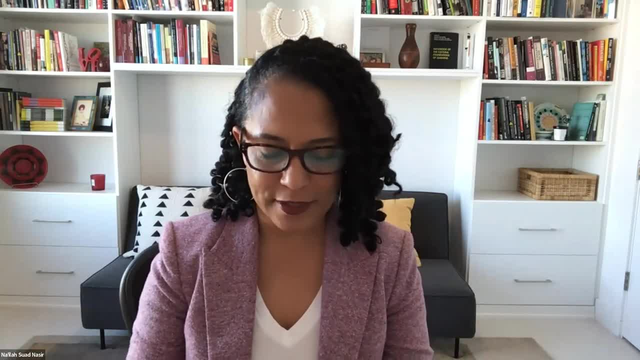 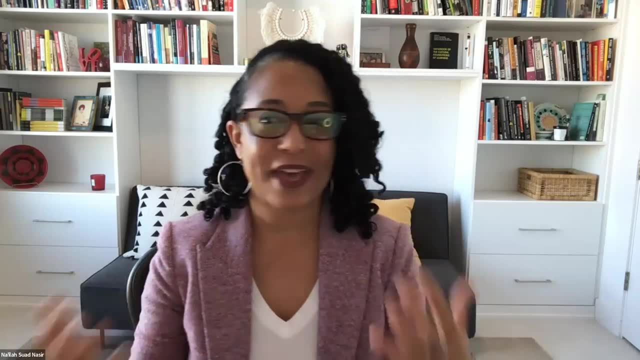 and, in particular, kind of civic reasoning and civic discourse. And you know, we point out first that there are some things we know that we didn't know 30 years ago. right, We know that learning isn't just a cognitive act, that it is a social act, that it is a cultural act, that it has to do. 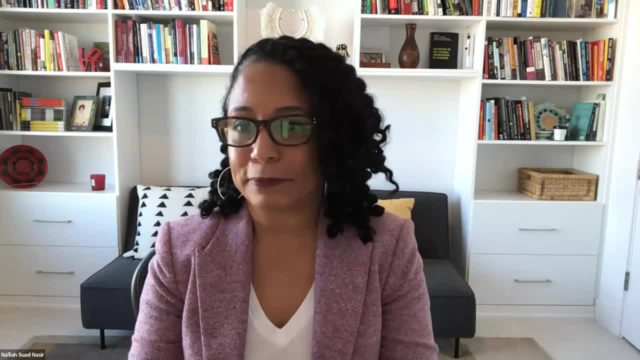 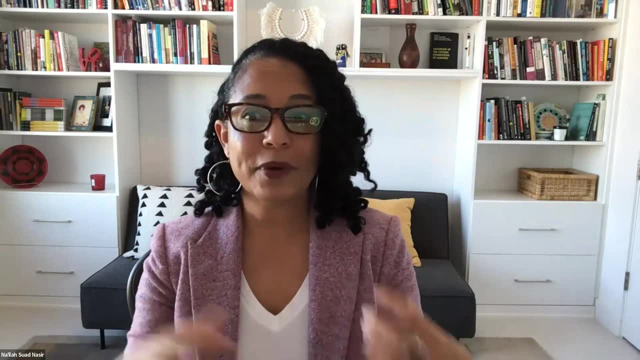 with identity and emotion. And we know that not just because we're learning. we know that we're not just from the studies of learning, where we can kind of see learners engage and understand what they learn. We know it from the neurological evidence on how we are hardwired as humans. 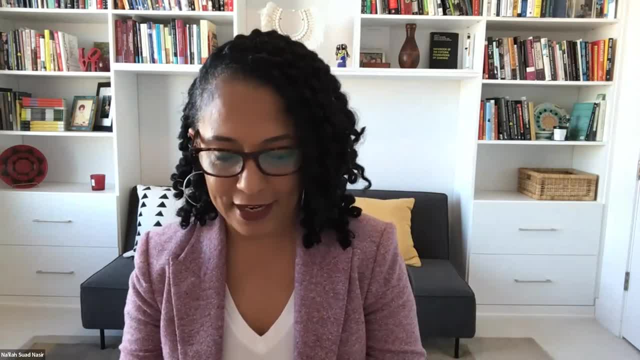 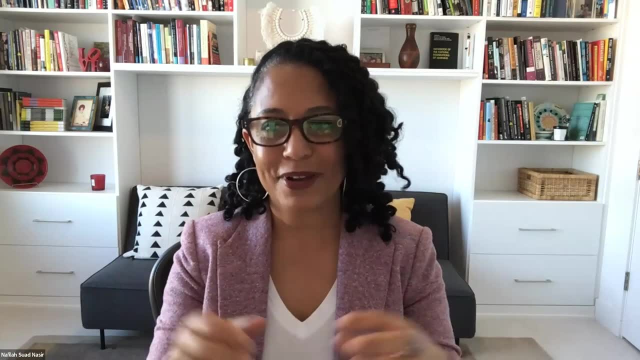 Well, that means a lot of things for this context, right, It means that if identity and emotion are critical to learning, these topics around that we take up under the umbrella of civic engagement actually are quite emotional and touch at the heart of people's identity. Well, 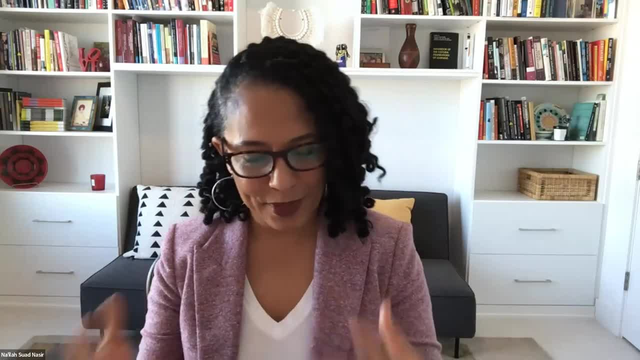 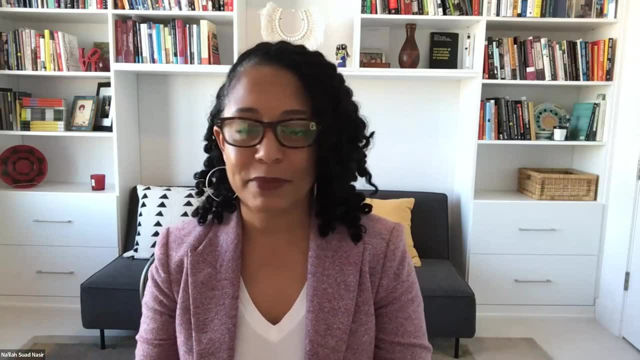 that's very rich fodder to create great learning spaces. We know that the seeds of civic reasoning and learning happen very early in development. Moral development and moral reasoning develops in very young children, as does the capacity for empathy. So in many ways we are hardwired. 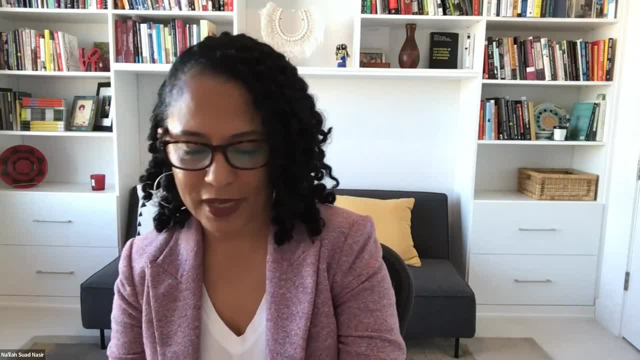 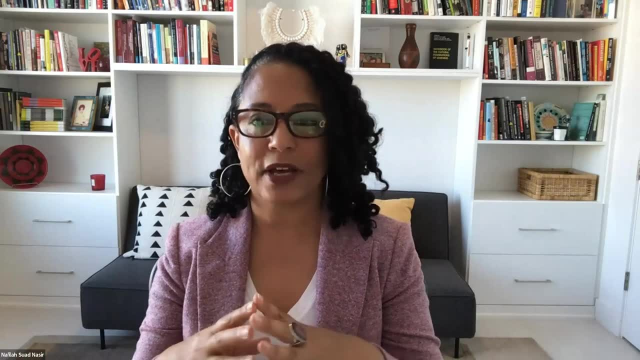 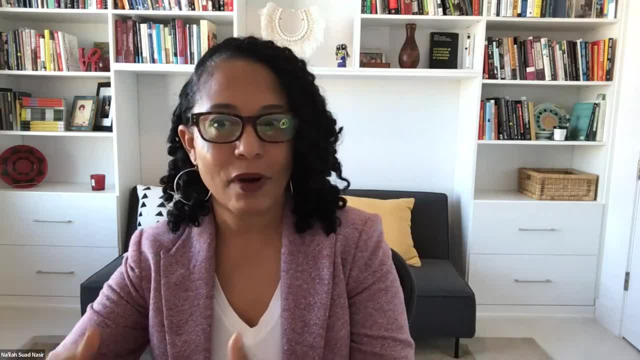 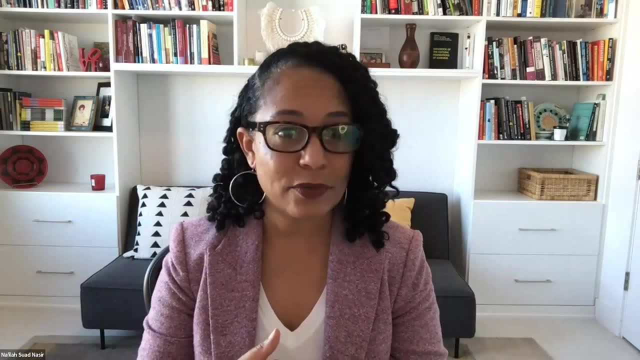 lean into what we know from the learning sciences and what we think we want and and and know that young people need to know how to do. Valuing of complexity and weighing different points of view is really critical to this kind of engagement. That's one. Two: making ethical. 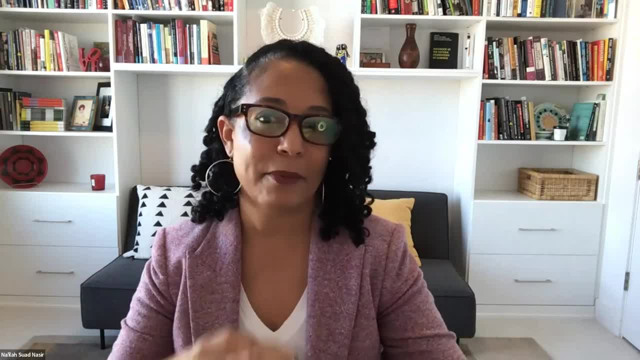 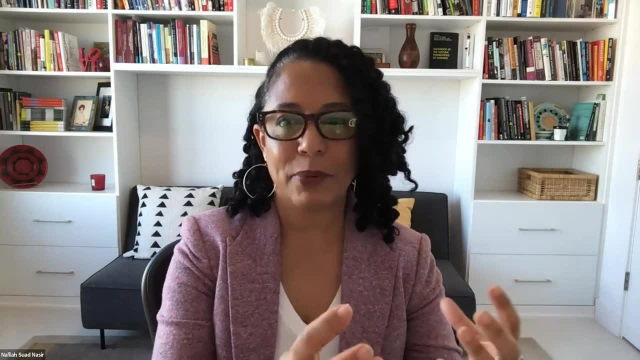 commitments to empathize with others, really centering empathy in our, in our conversations, and then valuing and doing good for others. So this combination of kind of empathy being a part of a community and complex reasoning we argue are really at the heart of 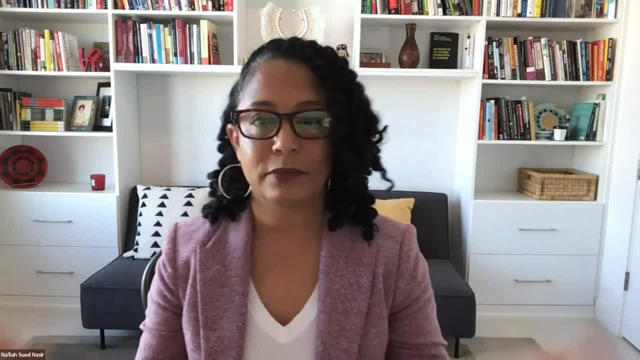 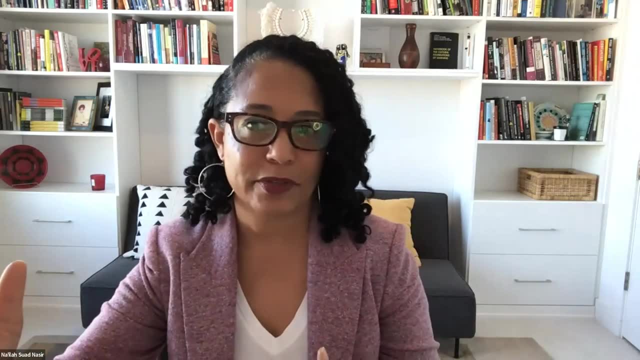 what you want to prepare young people to be able to do, And there are many, many ways in the context of the curriculum to do that. We take this stance that this should happen across content areas, across the developmental span, and that there are ways to to do that in classrooms. 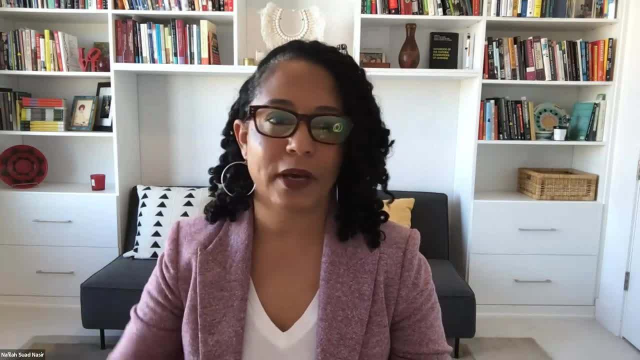 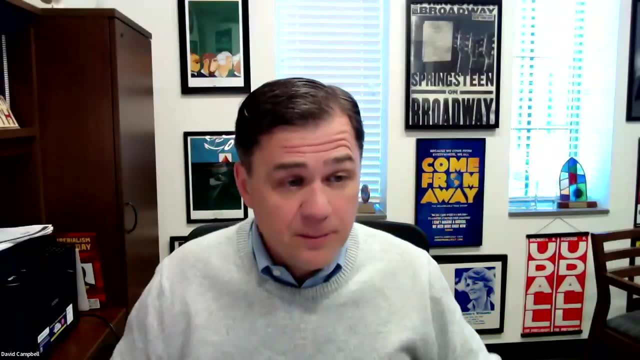 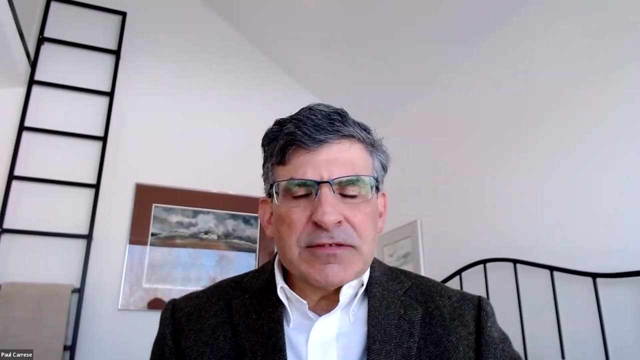 from very early children all the way up through adolescents and even college students. Thank you, Can I follow up? Yes, Can I follow up on that, Those very helpful comments And and wrap in some earlier questions you posed and some comments from the panel. 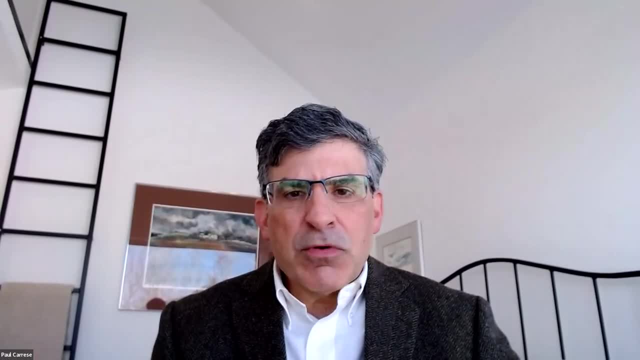 In the American- I'm sorry- the Educating for American Democracy report, we decided to talk about civic knowledge and civic virtues, as well as civic participation, civic engagement. So this middle term comes in and it's the old fashioned term specific to civics. 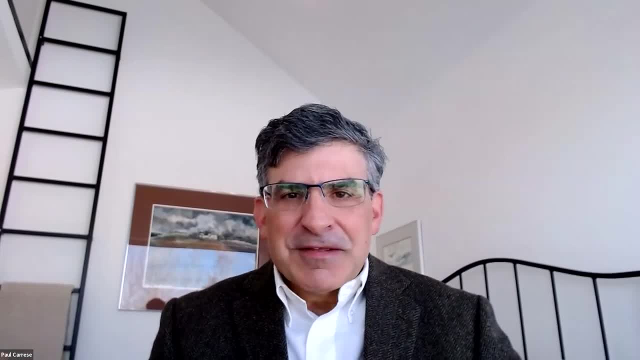 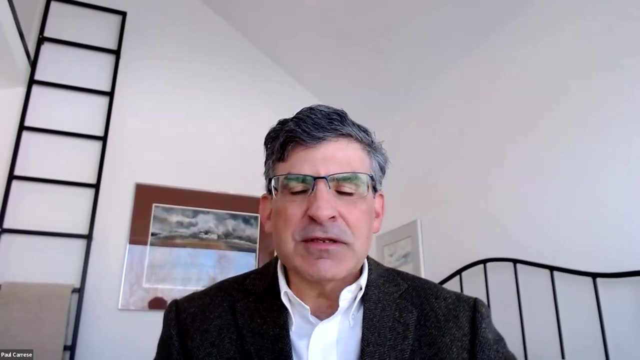 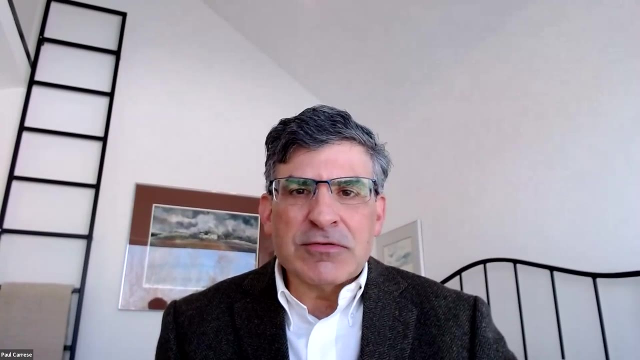 that addresses the learning and pedagogy sets of more specific social scientific knowledge. that is also a part of the report. There's a separate pedagogy appendix to the Educating for American Democracy report. But civic virtues is, or used to be, a natural term. 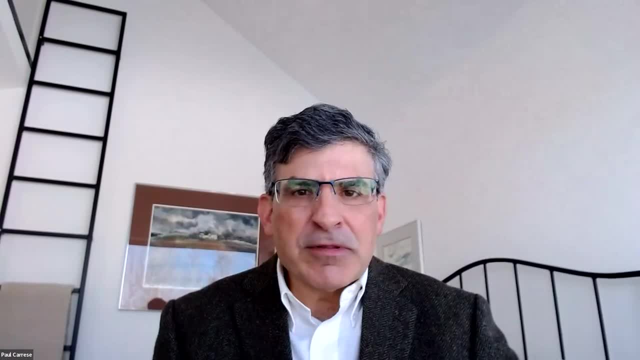 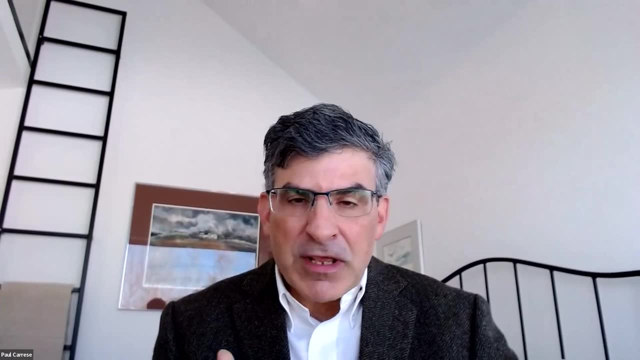 about self-governing peoples, democratic republics, that virtues are needed of the citizens and of the citizens of the republics, And so we're going to talk about that And expectations for the leaders. So one element of our democratic crisis right now. 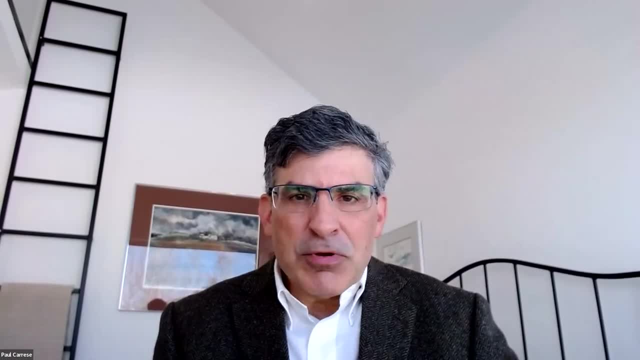 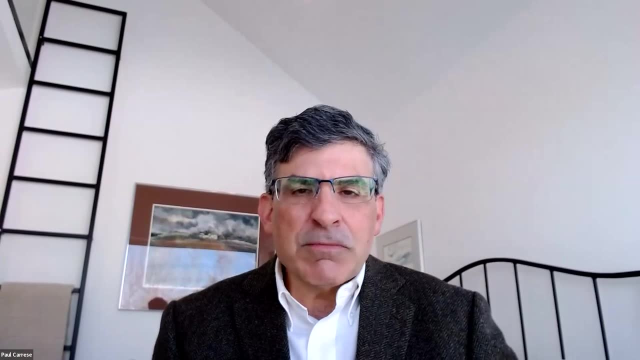 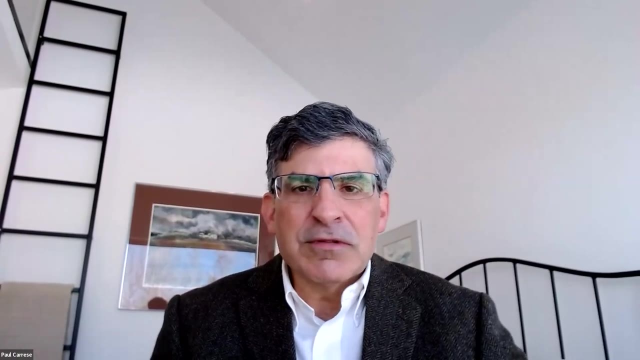 is the angry polarization and also loss of confidence in almost all major institutions and all major professions. And one wonders if a part of that loss of confidence is because so many people are disgusted with what politics is or has become now with anger. So the virtues, the old fashioned word virtues, 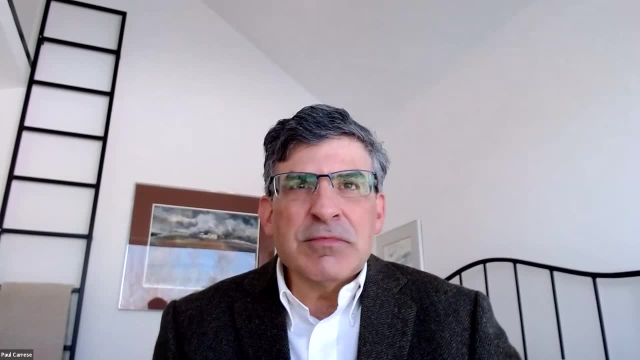 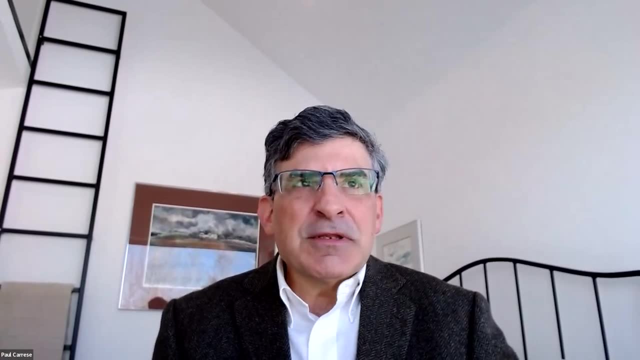 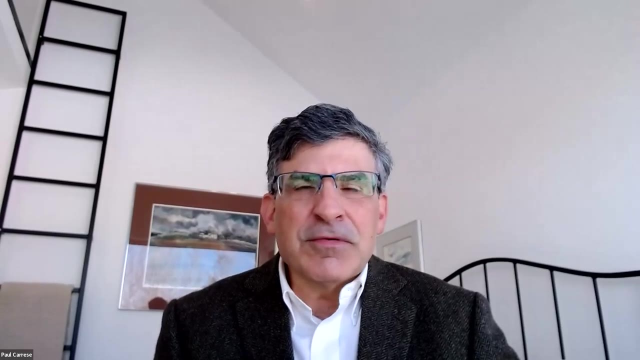 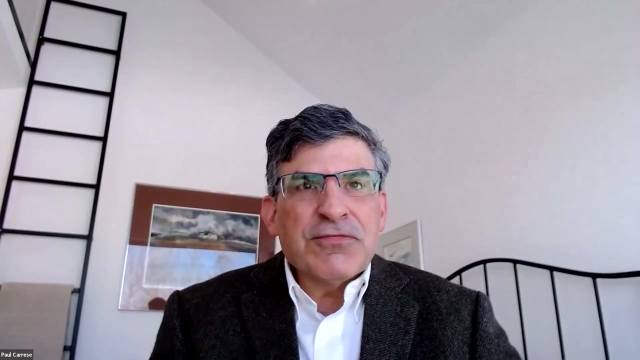 the educational pedagogy. language is about dispositions and skills and such, But that term virtues- can paradoxically be a grounding, a kind of grounding and a unifying set of ideas in civics education and even history education, If you put in front of teachers and teacher preparation. 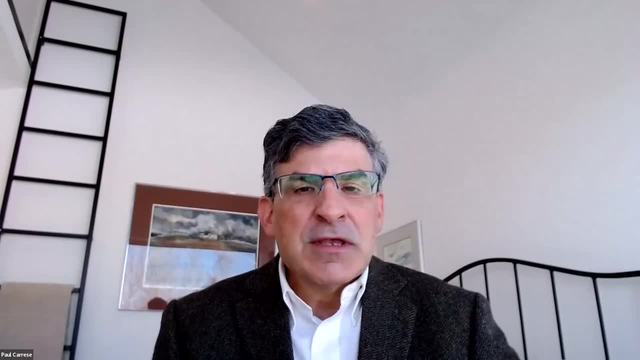 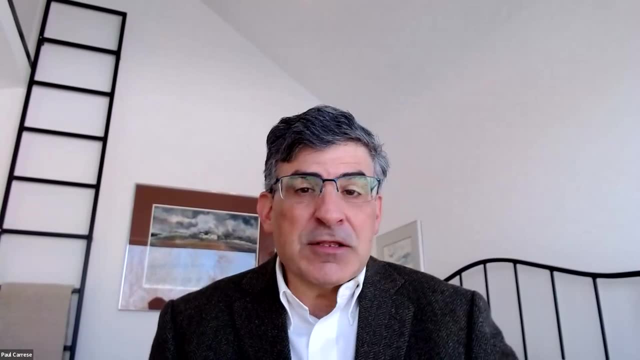 and then in front of students, school board, others, this idea that this is hard. being a free citizen, self-governing, participating, being an aspiring citizen, this is hard work. These are important multiple disciplines involved and the knowledge as well as the dispositions and attitudes. 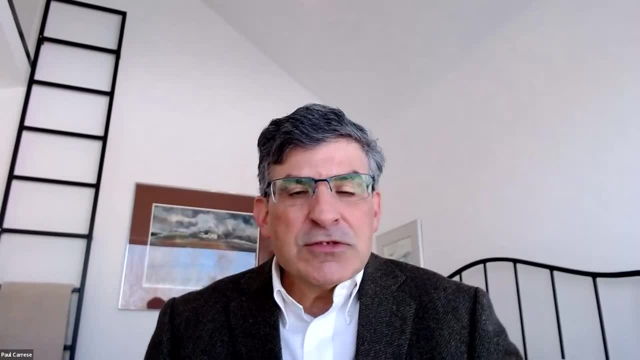 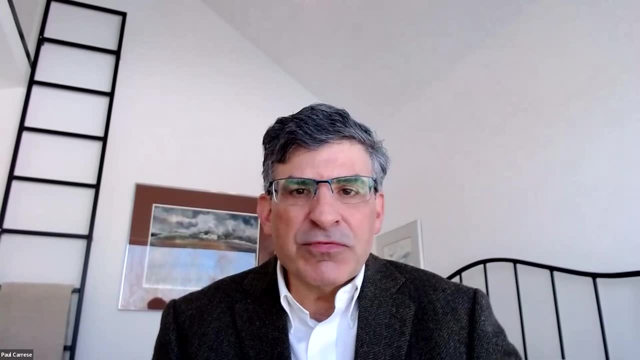 as well as preparation for engagement. this is hard work, So among the virtues that we've identified were patriotism in the American way, reflective patriotism, a term that Alexis de Tocqueville uses in Democracy in America when he visits us in the 1830s. 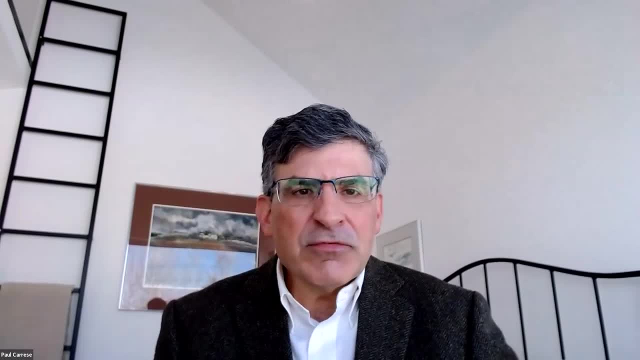 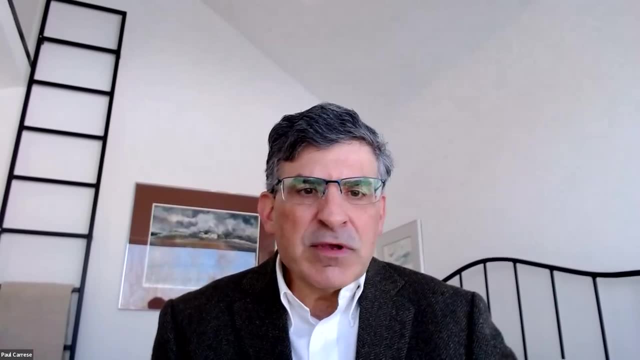 The Americans have a kind of argumentative, rational patriotism. They love America, they believe in America, they're proud of being American, but they want to argue about everything. Just what does America mean? Is the government doing what it should be doing? 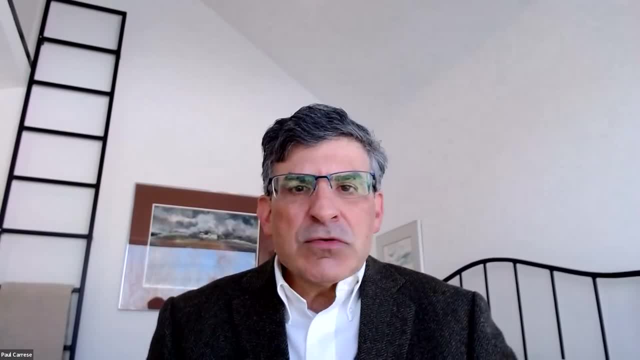 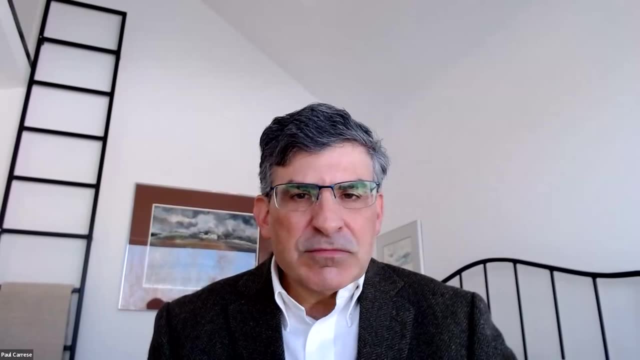 Is the government protecting our rights the way it should. So a reflective patriotism as a civic virtue, civil disagreement as a civic virtue. civil disagreement as a civic virtue. civil disagreement as a civic virtue. free people, Tocqueville says, are going to disagree about everything all the time. 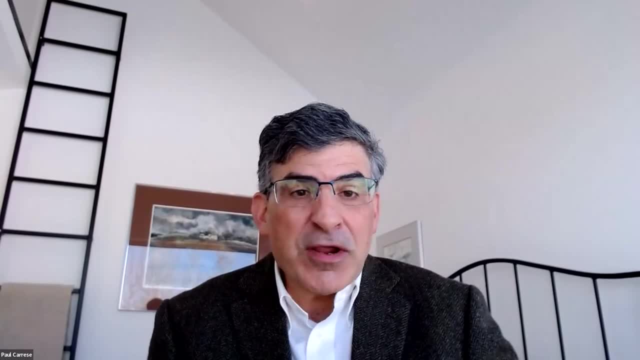 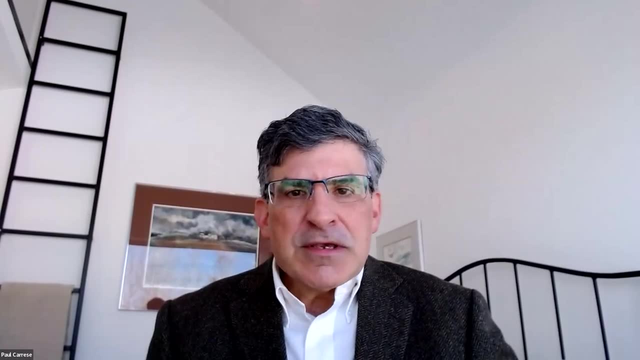 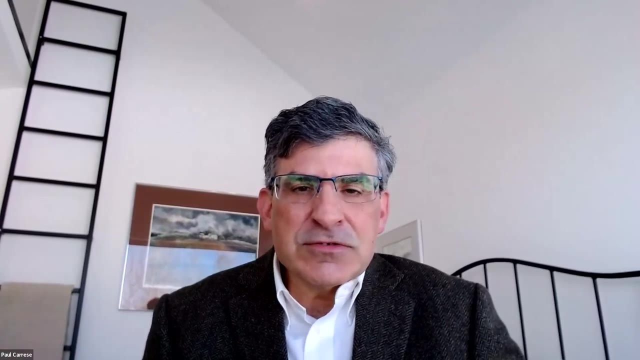 while also having in common that they are Americans. That's the patriotism part. We're in this together e pluribus unum. So reflective patriotism, civil disagreement and civic friendship. So I'm the conservative, I'm introducing these old-fashioned terms. 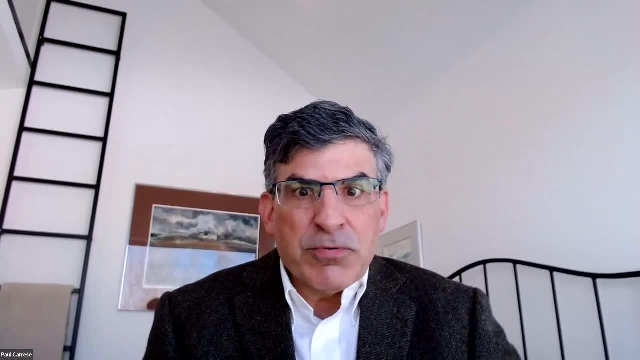 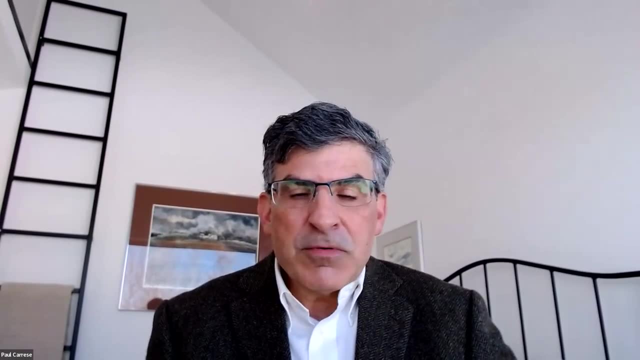 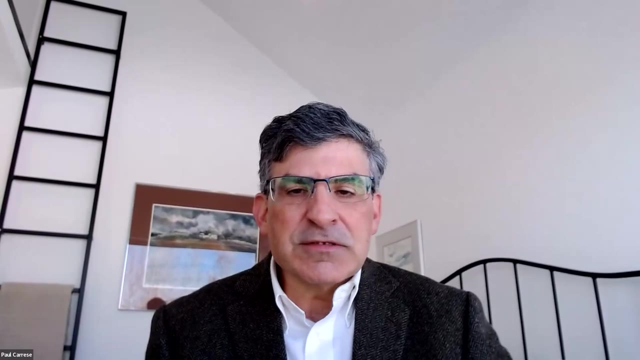 Civic friendship. Peter and I disagree about really important things. I respect that he's smart. I think he respects it. He respects that I'm smart. We respect that. we disagree, But we're Americans and we're fellow professionals and we live to talk another day about these things. 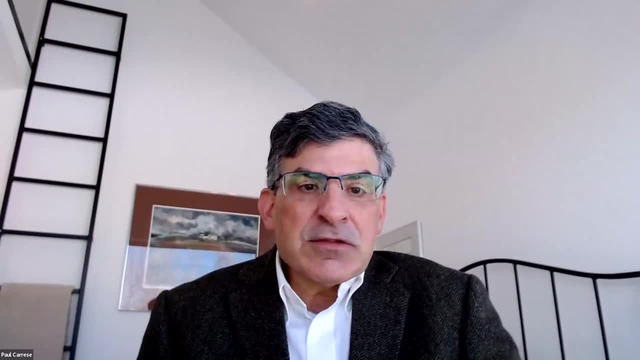 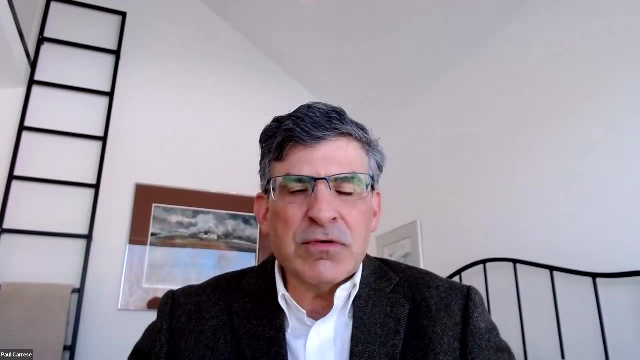 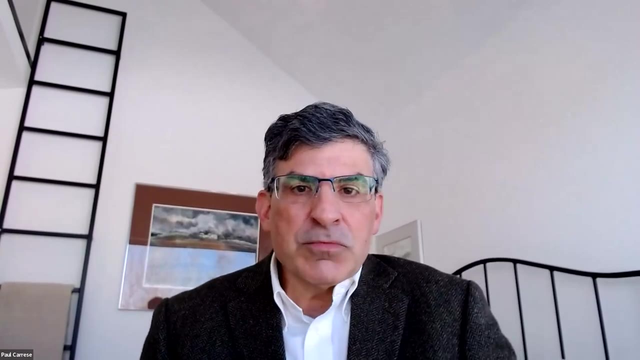 And eventually I'll persuade Peter that I'm right. But the civic culture of understanding that people of a different partisan philosophical view are not evil. you disagree with them, You think they're wrong And it's important and it's serious, but we're in this together. 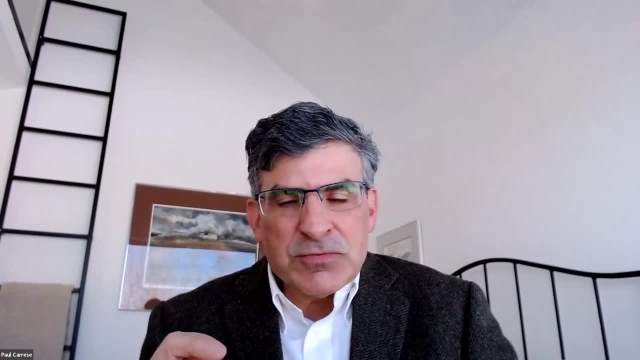 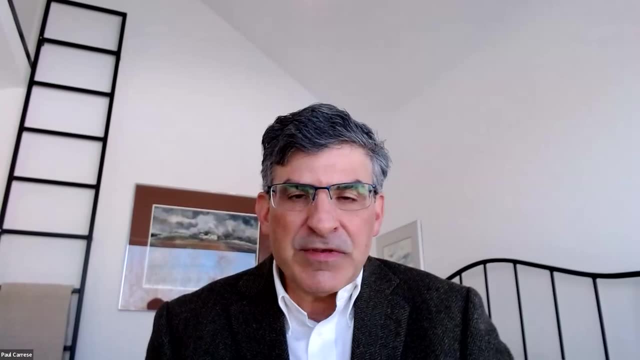 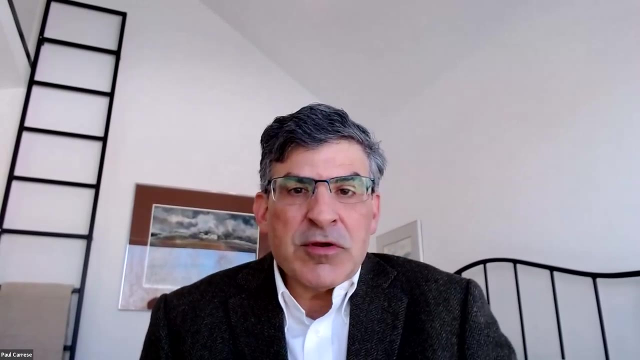 So that's, and just one final point- that set of language, those ideas, civic virtues can be motivating for students to think: hey, I'm an American, We're all Americans. There are people here who are immigrants, who are aspiring Americans. 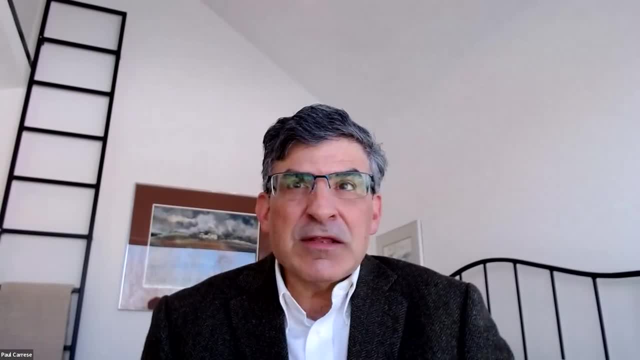 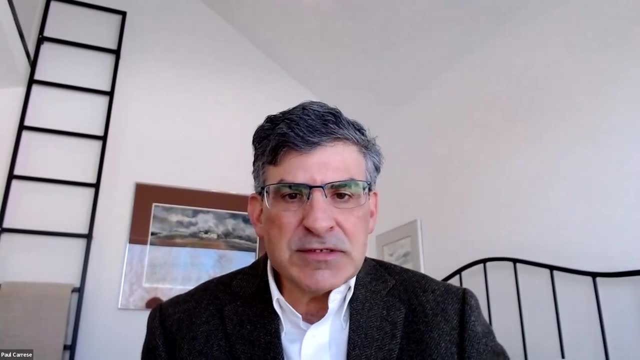 We're all in this together. This can provide a kind of positive culture in schools, which is a whole set of issues about public schools, a positive culture, And it's important to think about public schools. We are in this together. It's hard work. 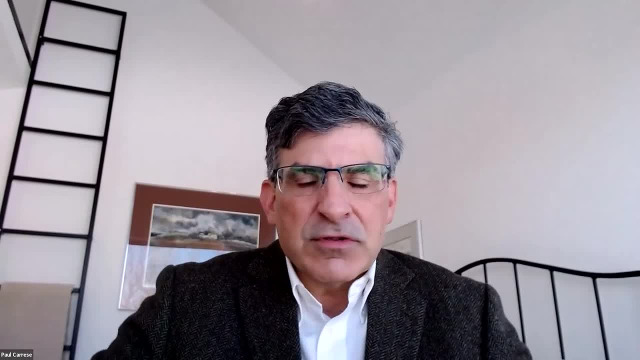 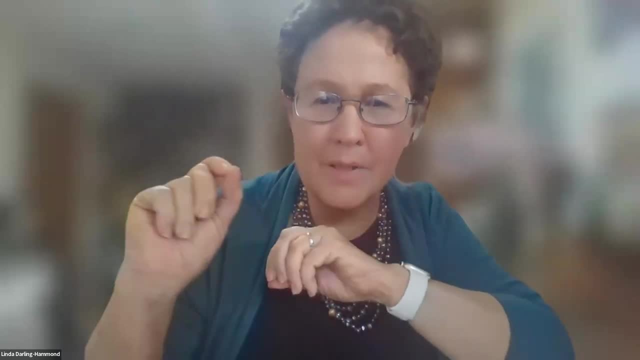 This is exciting. This is interesting. I have another dimension of life to look forward to. Yeah, As you're talking, Paul, I was thinking about marrying, the way in which one state marries the civic virtues with the civic reasoning. So, in Washington State, 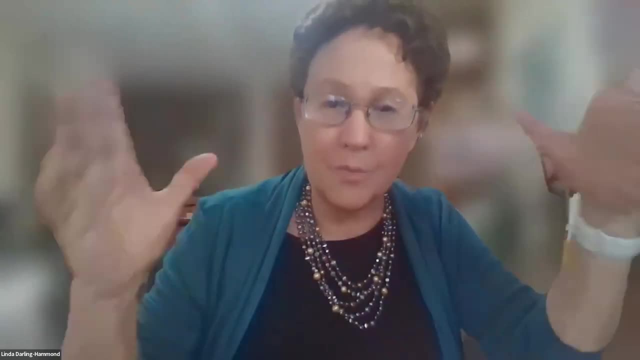 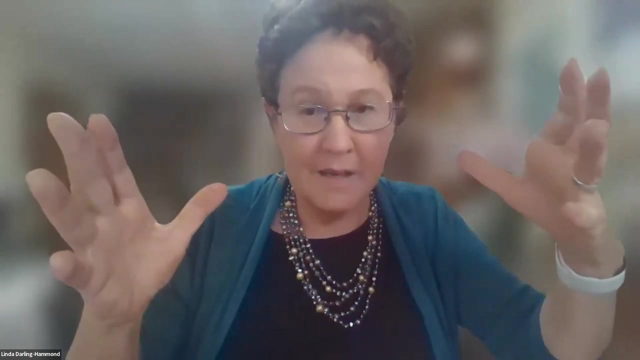 they have a set of performance tasks that are required of districts to deliver, but they're not used in accountability. One of them, for civics, is that students have to identify an issue about which they're not used in accountability. They have to identify an issue about which there's disagreement. 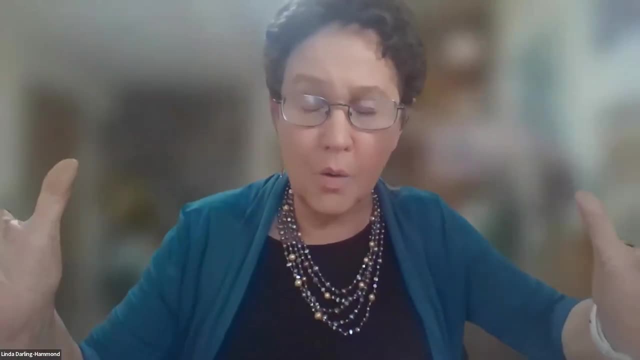 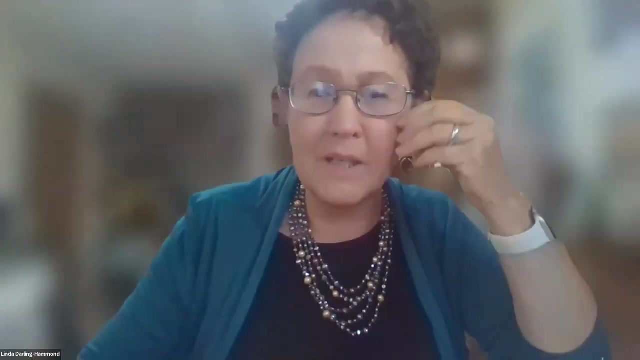 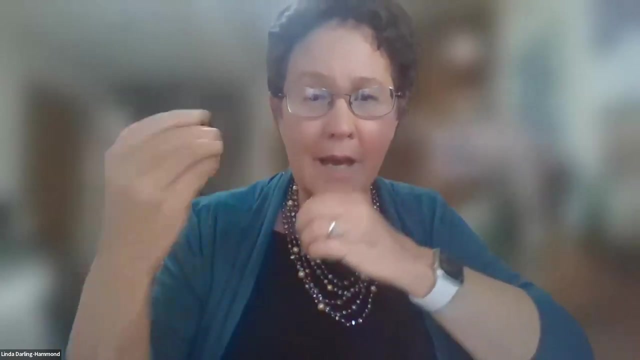 and in which there is a tension between the good of the whole and individual freedom. Then they have to research cases and legislation and sort of legal history around that issue and then kind of come to a reasoned discussion of how one can balance the e pluribus unum elements. 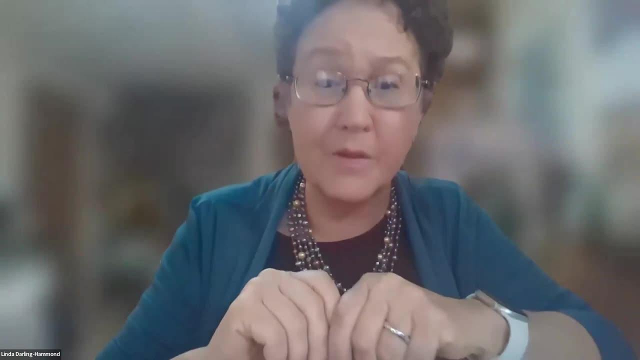 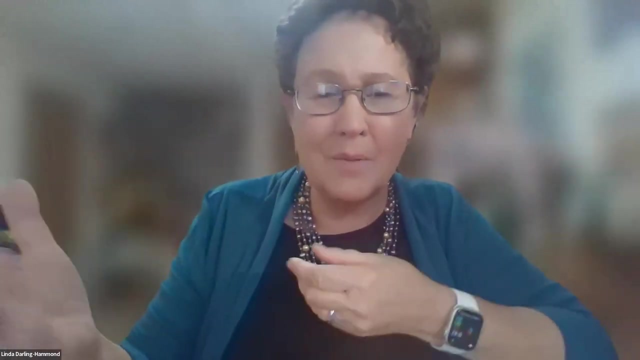 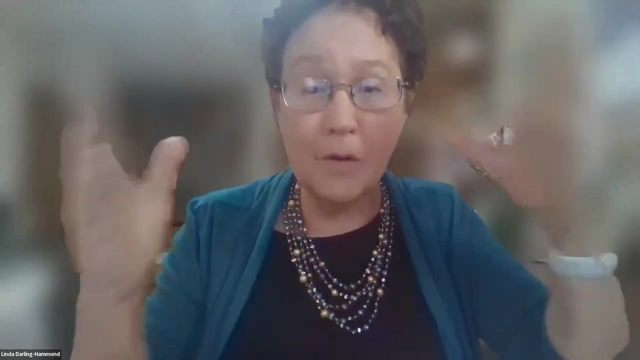 of the good of the whole and the individual. So that's something that everybody engages in And there are years of work leading up to both that understanding of the civic virtue and of the process of civic reasoning. I think if we could do more of that, 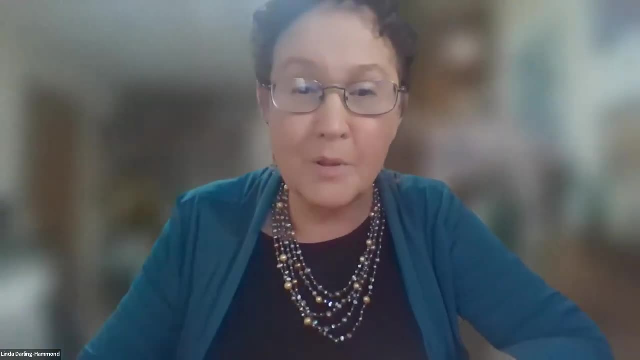 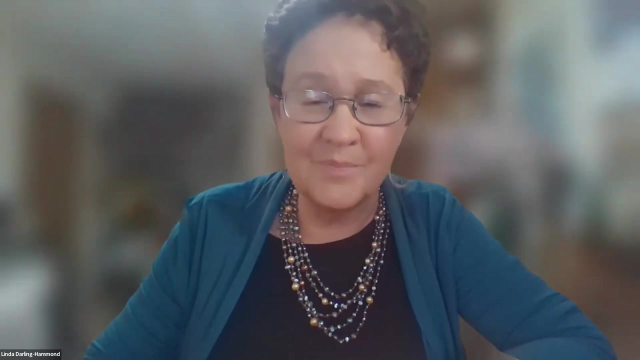 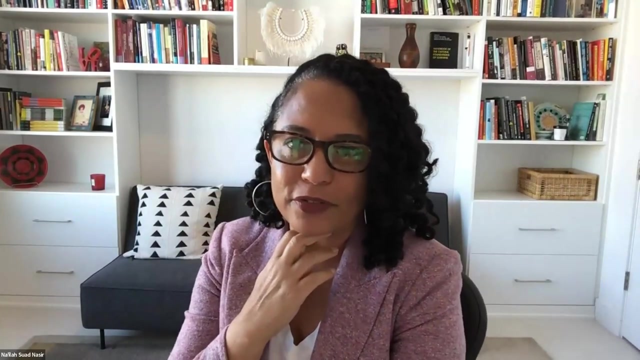 rather than just asking people to fill in the multiple choice civics test, we might get the kind of understanding that you're talking about there, But I agree with that. I also think that there's another element. you were talking, Paul, about reflective patriotism. 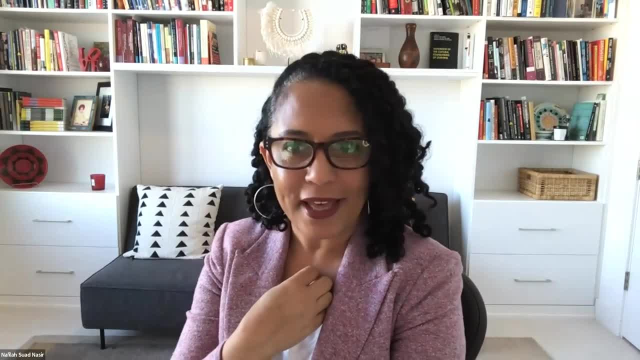 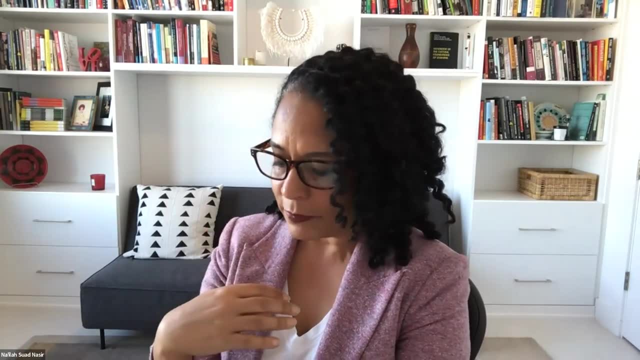 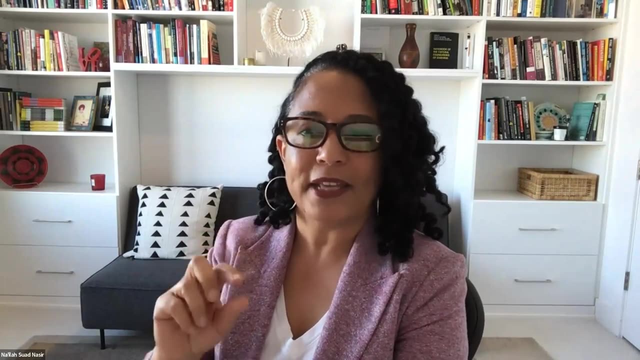 and I am wrestling with that. On the one hand, I think an important part of patriotism is that identity as American and the collective and what we all hold, And I think that part of what's happening in the public discourse is the recognition that, while that has been true in the ideal, 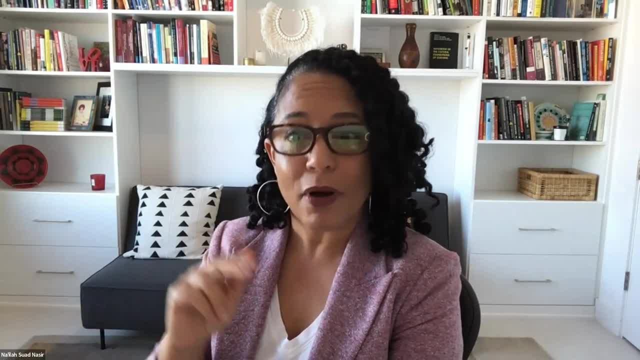 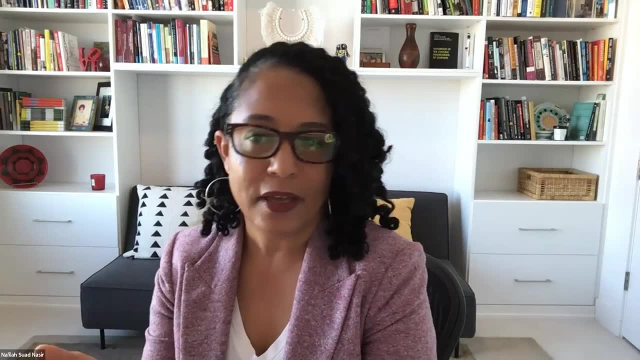 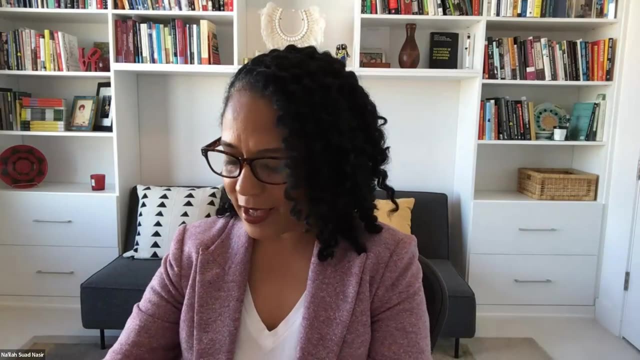 in the practice it hasn't always been true, And part of patriotic engagement is holding us collectively to a higher standard about how we offer enfranchisement across the board more fully, And so I think that if that definition of patriotism includes pushing us all to be better, 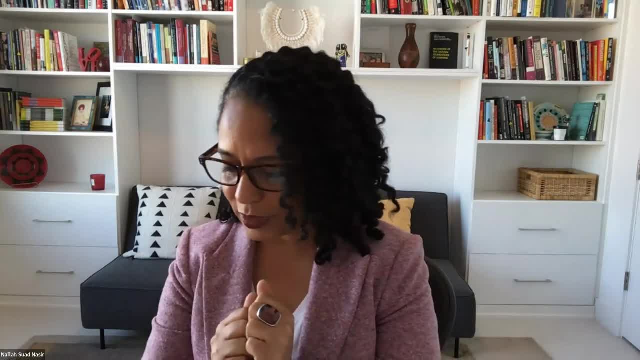 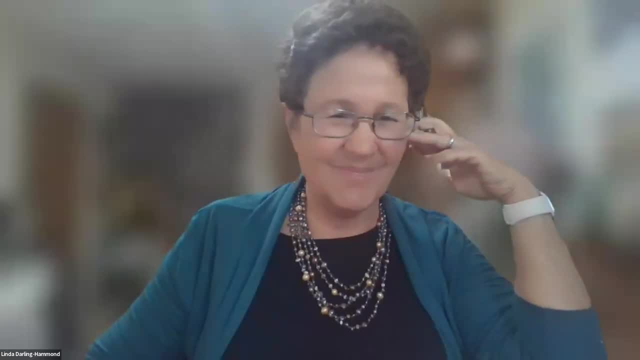 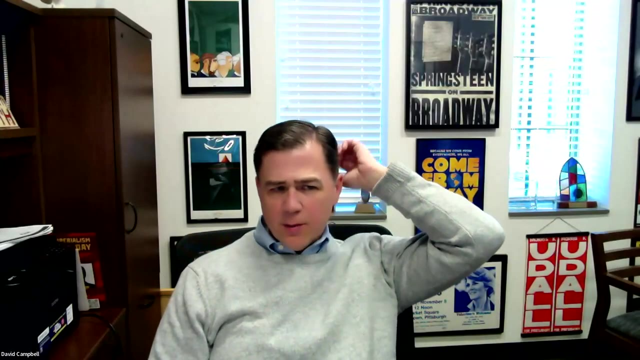 pushing our country to be better. I think that's just a really important dimension of that And it feels quite virtuous. I'm gonna shift us Just quickly. let's talk a little bit about two things, So we're gonna cover these two. 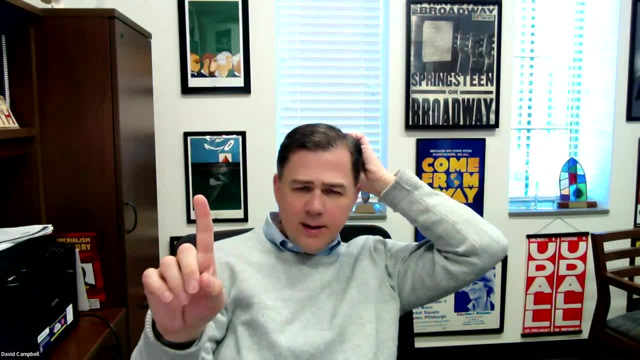 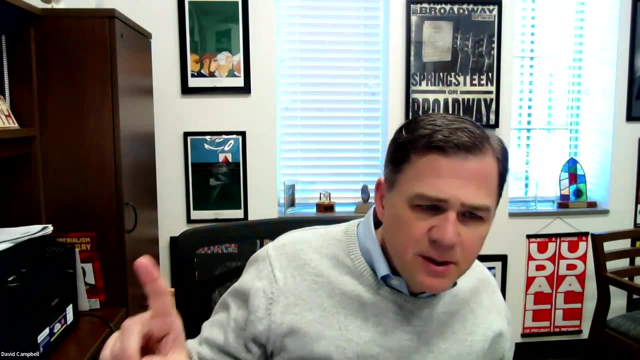 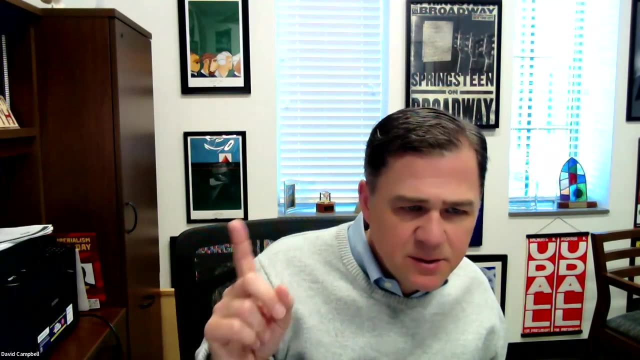 and then we'll move to Q&A One: teacher education. How do we train teachers to do what needs to be done in the classroom, given all of the tensions around civic education? So I'm talking about teacher education, and then we'll talk a little bit about policy writ large. 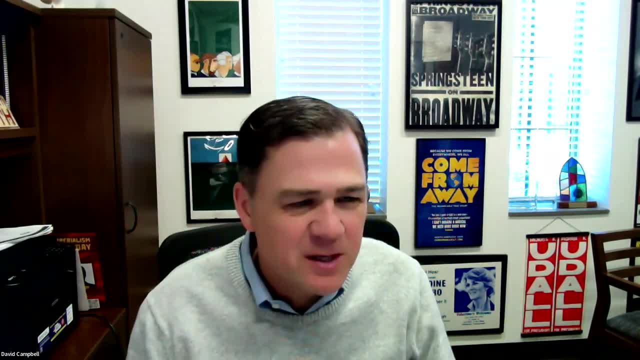 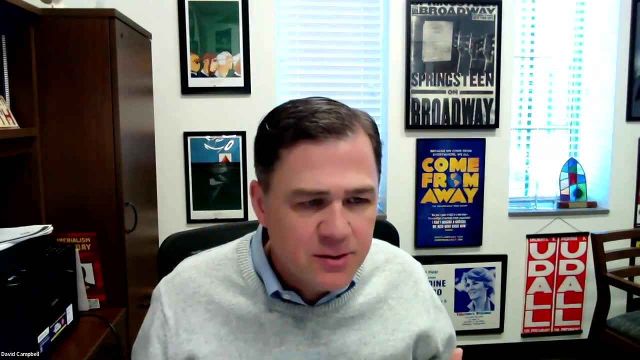 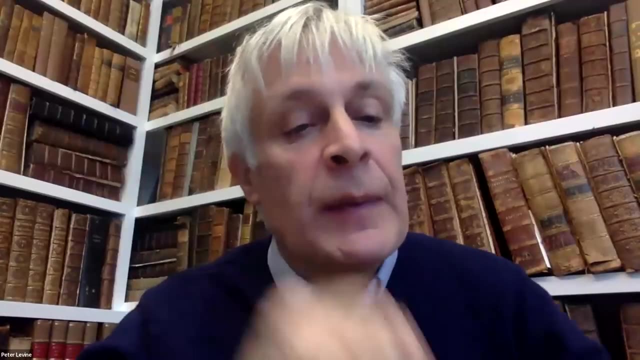 But not a simple question. but we're done. But let's start with teacher education. So what can teacher education programs do to prepare teachers for 21st century civic education? I'll just say a couple of words about that. I think there's lots of assets in the teacher force. 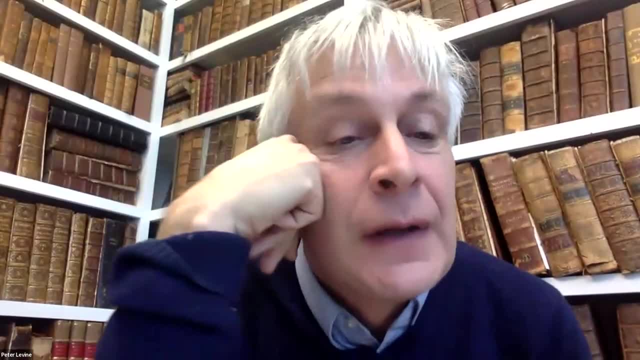 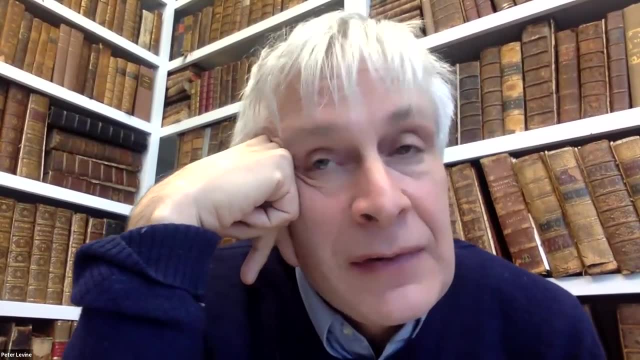 in terms of the. there are many, for example, especially social studies. teachers in middle school and high school are just the salt of their earth, center of their communities, and sometimes elementary school teachers too. But I think there's things to work on, And I would just name two. There is content, knowledge in history and 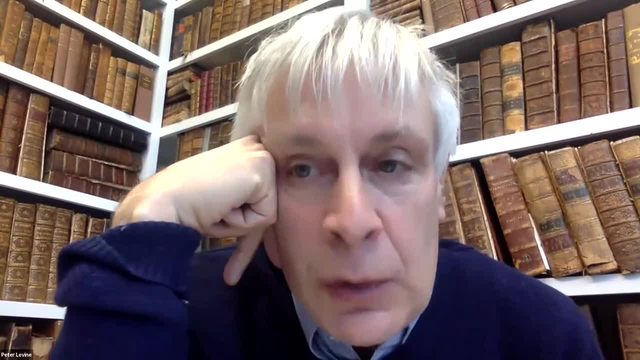 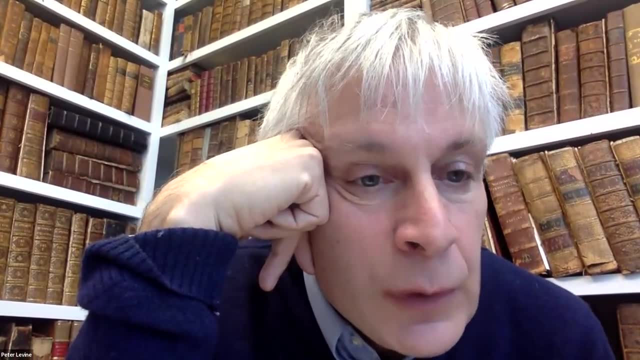 politics. that you know, particularly one of the Q&A questions asked about high school teachers who weren't really trained for that. But I would actually particularly emphasize elementary classroom teachers because we're really asking them to well. so let me say also that the 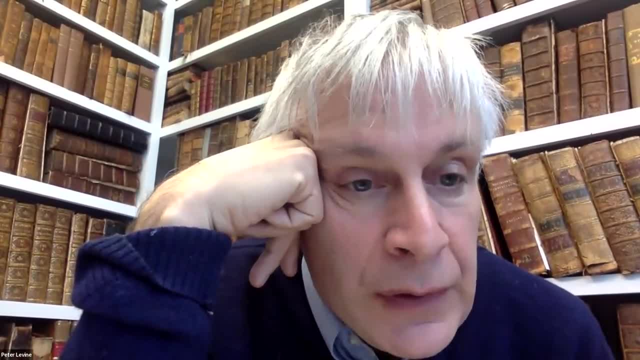 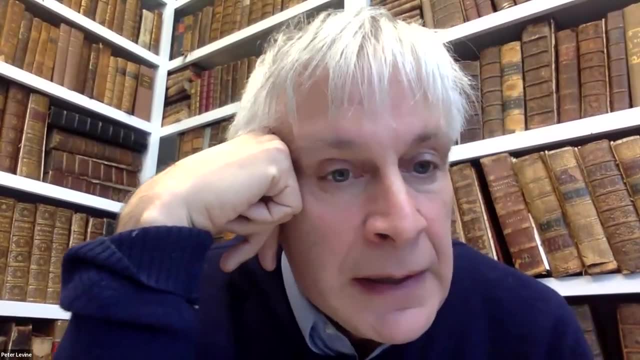 Educating for American Democracy framework is really asking for the most intellectually rigorous civics curriculum that has ever been offered in the United States. I don't buy the idea that back in the day we taught civics with so much rigor and now we don't. I think it was often. 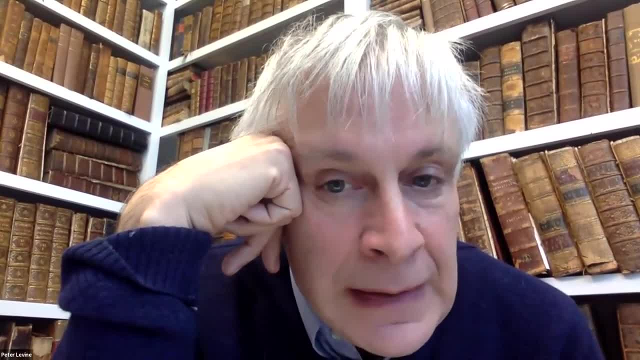 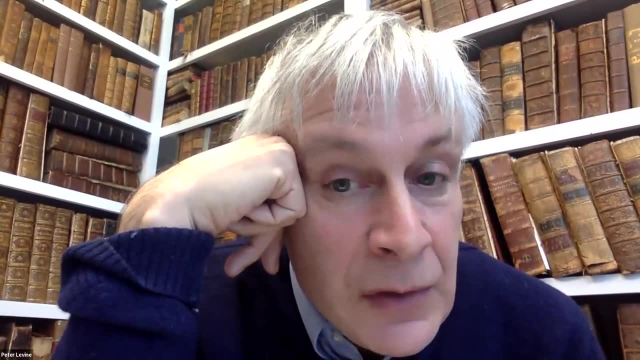 over history quite weak, But because of the needs in the 21st century, we're asking for the most academically rigorous civics to be offered at mass scale. that's ever been done And that's going to take some investment in content knowledge. 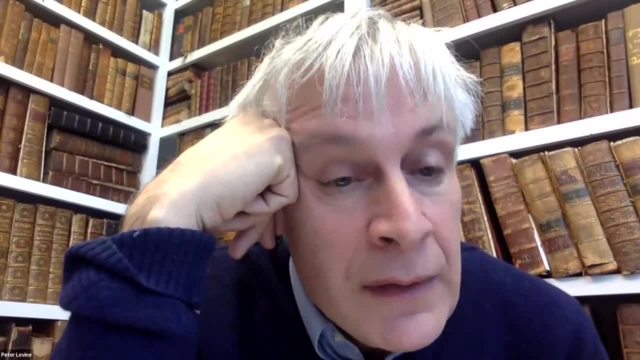 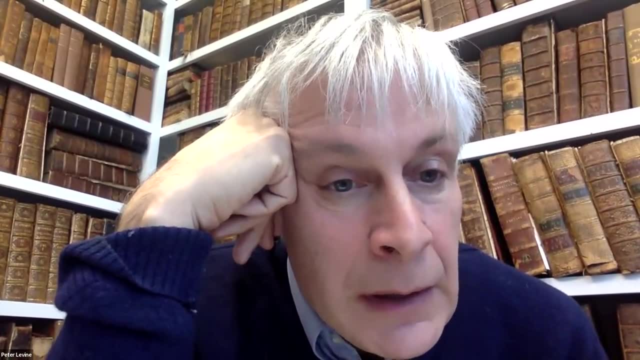 And, as Paul said earlier, that's not just on by any means, on the education programs and education schools and education departments. I mean, it's very much on the history department and the political science department in higher ed And, by the way, it's not just the teacher who needs it. 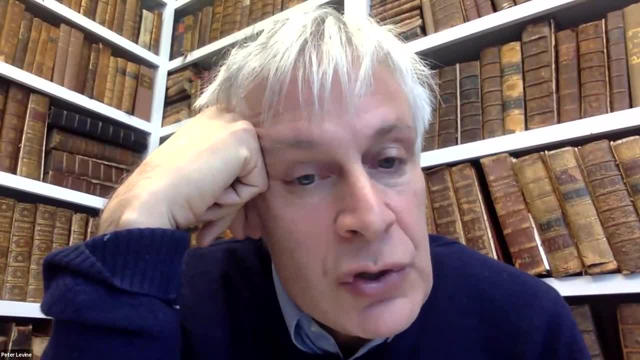 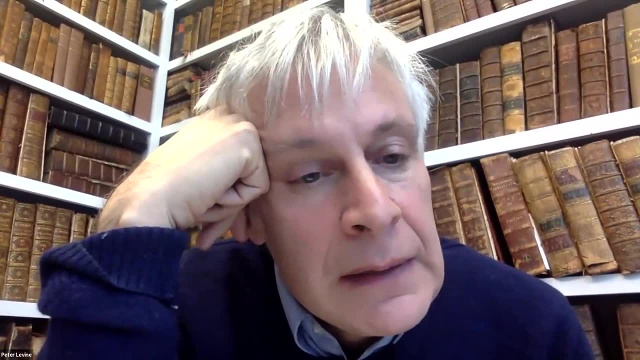 because we also would like the parents and others who have demand side pressure on the schools to have more content knowledge. So it's content knowledge. Content knowledge is my first bullet point And the second one would be the- and there are a bunch of people who are listening to this- 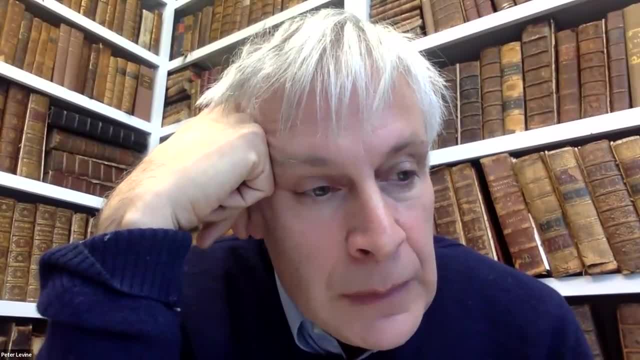 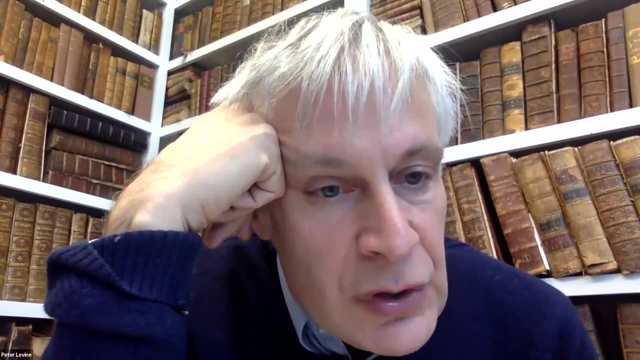 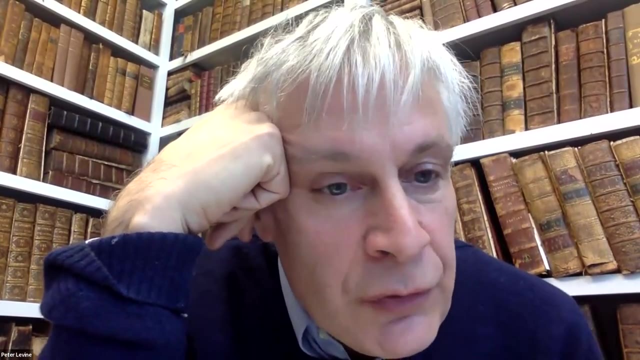 call who are real experts on this today. But pre-service and in-service education for dealing with controversy in the classroom, It's really, it's really challenging. You're talking about a situation that unfolds in real time. You can't prep for when the individual student says something extremely. 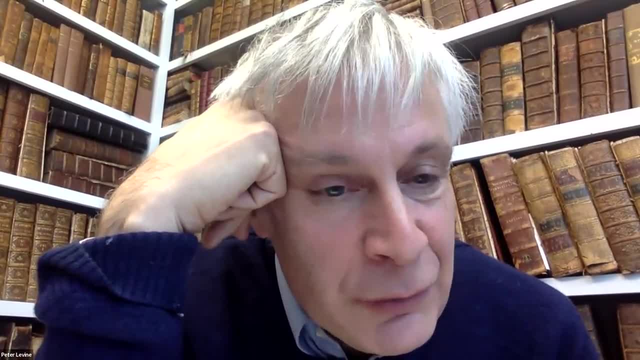 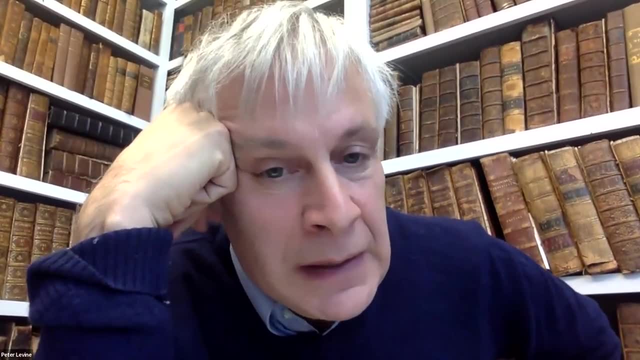 horrible about a category of other students in the classroom but exercising their free speech on a topic that you assigned. What are you supposed to do? And what are you supposed to do depending on the age level and the demographics and the content of the curriculum, and all that? 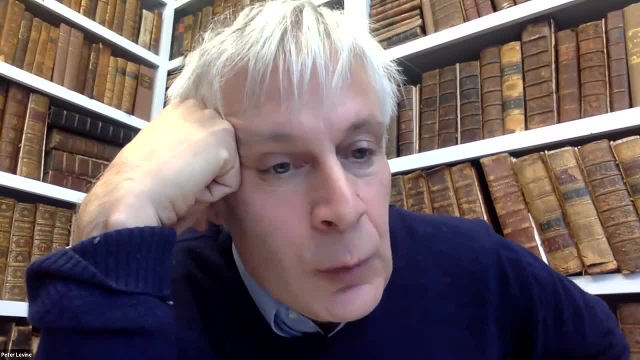 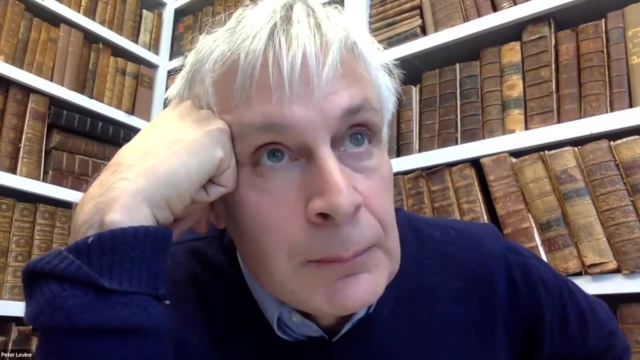 Yeah, I think you're talking about all kinds of other things And your relationship with the students and what's happened before and what's happened after. these are delicate issues and they can go badly quickly And I think you can't control those situations, but you can prepare for. 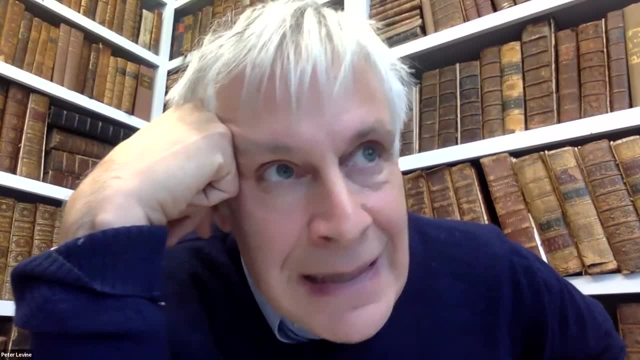 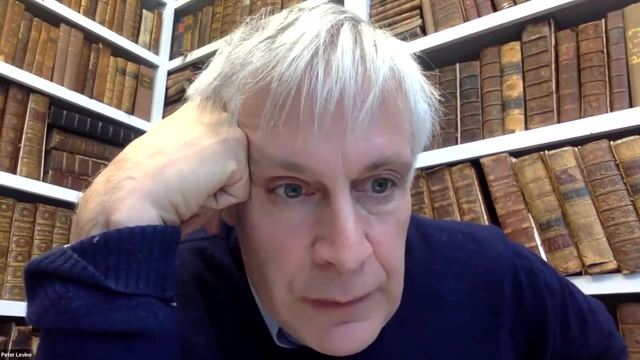 them and you can prepare for them with other professionals, And there's not much. I mean again, there's always positives out there in the world, But there's not much professional development, especially in-service for dealing with controversial current events. Thank you, 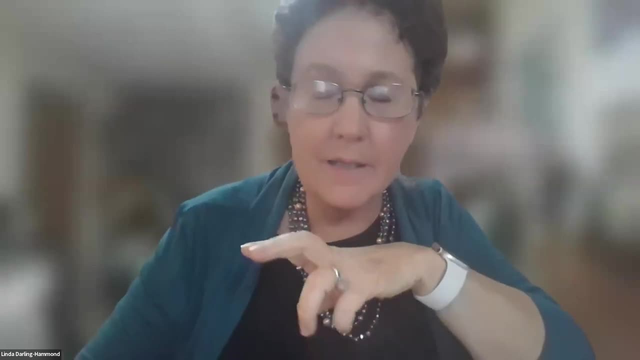 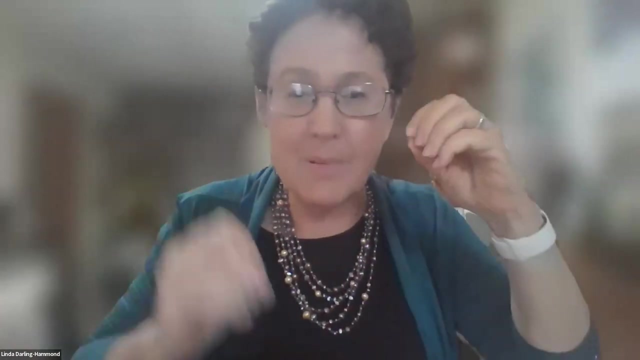 Just on the Go ahead, Leonard, linda, just at the point of um. how do you prep for that? i think um prepping for um, the controversial moment, or the you know thing that happens in a moment, um is one kind of prep, there's another. 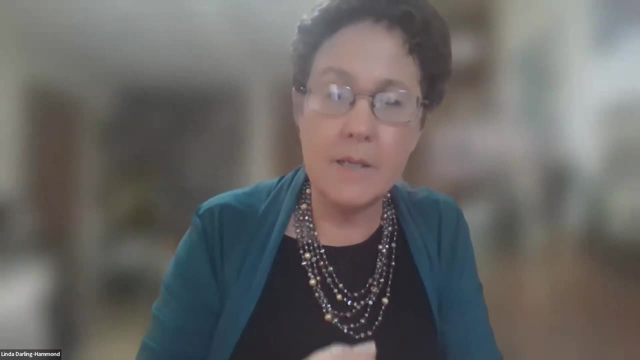 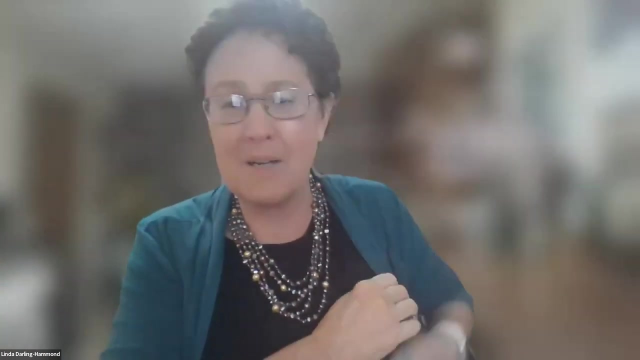 which is: how do you create a classroom community in which you can continually teaching the civic virtues and civic discourse that that is part of the warp and whoop in every classroom, in every content area, so that um people, so young children even- and i've seen this- you know um marvelously. 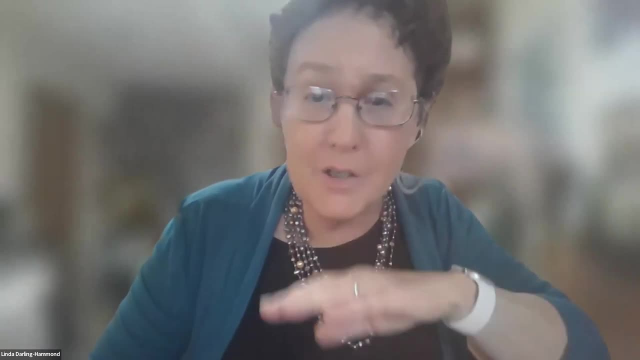 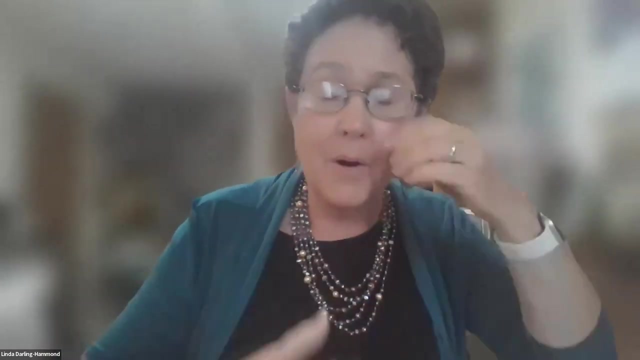 done in elementary as well as secondary schools. uh, learn how to talk to each other, learn how to deal with disagreements, learn how to be an empathic member of the community. part of that is grounded in deep understanding of the learning sciences that naela talked about earlier and then. 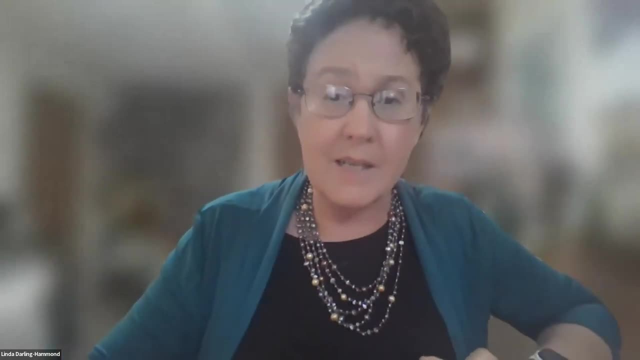 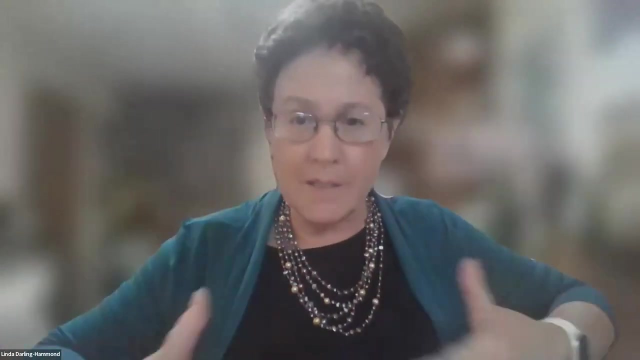 part of it is this set of you know um teaching strategies, um, that are both about the nature of the community in the classroom and then the way in which you manage discourse, civic discourse, and disagreements and so on. and then, when you get to that thing, that might first 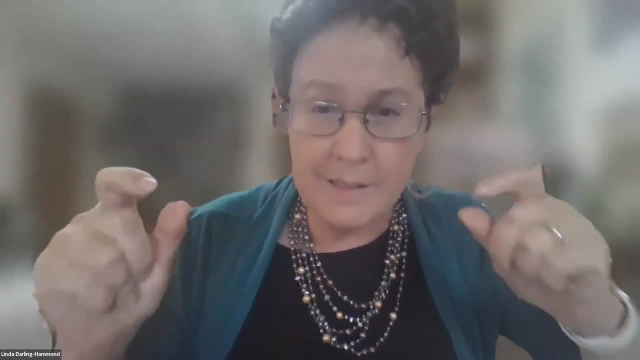 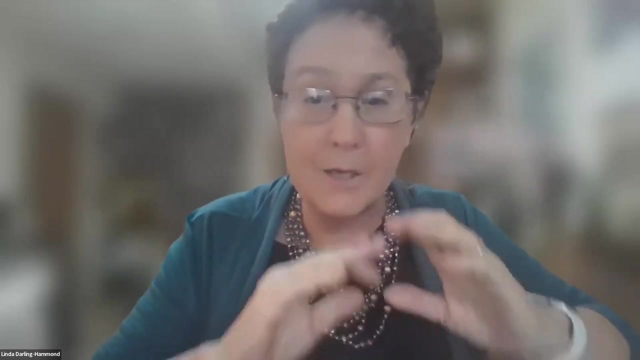 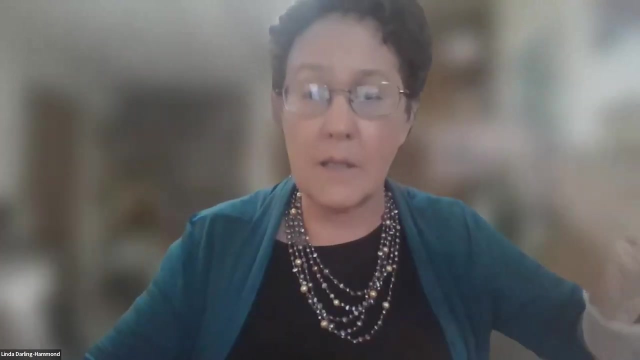 of all, you'll have fewer, uh horrific events where kids are, uh, you know, bullying each other or, you know, just being uh mean racist discriminator, whatever it might be, and you, when you get to moments that are challenging, you have more tools in the whole class to deal with them, and i think 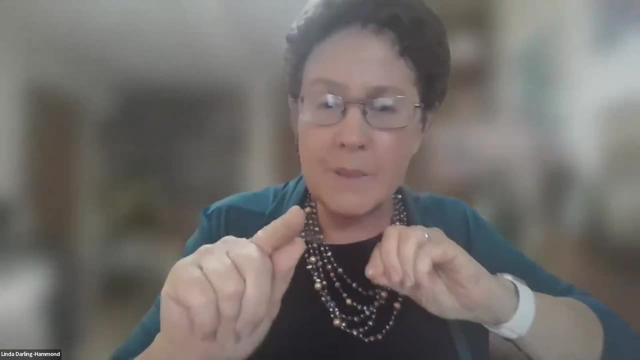 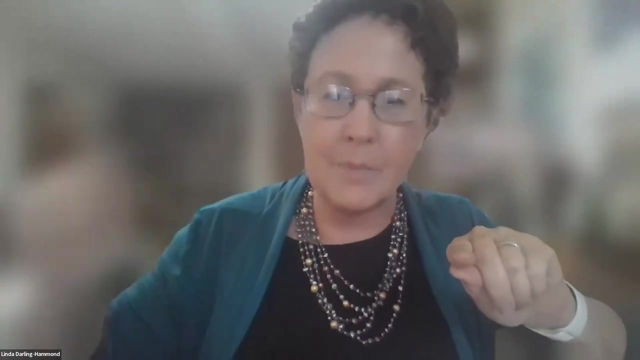 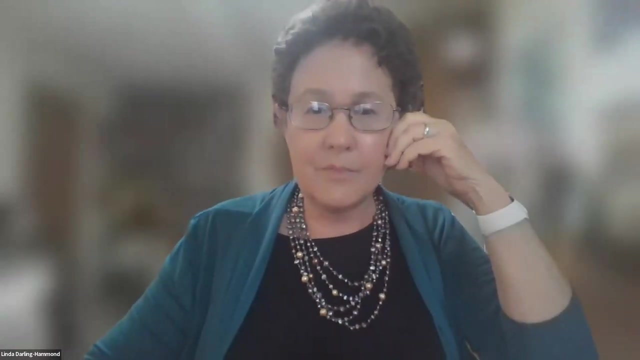 that's. you know there's. ultimately, there's a lot of evidence now that that doesn't take doing that doesn't take time away from academic learning, because it actually makes the academic learning more successful when you have done the work to create that kind of environment. i just want to note- thank you, linda, and everyone who's weighed in on that- that, um, just from the 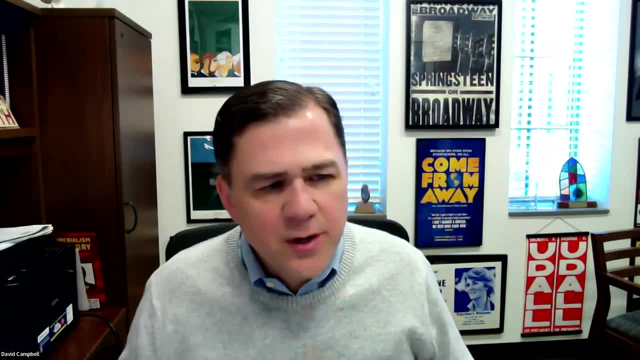 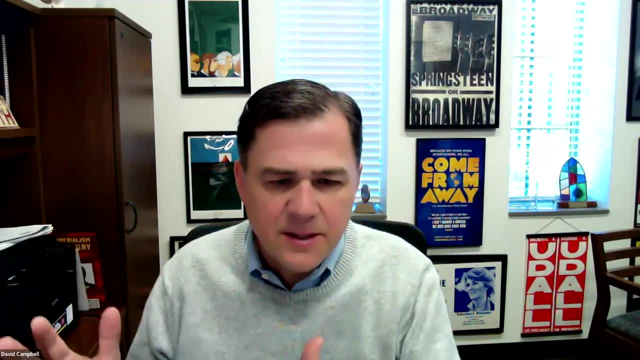 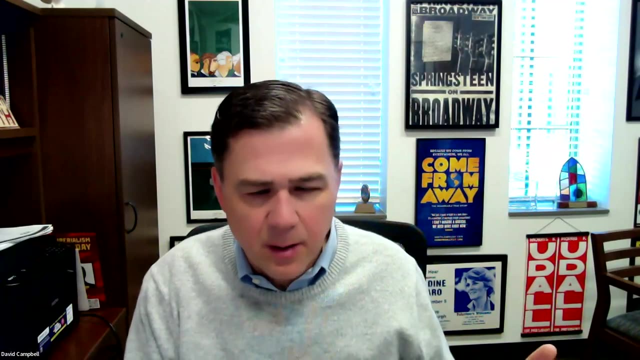 perspective of a political scientist. i i appreciate the emphasis that's been placed in this conversation on earlier grades than just high school. there was once a time in my own discipline when there was a lot more attention paid to what elementary age kids were learning about politics and civics and 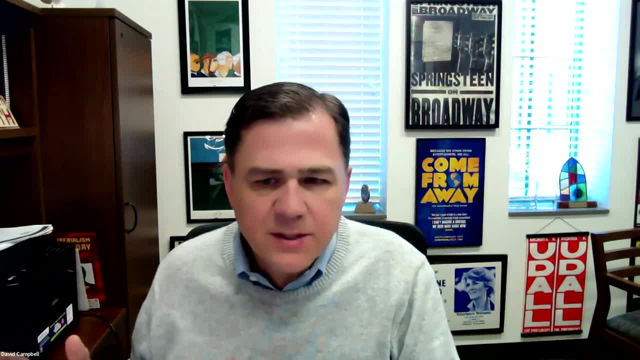 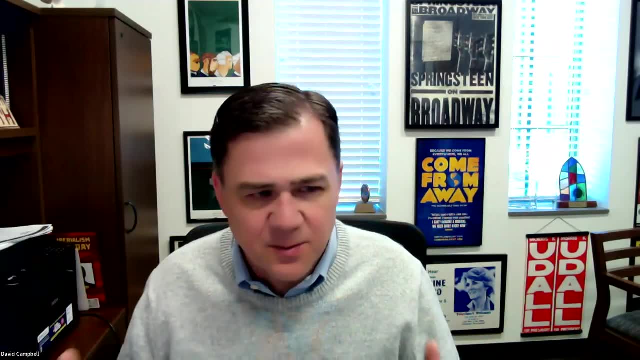 then that just sort of disappeared. there's been a slight resurgence of late, and i think that is all to the good, um, because, as we've just heard, that's what the learning sciences literature tells us we should be focusing on, and we should not be surprised that if we only introduce these. 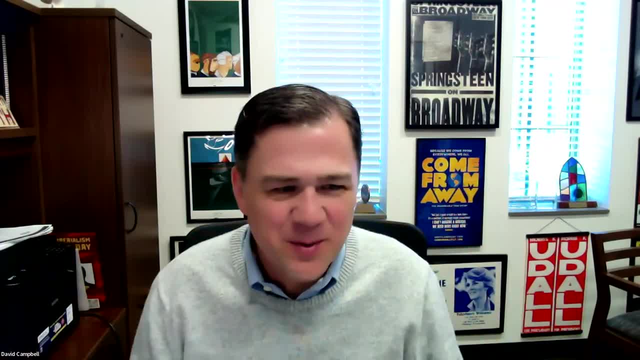 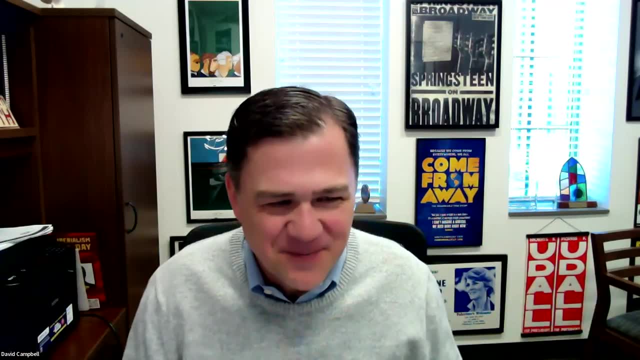 important questions of what it means to deliberate and reason with people you disagree with in you know, the 10th grade, that students aren't very well equipped to do it, that maybe they should start earlier on, and my sense is that actually good good teachers in the elementary grades are doing this, and so it's a matter of 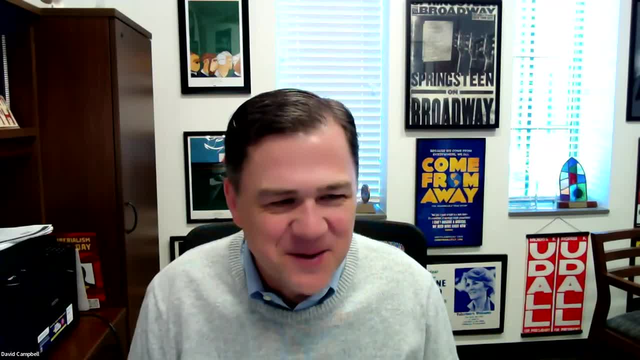 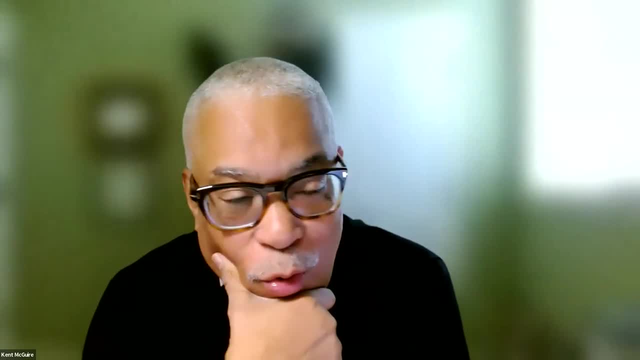 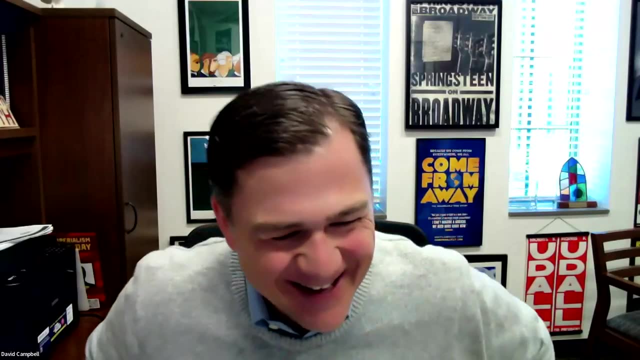 ensuring that they're they're supported, uh, in it, and that, you know, maybe even i have a. i have a five-year-old grandson. it sort of is proof, you know, that young, very young kids can argue. you know an agenda and, uh, you know, and a point of view that they're trying to, you know, to get across. 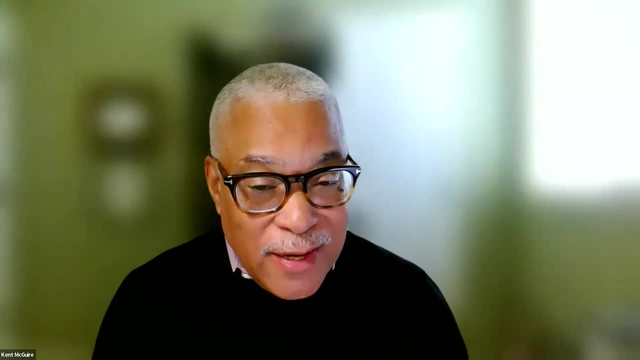 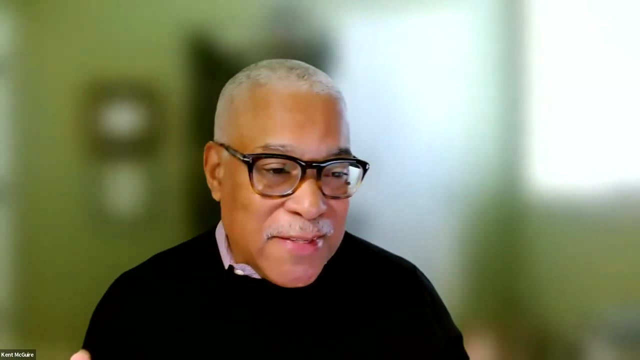 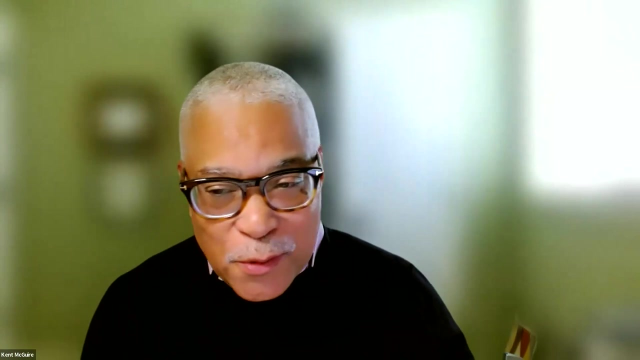 all to say. you know that i think systemically, uh, we've been in, we've left a lot of opportunity uh to get at these issues sort of on the table uh by not uh appreciating, uh you know, what very young children sort of bring with them, you know, into school and i think, unfortunately, you know, 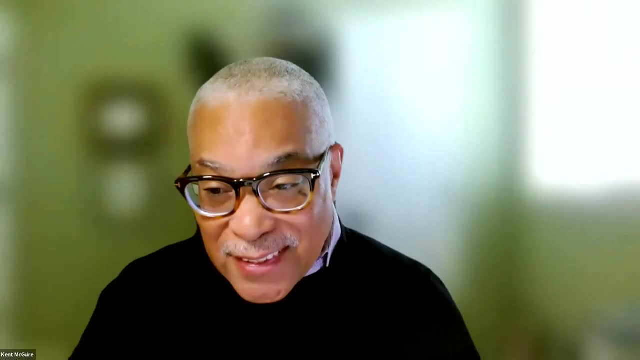 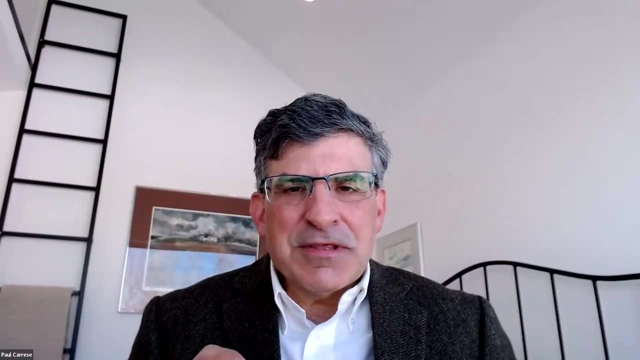 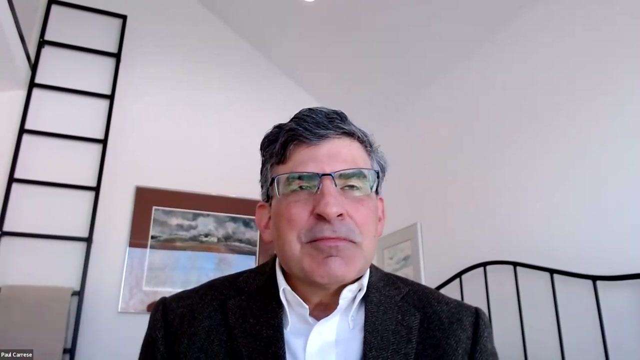 the current model grinds it out of them the longer that they're, then you know that they're there. that's, that's unfortunate. could i? could i jump in on the teacher teacher preparation question as a non-expert but a graduate of public schools and actually also respond to something nyla brought? 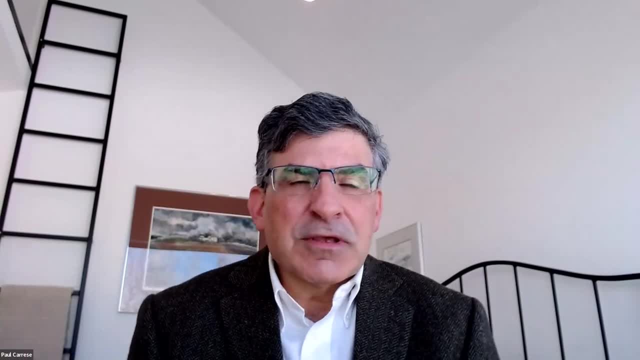 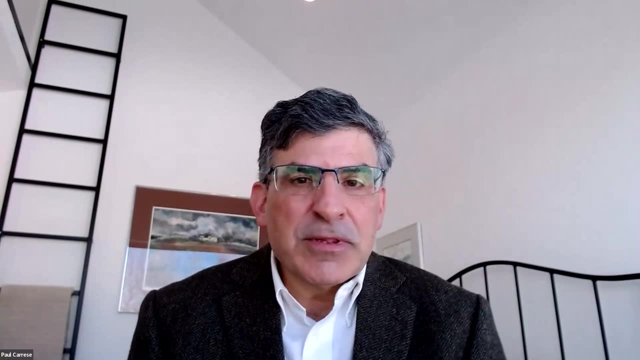 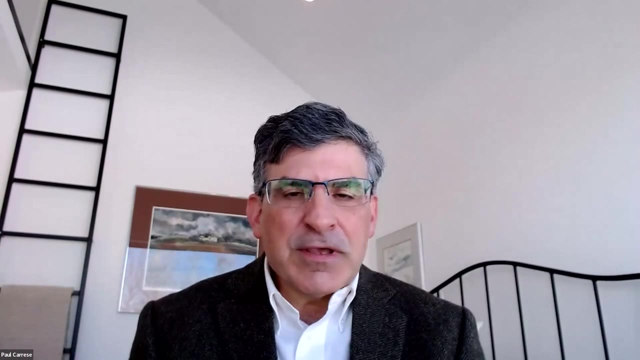 up earlier about the struggle of reflective patriotism for many people in the country who think that america is not such a promising place. america has crimes and errors and failings to the present day and address it this way: that teacher, as peter's saying- i've written this elsewhere- the 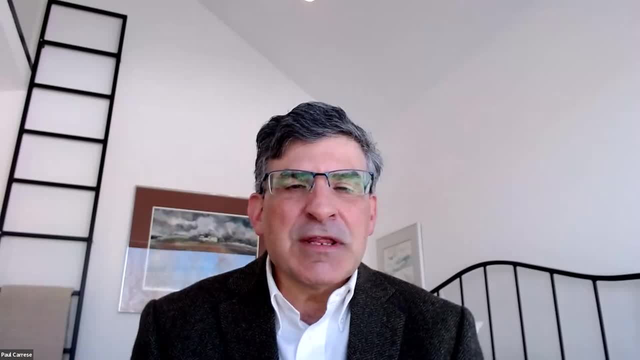 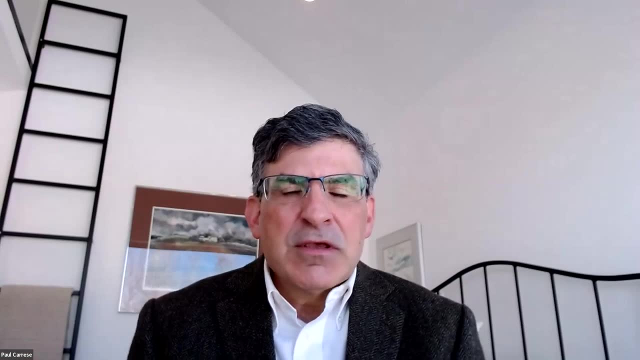 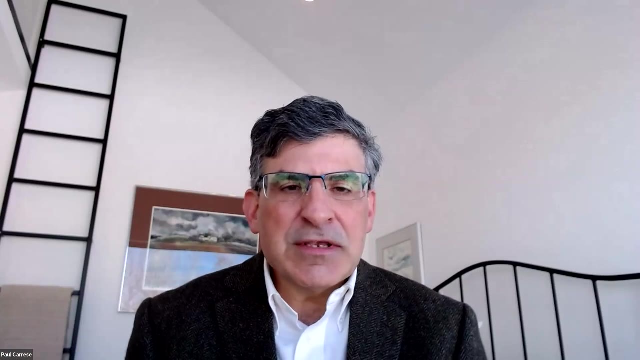 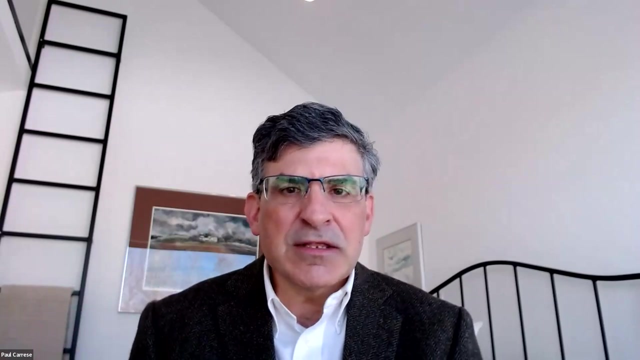 ead report writes this uh: that teacher preparation cannot be left only to the education schools and the teachers colleges. obviously they're focal to that, but the, the entire culture of a university, of a college, has to support civic education and and preparation for being citizens in the fullest sense of that self-governing. engage uh people with civic virtues as well as civic. 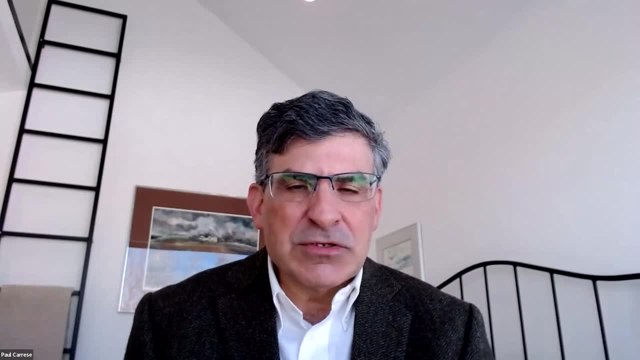 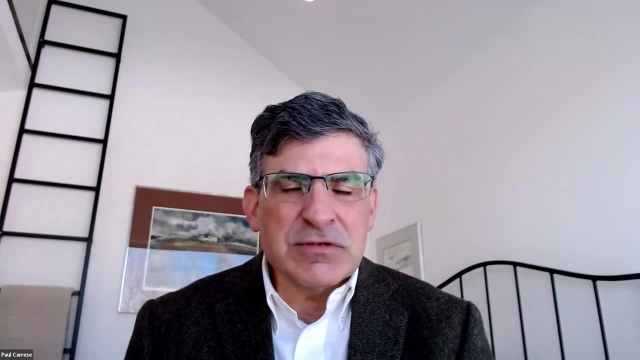 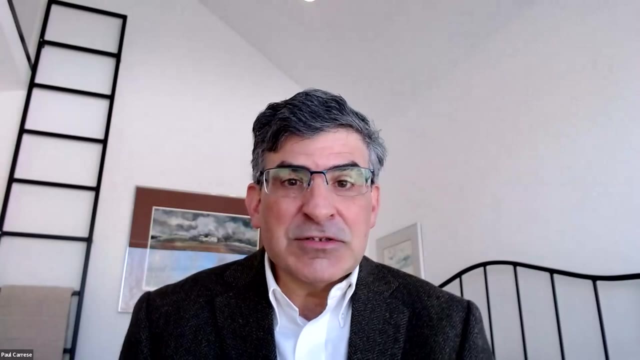 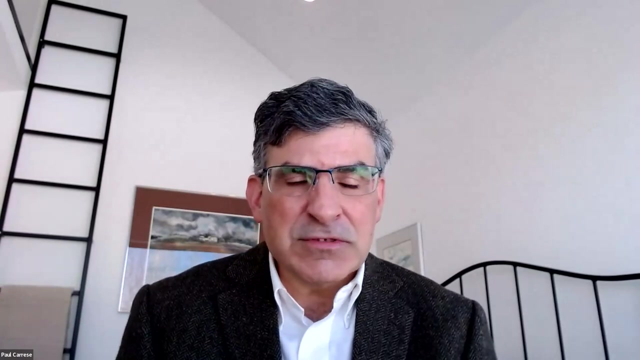 knowledge. so the the whole, the challenge of being a teacher in elementary school with some responsibility according to state standards or district standards for civics and and social studies and history education, uh is such a great challenge, and especially in the way that the the educating for american democracy report talks about it, that you teach about disagreement. 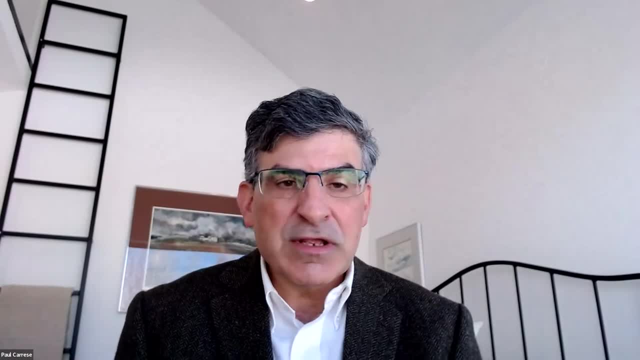 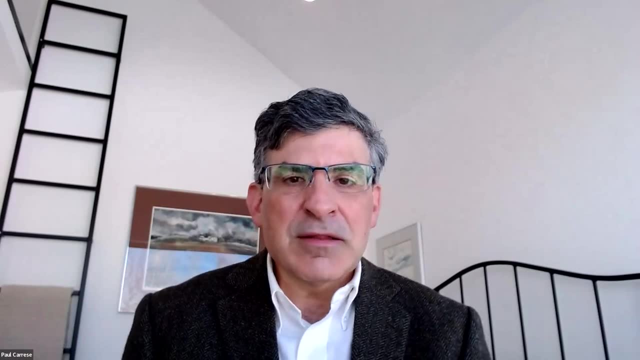 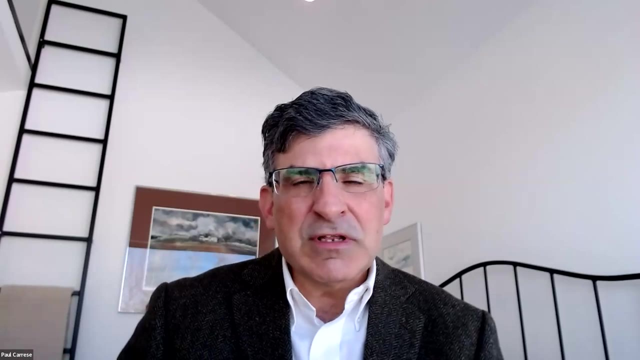 as a reality and you teach about particular disagreements and you try to develop both the knowledge base and and the civic virtues to to deal with that and and be productive. such a challenge that that's why, uh, you can't leave it only to a specific set of classes. 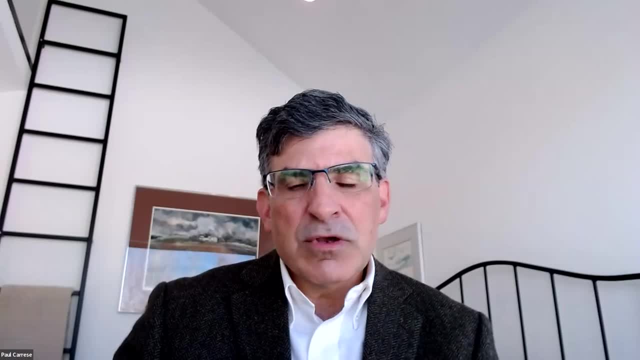 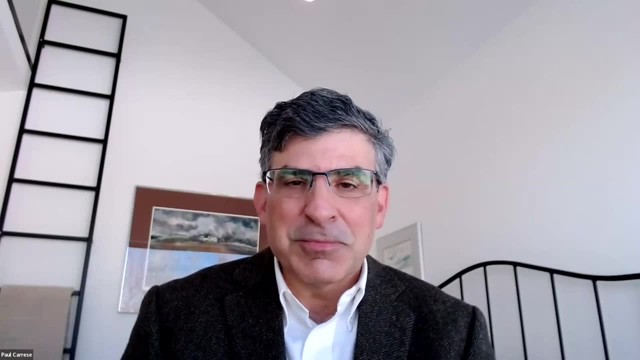 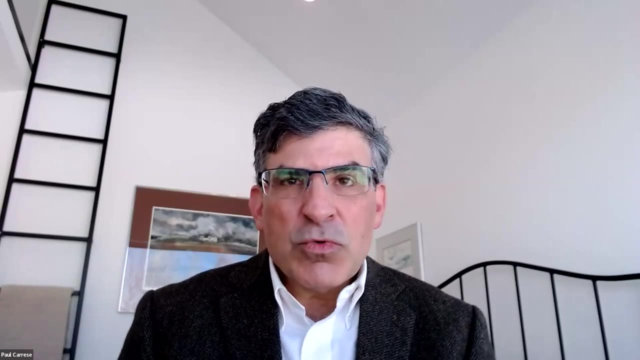 in teacher preparation coursework or even to in-service uh work. there has to be discussion about what is the, as peter mentioned, what is the role of the political science department and the history department, the philosophy department and other courses? what are the general studies requirements? i'll mention one book that came out just as we were finishing the decay: 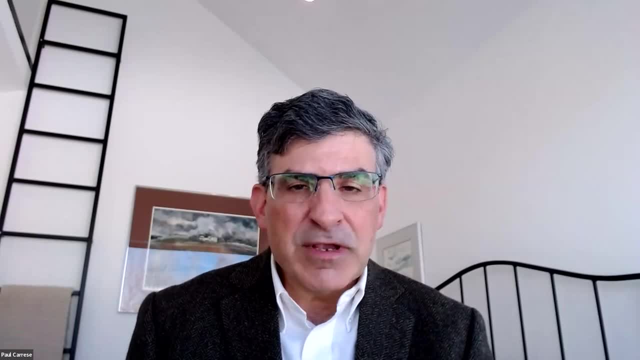 study by the president of johns hopkins university of all places right, the first research university in the country, and the title of the book is: what universities owe dependent democracy? And his answer is: every college and university, large and small, public and private. 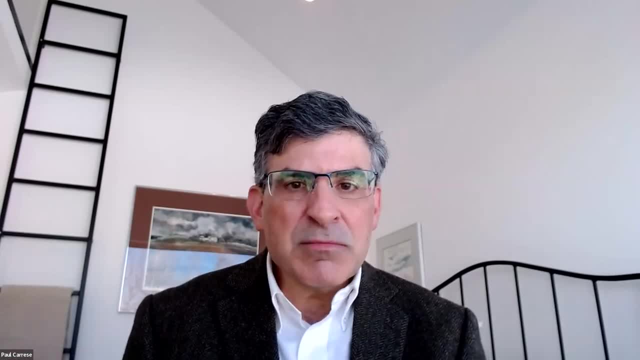 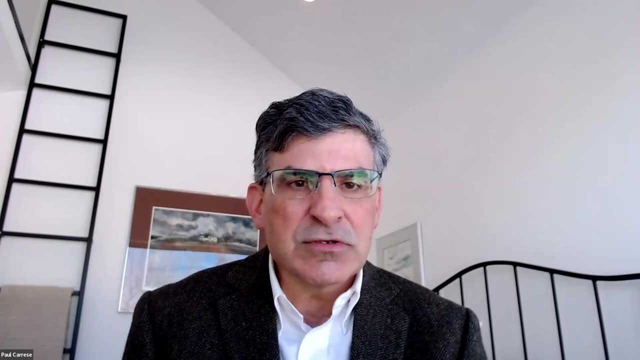 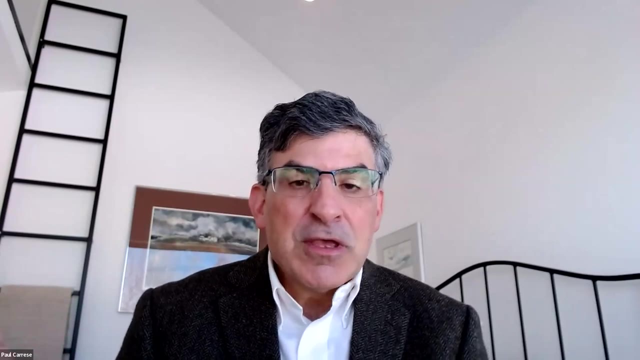 owes an excellent civic education, with at least a minimum of one course or two courses in fundamental civic knowledge about liberal democracy, American constitutional democracy, but also then broader ways of providing. he calls it pluralism, purposeful pluralism, providing the civic virtues. 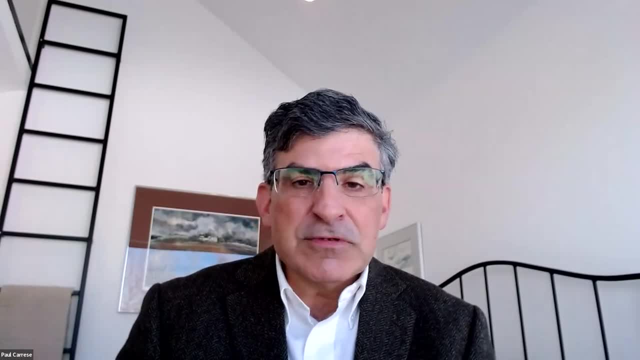 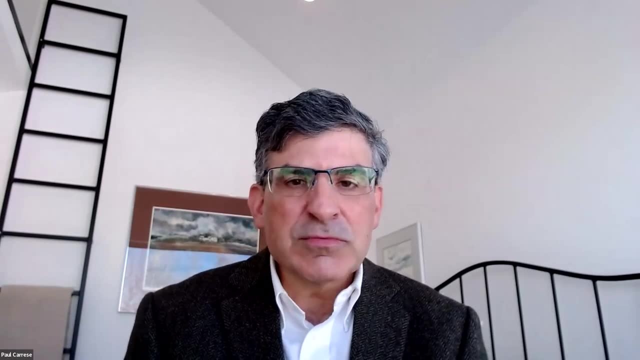 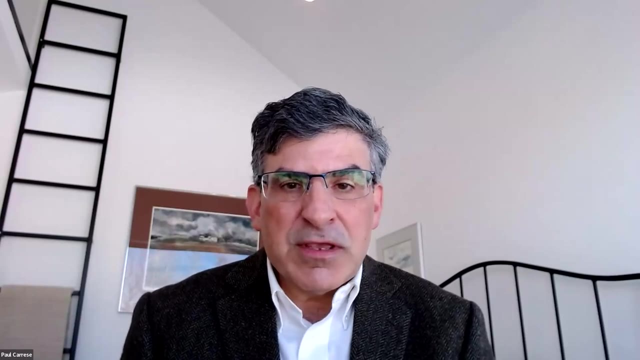 of understanding that there are free people who disagree, and what are the skills and the habits and dispositions about civil disagreement and hearing a diverse range of views and being able to respond constructively. So this is the civic crisis we are in, of our civic culture. 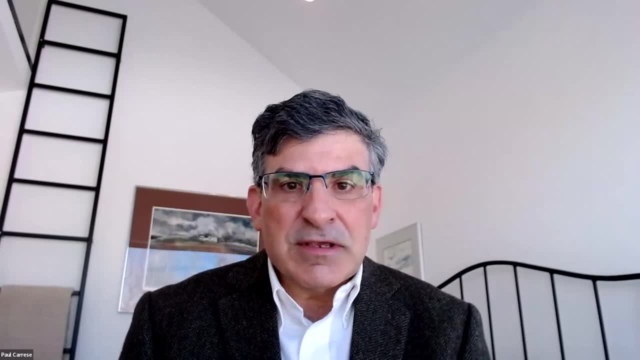 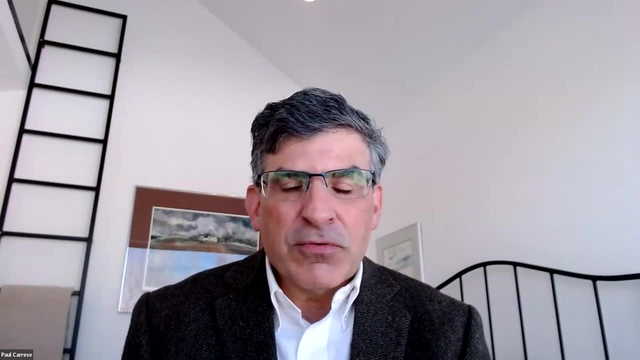 of civic knowledge is very serious. It's in the EAD report. I think we used- or maybe I'm just thinking we talked about it. we use the Sputnik metaphor. This is a real crisis. The difficulty for American culture is that the threat is our own set of. 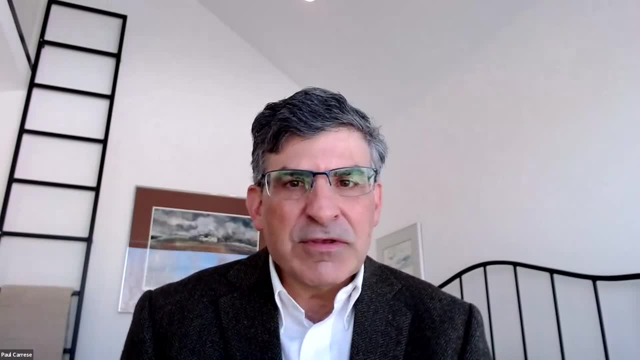 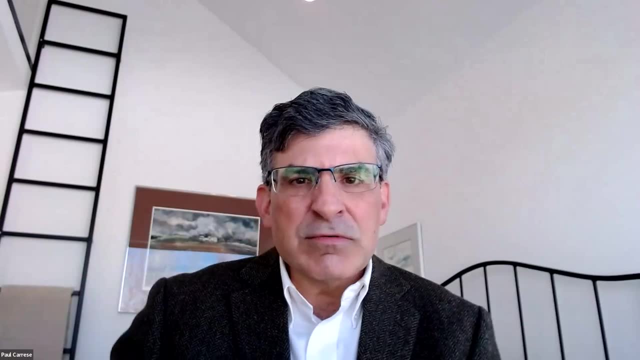 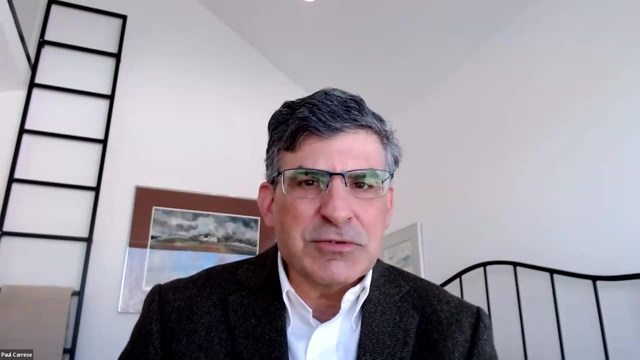 failures and our negligence about civic education. The threat isn't external. In the Nation at Risk report in the 1980s, the threat was external: These nation states and economies that we rebuilt in West Germany and Japan and South Korea. well, they're suddenly kicking our butt in economic 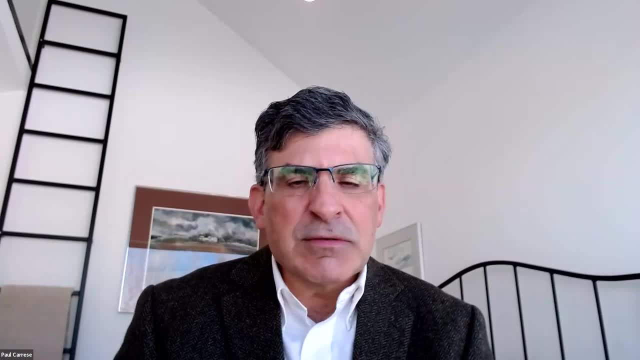 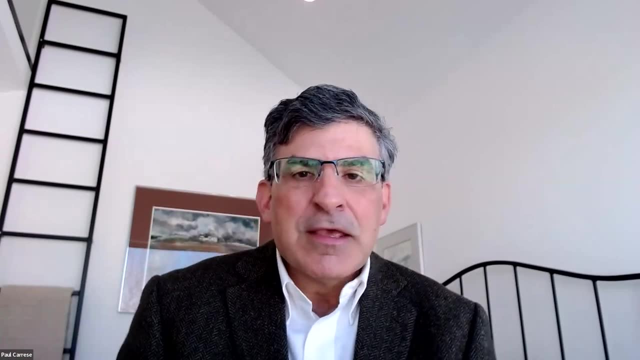 productivity, And so we have to focus. We have to focus on those kinds of academic subjects in the schools. The challenge is more like what Lincoln talked about in 1838, his first great speech as a nobody but as an aspiring politician speech in 1838 on the perpetuation of our institutions, called the Lyceum Address. 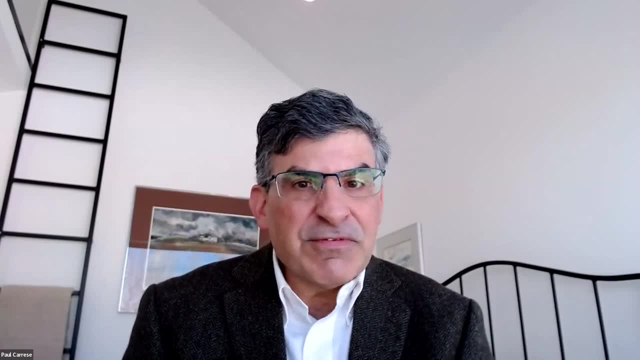 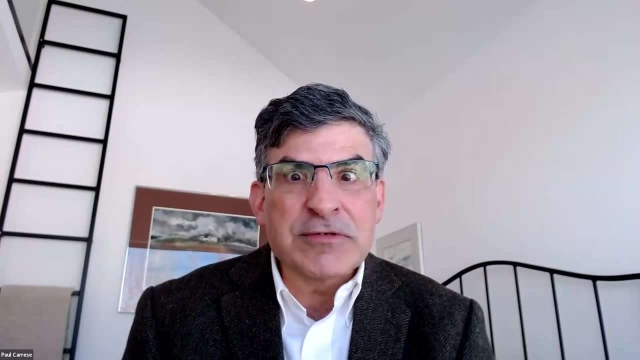 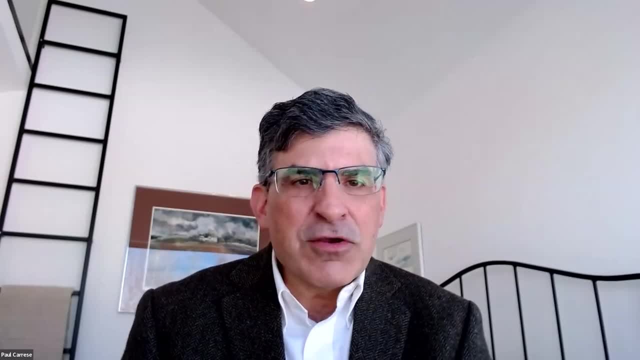 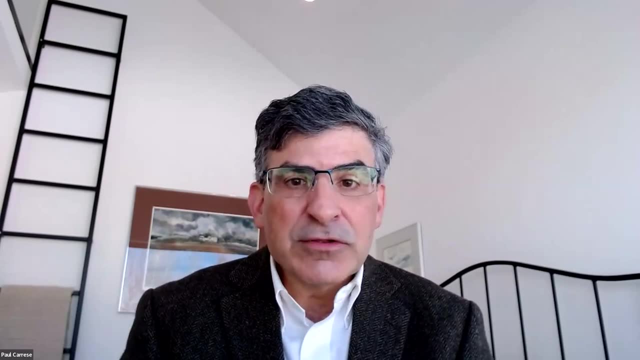 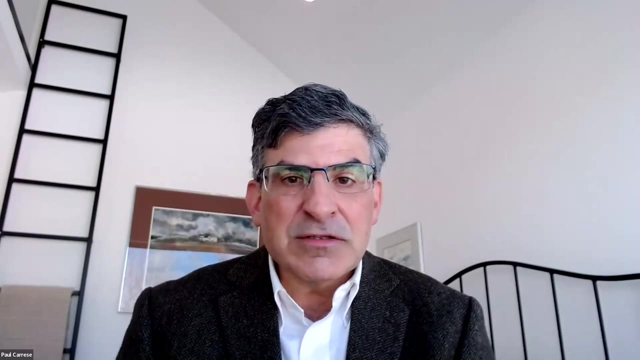 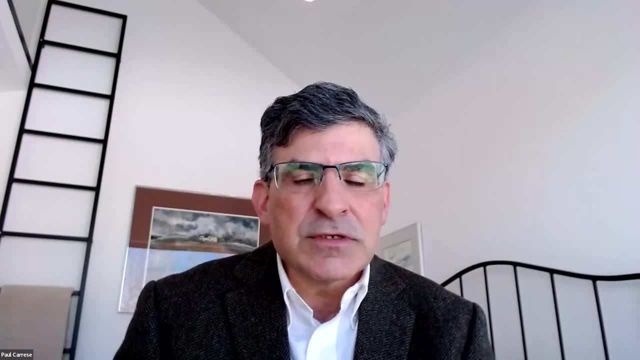 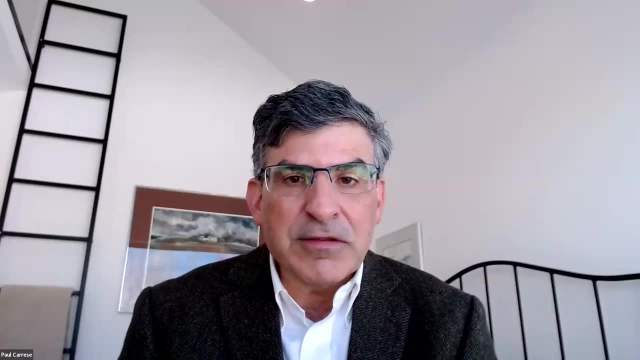 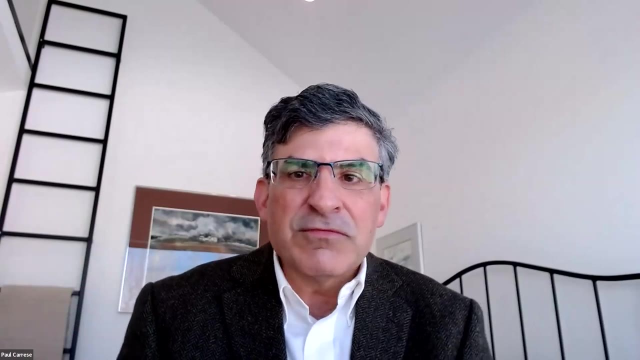 colleges and education schools, or just put it, on the K-12 schools and boards of education. We need to rebuild the whole ecosystem. Who's sitting on the board of education? Who are the parents? Who is the? if the principal has a degree in chemistry, you know what should their real 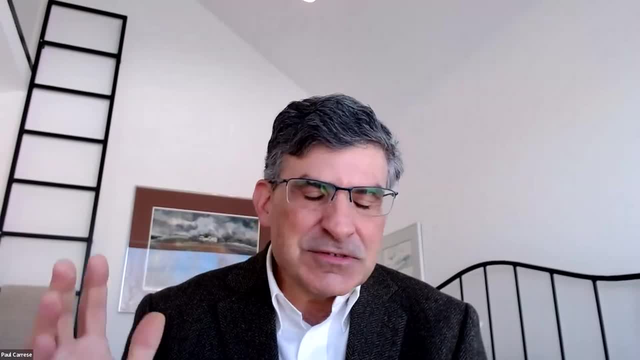 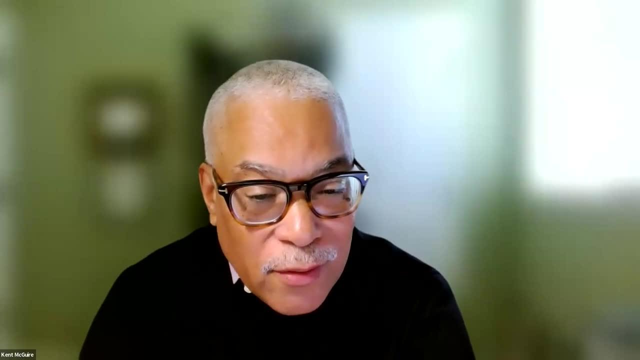 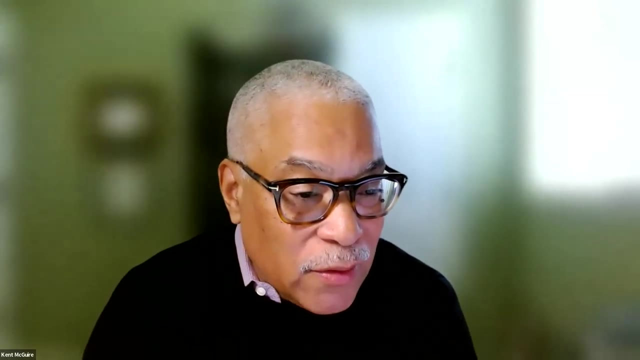 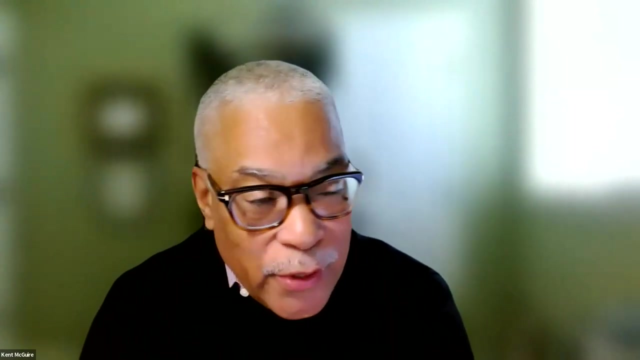 investment be in civics and history education. So, David, I know you want to get to the Q&A where there's a bunch of stuff there, but I just want to appreciate Paul's last point about the kind of responsibility and opportunity You know. I think you know the opportunity to get better at this doesn't rest solely you know. 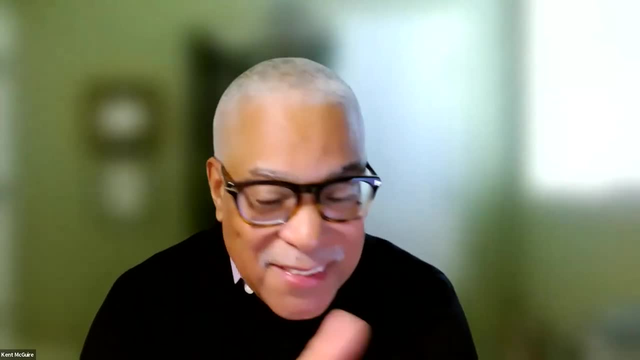 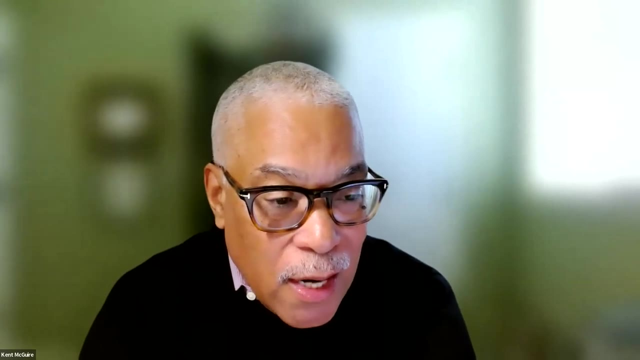 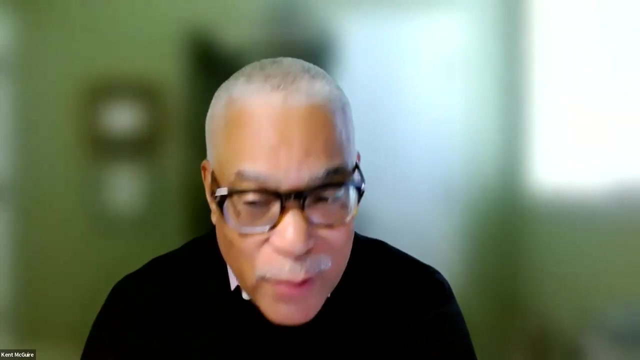 with, you know, with ed schools, even though there are lots of things that ed schools can and should do. I think to Peter's point to to get at it, But to the extent that the K-12 system gets its signals from higher ed, we could do with a better set of signals, You know, that'd probably help us. 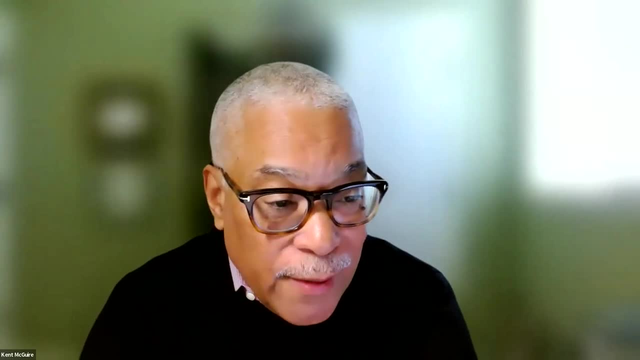 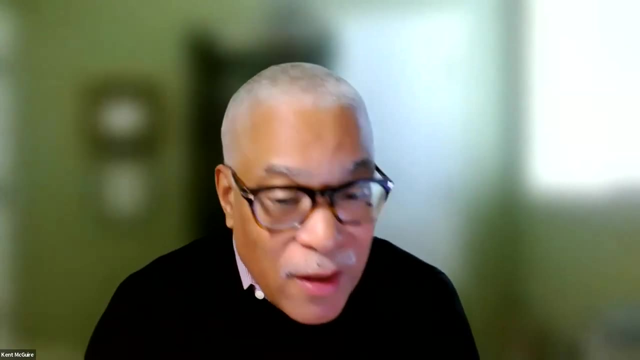 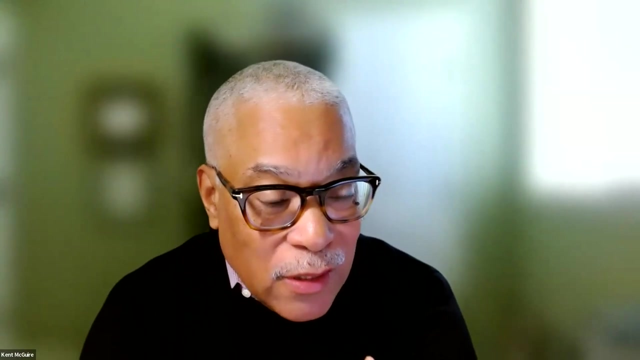 in lots of ways. You know we could do with a better set of signals. You know that'd probably help us in lots of ways On the policy front. it wouldn't hurt if we did have standards that you know looked and worked more like the. you know what is implied by EAD. But I think, Peter, 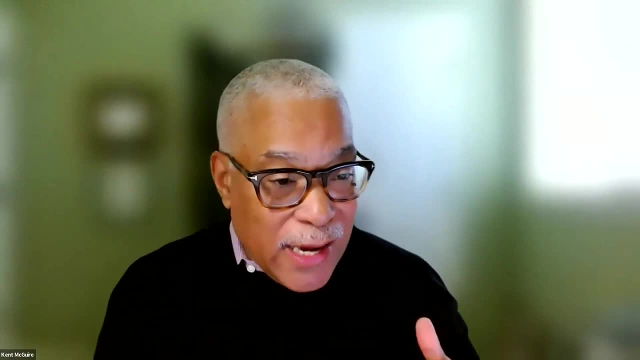 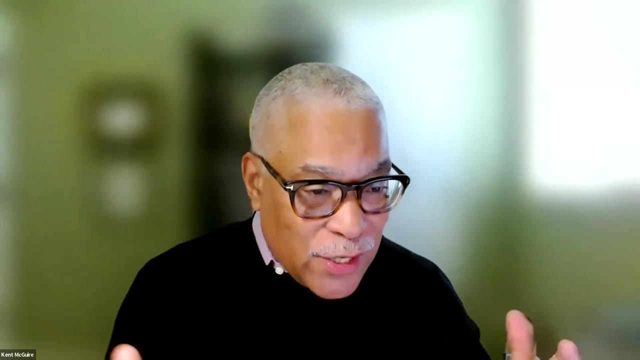 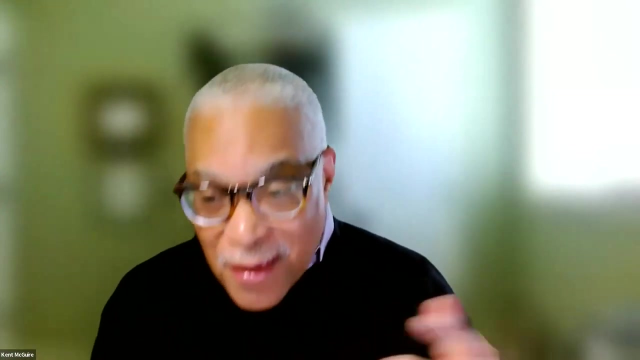 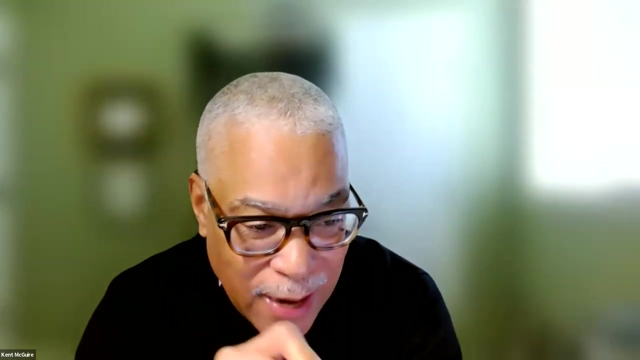 was suggesting. right now they're sort of all over the place and probably the weights are set a little more toward knowledge and facts than what to do with those facts. But but attention there would would help a lot. I could say more about it, but I'm sort of interested in helping. 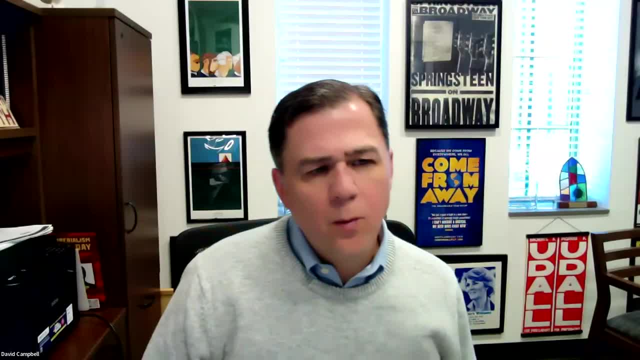 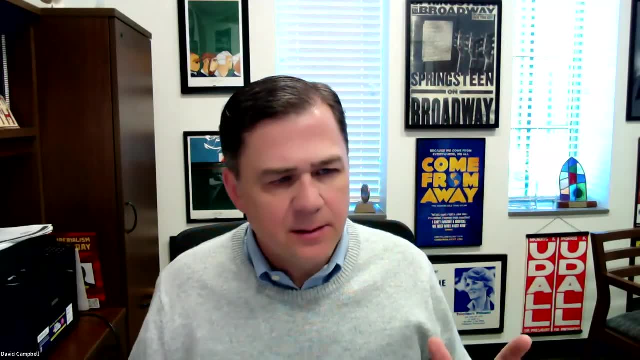 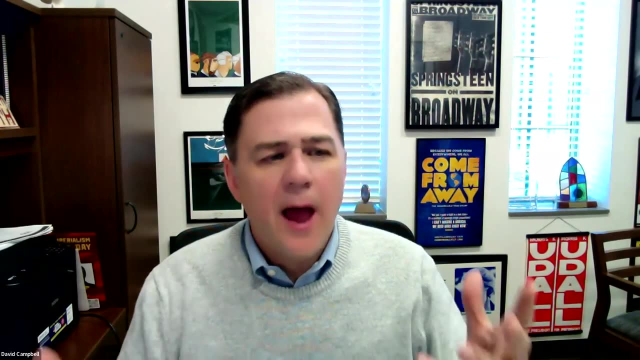 you get to the audience. So what I'm going to do is, rather than extend our discussion of possible policy levers, I'm going to move to the Q&A. Ken has already alluded somewhat to public policy. As our panelists are responding to the 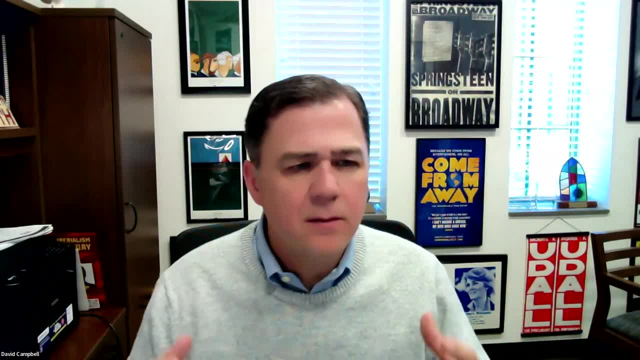 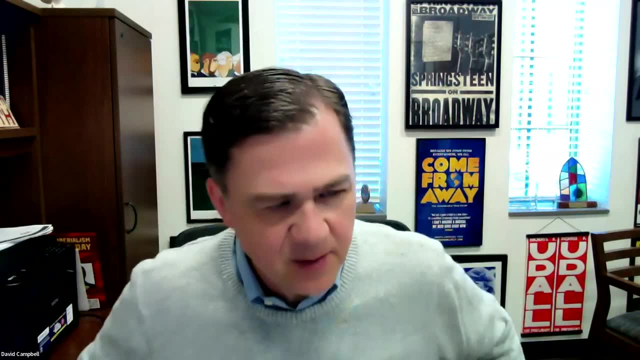 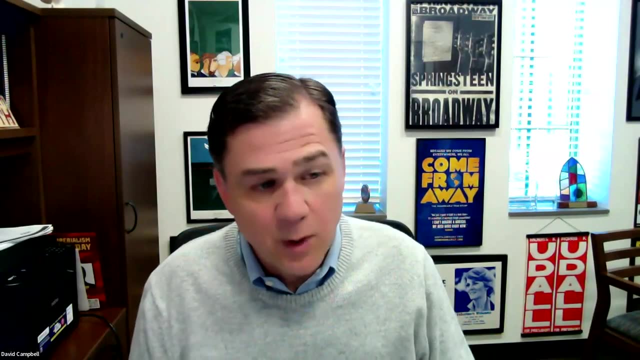 questions that come through the Q&A. keep in mind the policy environment, what might be done in state legislatures or even by the federal government or the local level, wherever the right level of government is to implement effective civic and and what? what they might? 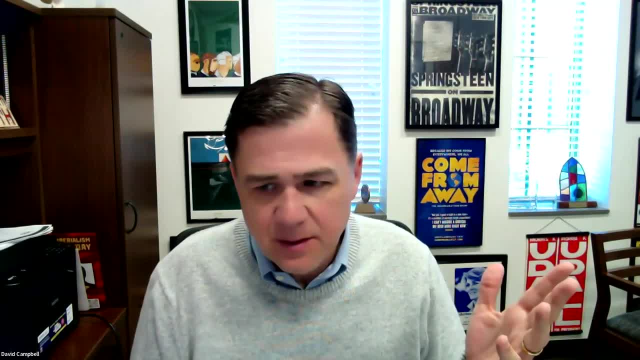 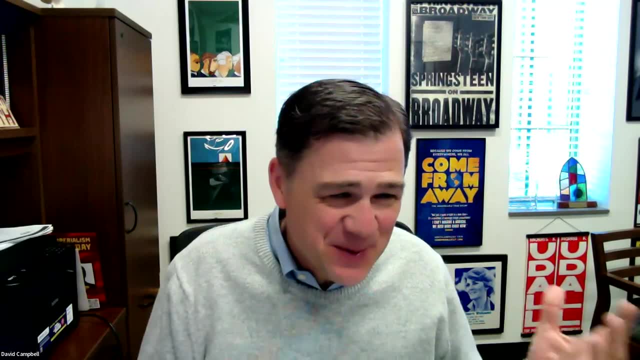 be doing Again, just as a reminder. lots and lots of questions coming through the Q&A. They're actually being moderated, So hopefully we will cover as much as possible what people are posing. but we may not get to everyone And I do apologize for that. But I want to start with a big question that came up earlier. 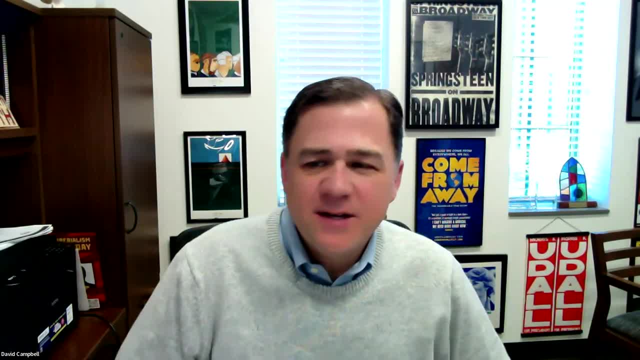 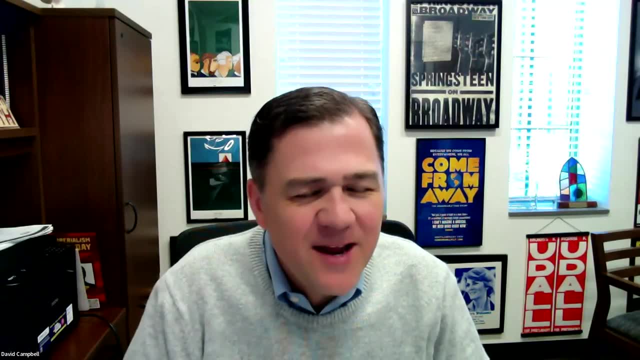 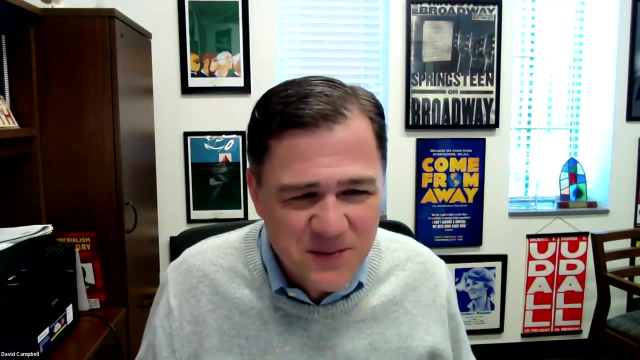 on that, I've sort of kept in the hopper. which is: what do we mean by a democratic crisis? Already, the theme of a nation at risk from the 1980s has come up and some people have posed in the Q&A the question of: is this just a nation at risk? 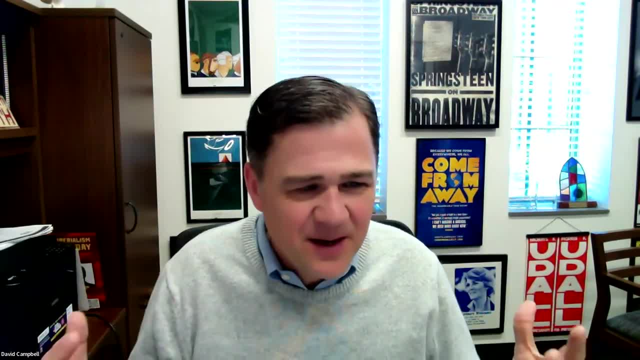 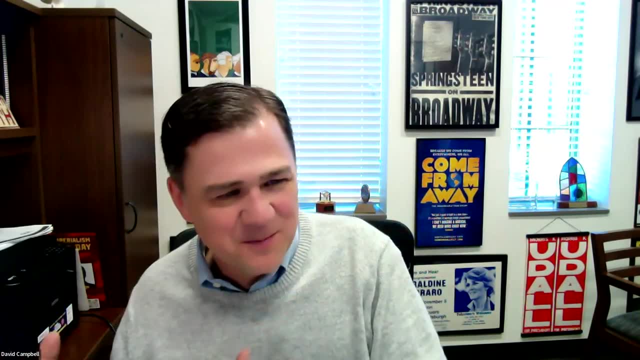 Is it all over again? Is it something different? What do we mean by the crisis? And I think by clarifying that, it'll help us address. well, what are we going to do about it? So let me just ask: what is the crisis? I've been appreciating those comments in the in the chat because I think it's 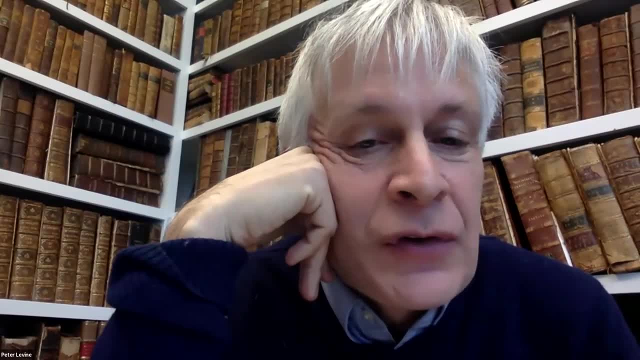 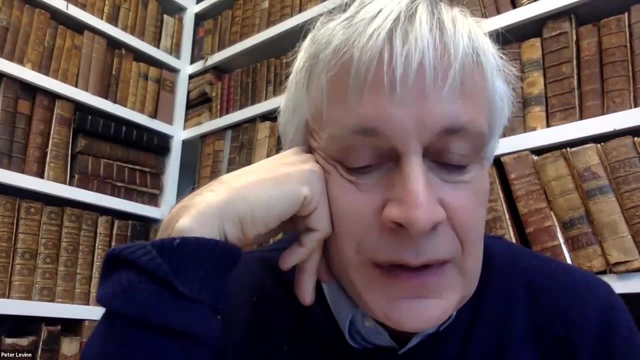 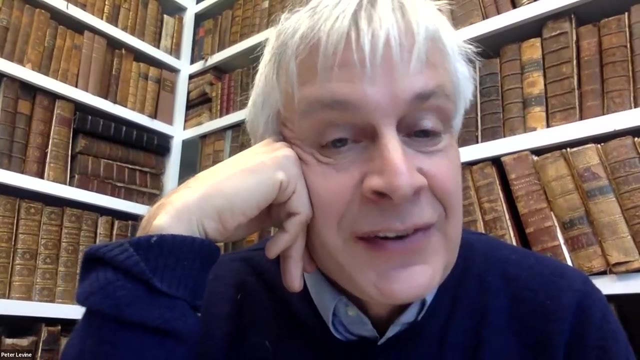 good to be critically questioning what the crisis language is. It's a rhetorical move that we, what we make in just in public life, we call things crises And I think it's it's worth asking whether that's what we have. I would. I would say we should be working on civic education. whether or not we, it's a crisis. 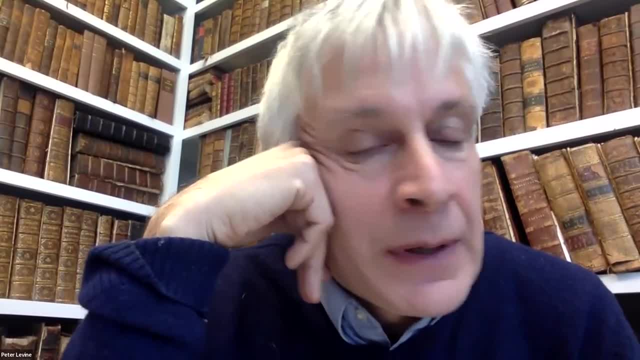 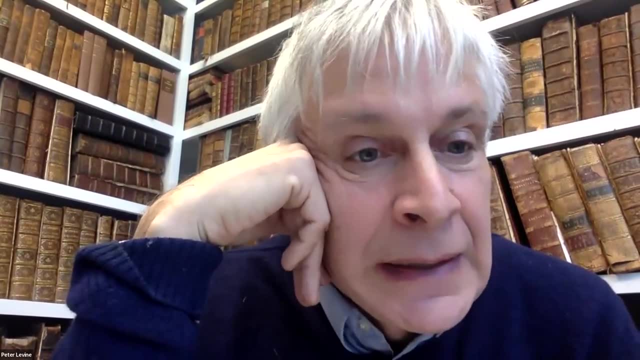 I've been trying to work on it for a long time. I also have been on this call and other work trying to take a kind of glasses half full and asset based attitude towards the education part of it, Because I think sometimes the crisis language ends up implying that everything's just completely. 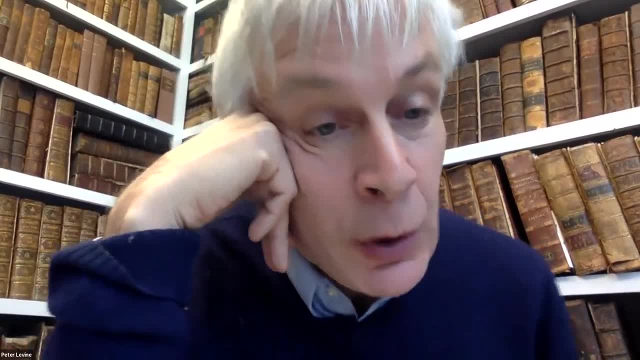 terrible in the on the K-12 side, And that's not not a good place to start. It's just not true, And it's also not a not a where to nowhere to go from it, And I think that's a good place to. 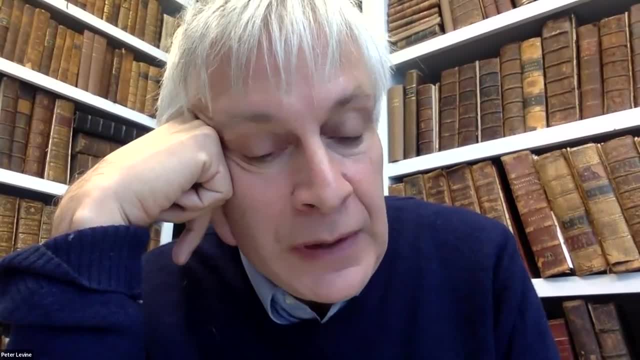 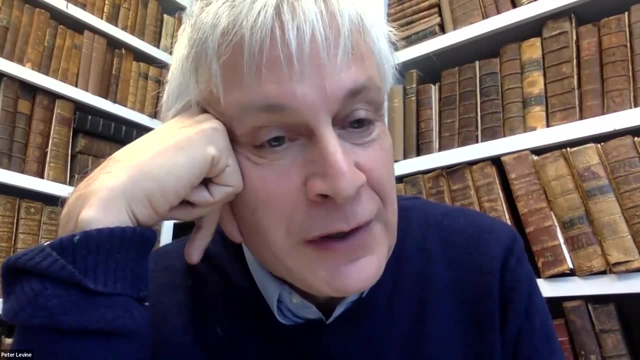 go from from there. But I would say just kind of atmospherically I think I mean, David is a political scientist. There are a lot of really distinguished political scientists on the call listening to us, So I better better answer this as well, But I do think there's just a. 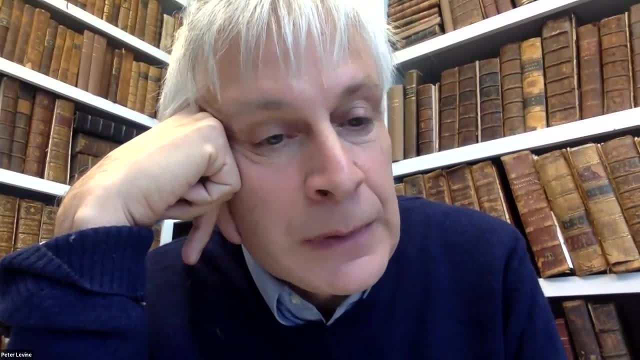 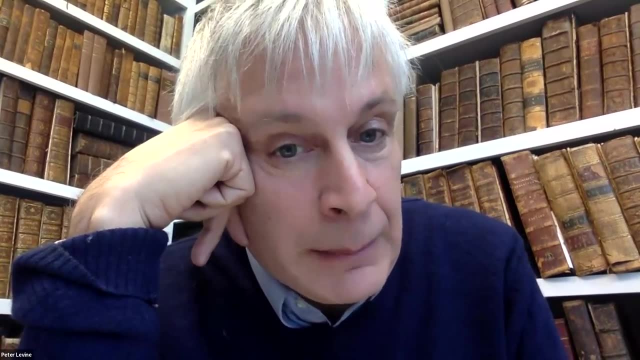 a sea change. you know, for many years the general assumption in political science was that we had a, a stable political political order, a stable constitutional regime. It might people might be very critical of it and actually upset that it's so stable because they might see built. 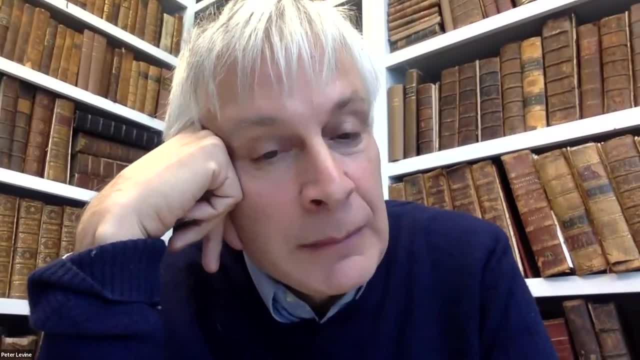 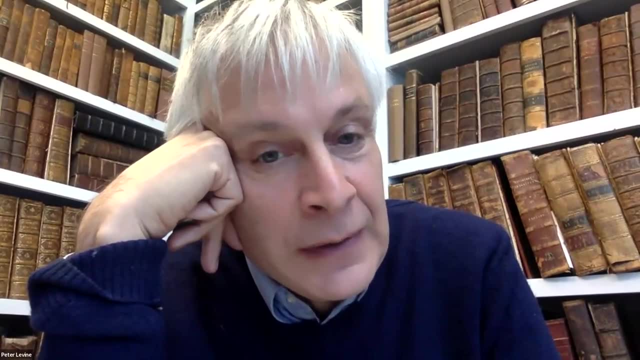 built-in injustices, but people thought it was stable And at this moment, books like How Democracies Die and The Four Threats, and these are, these are, I'm naming political science titles that are extremely influential, And I I mean there's a debate about whether we're in a 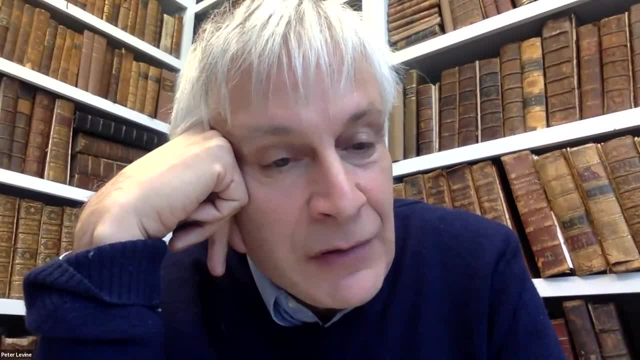 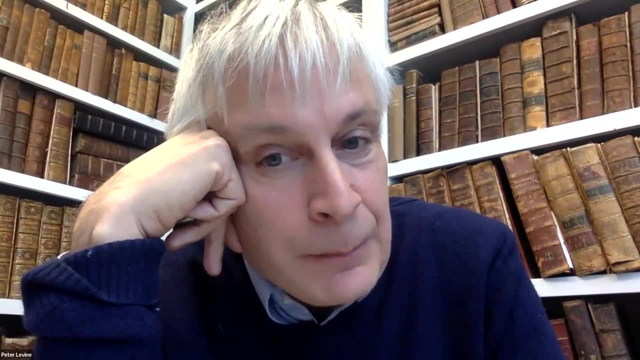 crisis and and we shouldn't foreclose the debate or pretend that it's just obvious that we are. But I think it's very interesting that the that the concern is about the fundamental stability of the political order. Some, some people also thinking that it'd be good if it, if it ruptured. 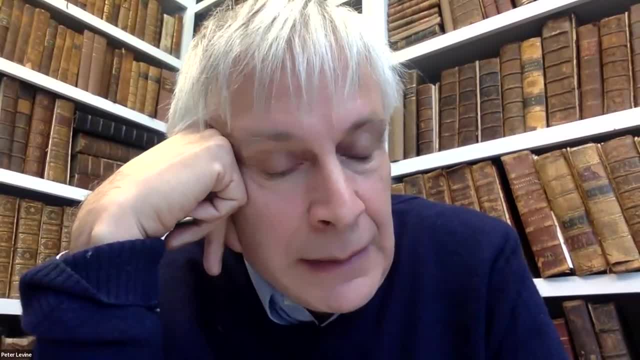 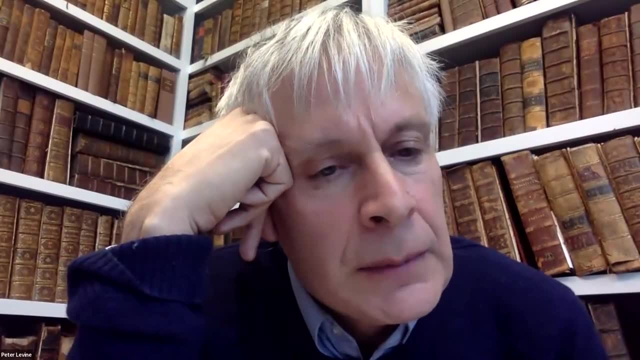 uh, because we could get to somewhere better. That's, that's certainly a line you can find, but, um, that's just a sea change And I think it changes the way you think about civics, because it used to be. this goes back to a point made much earlier. Um, maybe it might now, you love. 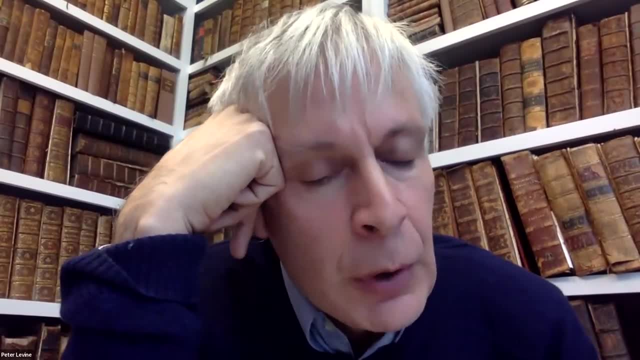 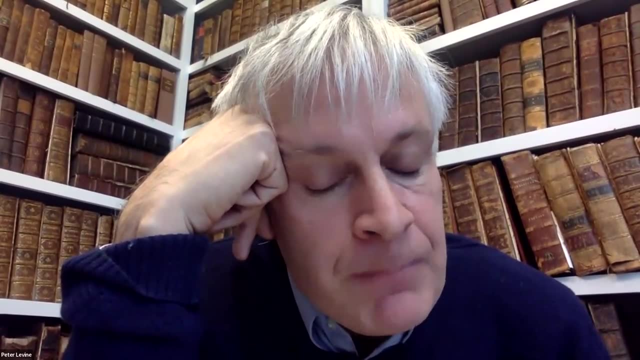 I can't remember who about sort of is um is is promoting, uh, or maybe it was on the. it was when we were prepping for this call. not on the call, but um, whether, whether, um. 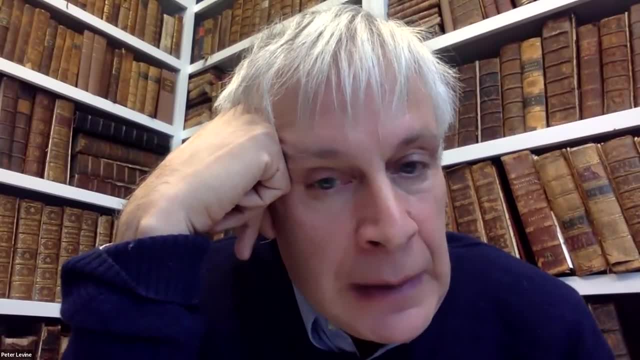 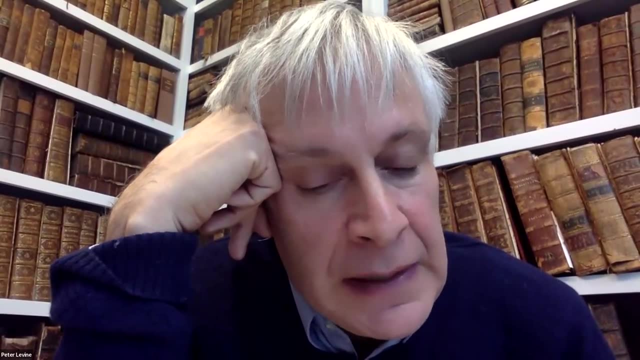 encouraging participation is what we need to do. Uh and I- I would just describe that. my own perception of the field over 25 years is back in the day in the late nineties, early two thousands. the idea was the political system was stable. Problem was there was sort of lackluster engagement. 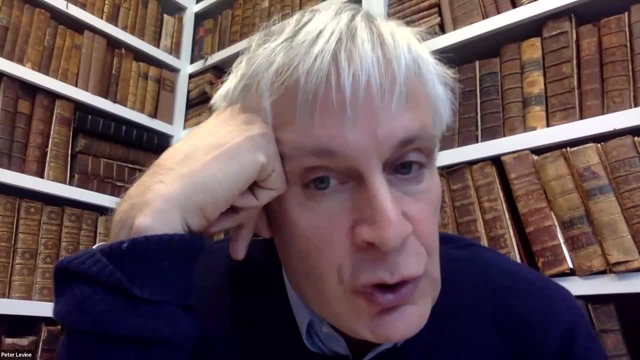 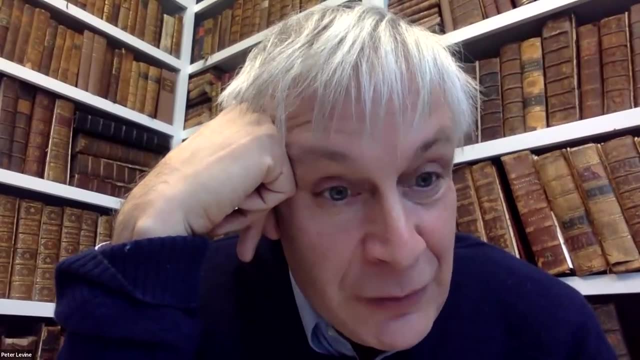 and participation, and it wasn't, and the engagement was unequal. So we were trying to drive up engagement, Um, and then those days, the books were things like the end of history, right, The Francis Fukuyama books suggesting that it's over. We don't have the, the, the, the regime is totally. 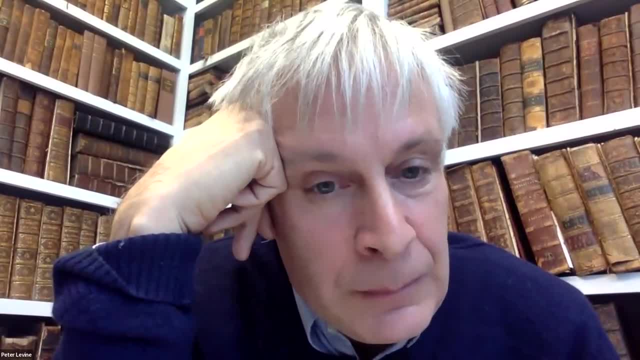 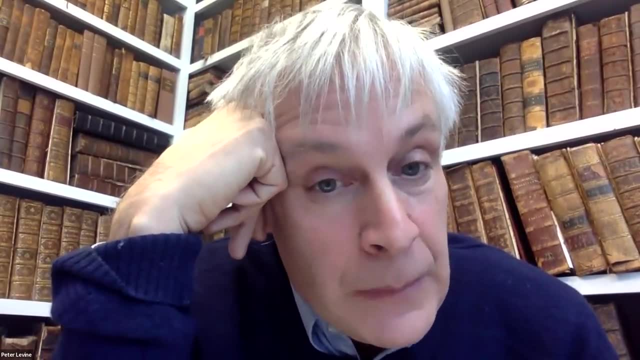 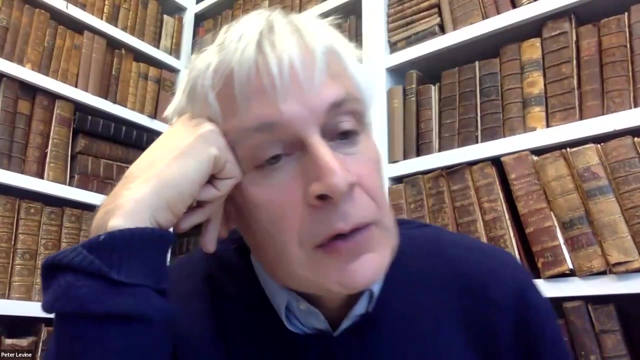 stable globally. And now I think you know the some of the participation looks- and it depends on your partisanship, but some of the participation looks downright bad. Um and uh, the, the, the institutions look uh, very unstable, And so that it's hard for me to avoid a crisis language when 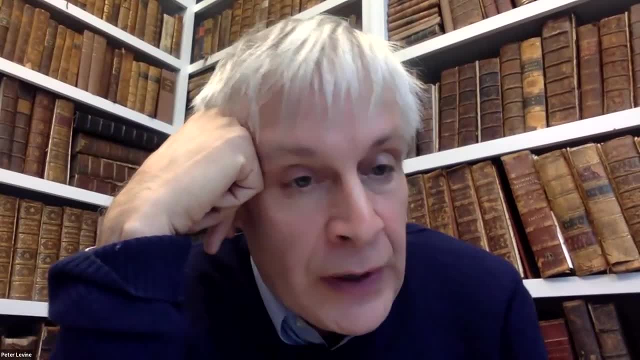 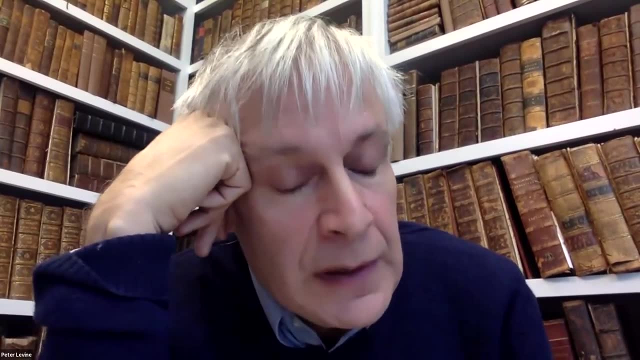 I'm talking about the institutions, uh, that the K-12 schools. I would more think of it as um in this, just speaking for myself. I would more think of it as K-12 schools have got to be part of solving the crisis. That's more on the side of the institutions. Thank you, Peter. I will note. 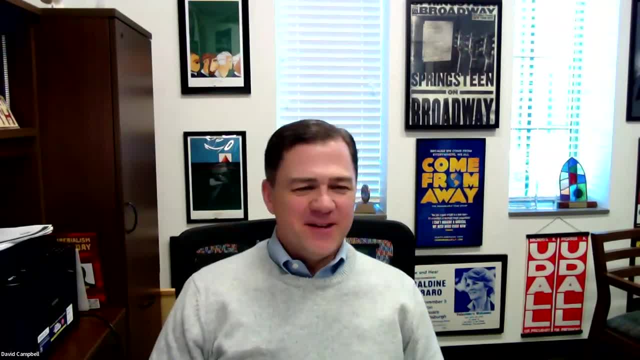 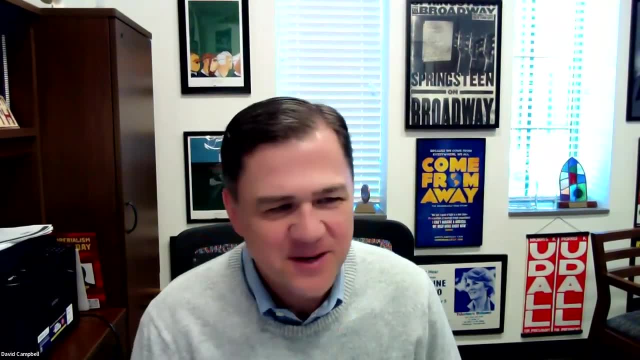 I just can't help but interject on this Um, on this issue of whether we should still care about participation. uh, we get pretty excited in the United States when presidential election turnout is 65%, So just think about that, That's. 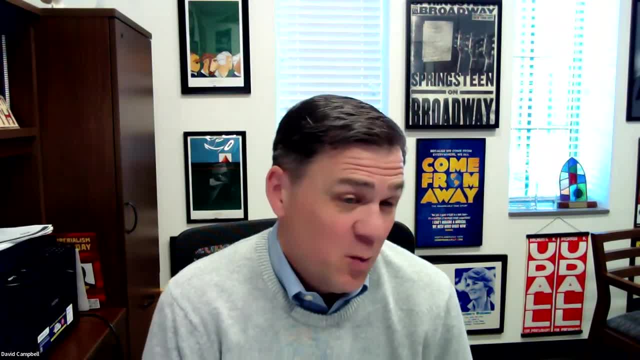 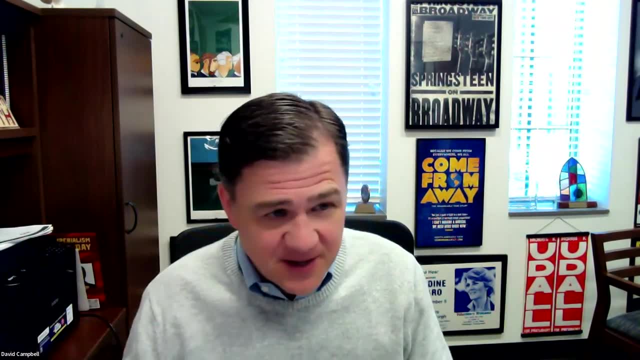 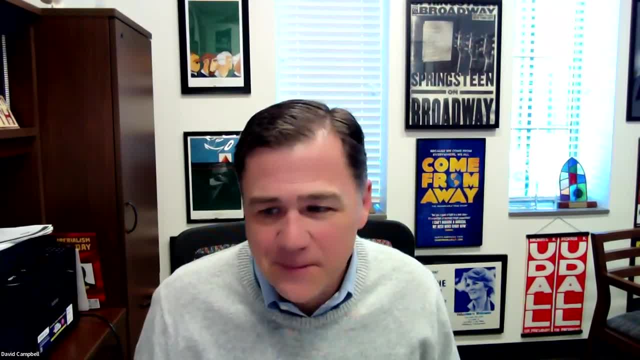 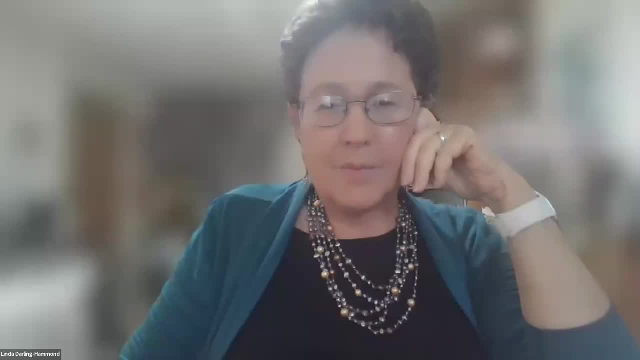 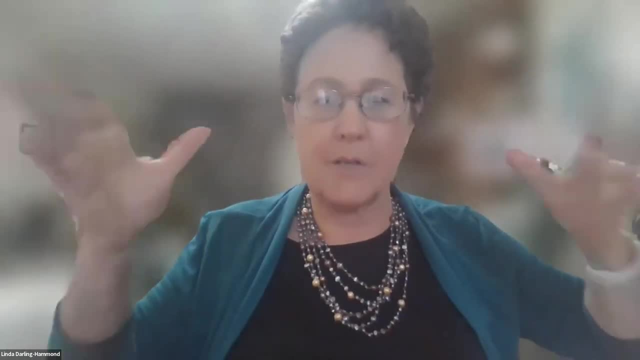 either other elections or other ways of getting involved. Any other thoughts on just what the crisis is? Well, yeah, I think that there's the question of what are we doing? We think of our public education system as the way in which we build a democratic sensibility, the reflective. 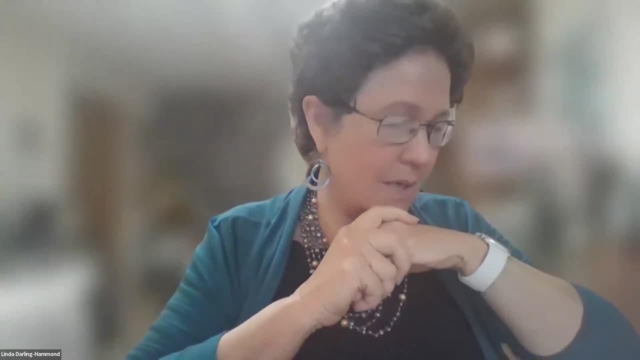 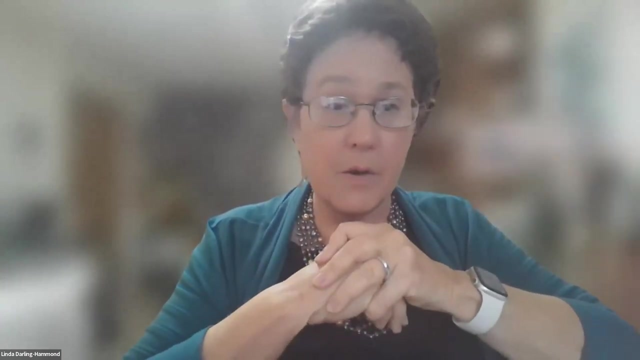 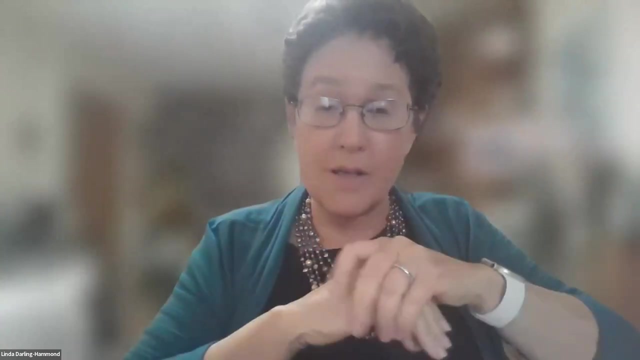 patriotism and all of the other virtues that Paul talked about. But we are in a moment where you mentioned participation. We have active voter suppression going on in many, many states, People to be taken off the rolls and you know all kinds of things going on. that way The rule of law is in. 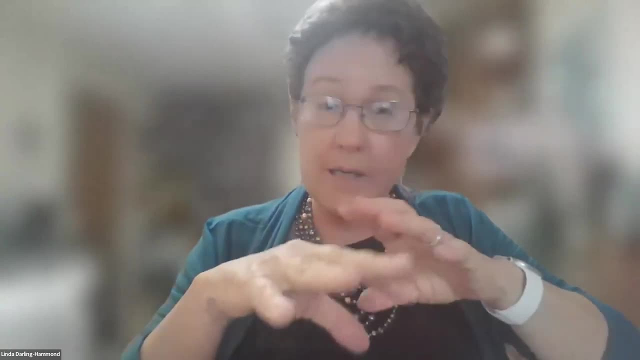 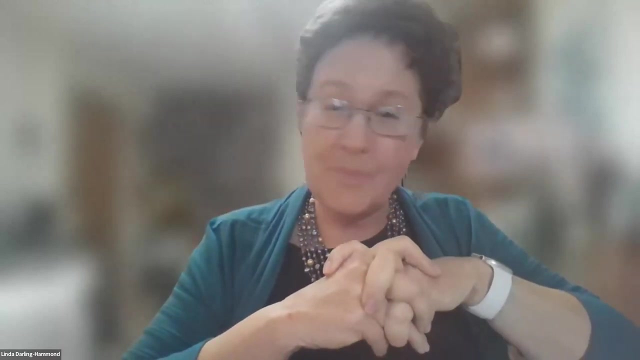 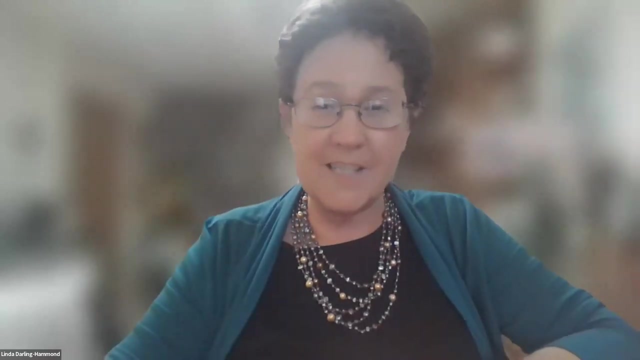 question The institutions are. you know, democratic institutions are being questioned and avoided even by, you know, people who are supposed to be part of the governance structure. The Congress is dysfunctional. Do we lay all of that at the heels of K-12 education? I think there are. 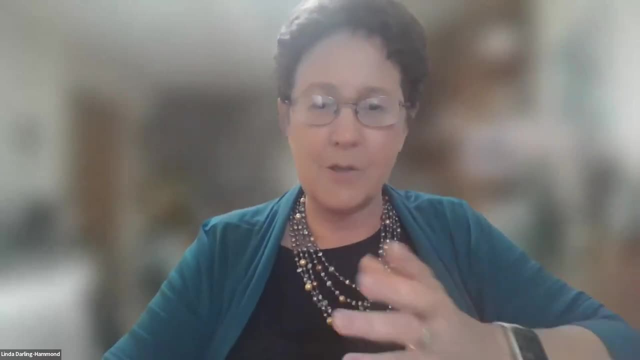 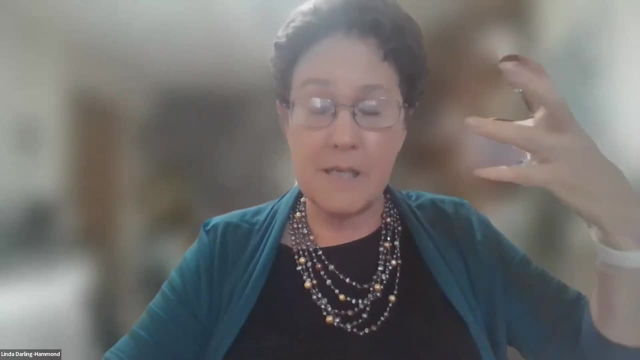 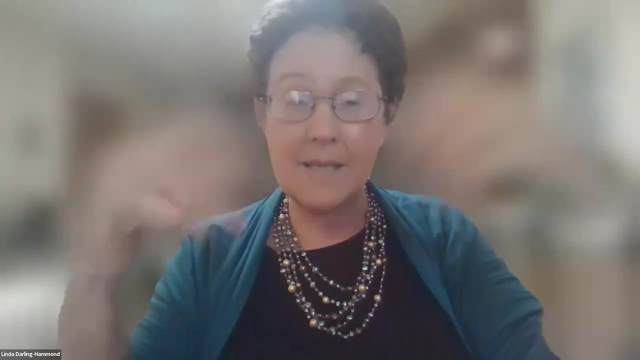 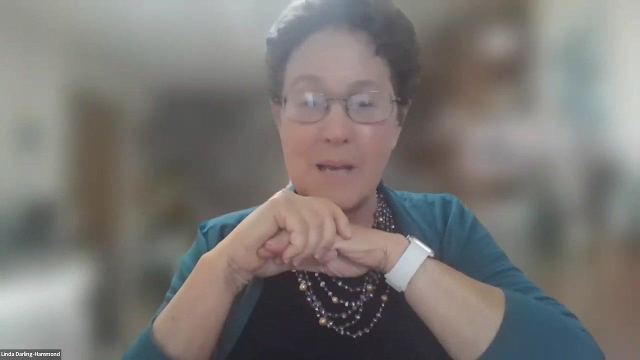 can contribute to the democratic understandings that could allow people to, you know, grow up and engage in less democratic threats than we are currently experiencing. But it's, you know, it's hard to imagine that it is because of what's been taught in school. I think it's because 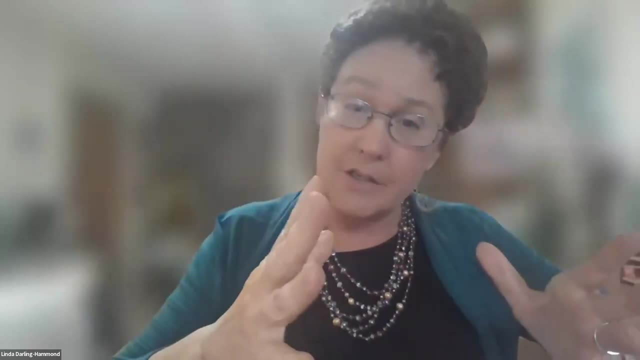 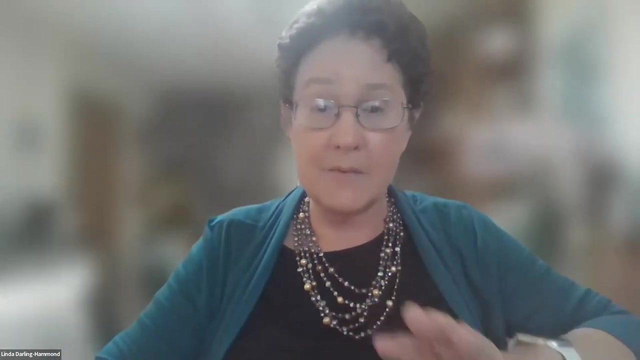 perhaps that you know we haven't developed the skills that we need to be able to do that. perhaps that you know we haven't developed the skills that we need to be able to do that. But there has been less attention perhaps to developing the sensibilities that are not only about 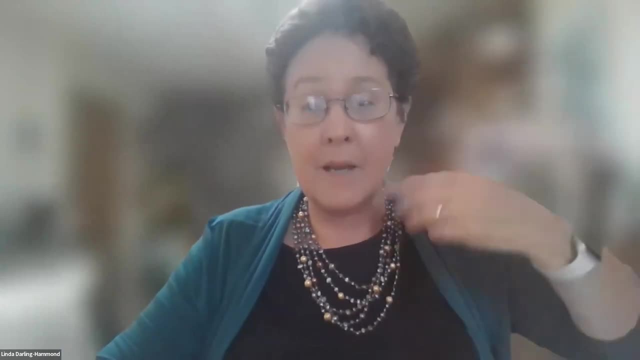 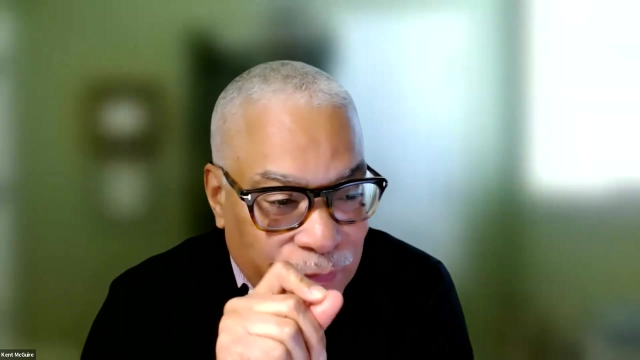 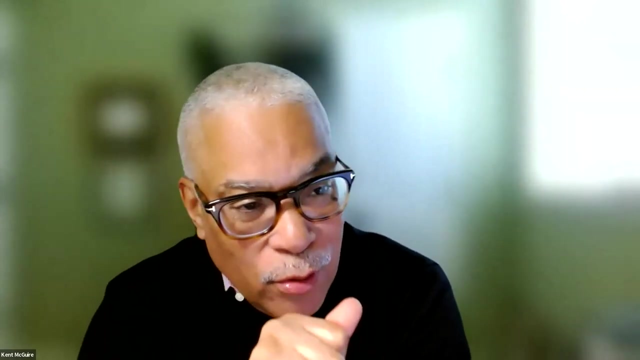 civic participation, but about civic reasoning, about being seeing oneself as part of the community. And you know the David, the market for bad news is much healthier than the market for good news. I just want to get that on the table. 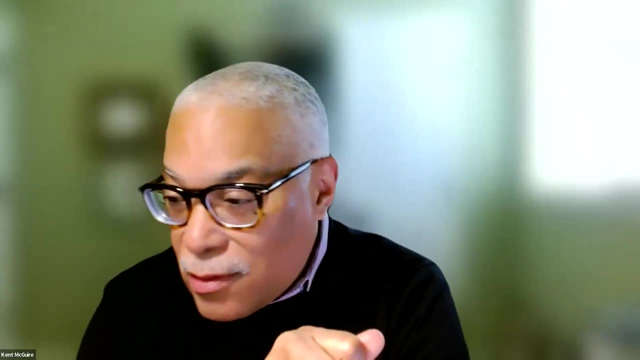 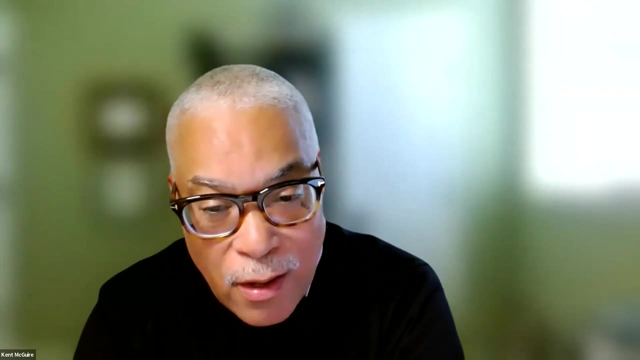 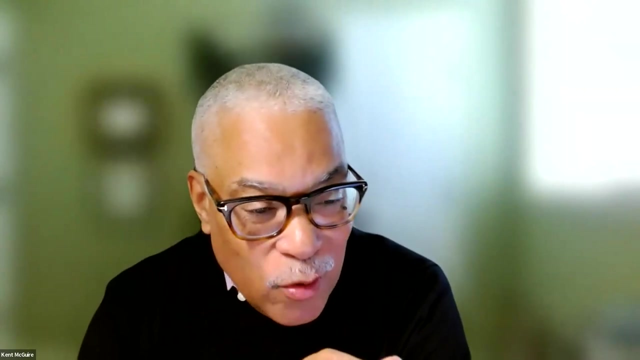 And note that, to sort of underscore Peter's point about, it's not as bad as it looks. you know we don't do as good a job of talking about. you know the good things that are going on or, more importantly, for instance, what parents and voters are for or what they want more of. And 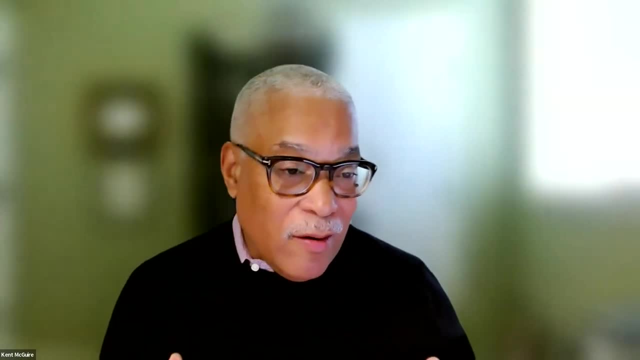 if we don't do as good a job of talking about you know, the good things that are going on or, more importantly, for instance, what parents and voters are for or what they want more of. And if more of that sort of got on the table, we might almost get to a glass half full point of view about you. 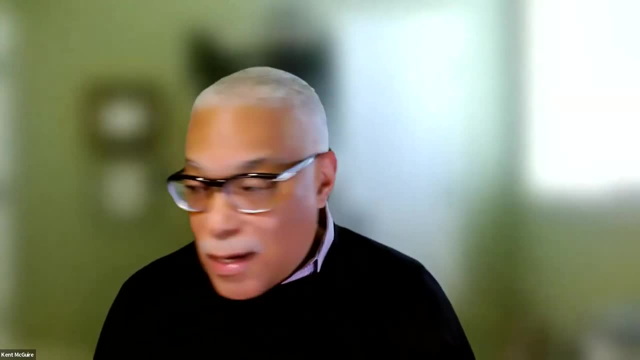 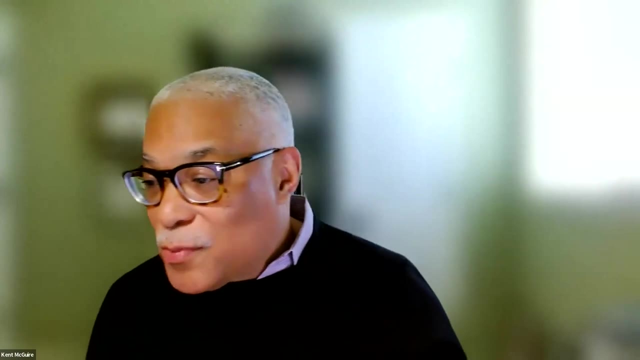 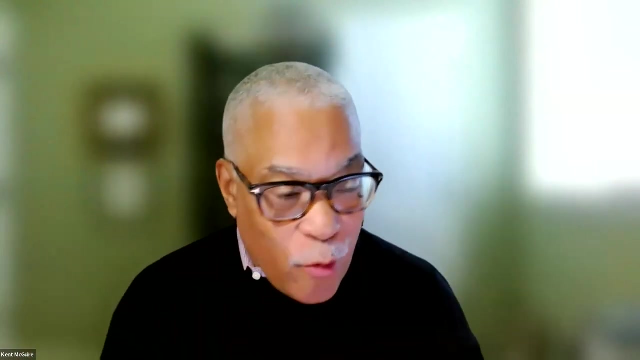 know what's what's possible here. But you know I'm looking at polling data that suggests that teaching critical skills such as problem solving and communication and teamwork and sort of getting along, you know over three quarters of parents and voters actually want that. 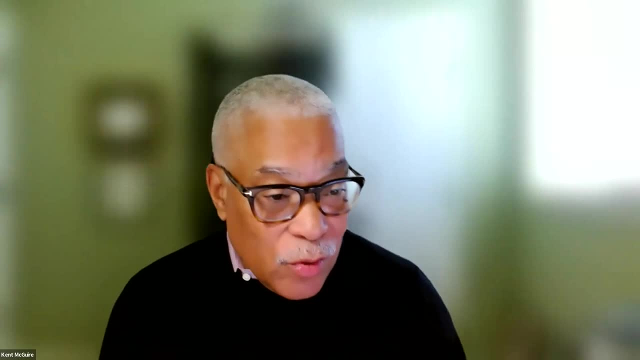 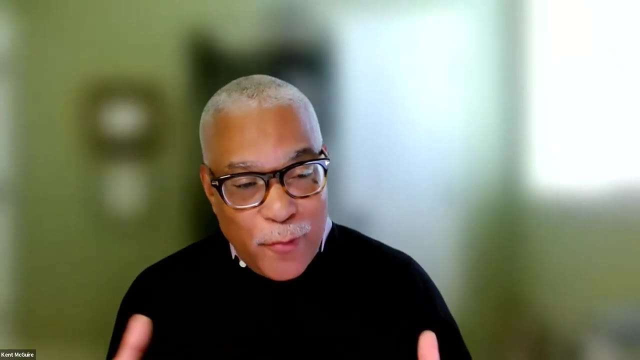 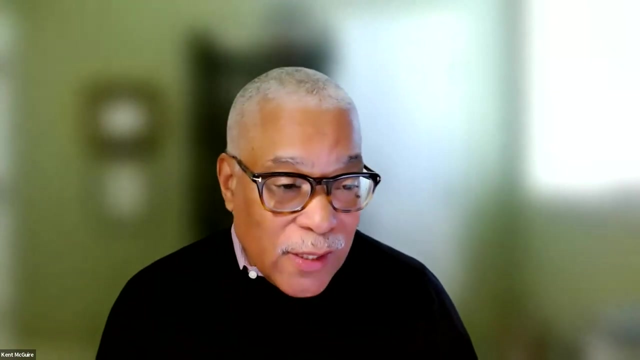 They also want an accurate history taught in the schools. So I think if we could, we could sort of zero in on the thing that a very large, if silent, majority claim to want. we might see that there's less of a crisis and more of an opportunity if we could decide. 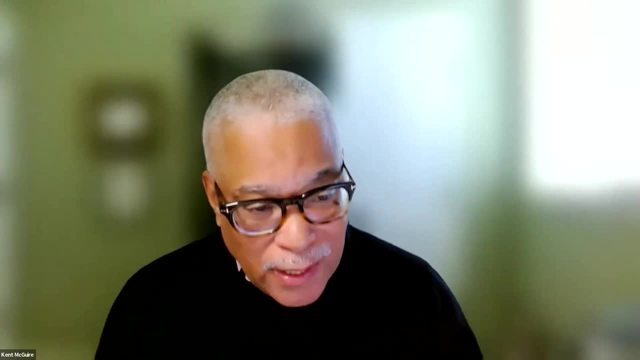 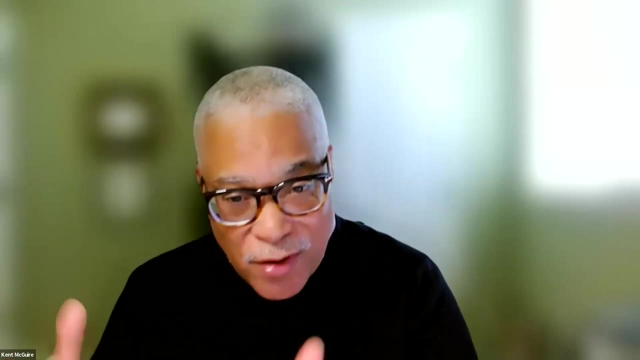 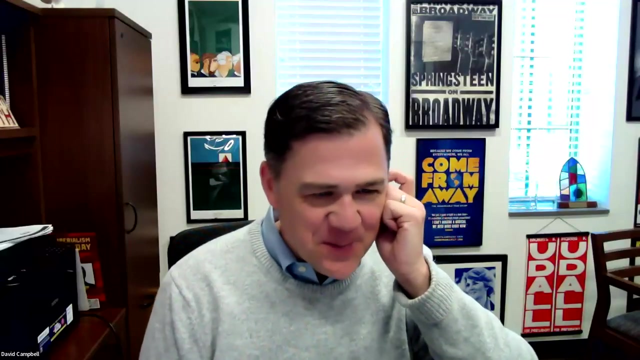 how to leverage public opinion, you know, to advance policies and actions that gonna move us forward. Yeah, thank you. On the glass half empty, glass half full issue, I'll just make my little editorial comment that people who complain about the kids these days, in my experience don't spend. 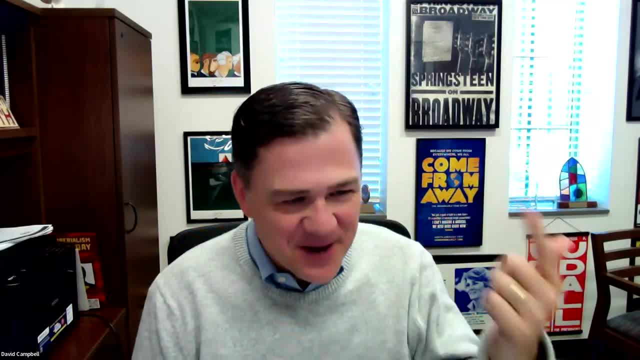 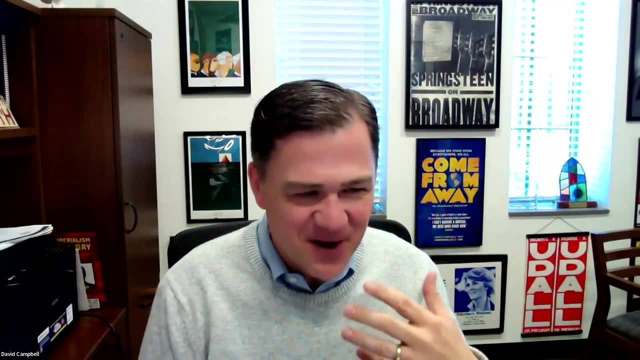 a lot of time with the kids these days that in my interactions with young people I actually do not come away discouraged, I actually come away discouraged, I actually come away discouraged, I actually come away quite encouraged that often they are very good at doing exactly the sorts of 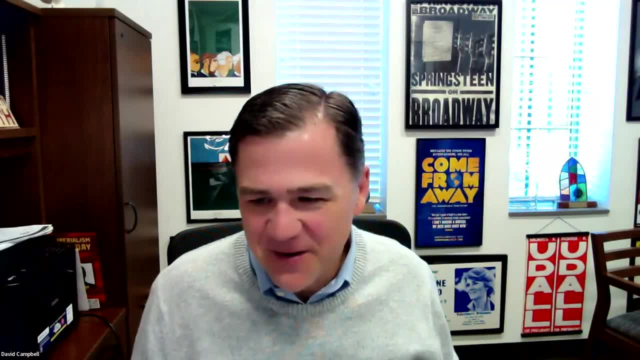 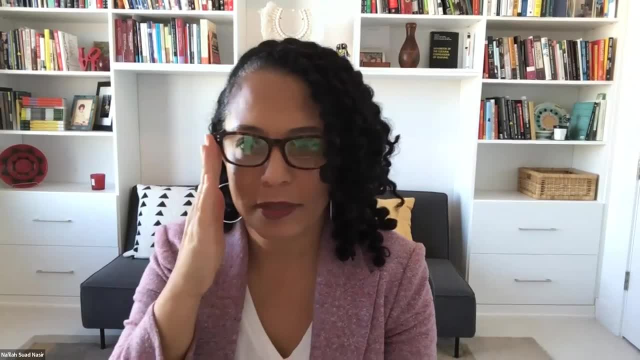 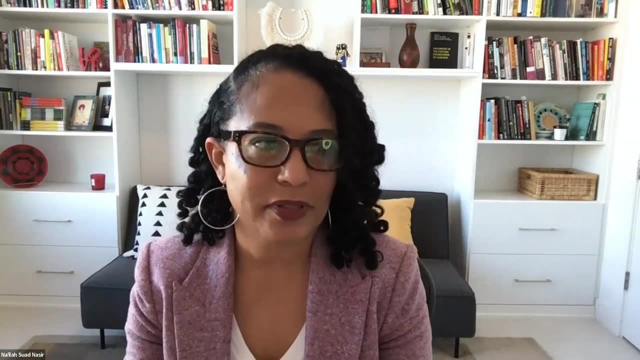 things that we're talking about, including disagreeing with one another. I want to make sure we don't end without acknowledging one other element of the crisis, I think is the crisis that teachers are facing in figuring out how to manage these issues in such a complex and contested. 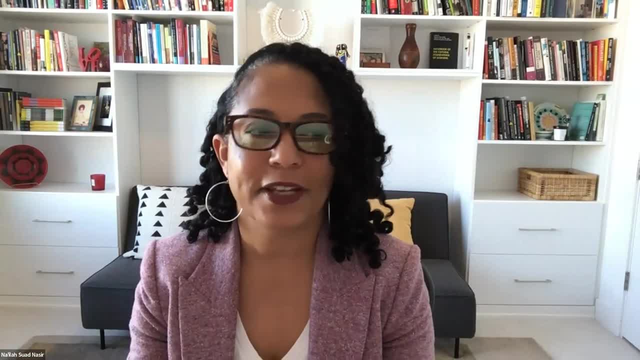 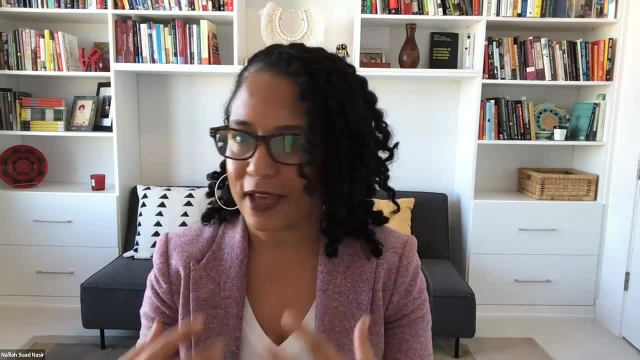 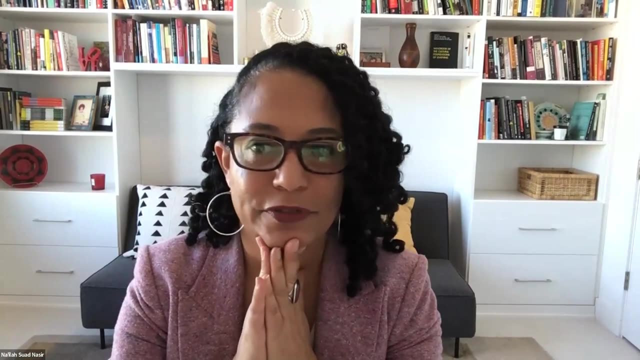 political terrain. So I feel an obligation to give voice to that sense of of crisis and terror and fear and anger, and you know all of the the ways these the current political moment is playing out for teachers who are trying to figure out what to do that's best for kids and 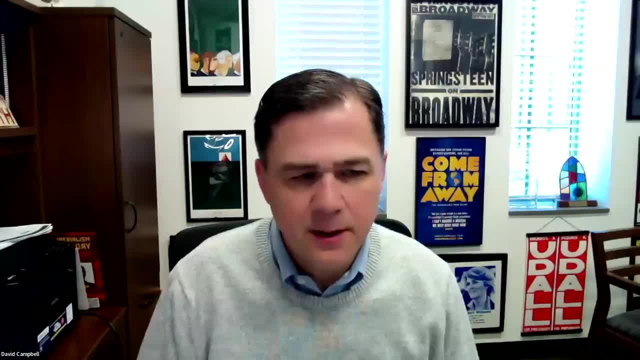 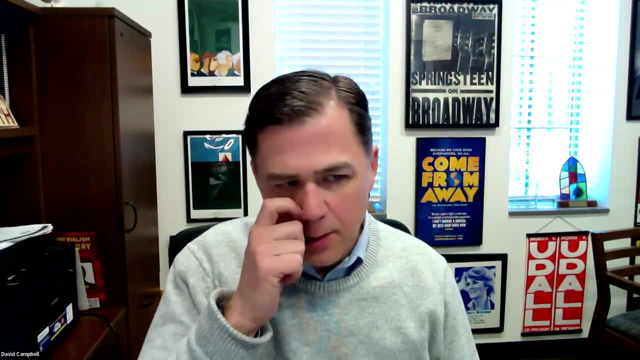 what to do. that doesn't doesn't get them fired, So just yes, thank you Again. lots of questions we'll get to as many as you possibly can, But one that came up early on that I do think is worth noting. this conversation has focused on 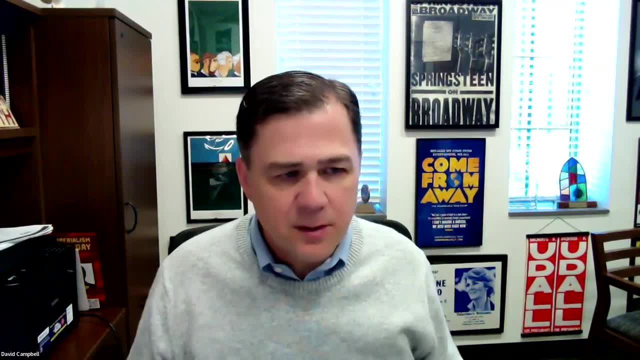 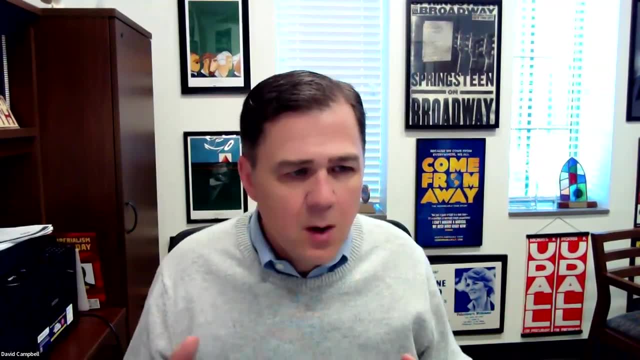 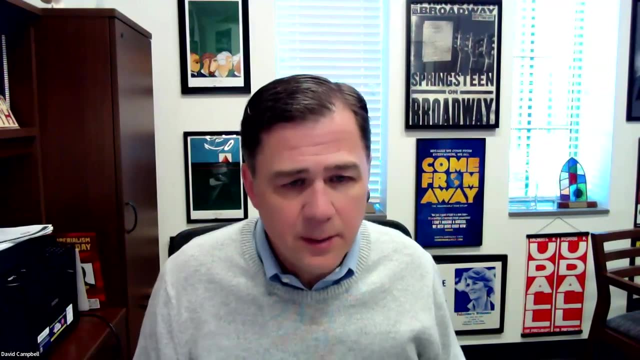 the United States appropriately, but it is worth acknowledging that civic education spans beyond the United States, And so I thought I might ask the panelists to reflect a little bit on what themes from our conversation might apply more broadly, and not only to an American context. 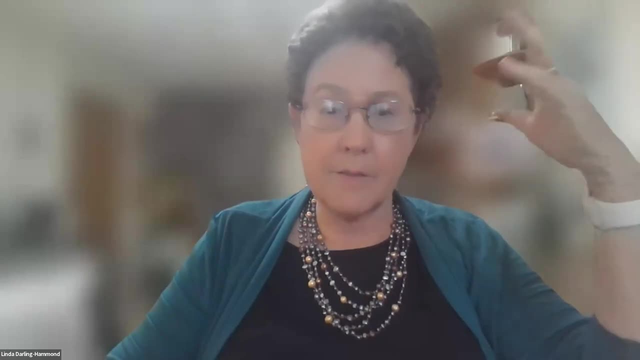 Well, clearly, there's been a lot of discourse about the rise of authoritarianism and fascism around the world, And so, in these times of great uncertainty- and we you know the human rights movement and the human rights movement in general- I feel that it's a good place to 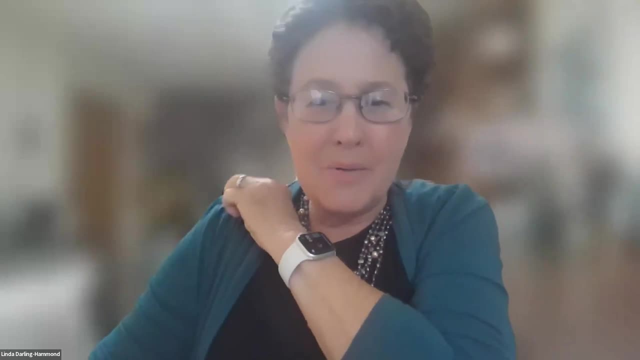 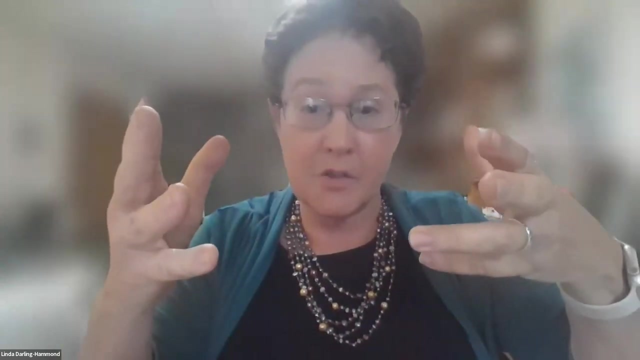 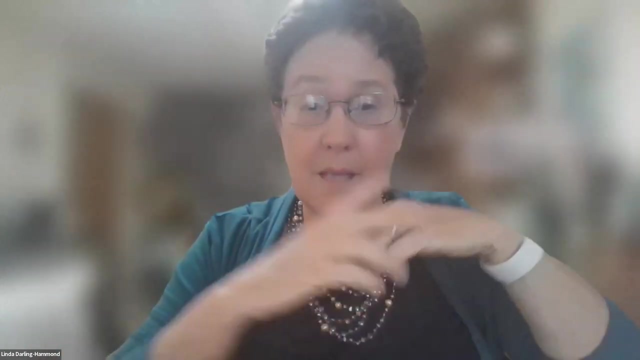 race is hurtling towards an unknown future here, which is creating a variety of other crises which I think may feed into this crisis. you know climate crises and political crises and famine, And you know there's all conflicts of various kinds And I think that may feed. 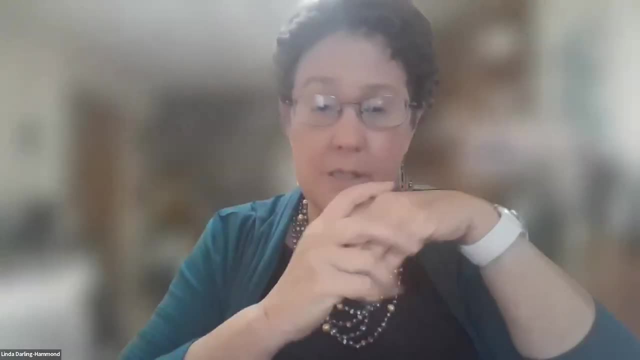 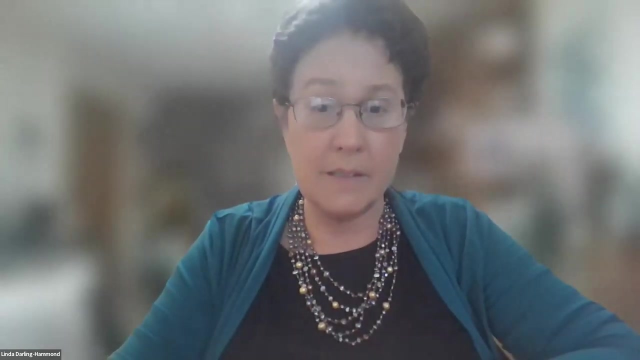 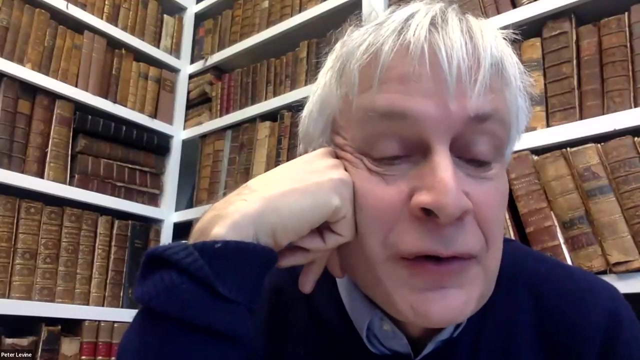 the tendency in many you know regimes to towards authoritarianism and away from democracy. So I certainly think that we're not alone in this moment in the world. I feel like I'm just playing the grizzled veteran of civics today. That's my role, So I again. 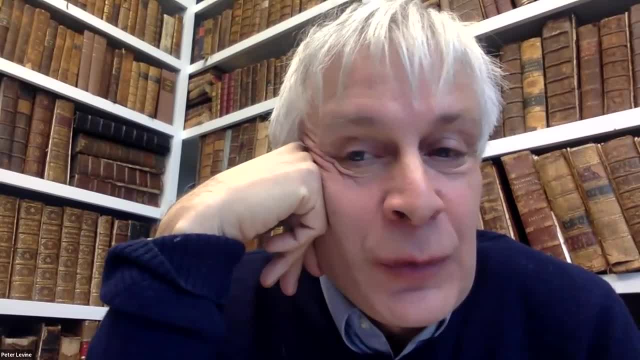 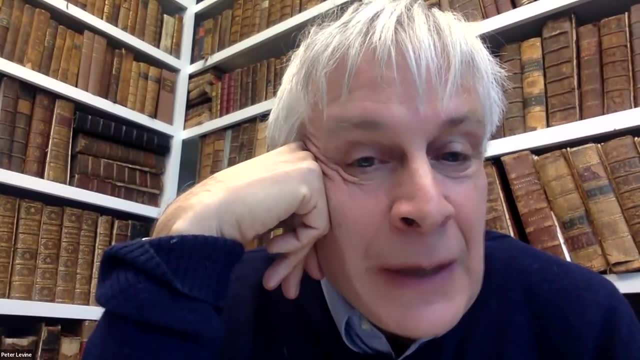 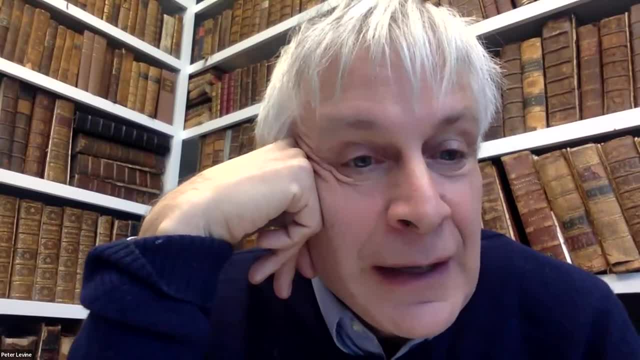 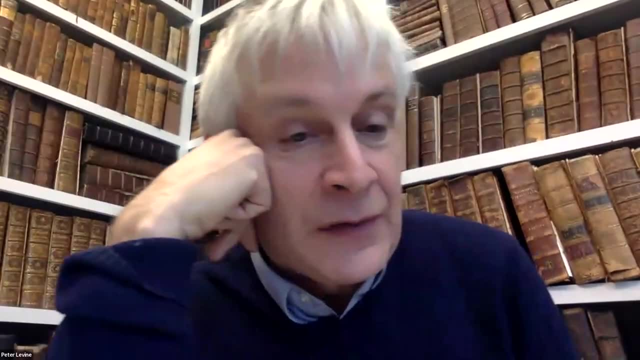 the era of telling people that you should do civics like we do in American schools is kind of over. And what's? what's more, much more interesting is figuring out what's being invented. I mean just as two quick examples. I know about Ukrainian colleagues who were doing 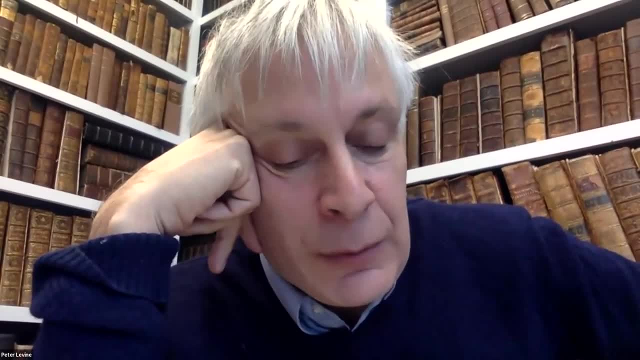 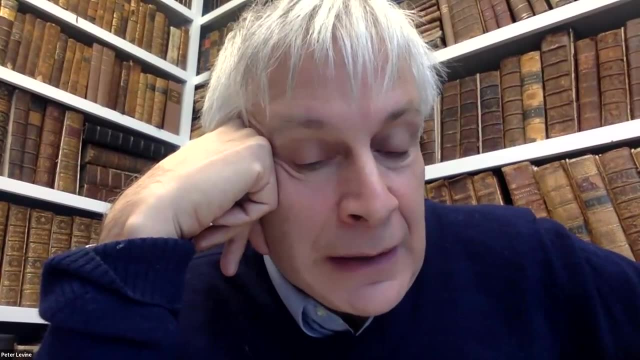 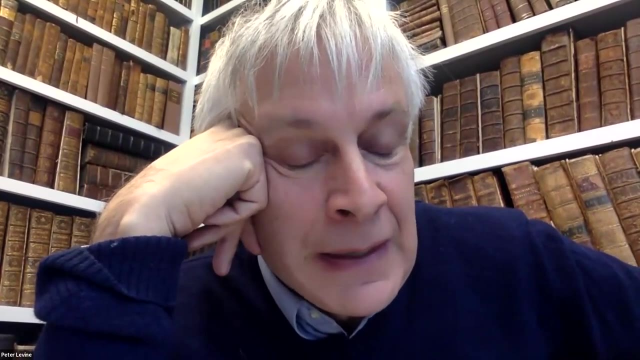 really interesting research around. I mean not research- so they were doing really good curricula around combating Russian generated online propaganda before we got focused on that And I would- I would- recommend learning from that. And then, just another example is participatory budgeting for 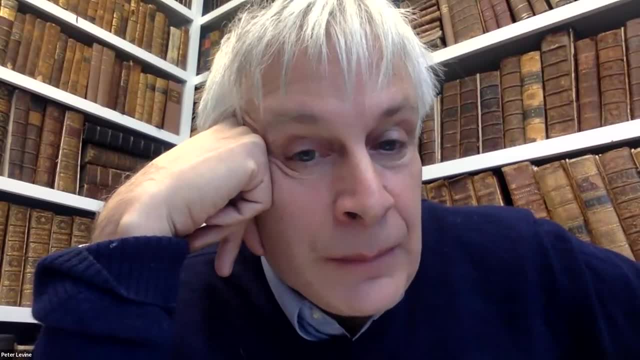 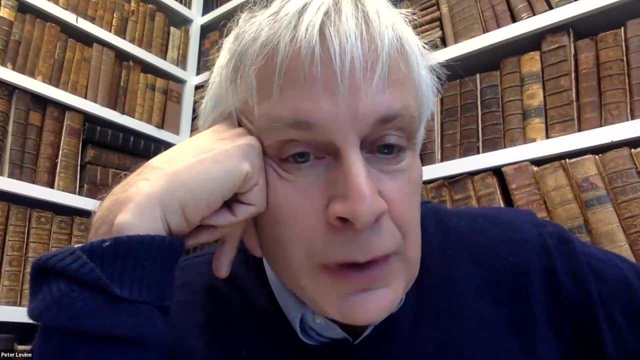 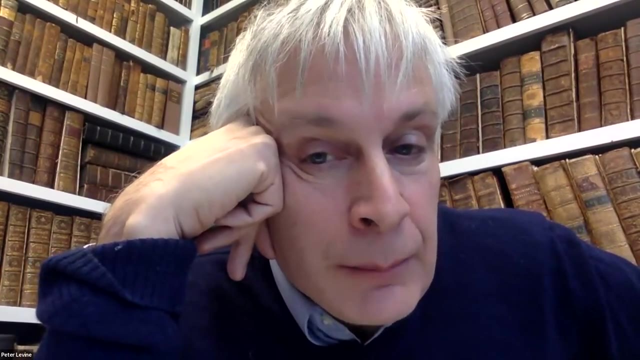 young people is quite common now as a as a experience where your young people are involved in actually allocating funds. I think I think some of that in your, your community, Paul in in in Phoenix, But that comes from Brazil, That's a Brazilian import, So I think we need to be in a 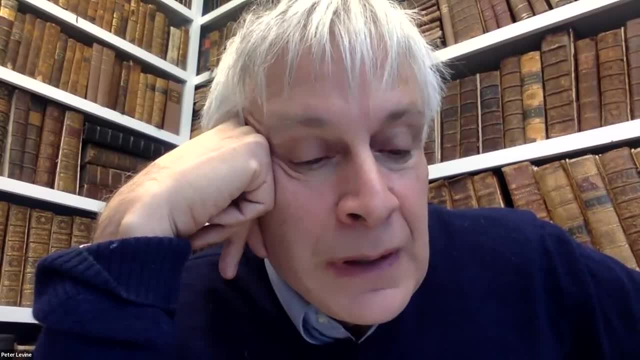 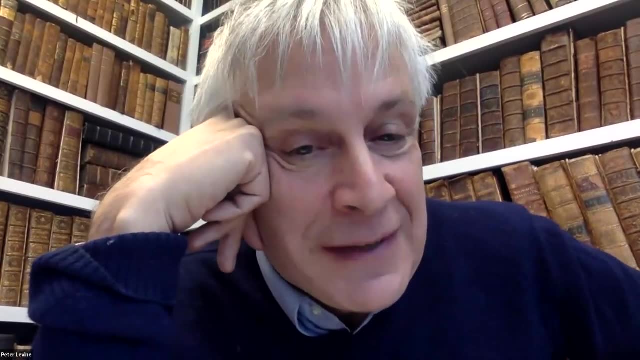 period where we're looking for, where, where a lot of the challenges are- whether it's propaganda or authoritarianism or or polarization are are widely shared, not universal- They no polarization in Denmark, but they sure have it in, you know, a bunch of countries- and- and where we can actually 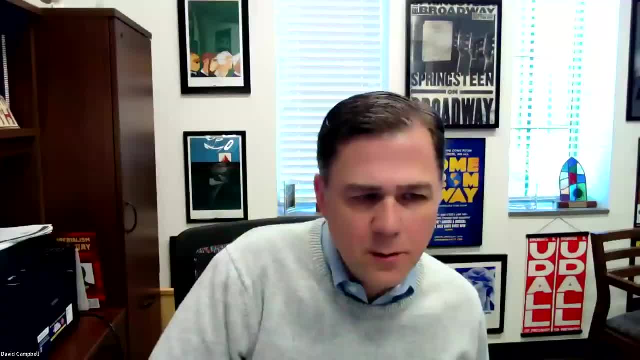 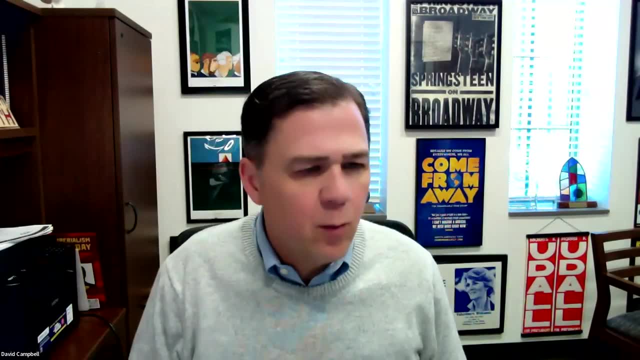 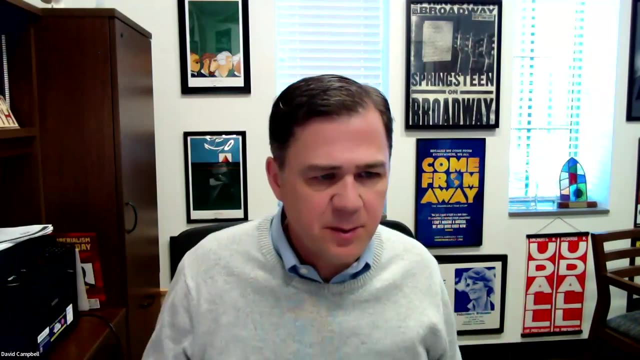 learn from from good practices in other countries. Thank you, Obviously, a lot more we could say about the global reach of civic education, but let's move on and talk about a theme that, while we discuss it a lot in the US, does apply elsewhere, And that is polarization. We've had lots of questions. 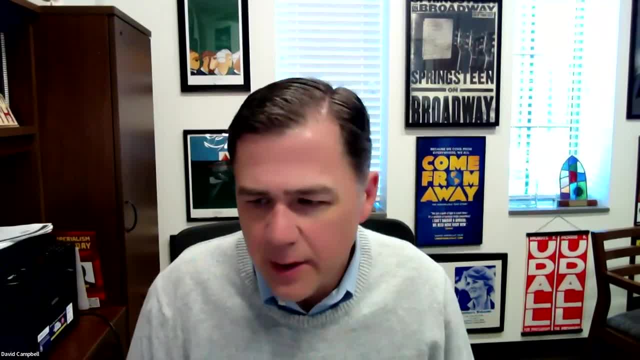 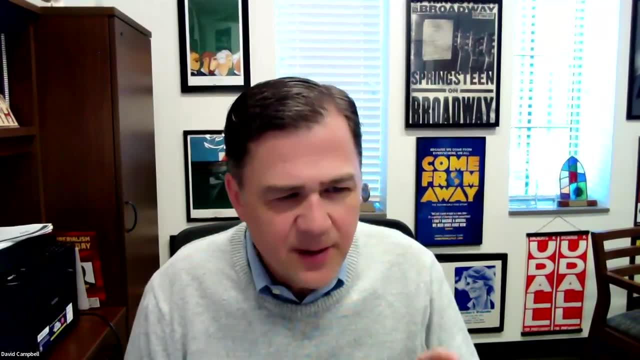 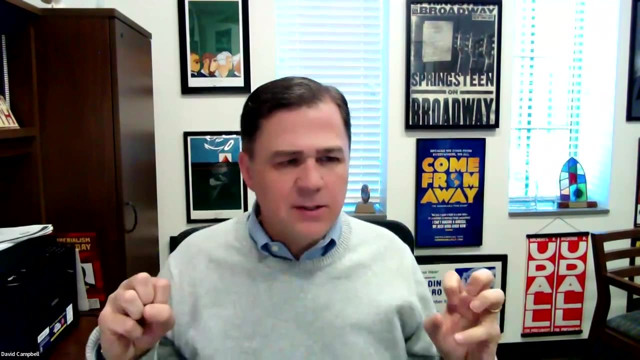 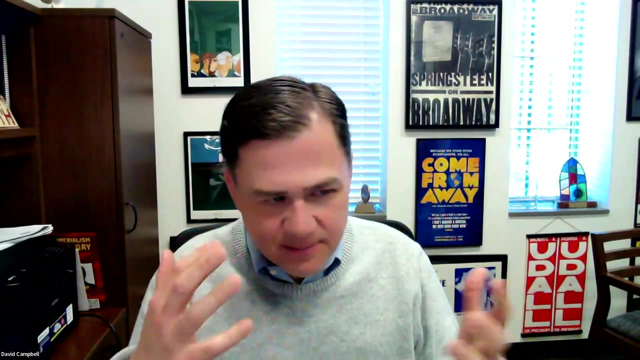 about polarization, but let me just maybe give a capsule summary. We have a lot of research that shows when people are faced with ideological opposition, rather than move to the middle or reason with their opponent, they often just double down on their own views. So one challenge of having discussions in a 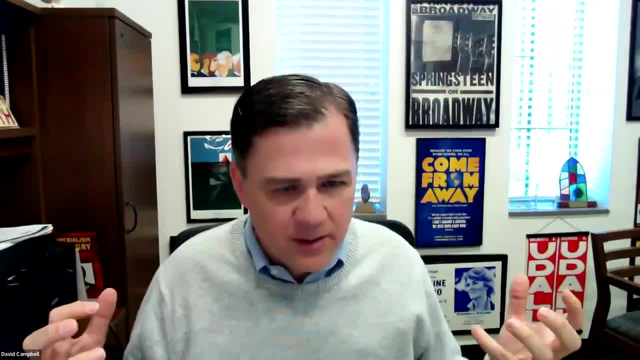 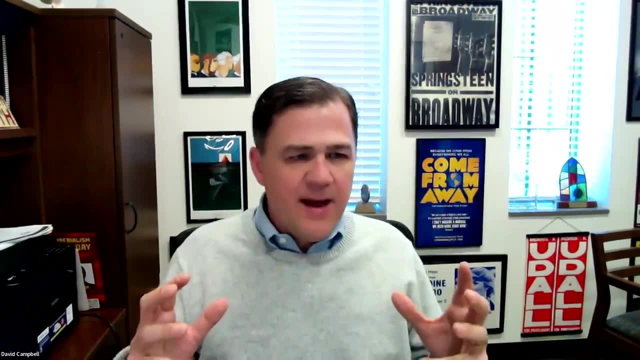 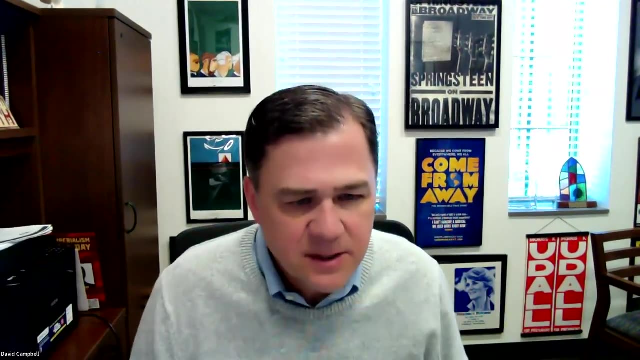 classroom setting is, you could actually exacerbate polarization rather than minimize it. So the question is what kind of classroom practices can counter that hunkering down, pulling apart tendency, so that if we do have these conversations in classrooms it really does serve the purpose of teaching the 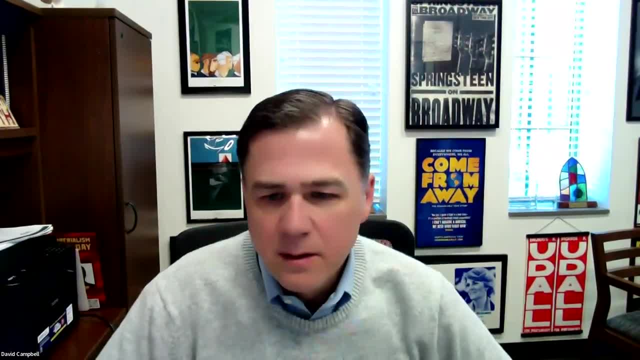 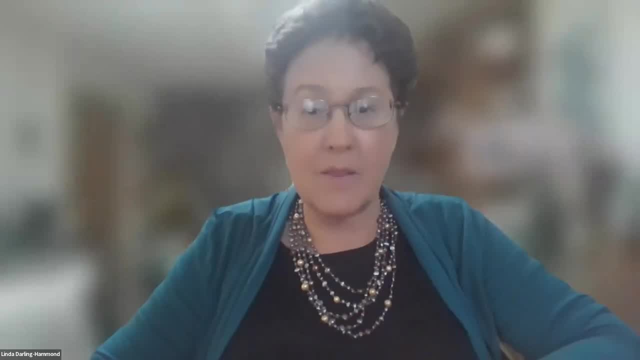 sort of civic friendship. that has been already mentioned. You know, we've been talking about the pedagogies that teachers might need to learn, And one of them is this way of developing disciplined understanding and listening, And I think that's a really good question. I think it's a really good. 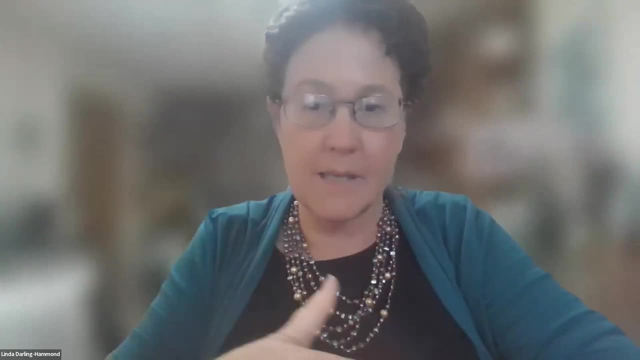 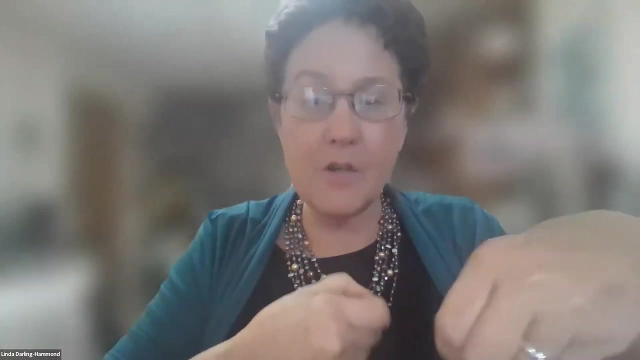 question in some ways. Thank you, I think this question definitely is true, And so I've been learning and I've been listening and thinking and so on. So seminars are one of the ways that, one of the tools that teachers can use. There are lots of other. 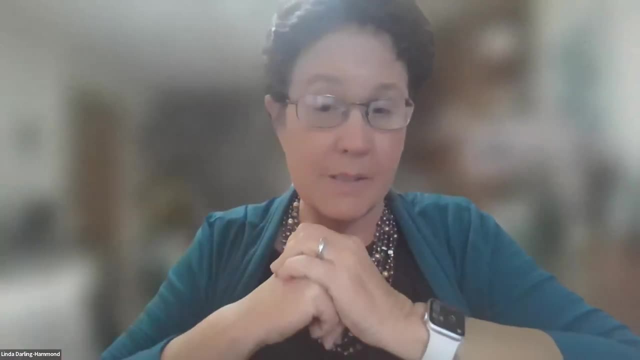 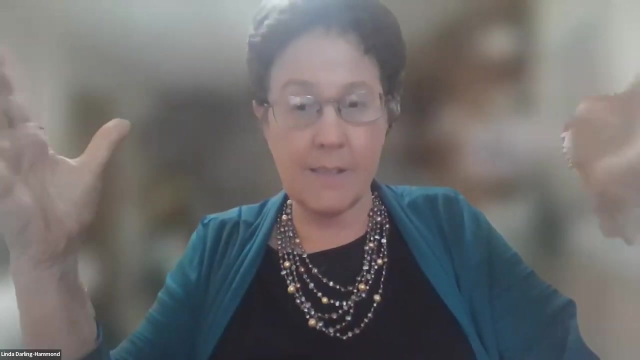 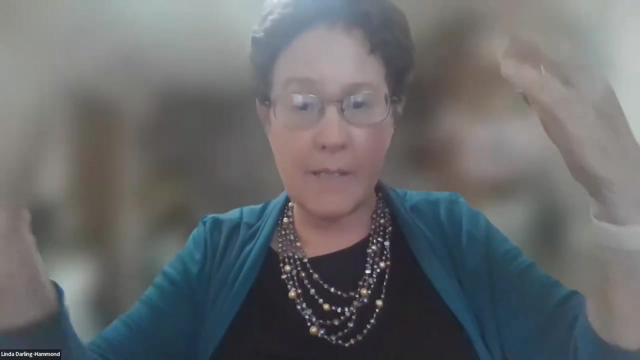 ways by which students can learn to have to at least listen and take into account and perhaps pursue further evidence about the- you know- places where there can be disagreements. I gave the example of the assessment in Washington State, principles that are intention and then reason through and acknowledge. you know the other point. 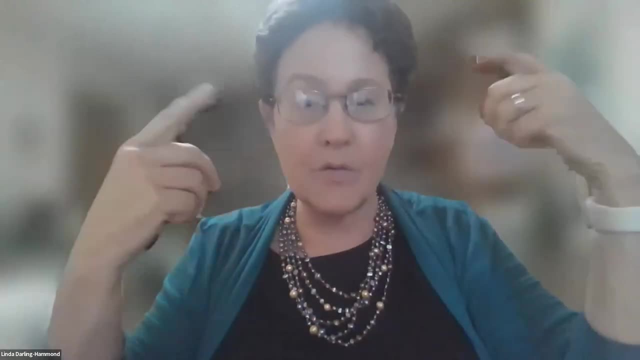 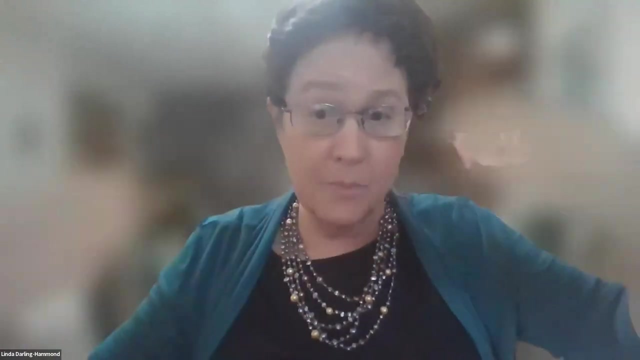 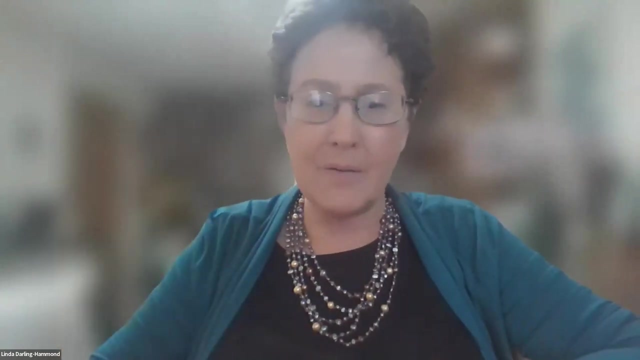 of view as they come to their own judgment. that mode of thinking, that way of analyzing and evaluating and thinking through and having to respond and then doing that in the classroom, can be taught and it has to be part of the you know kind of warp and woof of the, of the way in. 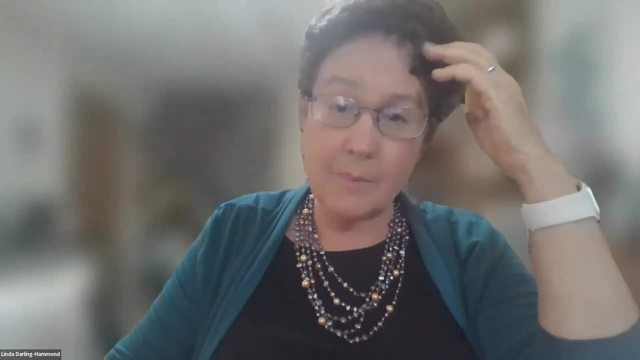 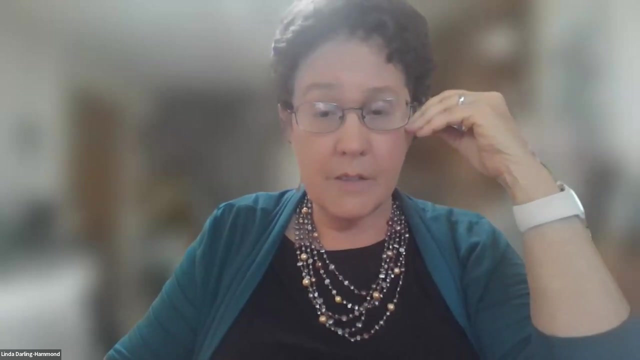 which we're teaching and learning, and one of the things that we haven't mentioned- but I think it has been a challenge- is that, you know, early in the 2000s the No Child Left Behind Act called for annual testing with high stakes attached to it, and many states beyond the reading and math tests. 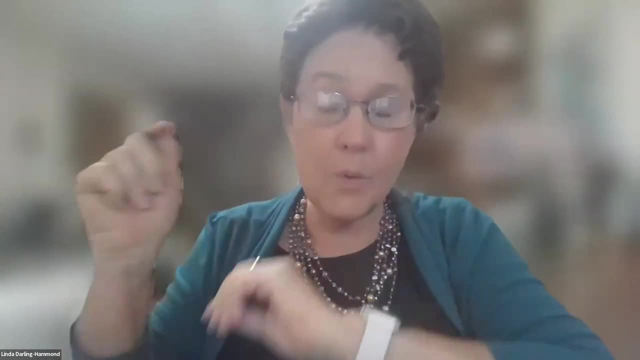 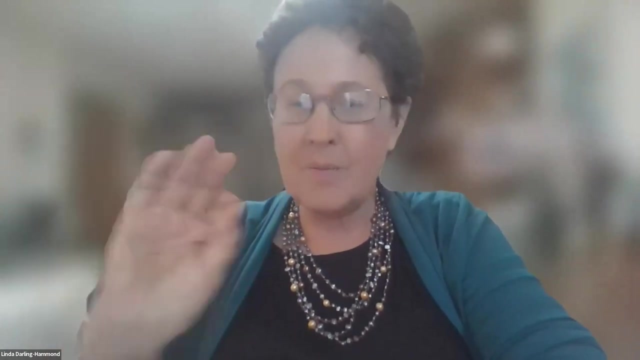 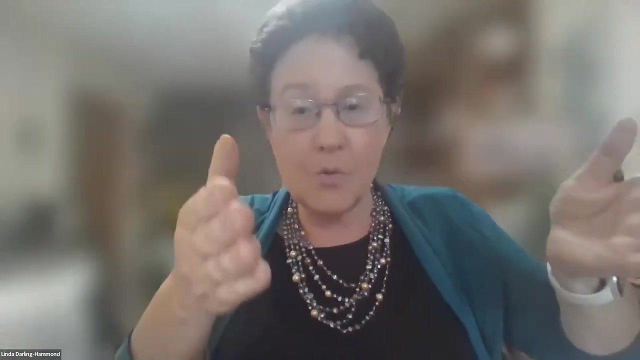 required were also then testing in other subject areas in ways that, in the United States, are almost entirely multiple choice, whereas in other countries you know the, the reasoned essay, the, the, the, the, the and discourse is actually part of the assessment system as well, so schools really felt like they. 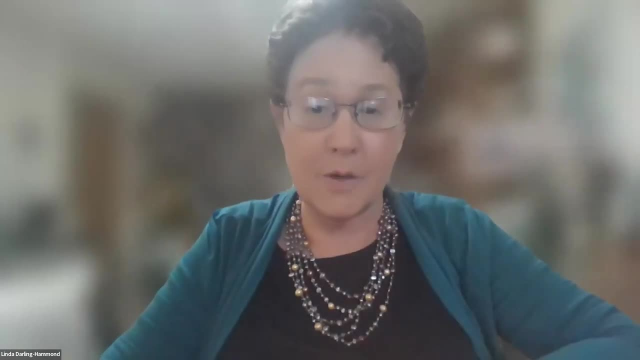 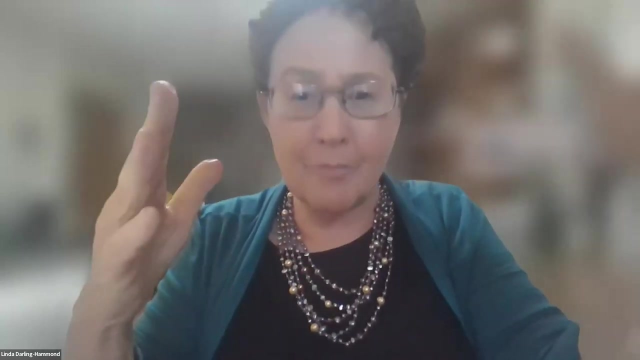 had to get the facts in in a way that kids can find the one right answer out of five, and that and a right answer way of thinking, which is very different mode of thinking. it's not that you can't have both, but you have to make room for a mode of thinking in which you're weighing and balancing. 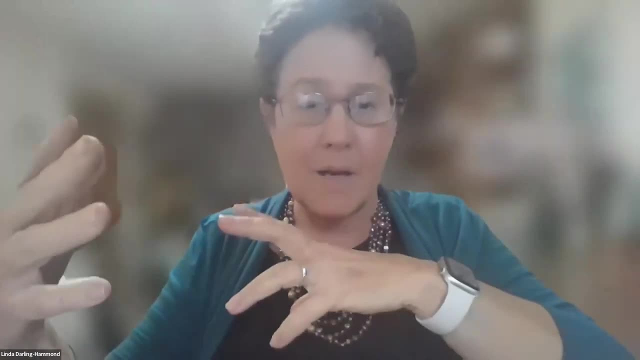 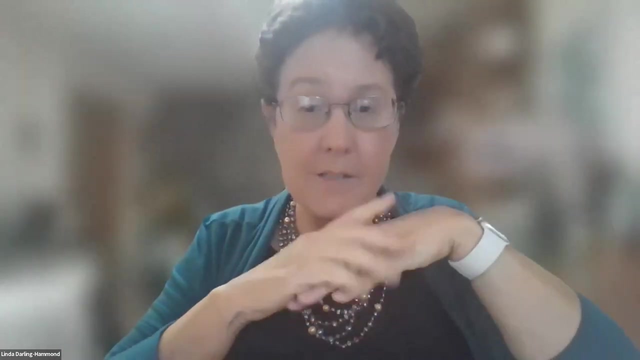 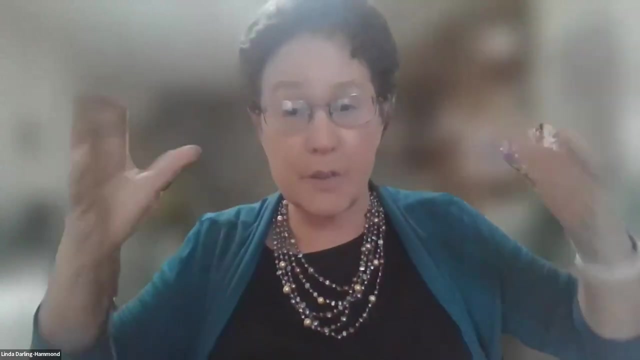 and you know, considering and evaluating and so on, and that really did. there's a lot of evidence that that mode of thinking is part of the assessment system as well. the thinking was deemphasized during that era of public policy, and so I think we have to think about how do you both build the curriculum systems and the assessment. 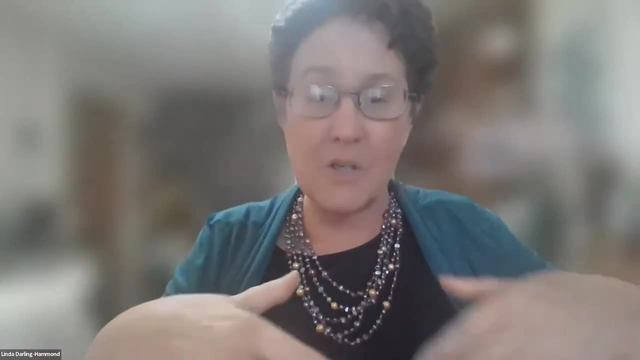 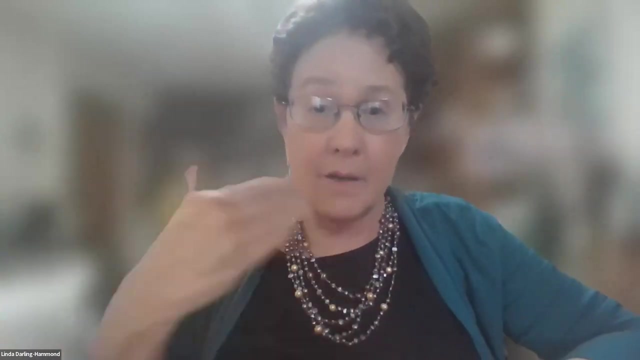 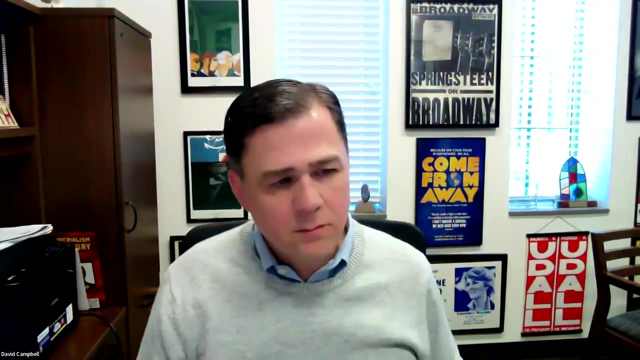 systems and the pedagogical systems in which the the mode of thinking and weighing and balancing, listening, thinking, evaluating evidence and considering alternative points of view is part of the work, and we're from a learning like. So I just you know- I think Linda just talked about the fact that, well, probably this is like being a student of the new government and you're just thinking that you're raising yourself and so on and so forth, and I think it's kinda interesting that you're really trying to focus on the topic of the work and the work that you're doing right now, that you've been working on for 10 years as well, and I think Buddha will have to give a good answer for that. 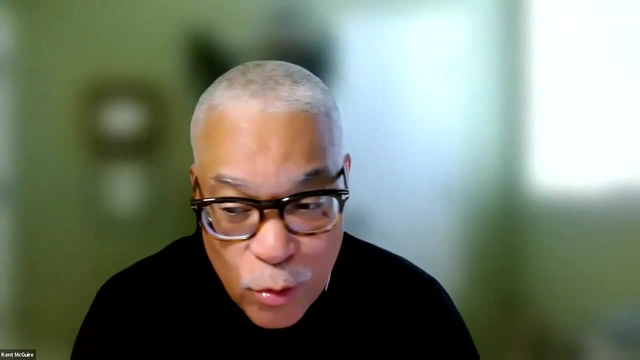 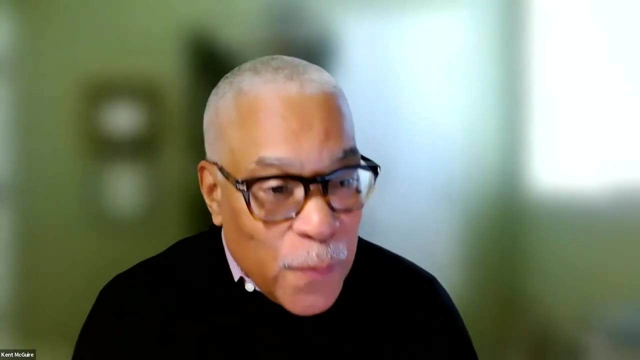 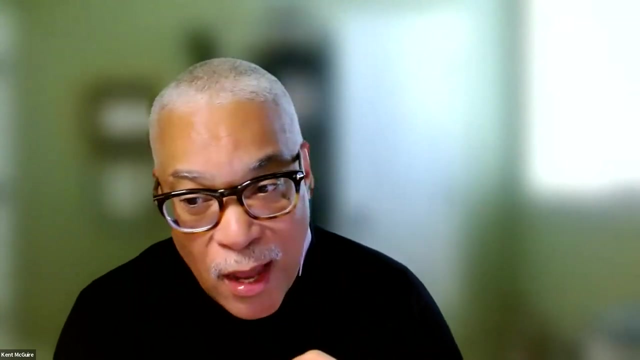 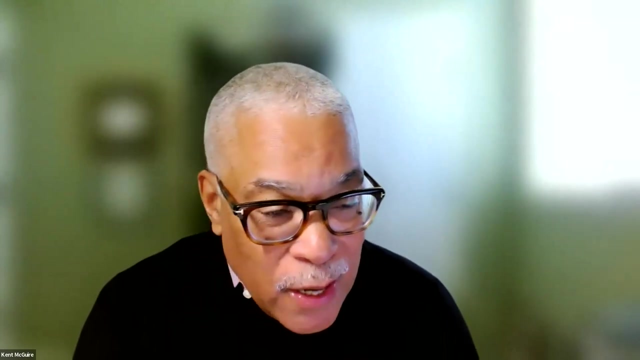 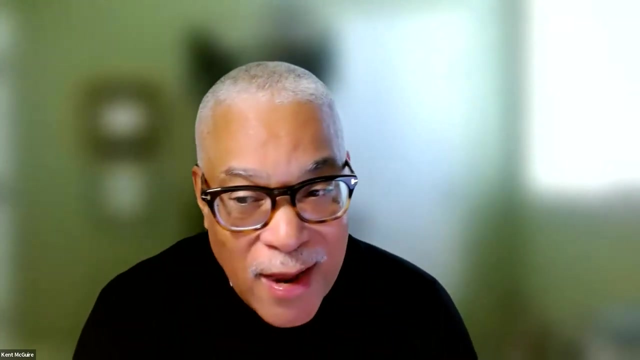 just describe the two or three rather obvious policy leaders that could be pulled more or less in concert to deal with. I just want to add a small point. It wouldn't hurt if we introduced a little more data into the system about what the kids actually want to do, And I think we'd be. 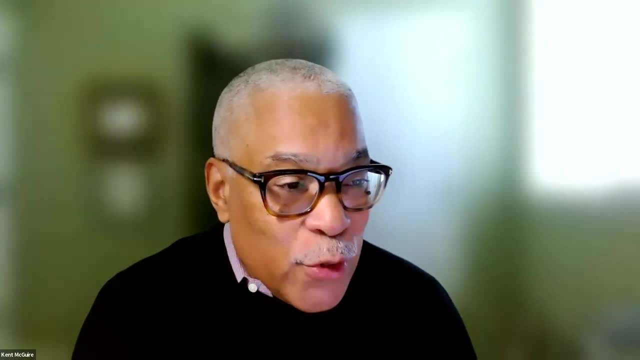 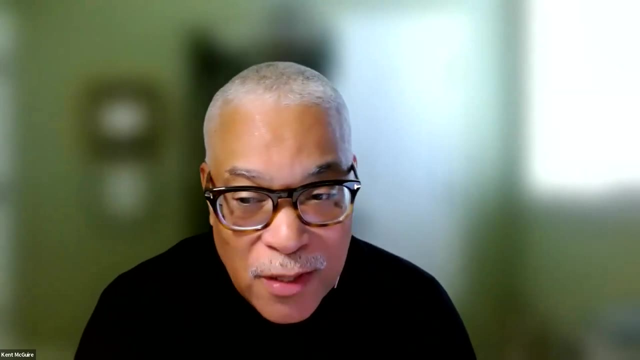 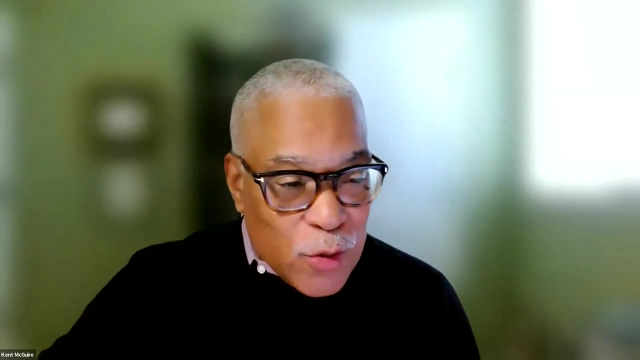 stunned- I think it was your point, David, about you're actually hopeful when you get in front of young people. I think you'd be stunned, the correspondence being the kinds of things kids actually want to work on and the kind of schools you'd need to organize. 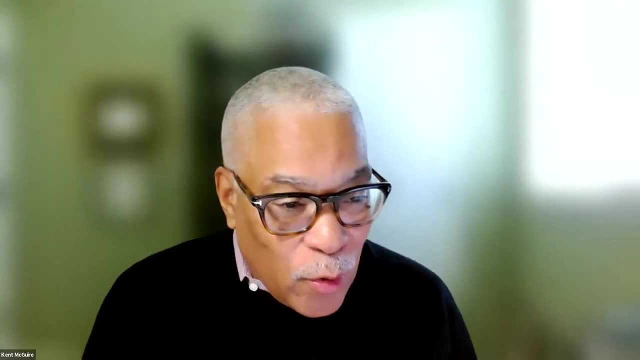 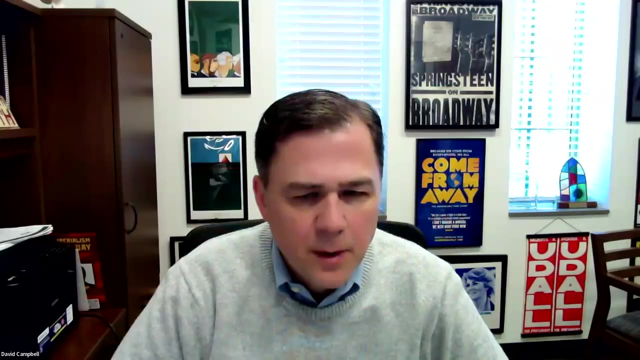 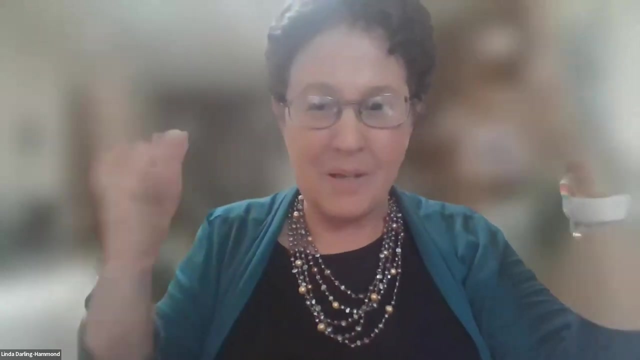 In pedagogical practices you would employ to kind of leverage. you know their own motivations and interests, Thank you. And, by the way, they love to discuss things and argue And you can teach them to argue productively and with attention to each other's. 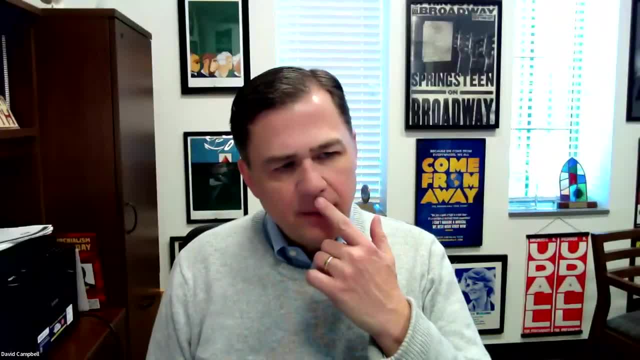 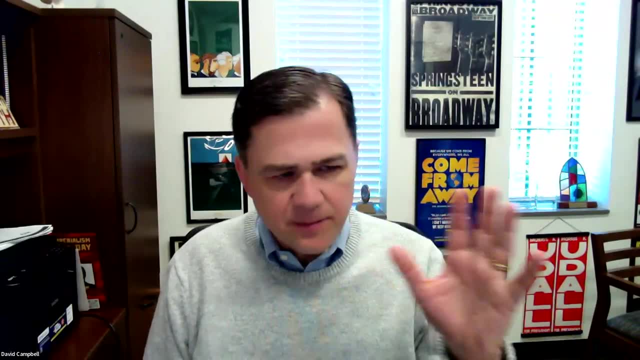 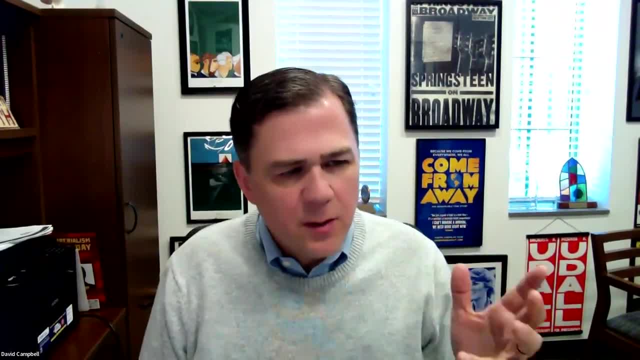 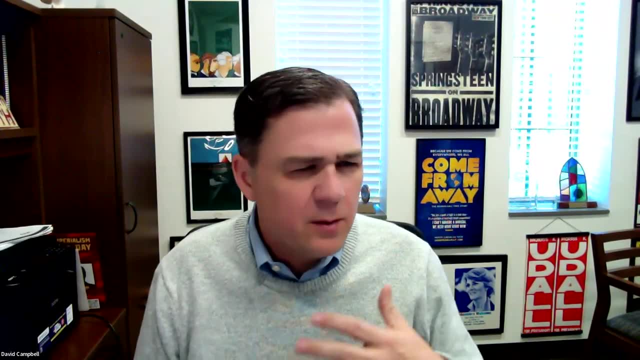 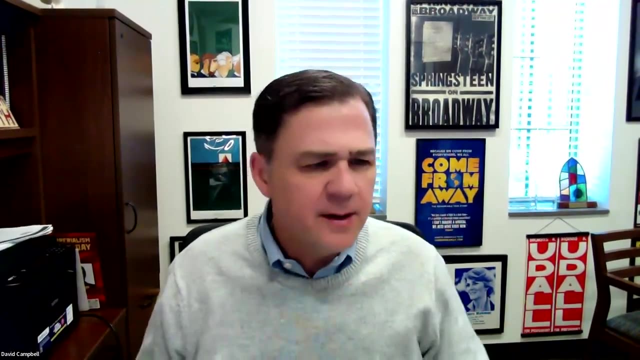 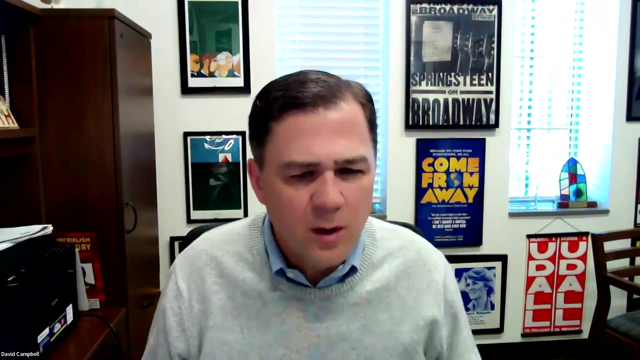 What do we do about connecting with students who feel marginalized or disaffected? Who decides what civic education is? You know, there's a lot of concern about a colonial narrative or, you know, presenting a vision of America that maybe doesn't feel inclusive to everyone. This, of course, is a huge issue in civic education and it's not 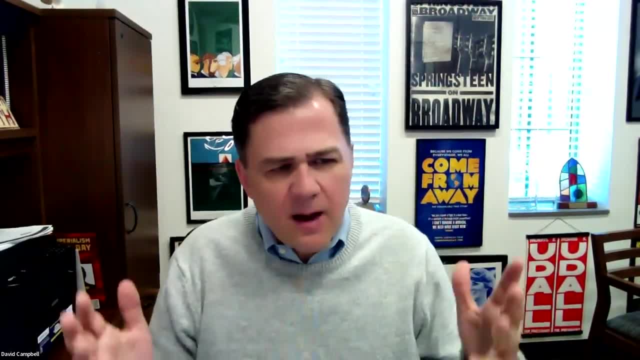 one that's really concern-ловened, It's not one that's really concern-lovening, It's not one that's that we should ignore. So let me just ask the panel: how do we do that? How do we make sure? 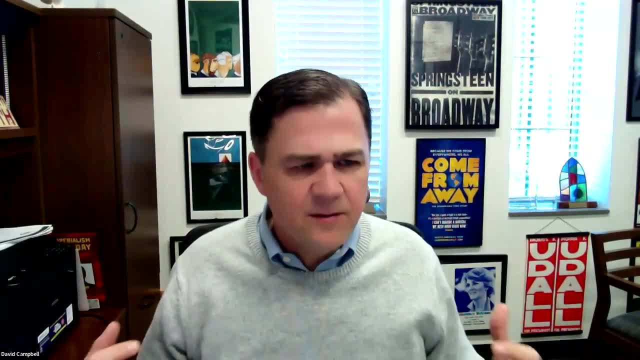 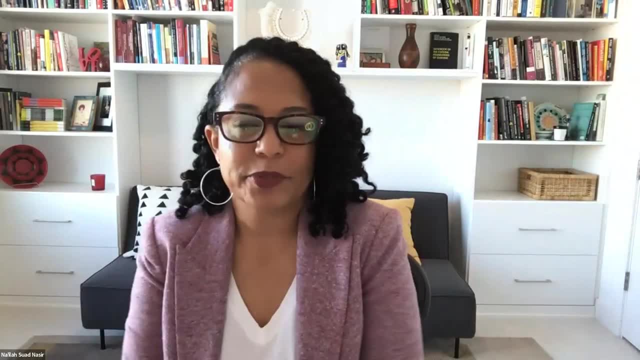 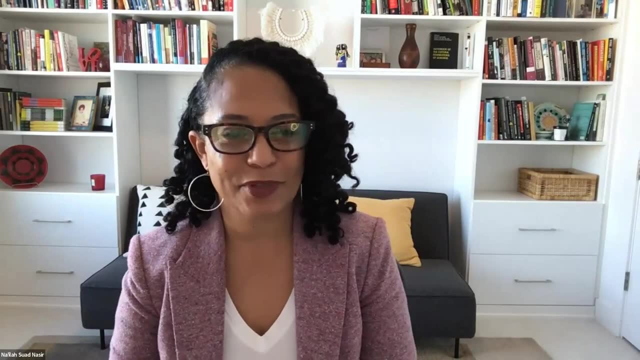 that disaffected, marginalized communities feel fully a part of civic education. I'll get us kicked off and would welcome other perspectives. I would argue two things. One is accurate: history is really critically important And I think sometimes we're in the midst of major 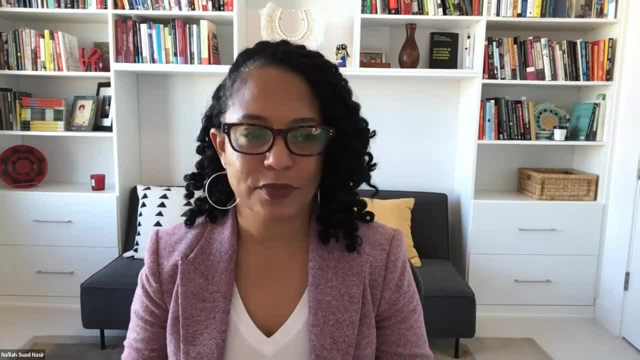 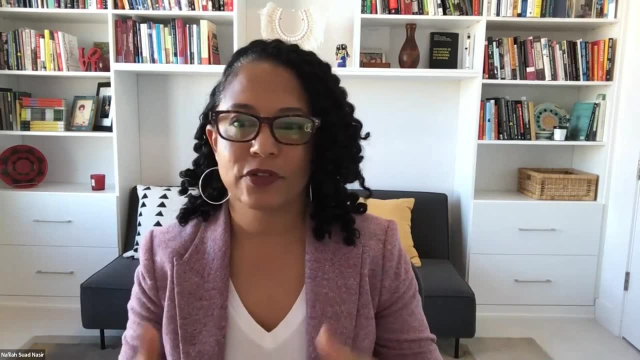 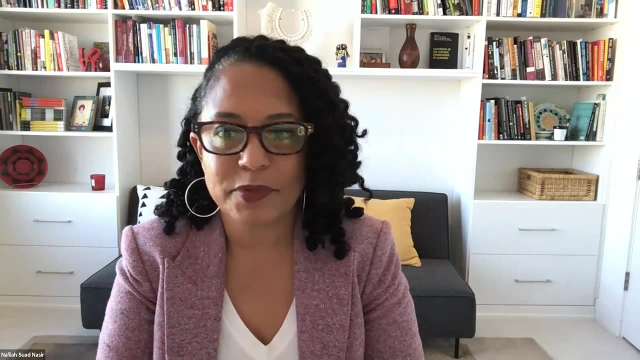 controversy about this right now nationally, And I think it's really important that we have a shared sense of the actual and accurate history of our country and of the journey of many different groups in that history. And then, second, I think it comes back to something we've 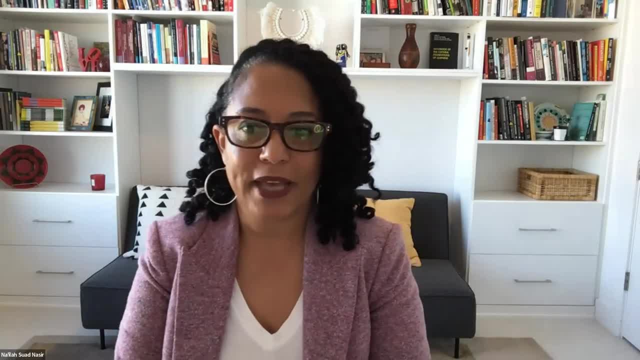 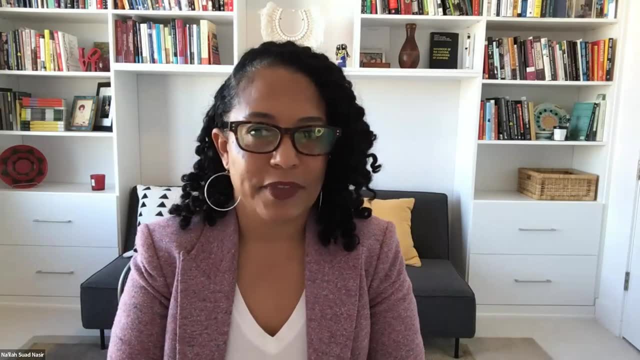 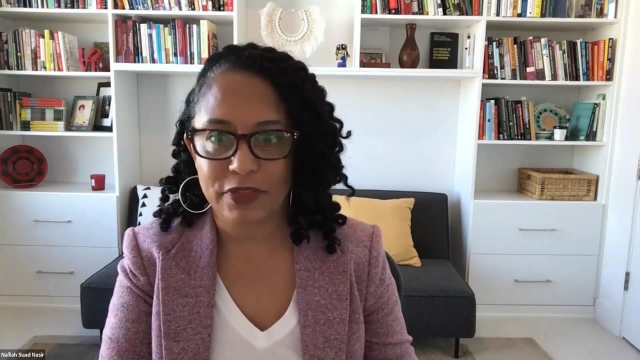 been talking about all along, which is civic issues play out in everyone's communities, And so how do you have curriculum that really roots in? what are the ways civic issues are playing out locally and creating opportunities for young people to really engage and be thoughtful- and be critically thoughtful- about what those issues are that are 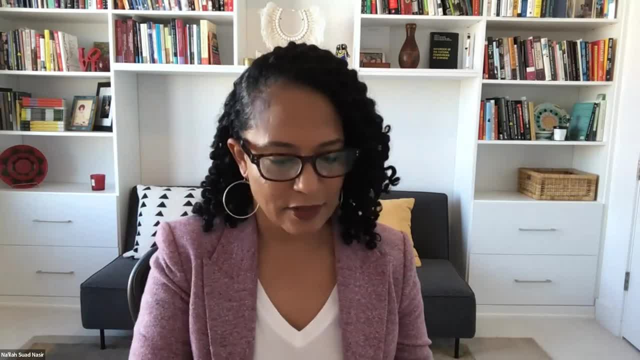 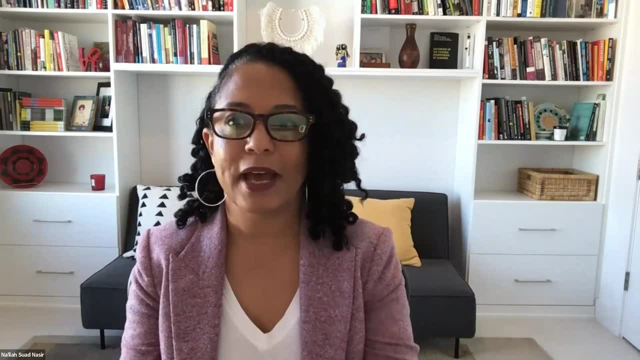 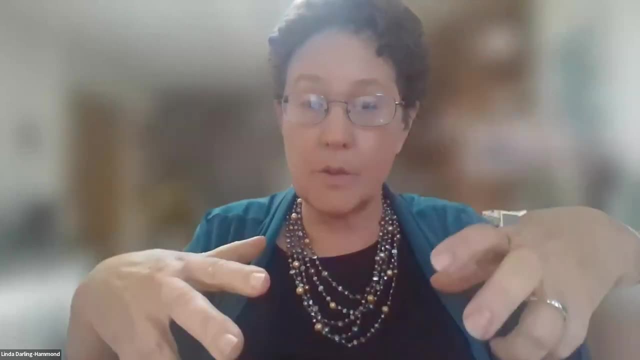 playing out locally as well as nationally. But I think that both accurate history and really creating space to take up issues that they play out in ways that are relevant to young people's lives, And I love those two And I want to just add one more, which is that in the school itself, 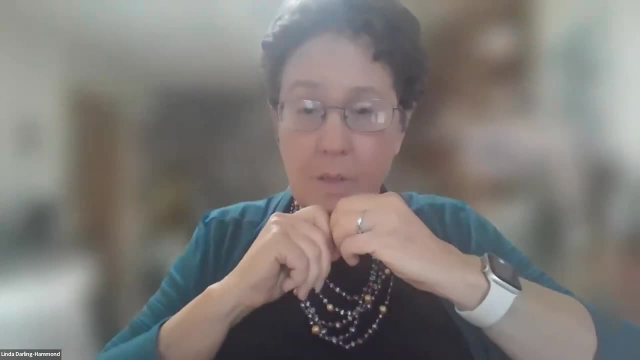 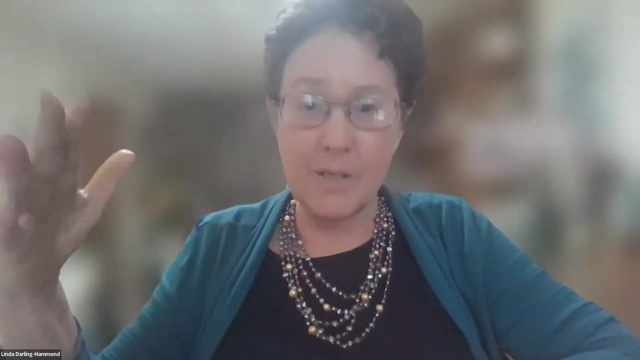 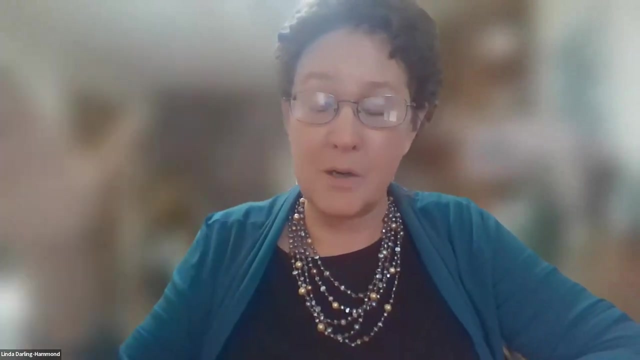 students- all students should be. you know equal members of the community. That you know there's a lot of ways in which schools can further marginalize and minoritize and create. you know the experience of discrimination that we're so afraid to teach about these days in the states that are taking up anti-CRT. 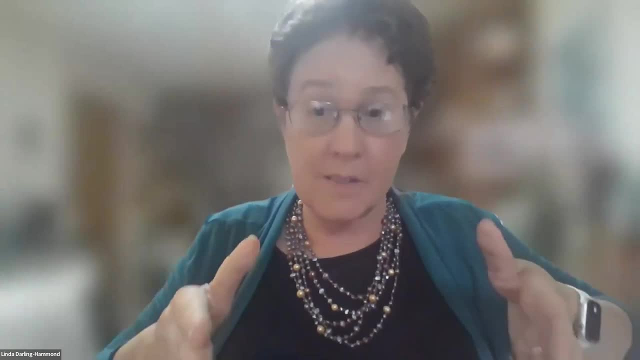 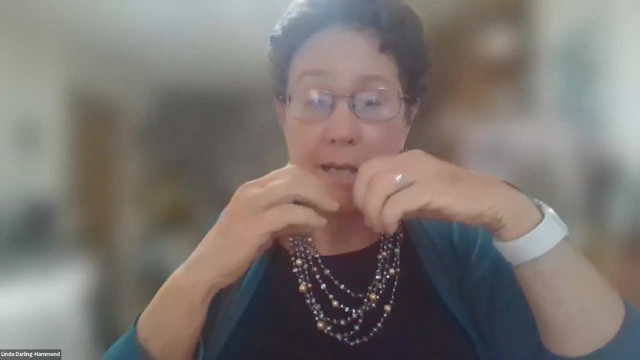 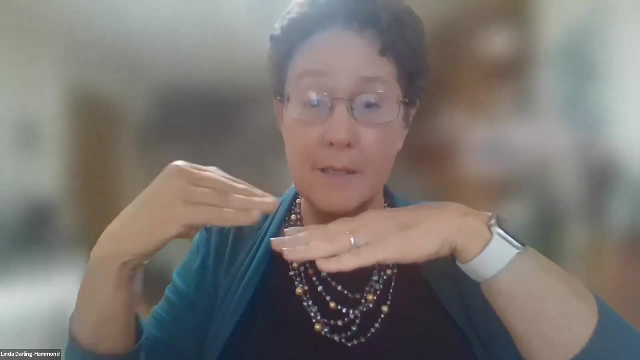 legislation and so on. So the experience that's in school itself is how people experience being citizens, And they, you know, we need to be sure that every student is experiencing full citizenship and recognition and support for their learning, which is not a, you know. 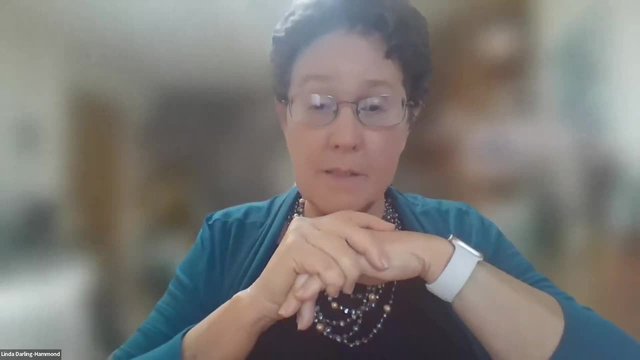 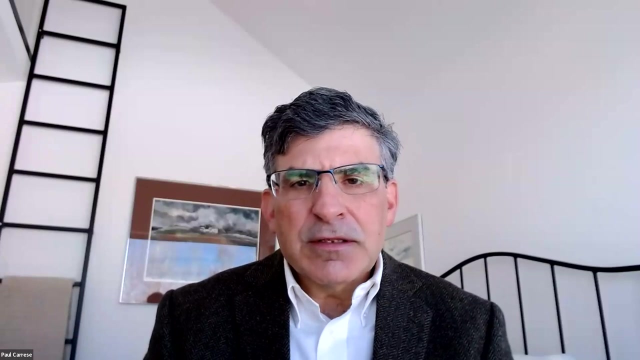 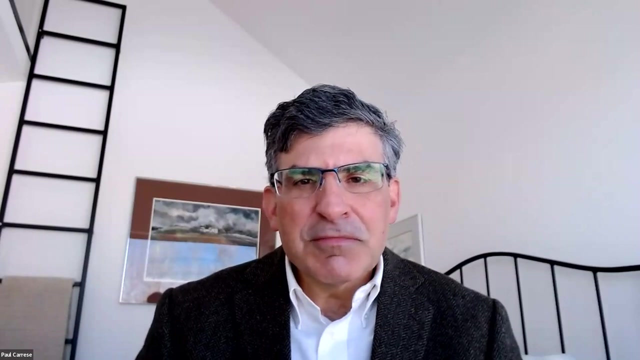 simple thing in a lot of school contexts. In the Educating for American Democracy report we tried to address what Naila and Linda have just addressed, that the phrase- the Latin phrase I used earlier- sort of the motto of the United States e pluribus. 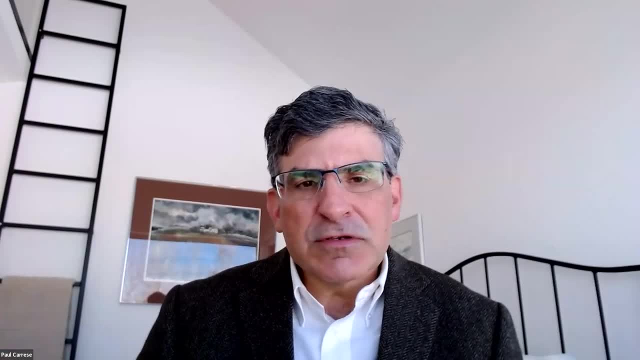 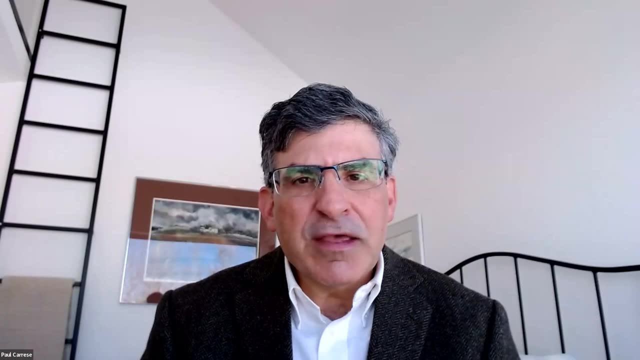 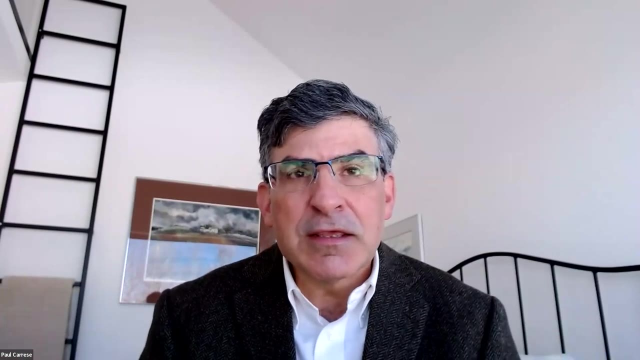 Unum has a new meaning in the 20th century and the 21st century, with the vastly more diverse range of immigrants we've had in the past centuries and the range of communities. And then we just have finished Martin Luther King Day, the, I think extraordinary. 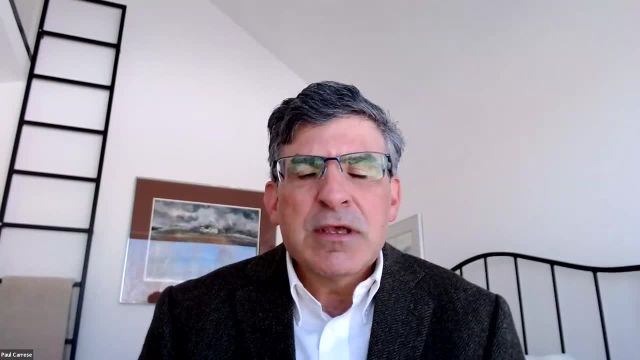 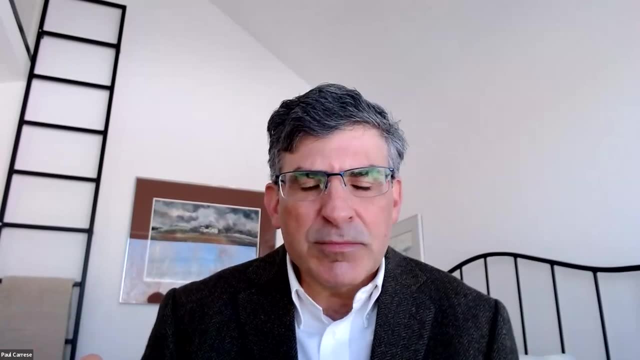 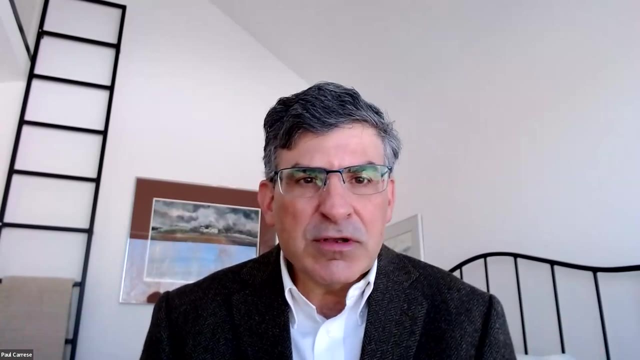 effort in 1960s to come to a new constitutional settlement about civil rights and equality, and equality of opportunity And participation for all Americans. So the challenge of e pluribus unum is at the center of the EAD set of curricular guidelines. Again, this is an effort for states, local education. 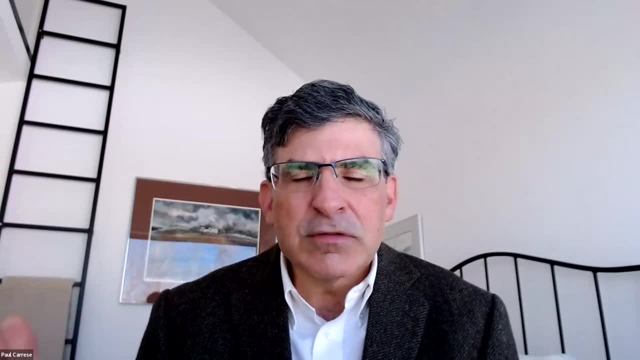 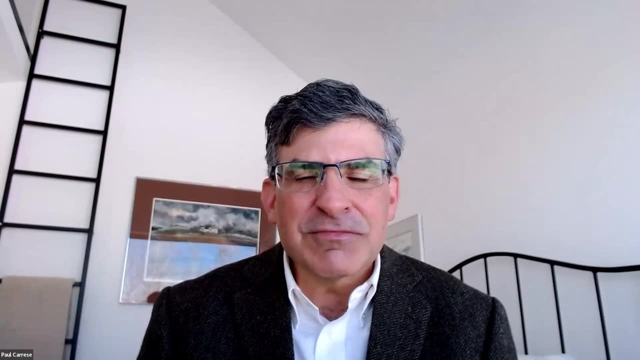 authorities to take up on their own and they would address, you know, the 50 plus states and territories, and thousands and thousands of local education authorities would address that in different ways all the way down to the school, And so I think that's a really good point. 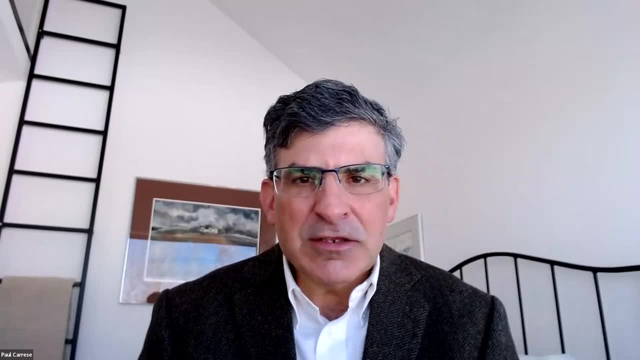 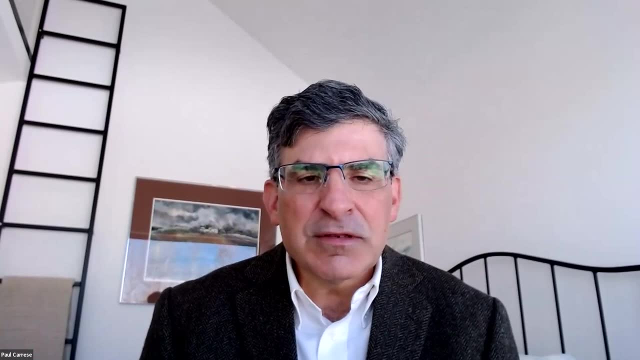 And that I think that's what we're trying to do, and I think that's what we're trying to do at the school level, But to, as Naila said, to teach accurate histories. But again, with this, the whole set of balances, the EAD is trying to achieve that. that it's. it's difficult to get students interested in civic education and American history education if they think America is. 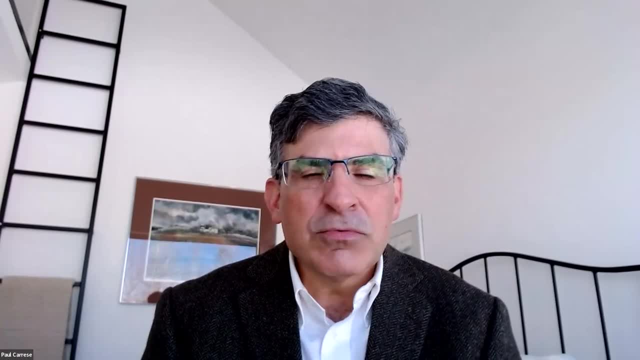 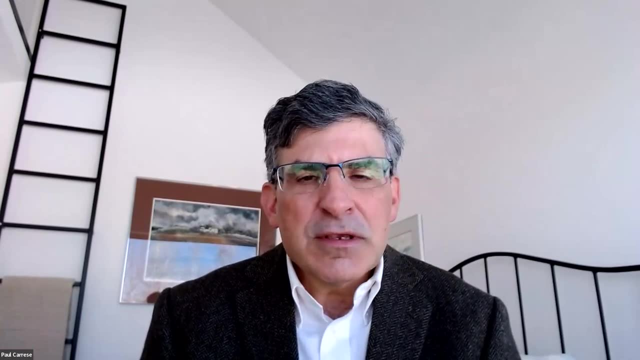 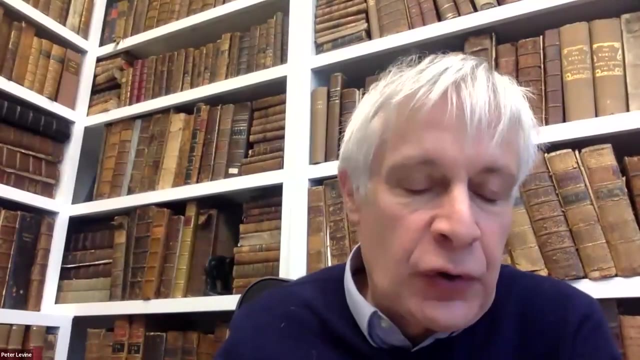 fundamentally a bad idea. So the report takes the view that we were patriotic about America in that reflective, critical. So the report takes the view that we were patriotic about America in that reflective, critical, argumentative way of being um patriotic. just make a quick, um argument for, or at least a placeholder. 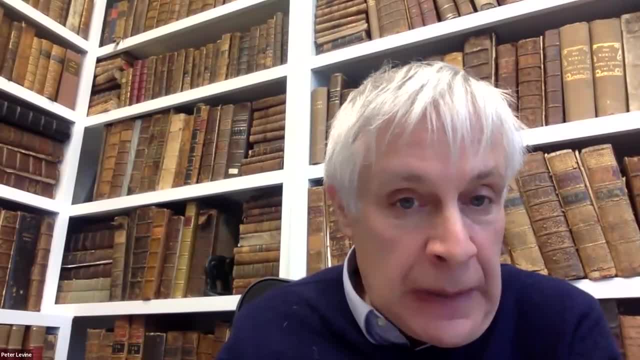 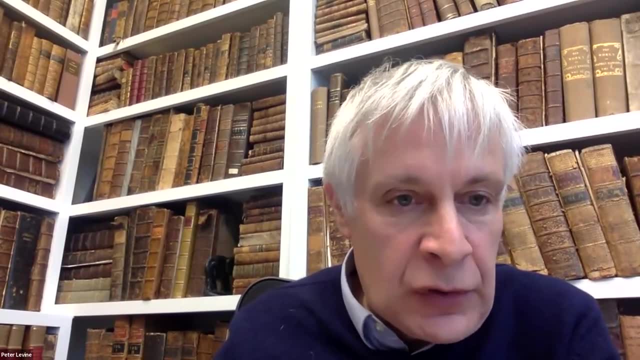 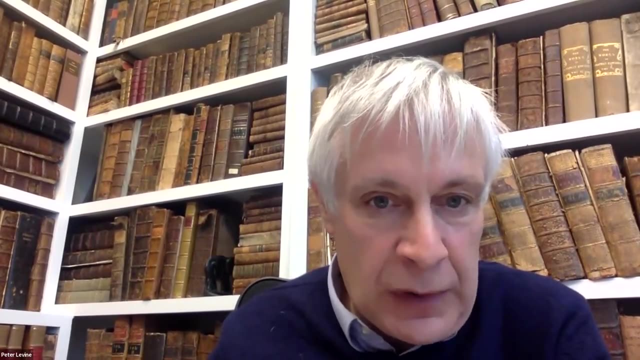 argument for some decentralization and public- and actually public- consideration of these issues. um, you know, there's a tendency to think it's a scandal if, um, different states and different communities are doing civics differently. there was a new york times piece about a year ago, apparently proposed as a kind of expose that the mcgraw-hill textbook is different in. 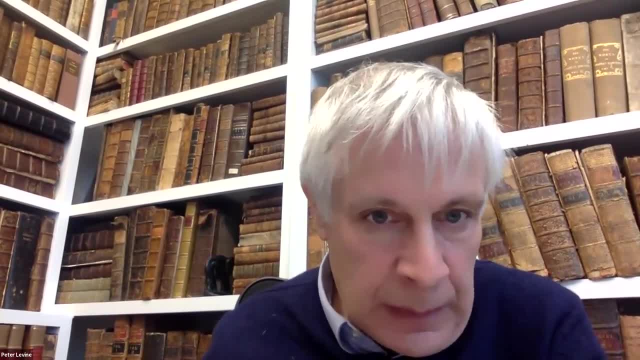 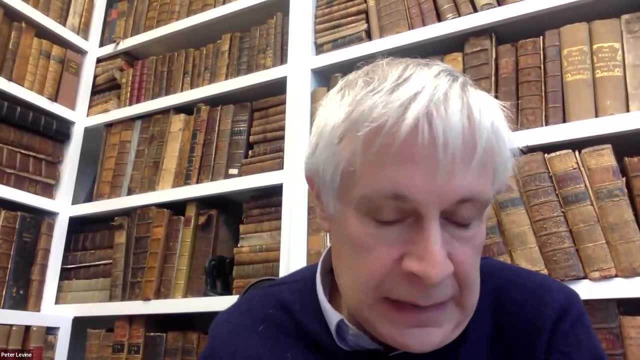 in texas and in california, but i think we're a federal republic, the textbook quite likely should be different in texas and california and also, if you have people involved in their in this debate, they're going to come land in different places given the different partisanship of the states. 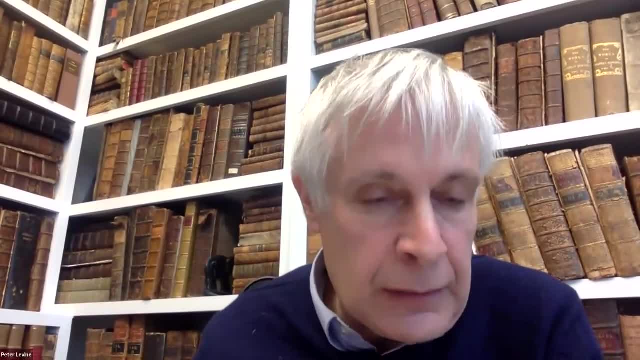 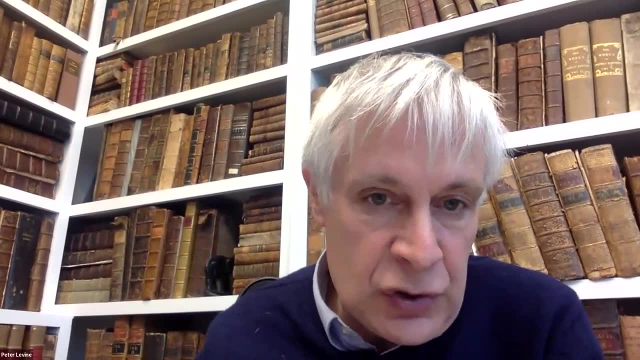 and it's actually better for there to be a diverse set of of curricula, not just at the state level, but even even more locally and even in the classroom. so some, some decentralization and then and then you know the current debate is um ugly in many ways, and that's. 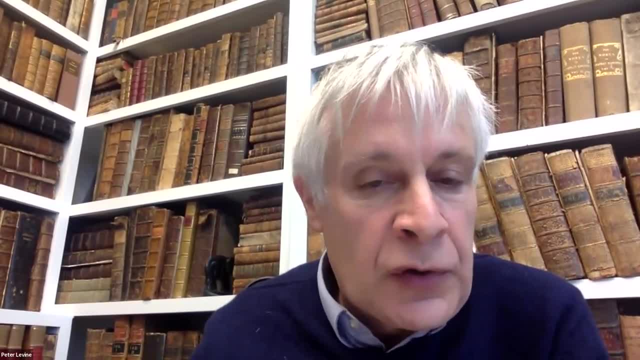 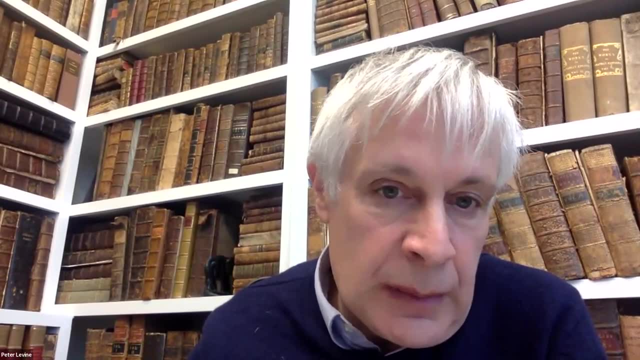 what my my piece for the volume is about, and it's- and you could spend a long time talking about why it's bad, but i also see a sort of silver liner lining. i think it's appropriate that people are debating what we teach our children about our country, um, and the alternative that we've. it's. 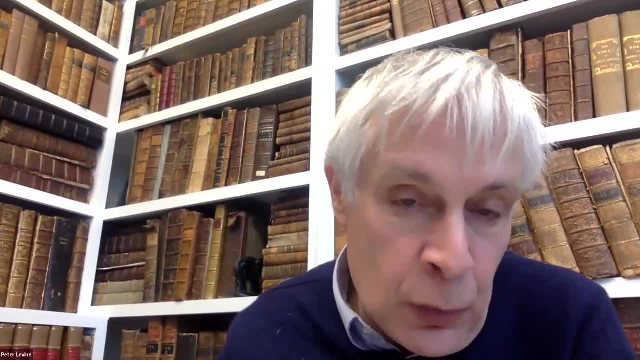 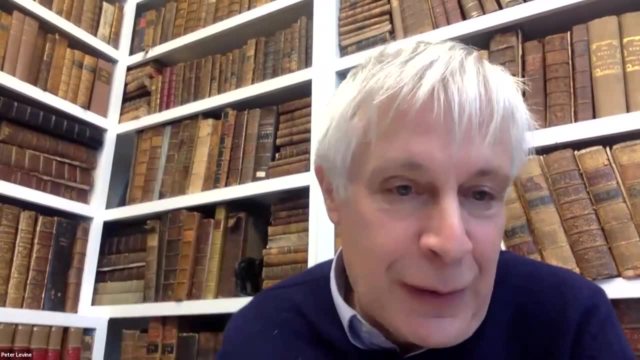 been more typical is that nobody pays attention to that at all, except for certain specialists. so the state convenes the committee to write the standards on the textbook company, hires people like me to help them write the textbook and it's all kind of not intentionally secretive but it's. 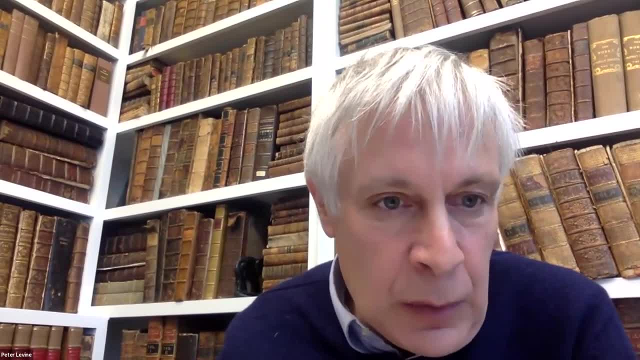 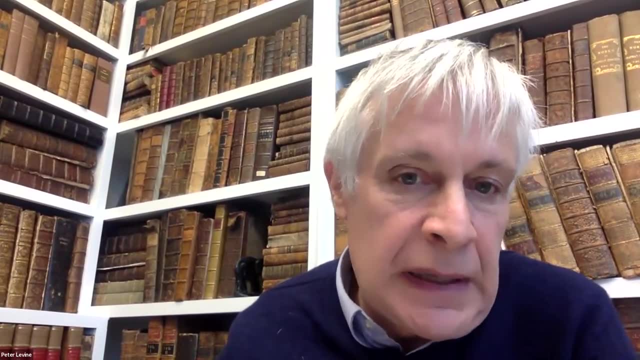 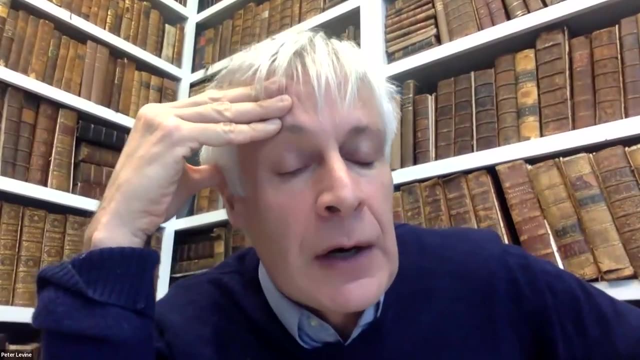 very, very low profile. it's not very democratic. so i think what we're seeing at the moment is um is ugly. but it's also- and there's it's also- appropriate that we should be debating what our various communities are, are teaching our children about, about america and about their, about the communities i think we have 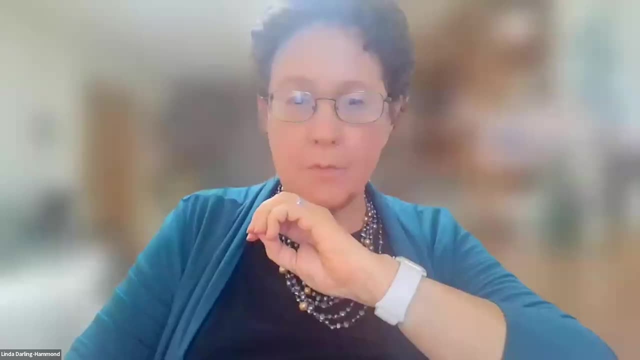 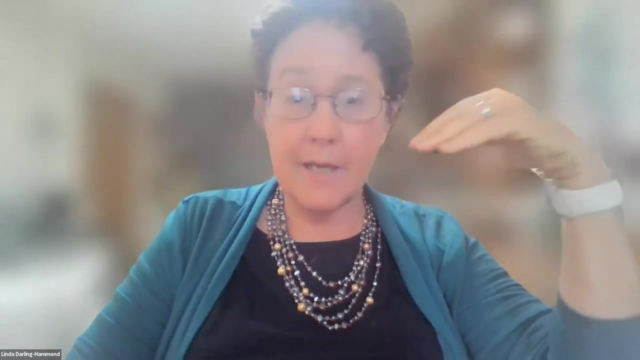 to recognize the rub that if you know there may be decentralization and different you know- views, but if what's being taught in texas is not accurate, if you know slavery is viewed as an individual freedom, um, you know that we, you know, should be honoring even today. you know we do have some fundamental questions about equality in this. 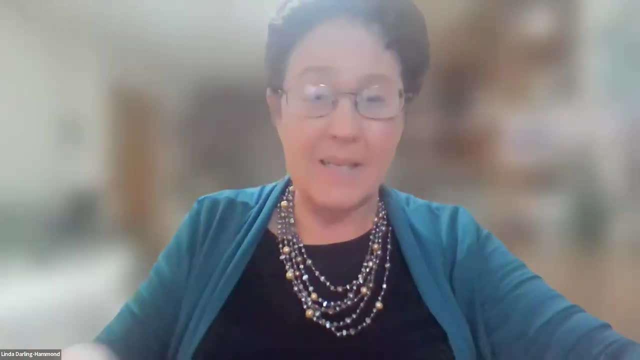 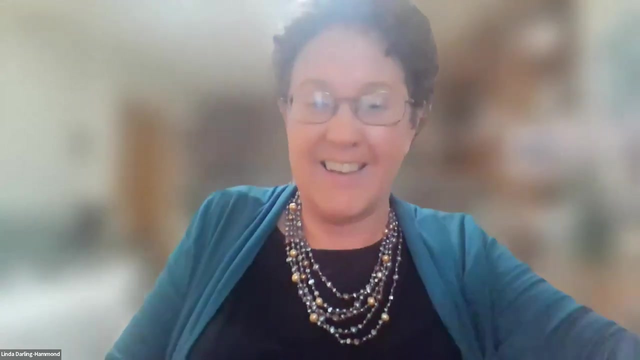 country that um are being litigated. you know, being litigated, if you will, and um actualized in these debates that we have to recognize um in the in the quest for a more perfect union. you know, it's not everything is not everything. no, i agree. and just to reinforce that, i mean if, if the florida, african-american 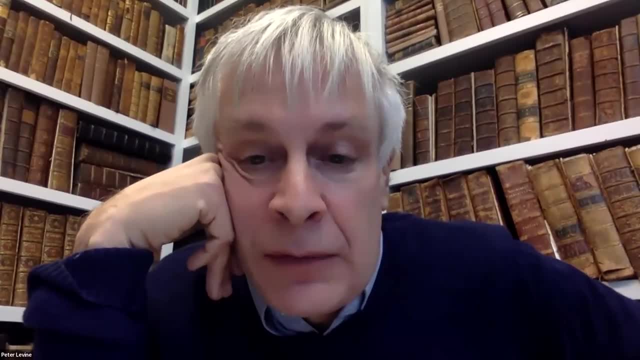 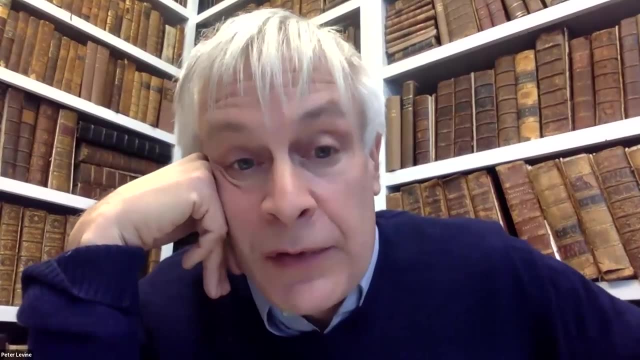 history standards. they seem to be my business. i don't live in florida, but i don't like those standards. i i i thought about them, i read them carefully, i read various critiques, i read defenses of them. i am against them and i think that's my business as a, as a somebody who cares about the. 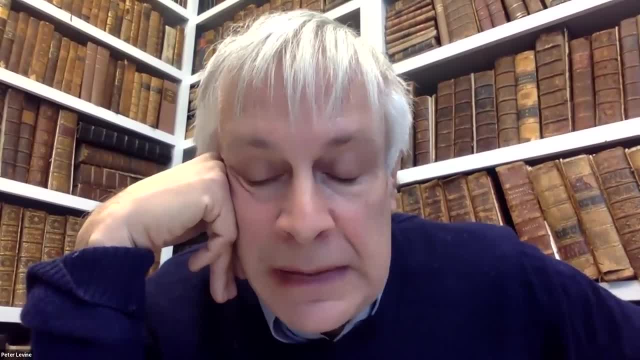 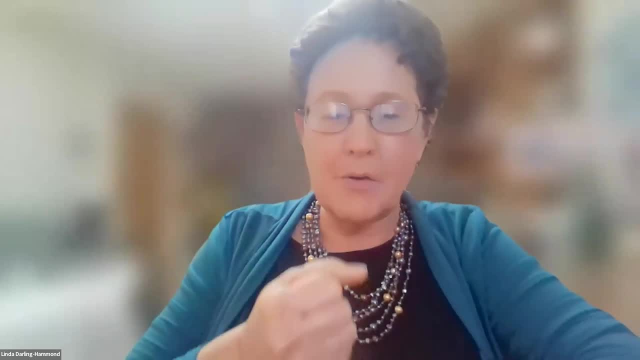 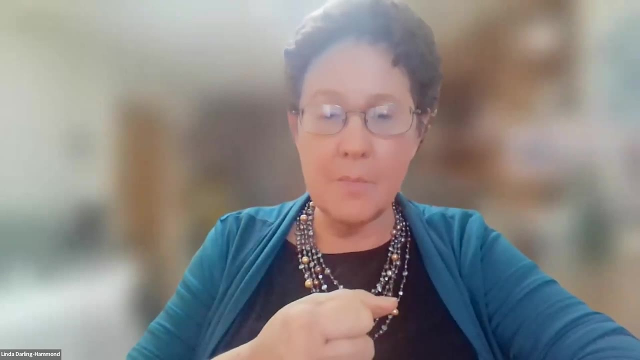 united states, uh, the republic. so it's not a matter of just completely delegating everything to localities, although i do think that was a particularly problematic. the question about is: there is there a common? uh, to back to the sort of um civic virtues: they rely on some common. 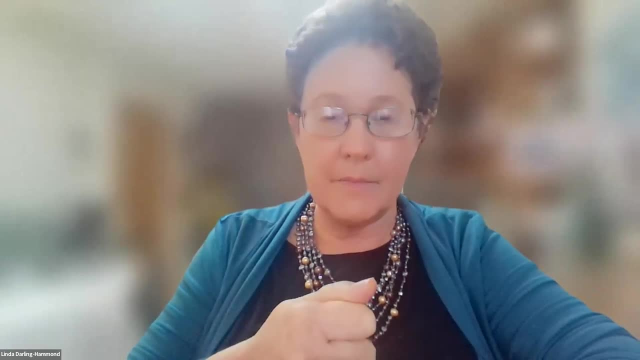 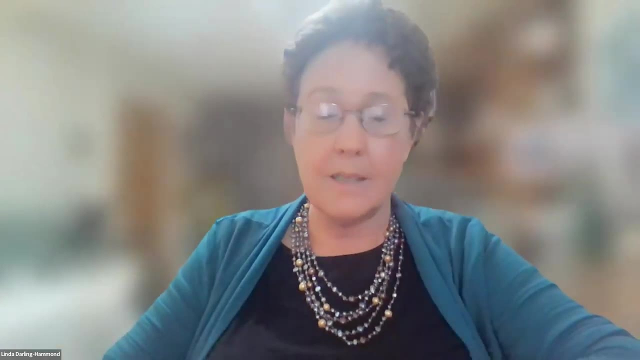 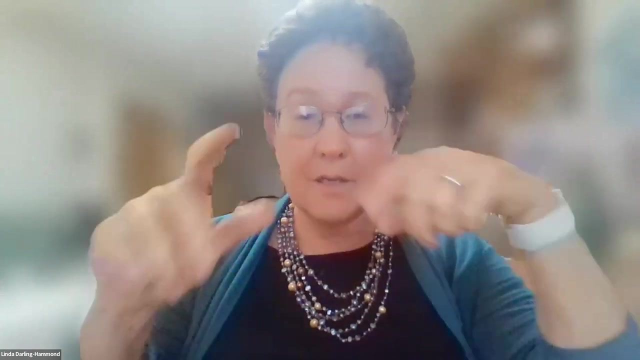 understanding about principles of equality, and i think, when those are shaken, as we see them increasingly again, it's not that they've never, you know, been settled, um, but uh, that that i think that that, then, you know, raises the question that how do you have the civic engagement, the 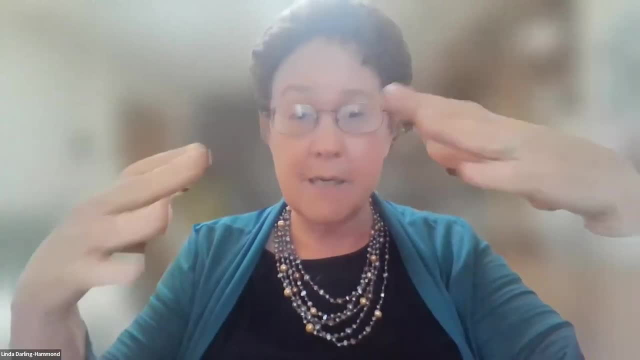 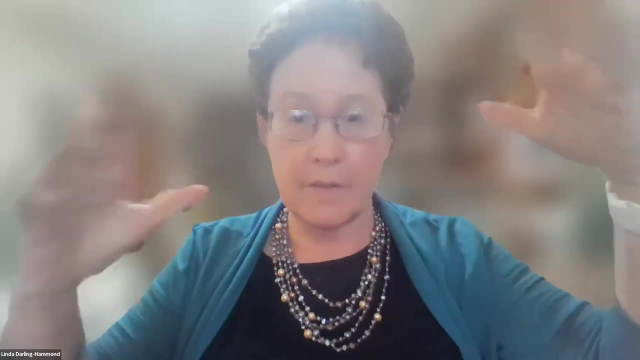 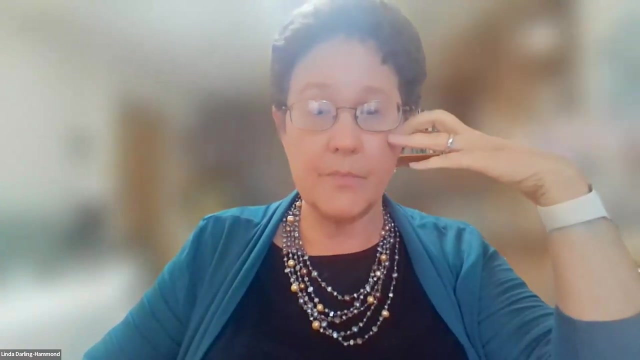 civic discourse, the, the, um, necessary, uh, repair functions in a society that where you see the fraying of those core principles that would enable the democracy to move forward. now to pick up on a theme mentioned earlier i can't mention. you know there are, there are some polling survey results. 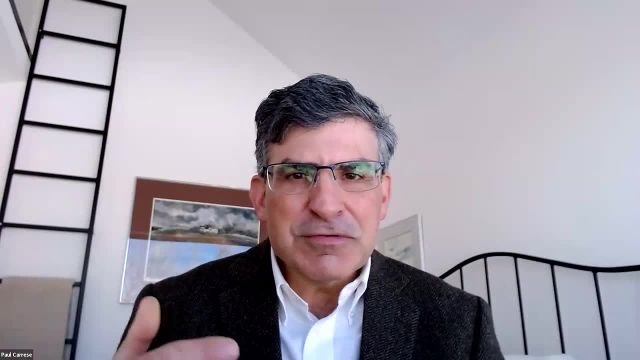 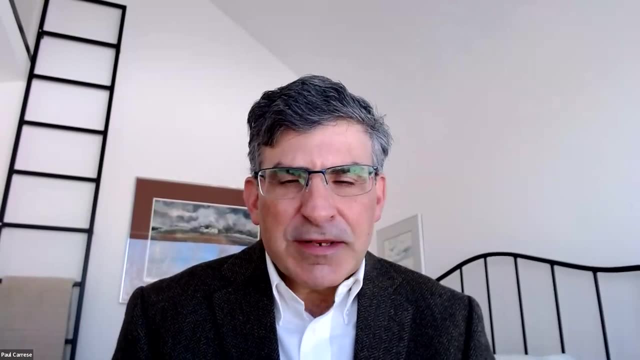 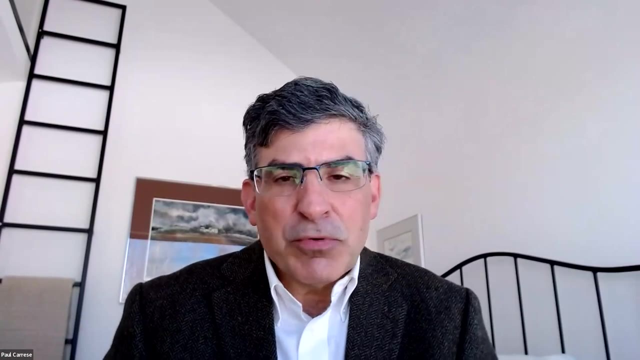 which suggest not all the news is bad. um, i guess you know, peter, just mentioning it's a good thing. we have controversy about attention to civics education. this, this is the silver lining in the crisis and i can't mention there. there are- uh, there is evidence that there is a broad middle. 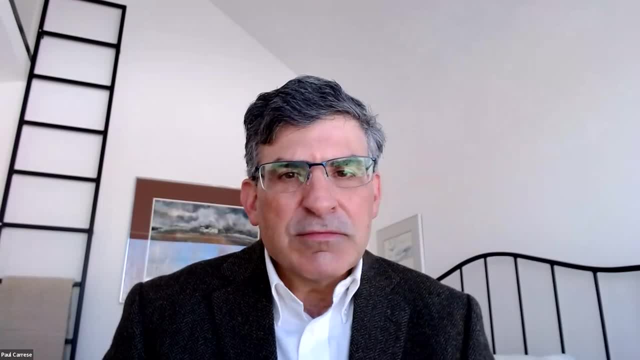 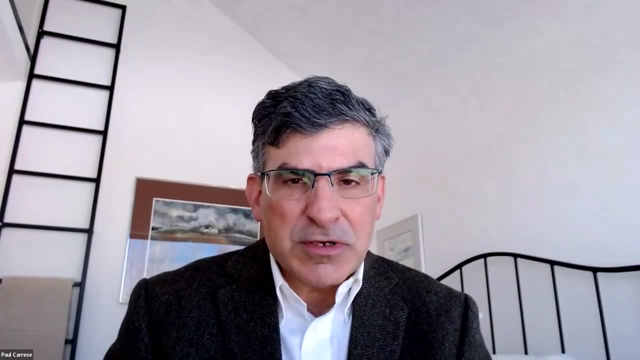 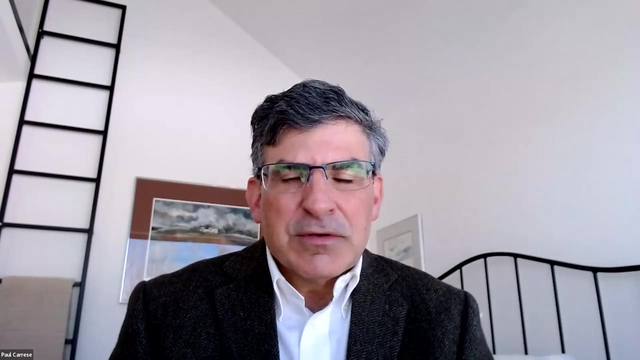 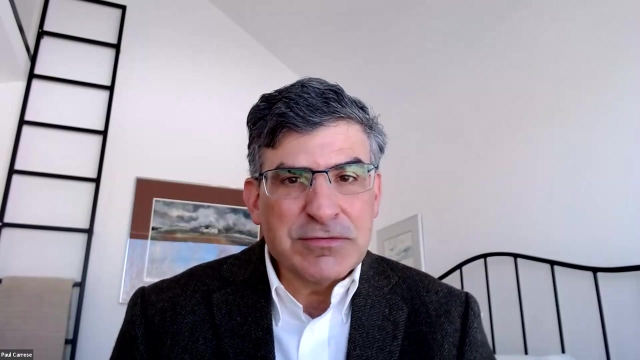 so to speak. that's what we tried to represent in the ead report of parents and and other adults who think we should teach accurate histories, but we can also be patriotic about america, just to have that point. but this is, this is very hard work, uh, and i there, while there is some good news, it really, it really is a crisis. just to take two: 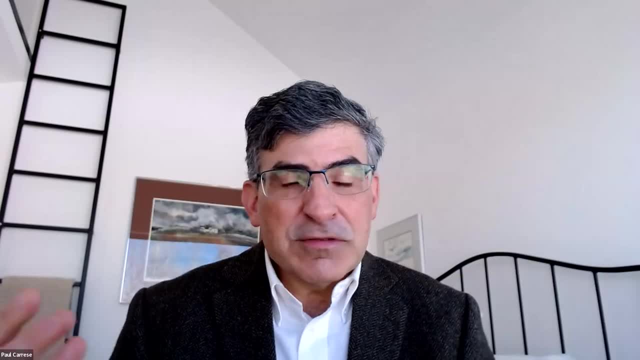 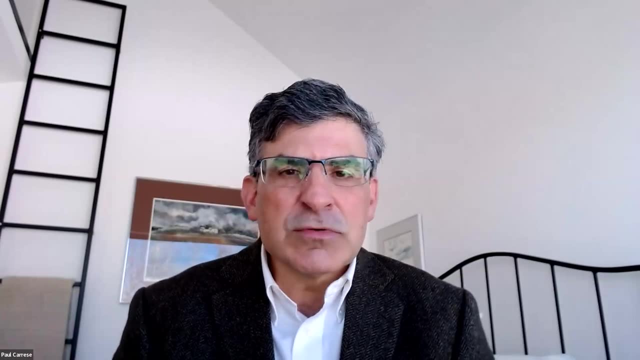 two pieces of evidence. niall is talking earlier about the. you know the difficulty of being a teacher, that the stress of being a k-12 social studies civics teacher and even elementary school teachers who think that civics, social studies, history education is important. uh, at my, just an. 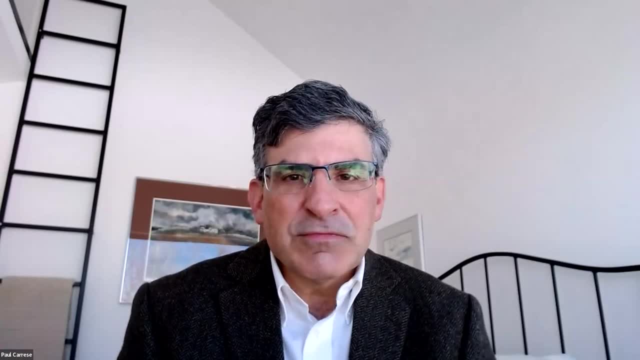 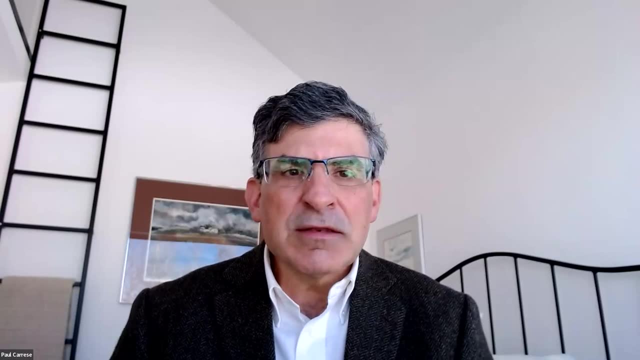 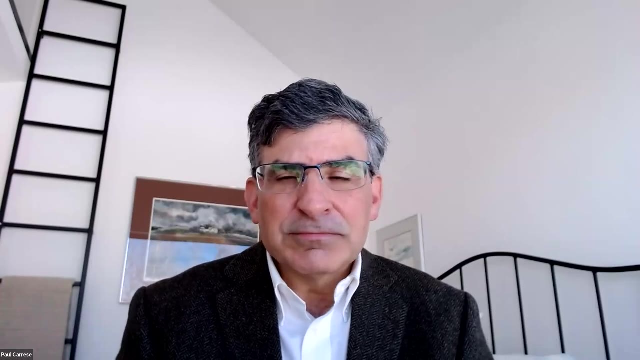 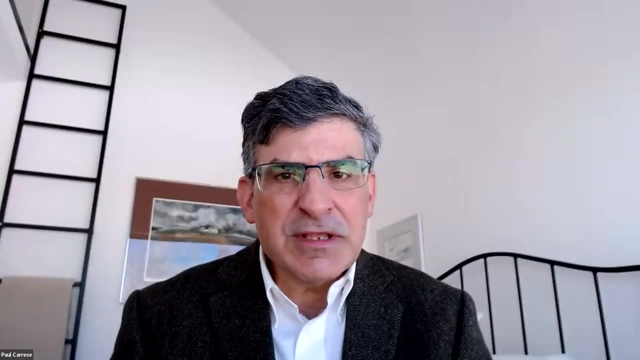 anecdotal piece of evidence at my university, arizona state university, the largest university in the country, which has sustained student enrollments by having a very large online capacity, online degrees- uh, you know, enrollment in the teachers college is down and you can understand why. for a whole, a whole range of reasons, but another very troubling set. 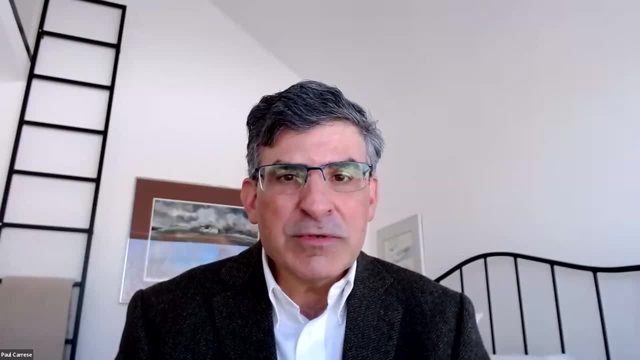 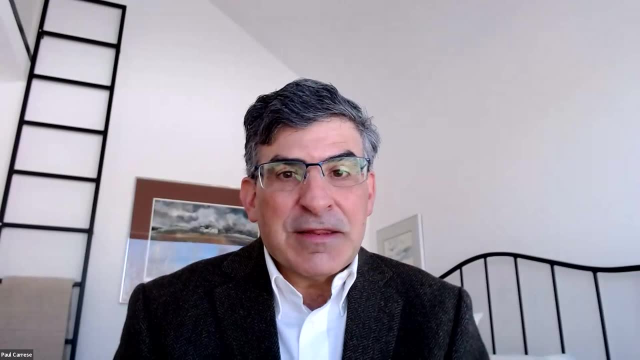 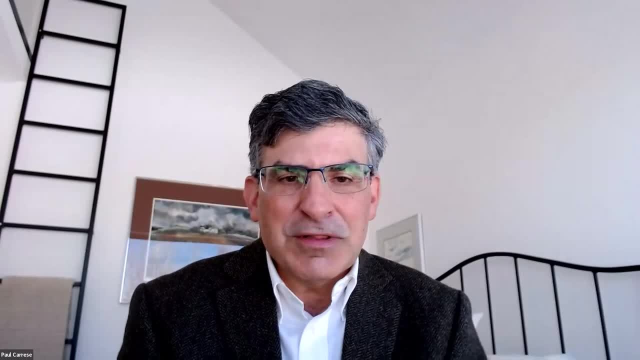 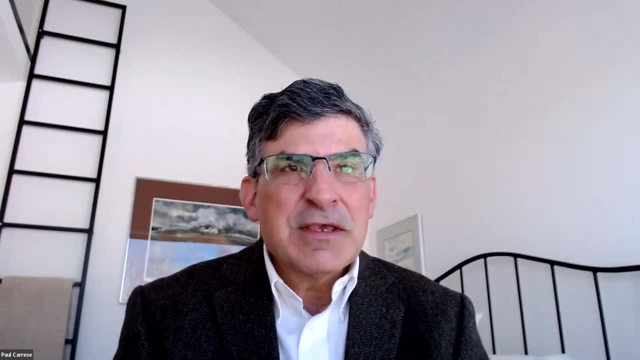 um and and the polling on a civic attachment, as the social scientist would call it right. do you think america is a good idea? are you patriotic? uh, do you think it's worthwhile to live in a democracy? if you look at the numbers in the various polling results for people under the 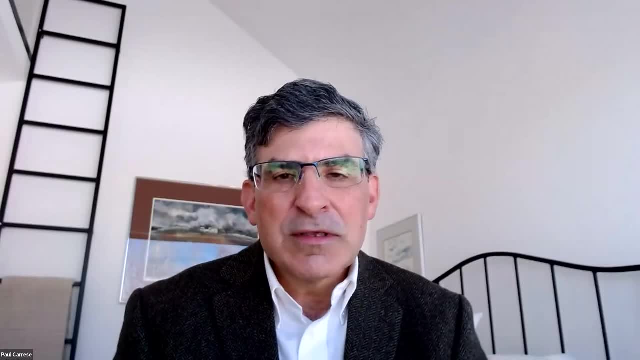 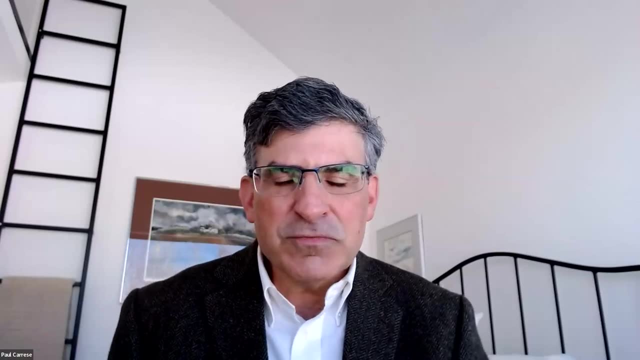 age of 30. it's underwater, america is underwater. so are there a question: are there enough people in the adult community, across a whole range of professions involved in the movement, and is there enough people in the adult community, across a whole range of professions involved in the movement? and is it something that's not going to be able to be done ultimately, because then you're not going to be able to do anything exactly? 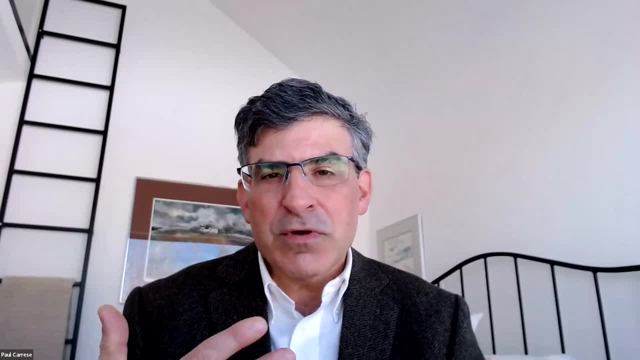 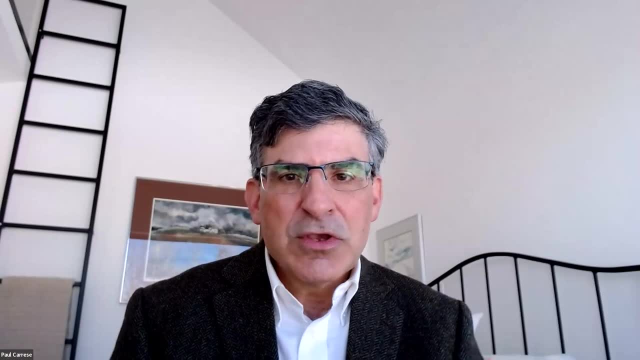 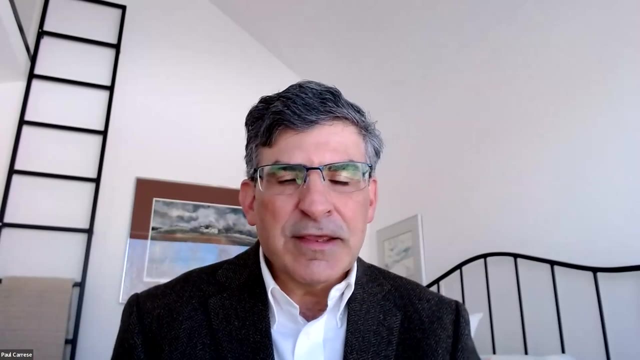 in this debate. are enough people who respond to crisis with turning toward compromise in some way, listening to each other, hearing each other out, making some difficult compromises- or is the response to crisis to double down on your own side and, in a way, continue to fuel the polarization? 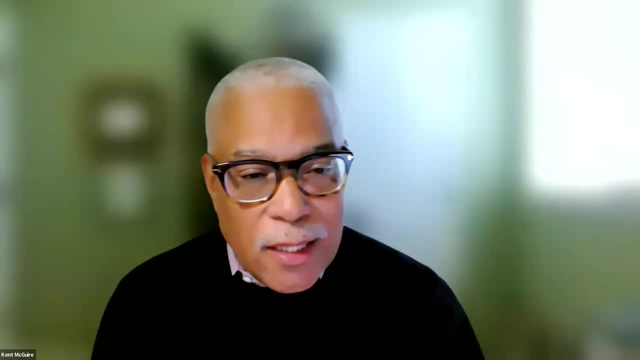 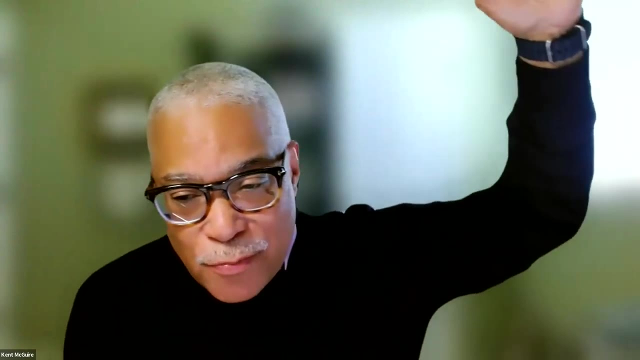 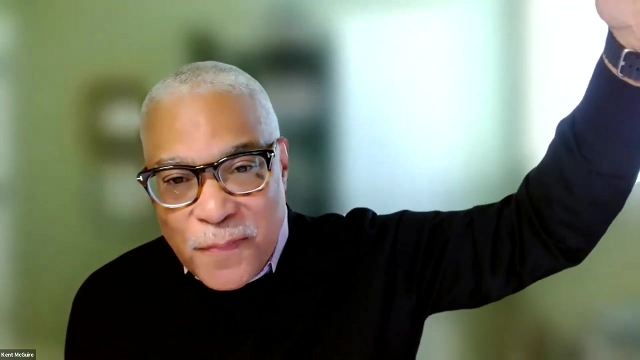 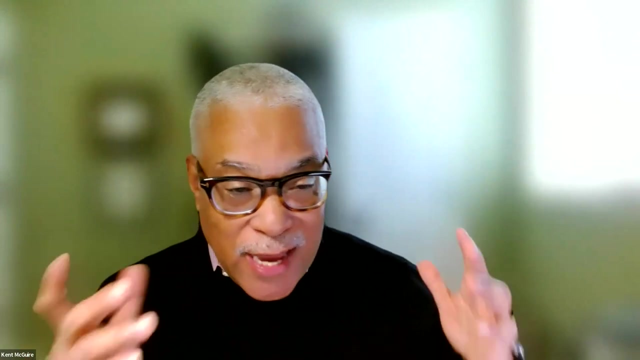 and the anger, Yeah, and that all seems right to me, Paul, And it's a problem that sits above this conversation about what the schools should be doing. I mean, I do think that, at the same time that we wrap our minds around some 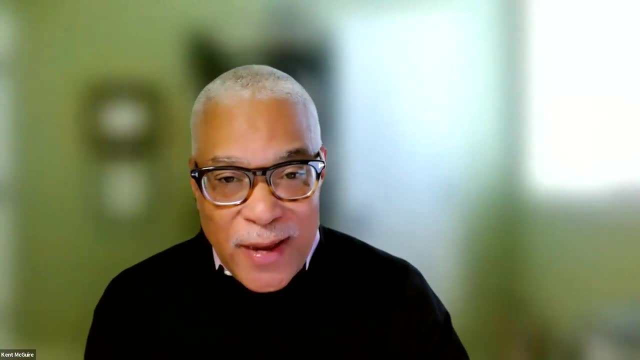 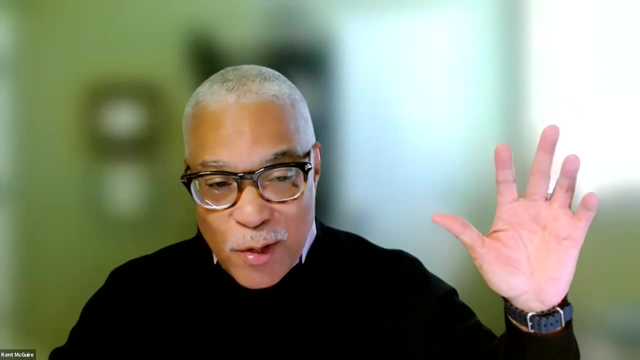 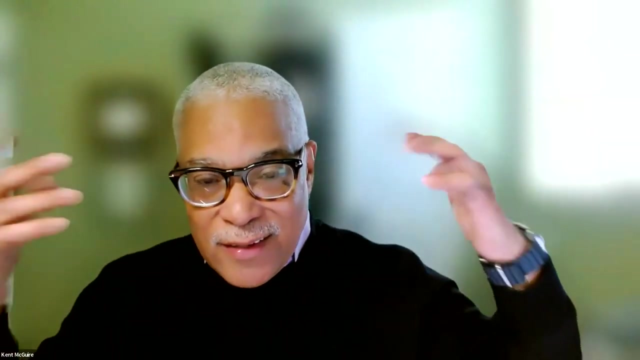 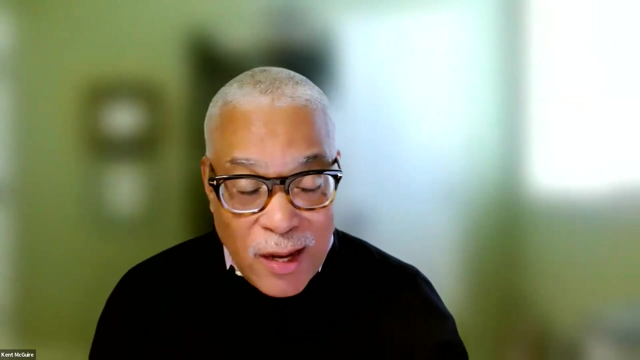 obvious ways the schools could get better at this. I think you aptly describe a world in which you know, I actually think bad actors are sowing mistrust in democratic institutions broadly speaking, And unfortunately, just to connect the dots, they've decided that the public 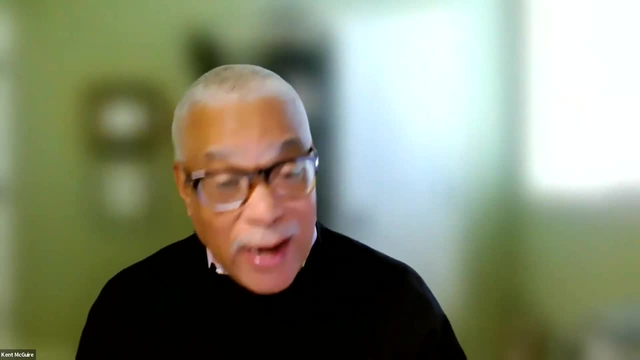 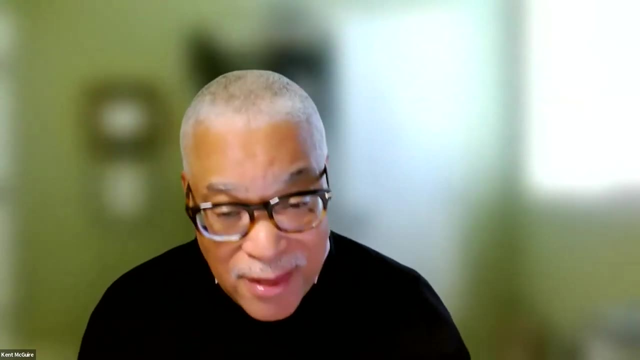 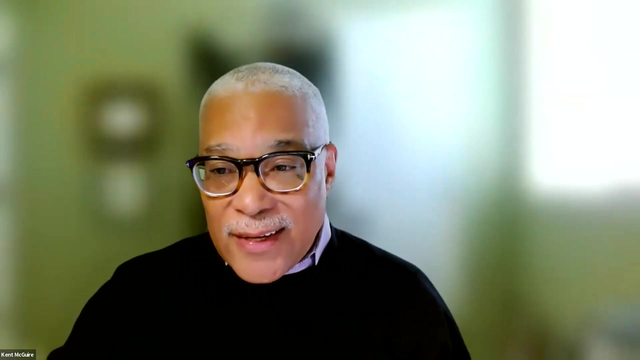 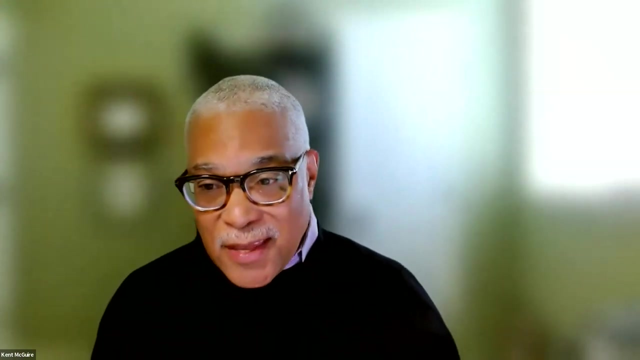 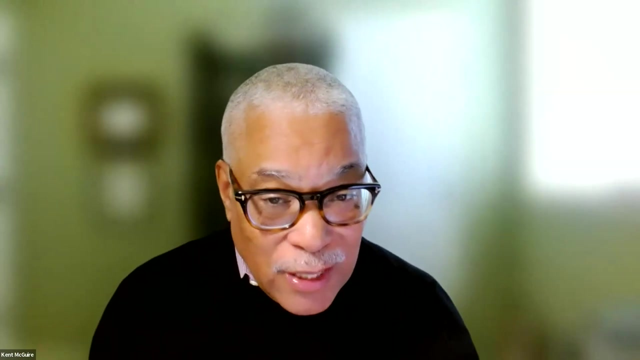 schools are easy Right In which to do this, for reasons, I fear, that have little or nothing to do with the schools themselves, but leave these chilling effects, to which Naila spoke, you know, for us to deal with. So we it that's, you know. I wish it weren't so. The glass half full guy in me, sort of. 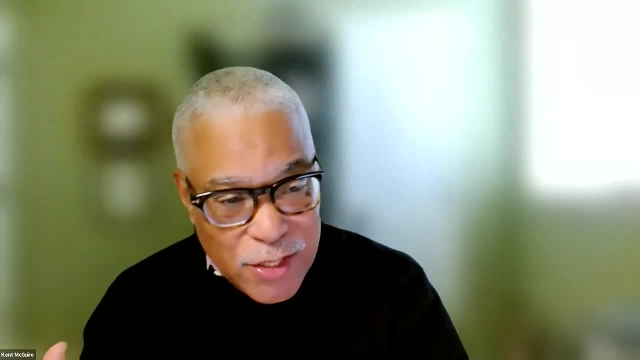 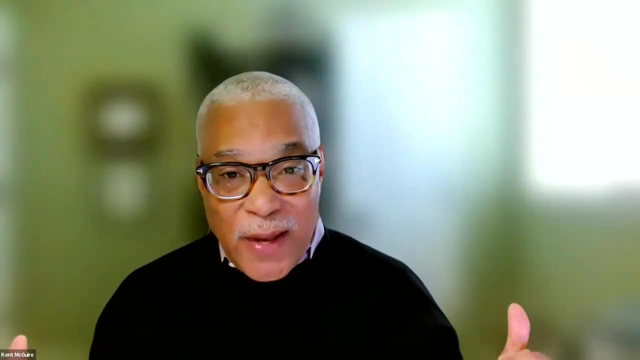 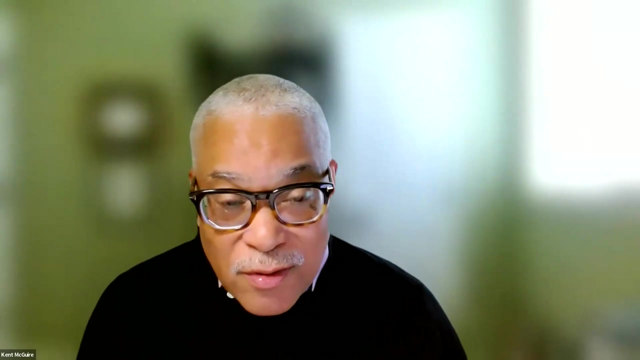 comes back and and lands on the fact that, you know, most reasonable people don't want the world to look like that, And so we really need to figure out how to wake them up and, I think, help them, you know, sort of engage in, I think, these very serious issues that you, to which you refer. 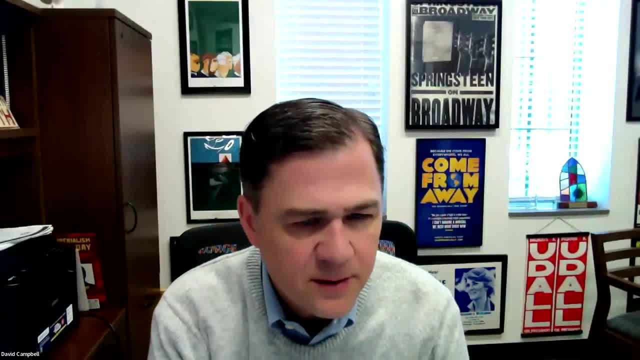 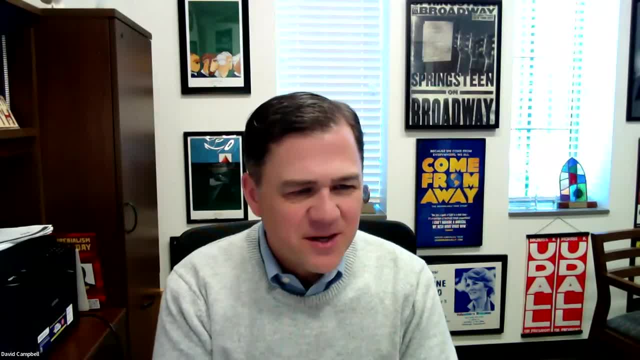 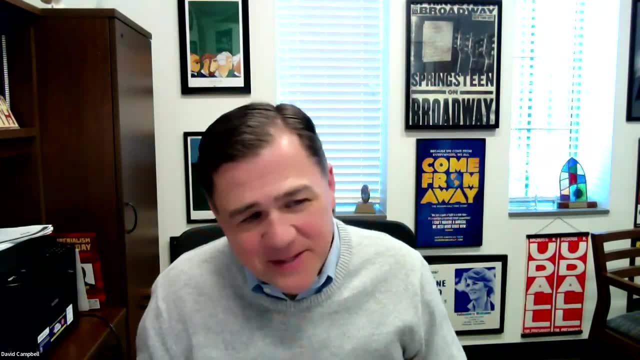 the questions. There were a few mentioned that we won't have time to discuss, but I nonetheless will flag here because I want us to walk away thinking about them, And one of them is, frankly, kind of a juicy topic for this panel, which is the role of private foundations and philanthropy. 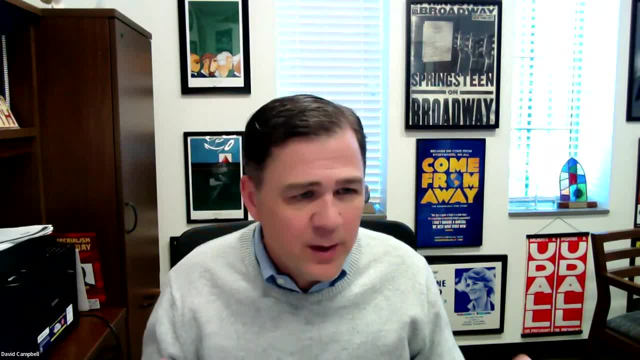 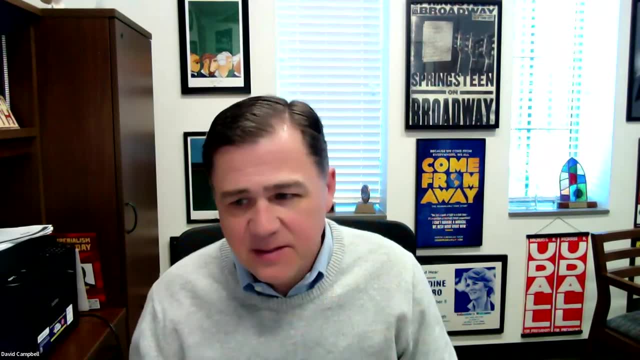 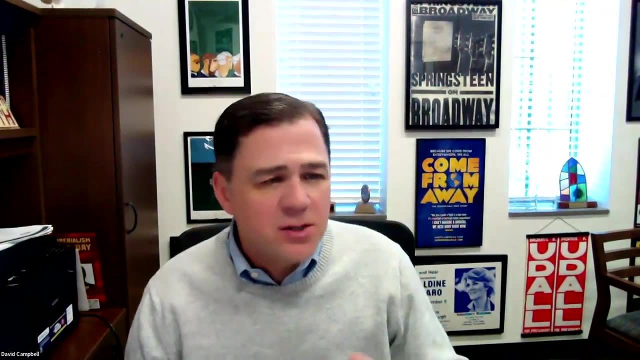 in civic education. What does it mean when we have a larger role for private philanthropy? Does that mean that the state is receding And what does that say about our civic life? I think that's a big question. It's worth thinking even more than we have here about marginalized. 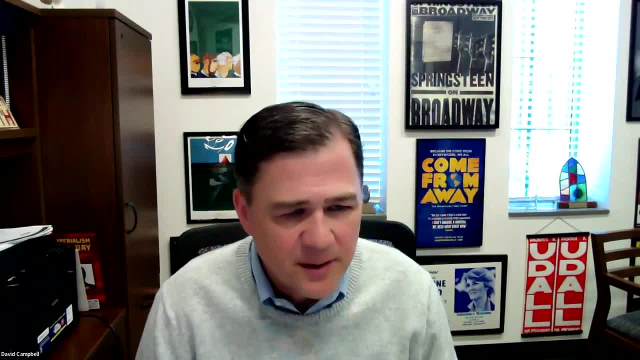 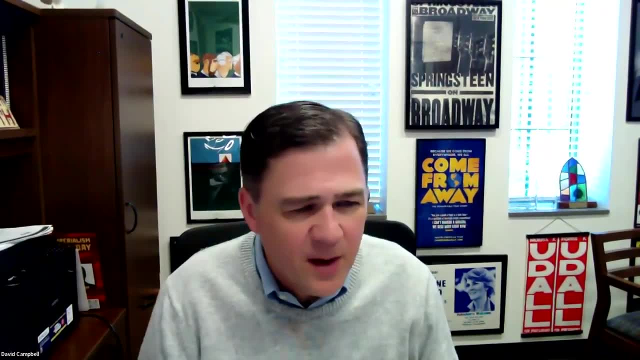 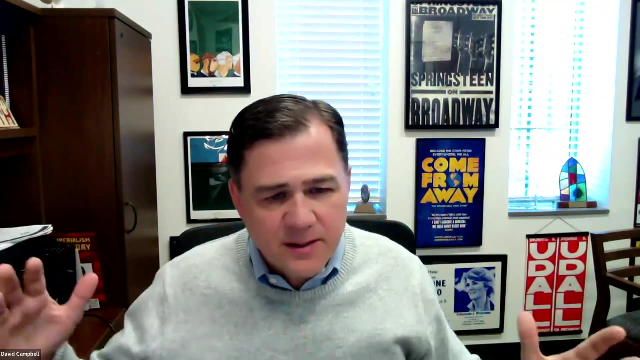 communities and how they can be fully incorporated into civic education, And we've had a little bit of disagreement here and it's worth wrestling with the idea of how much of civic education across at least the United States should be common, and how much variation would we expect to see. 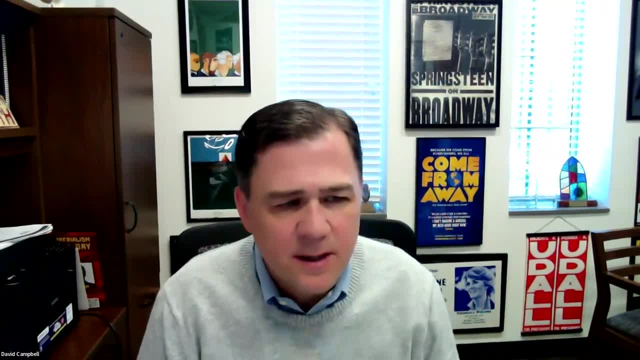 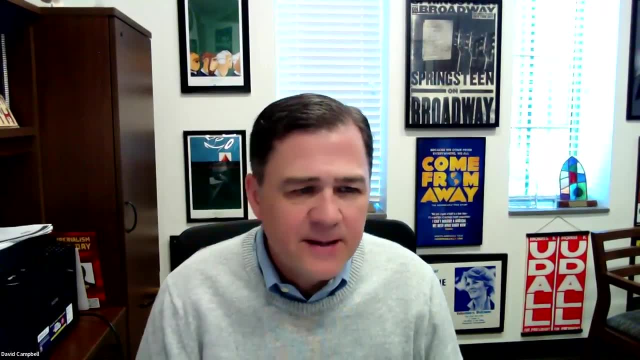 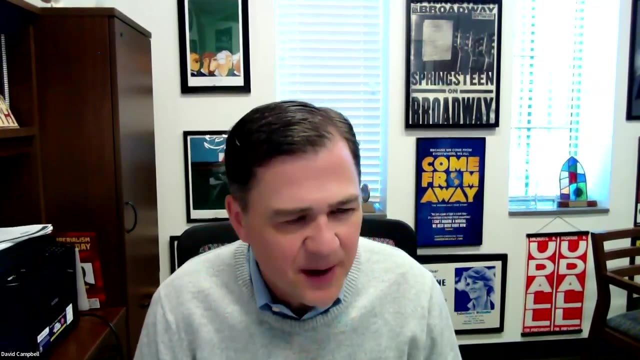 across communities and states, And I think that is a tough question and one that we've seen a little bit of disagreement here on, and one worth thinking about. But, as I said, our time is up, and so we won't be able to cover all of those themes, But let me just wrap things up by once again reminding 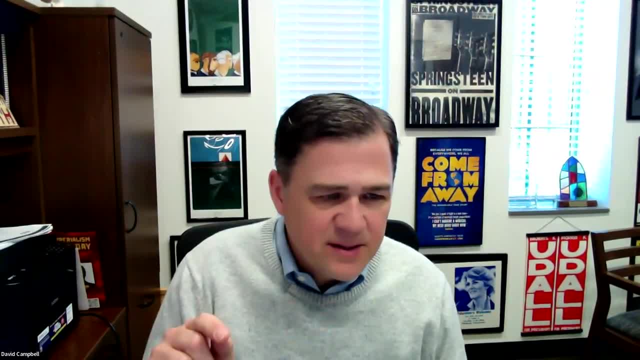 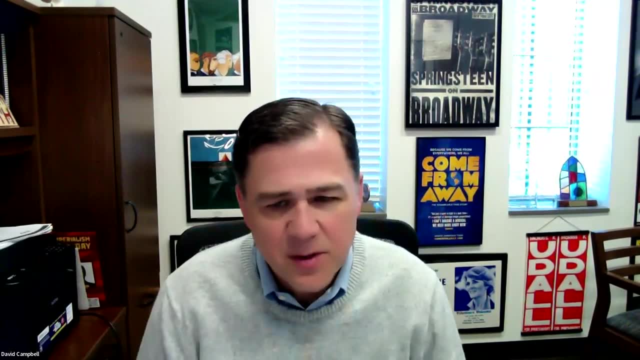 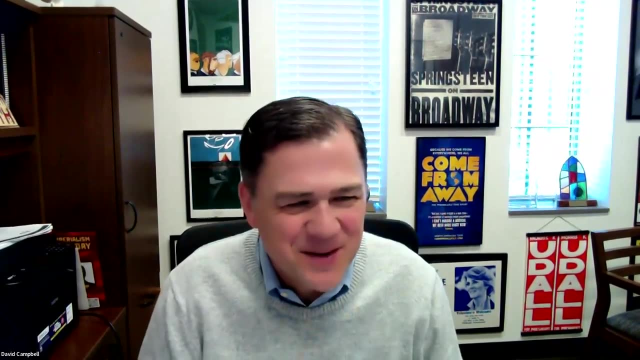 everyone that many of the themes that we've discussed here, and even more, are contained in the issue of the annals of the American Academy of Political and Social Science titled Education. There it is in a time of civic education, in a time of democratic 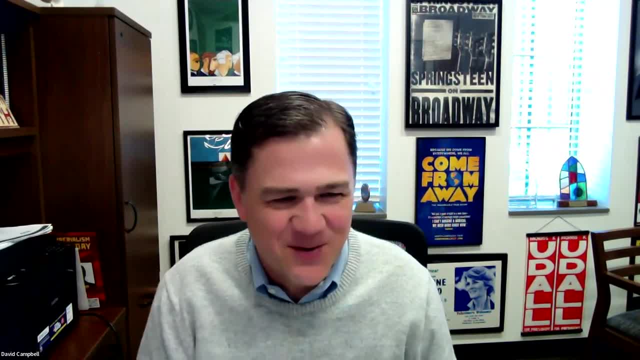 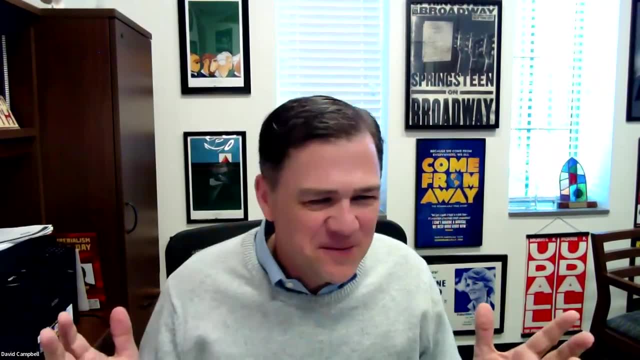 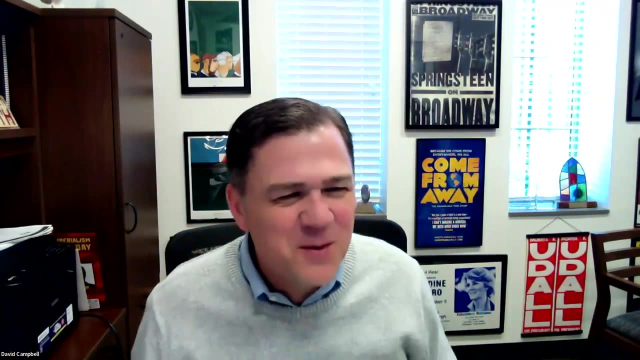 crisis. It is free to the world for roughly the next month or so. We encourage you all to check it out And again, don't just download it for the sake of downloading it, but read it, engage with it. Please use it as a. we want it to be a force multiplier in the world of civic education. So 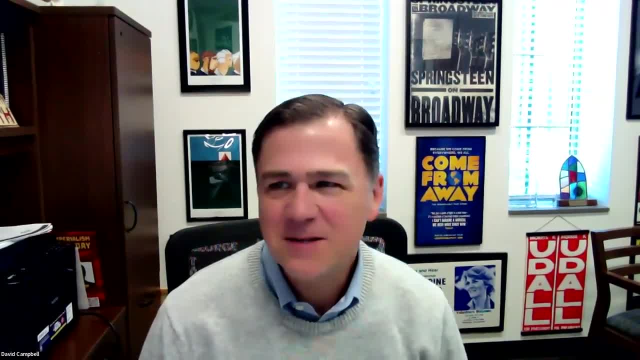 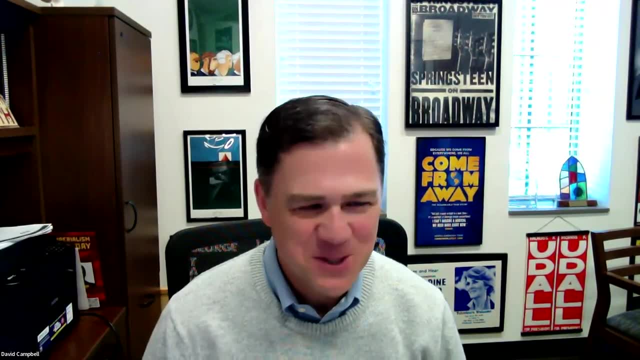 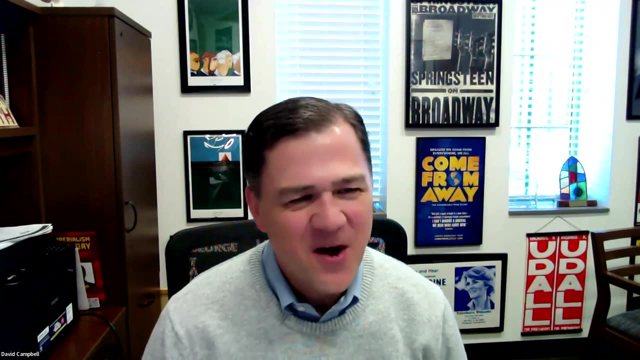 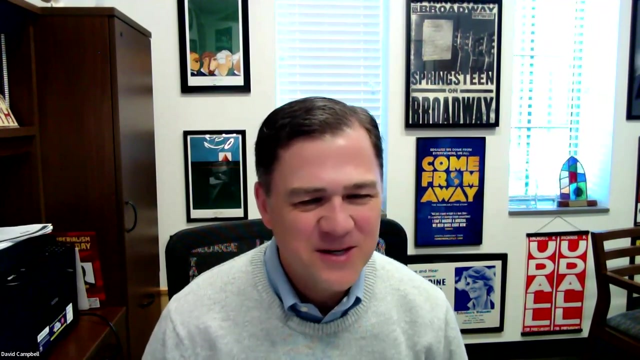 hopefully there'll be further conversations about it. Let me also take a moment and thank all of our panelists. I am grateful for their time across many time zones, that they have taken their time to participate with us, And let me thank all of you who joined us on the webinar. We had a fantastic response to this, which I think is an.